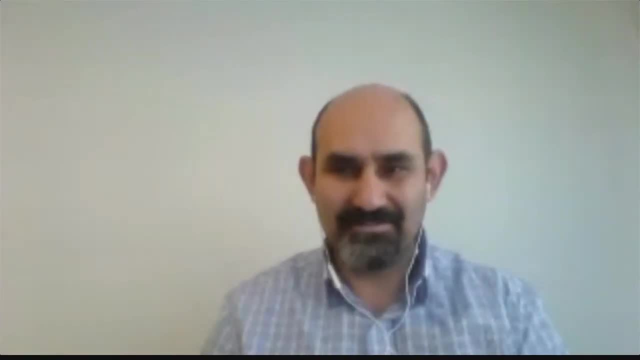 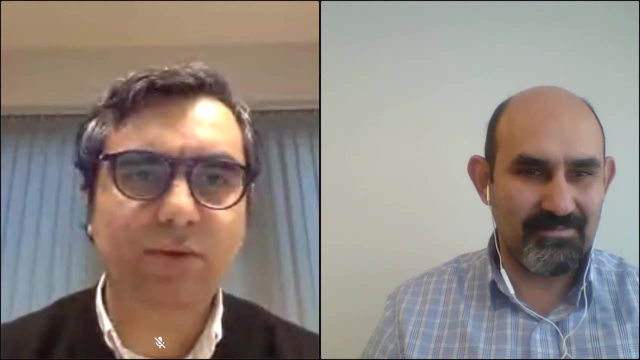 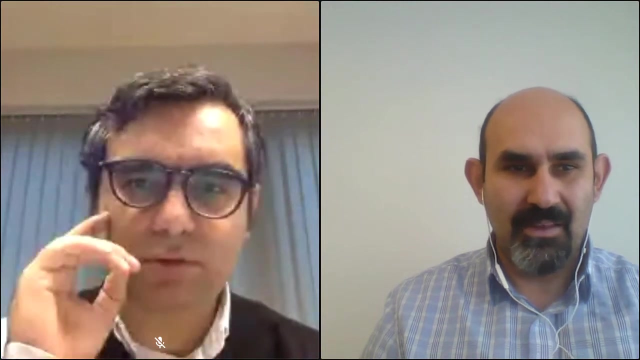 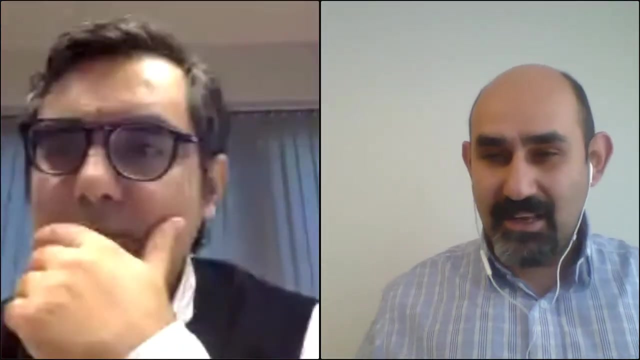 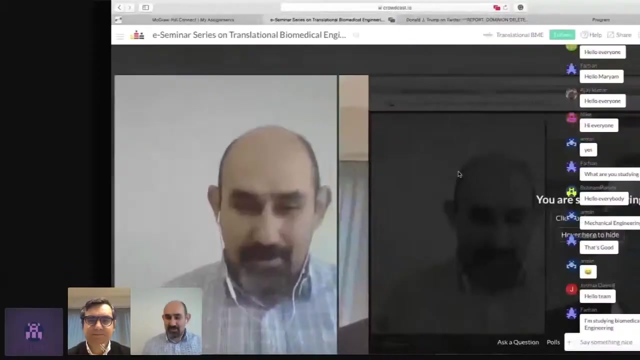 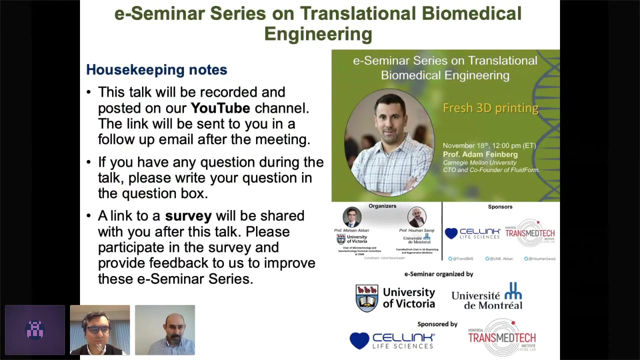 Thank you, Thank you, Thank you. Okay, So maybe we can start our housekeeping notes. Hello everybody, Thanks for joining us today. We're going to get started in about 15 minutes. Okay, Let's begin as usual, we start with some housekeeping notes and then we have the presentation of our our 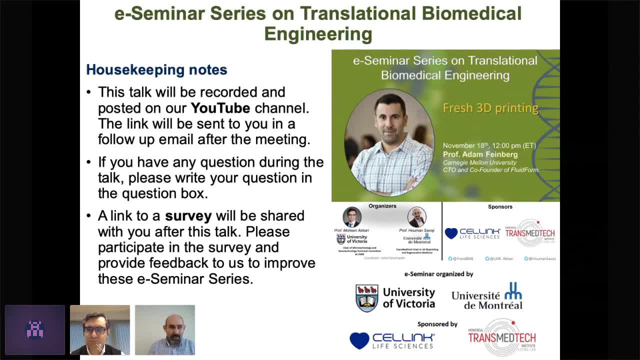 speaker, dr Feinberg. so today we are very pleased to have a professor Feinberg from Carnegie Mellon University. he's talking about the first easy by printing, and I see that the title here is not that correct, but we have the title that dr Feinberg will share with us, so this talk will be recorded. 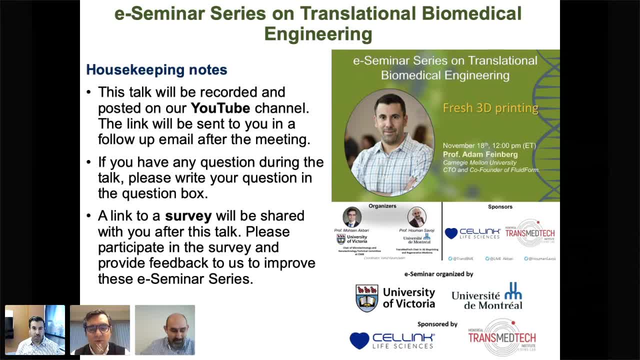 dr Feinberg give us permission to to post this talk on YouTube channel. and then we have also Q&A box. as always, you can put your questions during the talk in the Q&A box and the. and also there is a poll section on the bottom of your screen so you can take the poll to, kind of. 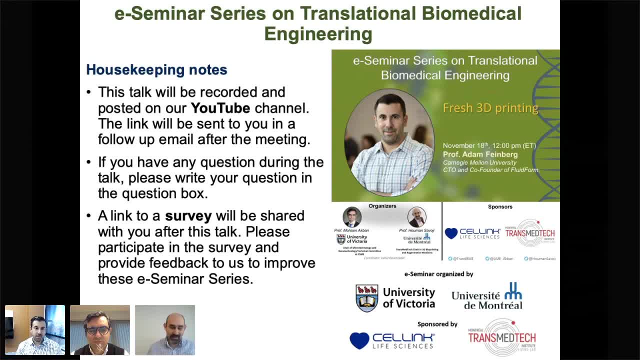 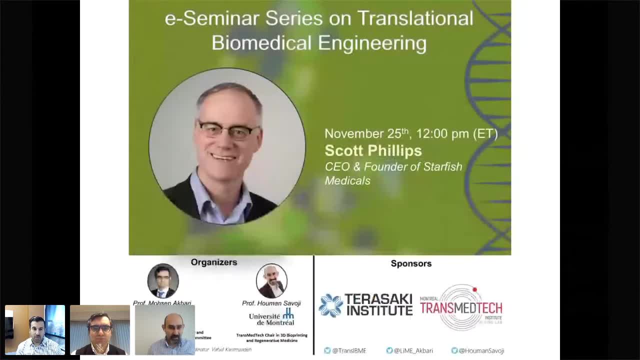 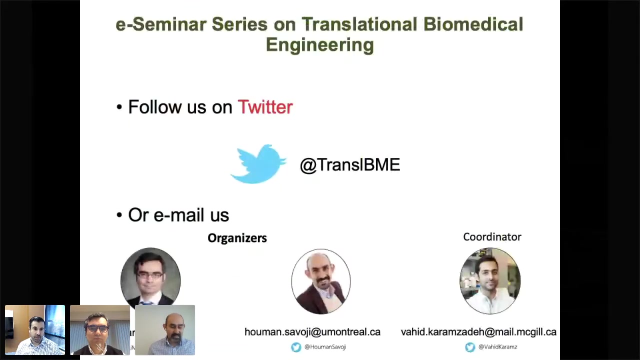 you know, give us feedback to improve the quality of the seminars. so by that, as always also, I mean, and our next seminar is gonna be, it's got Mr Scott Phillips, from CEO and founder of starfish medical, and he will share with us the story of, you know, starting office, the starfish biomedical companies and and next the next, 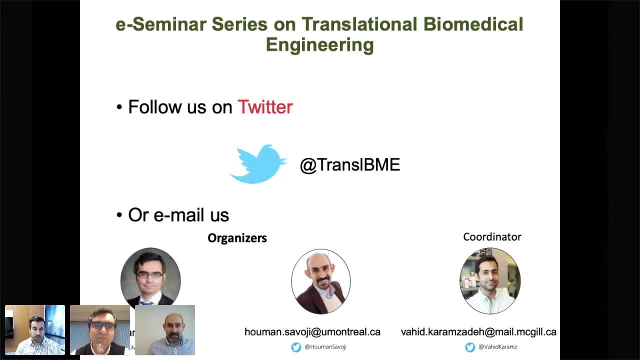 Wednesday at noon and then, if you have any questions or concerns, we want to get any updated. you know information about our upcoming seminars. follow our. follow us on the, on the, on Twitter, and also we can contact the team through wwwstarfishmediacom. see you in the next one. 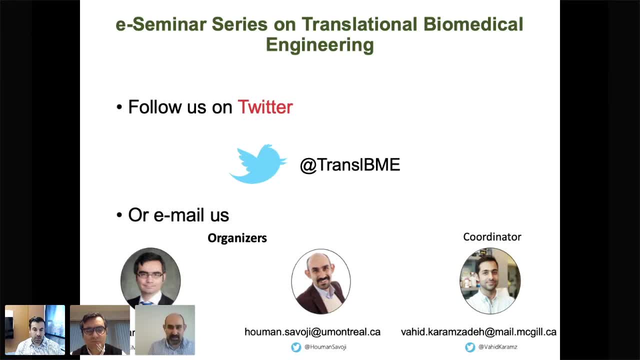 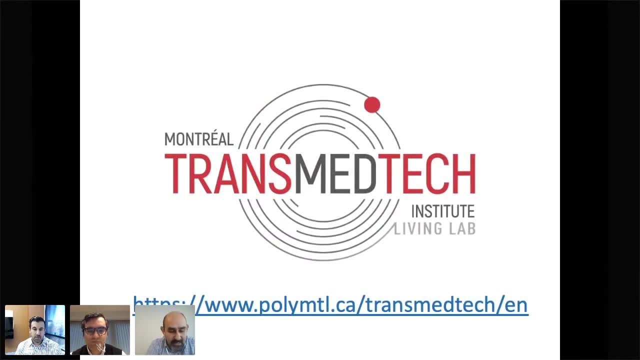 Dr Achbari, myself and our coordinator Vahid. As always, we cannot run these seminars without the help of our sponsors, our continuous sponsor, Montreal Transmedic Institute, which aims to support the accelerated development of next-generation medical technologies. 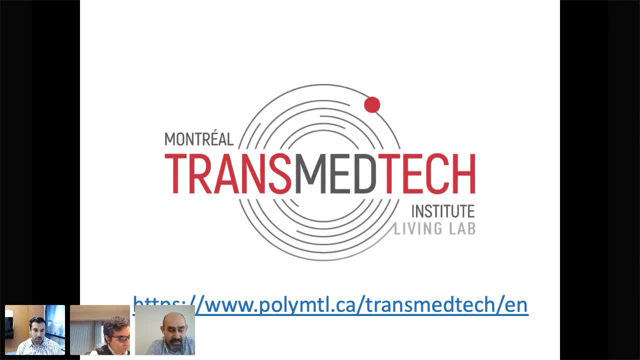 applied to three broad categories of disease, for example, cardiovascular, neuromuscular, skeletal and cancer, in order to facilitate their implementation in the health system. And also they aim to train the next generation of medical technology professionals and make the innovation in life sciences. 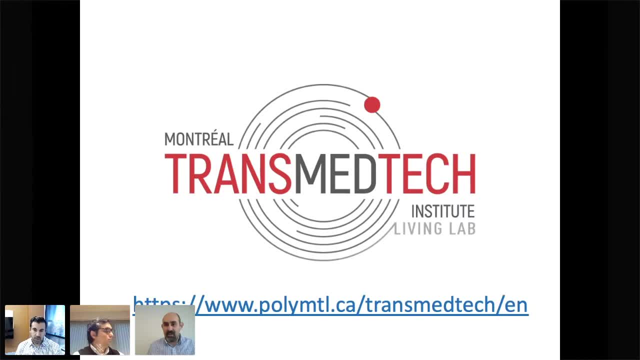 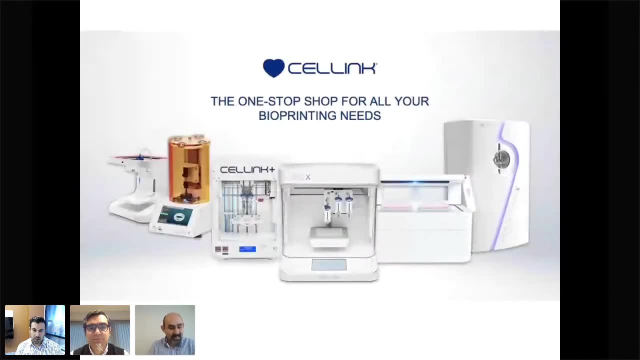 and engineering a source of wealth for society. We also would like to thank the sponsorship from Cell Inc Company. Cell Inc is creating the future of medicine by providing technologies, products and services to create, understand and master biology, While aiming to create the future of medicine. 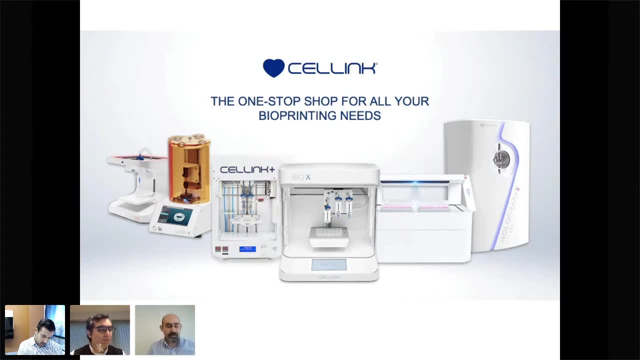 Cell Inc has focused on three application areas that are essential to cell culturing: bioprinting, analysis and liquid handling- bioprocessing. So, with the combination of persistent passion and innovation, Cell Inc catalyzed, accelerated the genesis of the bioprinting industry. 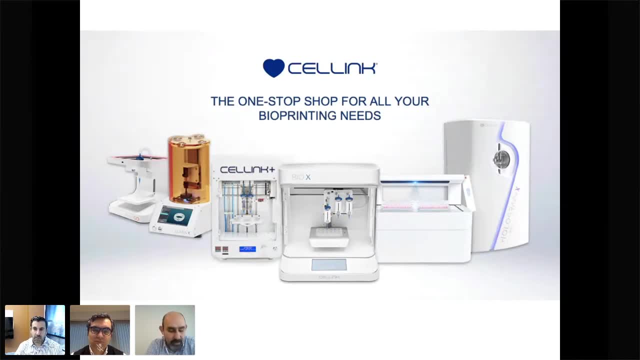 by bringing bioprinting technologies from the lab to the clinic with unprecedented speed. In doing so, Cell Inc has transferred its technology into a globally recognized pioneer of the 3D cell cultivation system in pharmaceutical research and drug development. We thank Cell Inc and TransmitTech Institute. 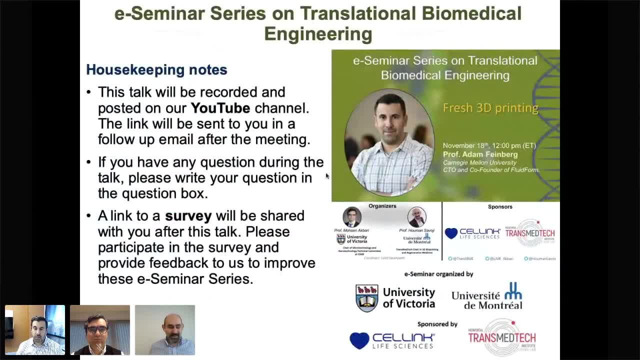 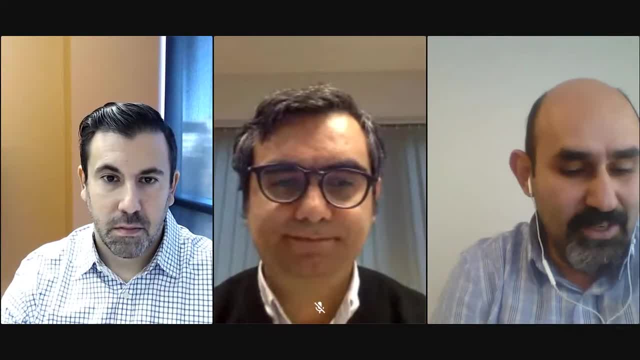 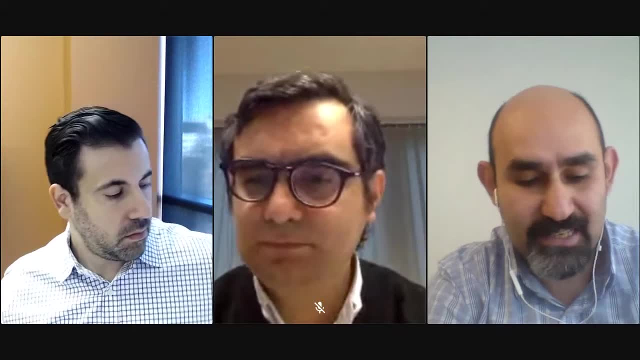 And by that I would like to introduce our speaker, Professor Feinberg from Karno-Ferrer University. Dr Feinberg is a professor in the Department of Biomedical Engineering and Materials Science and Engineering at Carnegie Mellon University. He is also the principal. 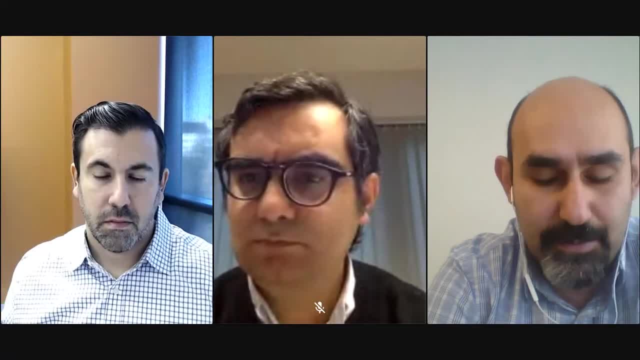 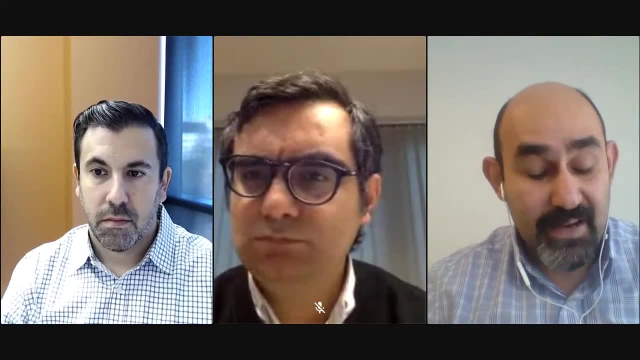 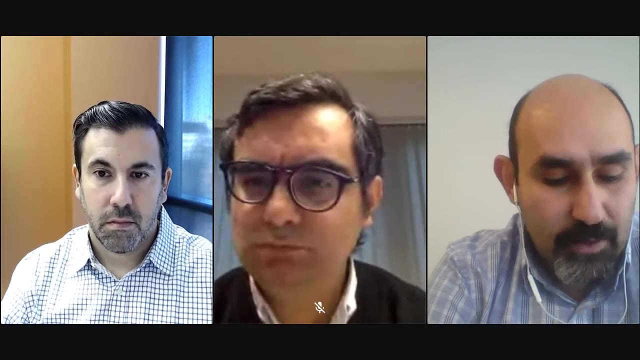 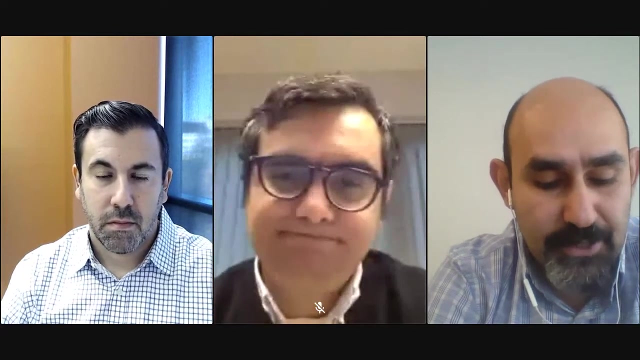 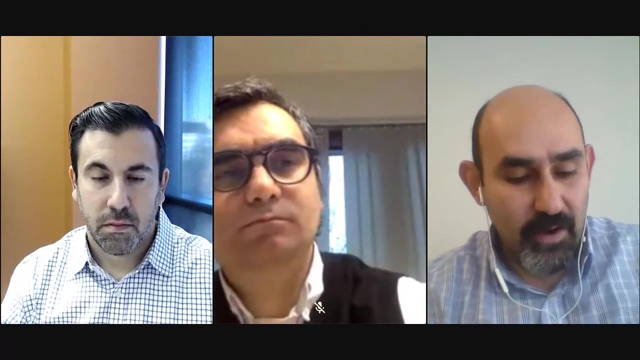 investigator of the Interactive Biomaterials Anthropology group. This group develops materials-based engineering strategies to control the cell organizations and assembly of various cell types into tissues. The goal is to understand the emergence of high-order functions in biological systems, especially in ophthalmic, neuromuscular and cardiovascular systems. Current research. 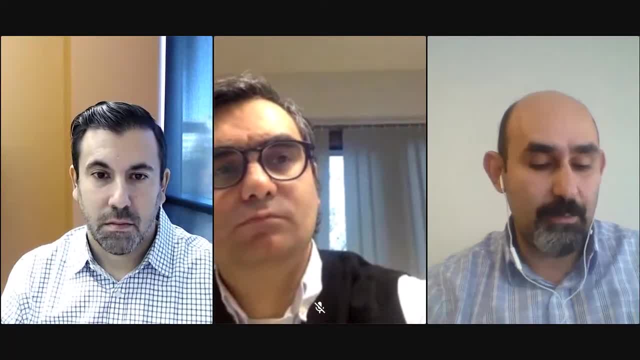 projects in his lab include biomechanics and econobiology and biochemical engineering. First-class research projects include biomechanics and econobiology. Second-class research projects include biomechanics and econobiology. Third-class research projects include biochemical engineering. 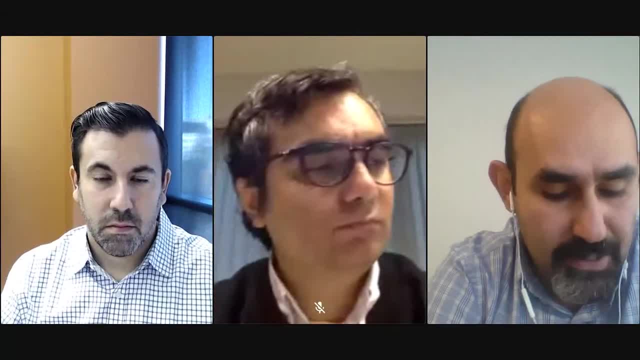 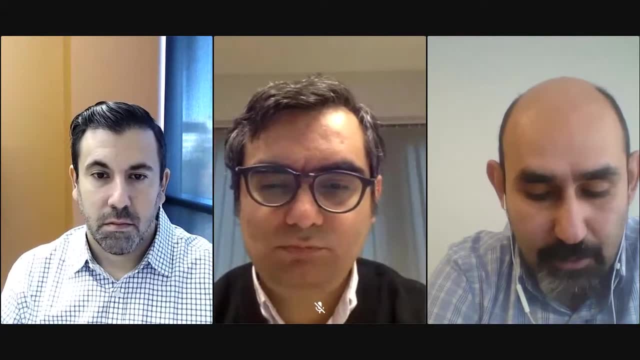 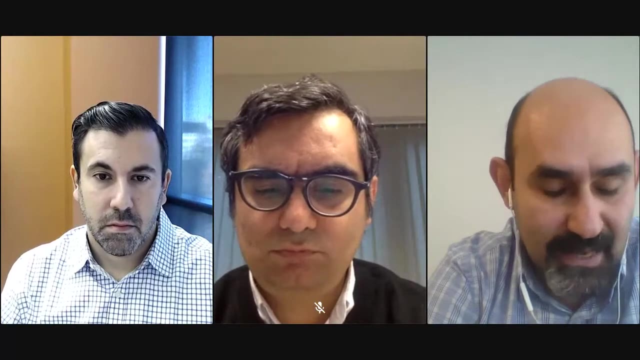 of fibrinating laminin collagen nanofibers. development of new methods for fabricating ECM scaffolds, engineered basement membranes for regeneration of the cornea, endothelium and cardiac tissue. engineering using 3D-structured ECM scaffolds, 3D bioprinting and advanced wire fabrication approaches. 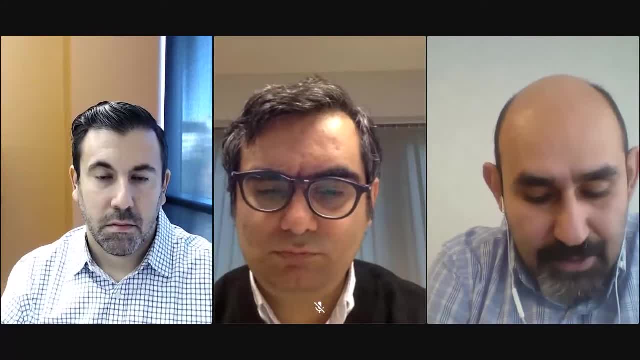 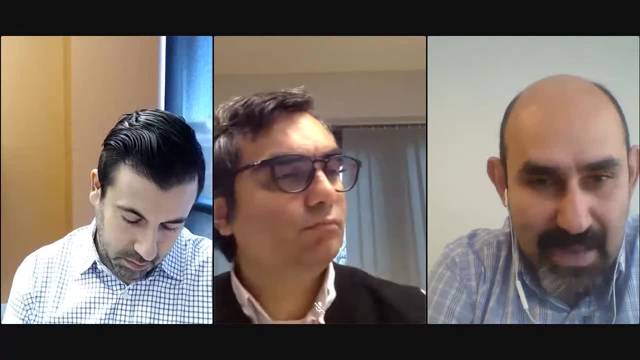 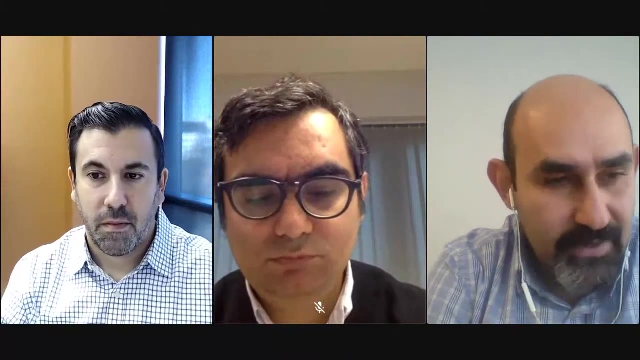 Dr Feinberg and his bachelor in material science and engineering, with an option in bioengineering, from Cornell University, followed by his master and PhD in biomedical engineering from the University of Florida. He completed his postdoctoral training at Harvard University in the School of Engineering and Applied Sciences. 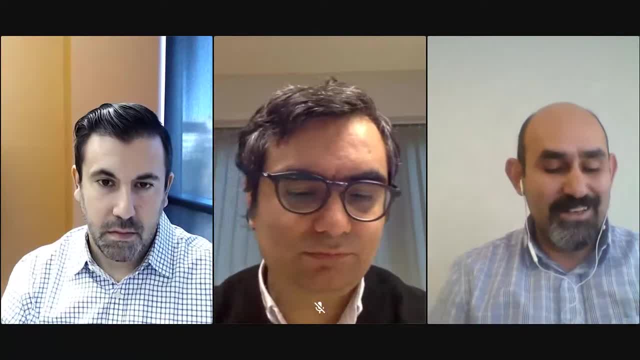 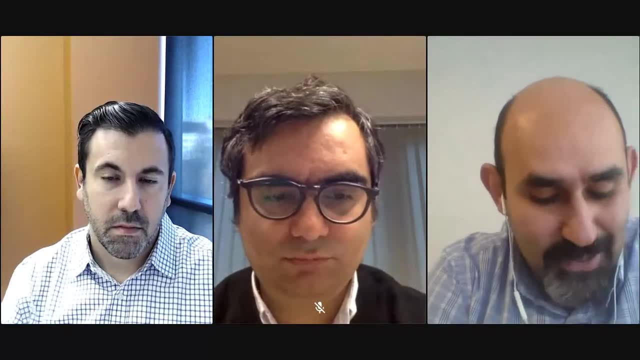 before he moved to Pittsburgh Most recently, Dr Feinberg was the recipient of many prestigious awards, including National Institutes of Health and Human Services. National Institutes of Health and Human Services Institute of Health Director's New Innovator Award in 2012,. 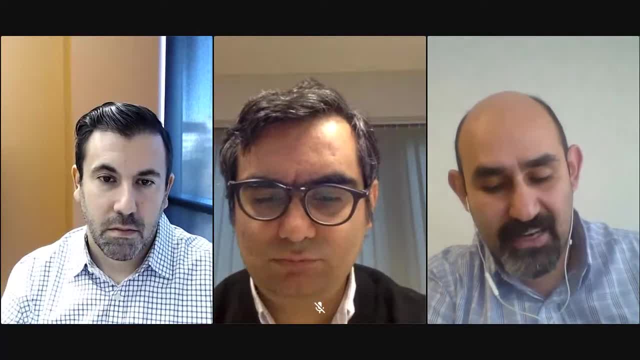 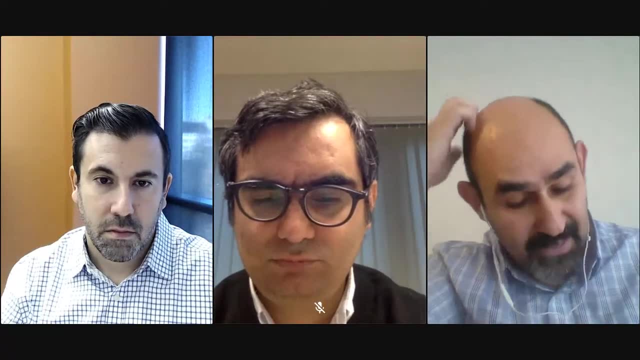 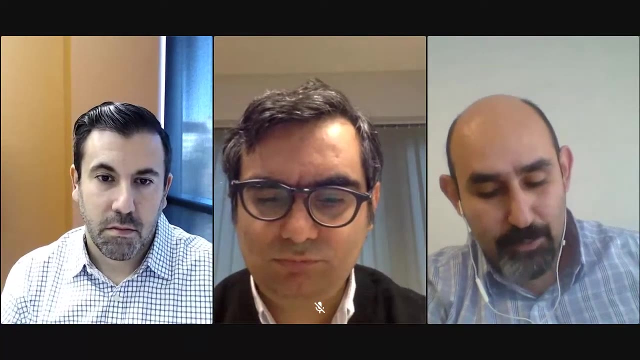 George Palman, Ladd Faculty Research Award, Carnegie Institute of Technology 2013, and National Science Foundation Carrier Award 2015.. And also Arthur Hammerschlag, Carrier Development Profession Professor. she's 27.. So Dr Feinberg currently holds more than. 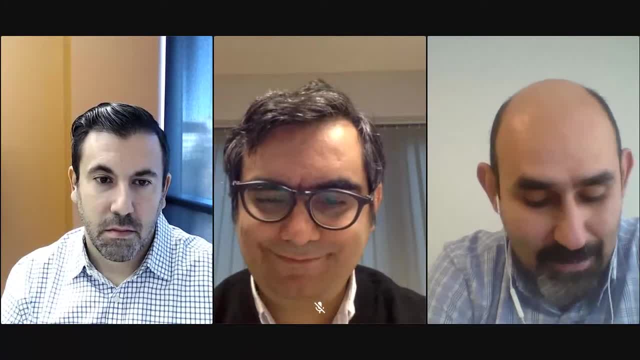 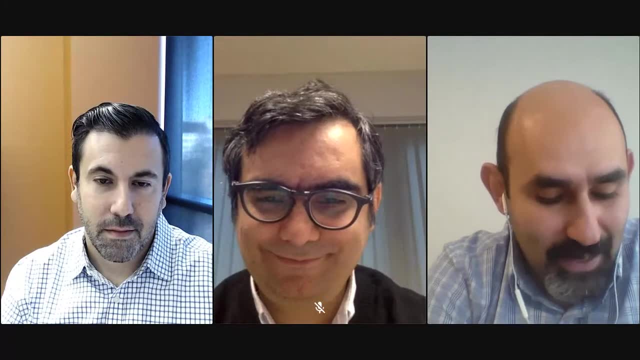 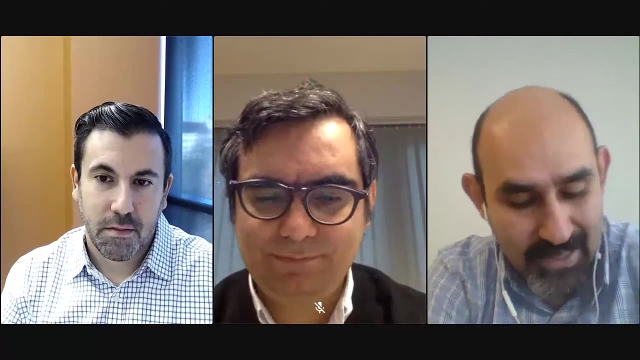 20 patents and patent applications and is a member of the Materials Research Society, American Chemical Society, Society for Human Materials, Bio-Physical Society, Biomedical Engineering Society and the American Heart Association, among others. He's also a co-founder and CTO of Floyd Forge Company. 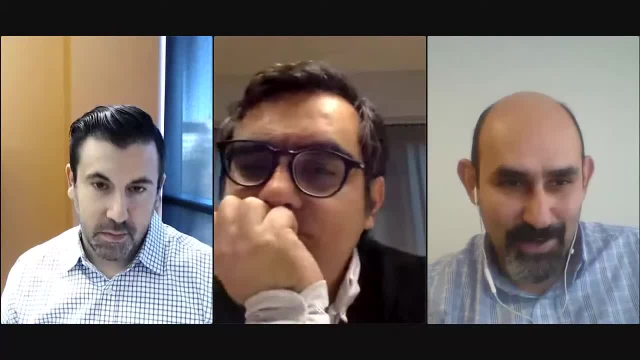 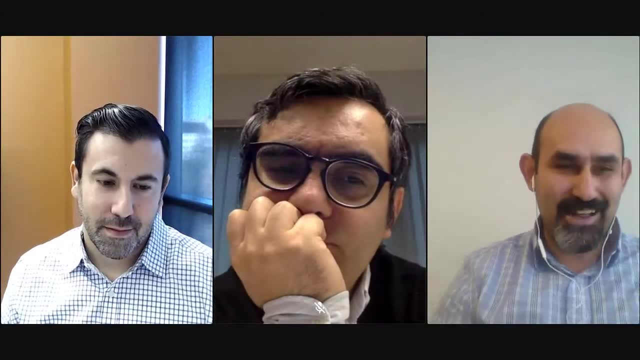 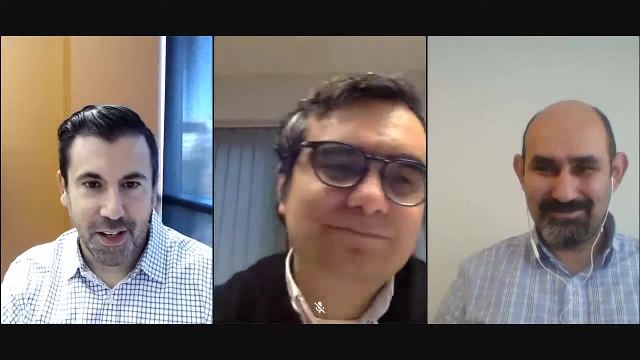 a startup focused on soft materials and 3D bioprinting. By that, I would like to invite Dr Feinberg to share his screen, and the virtual floor is yours, Dr Feinberg. All right? Well, thank you, Dr Agbari and Dr Spoggi. 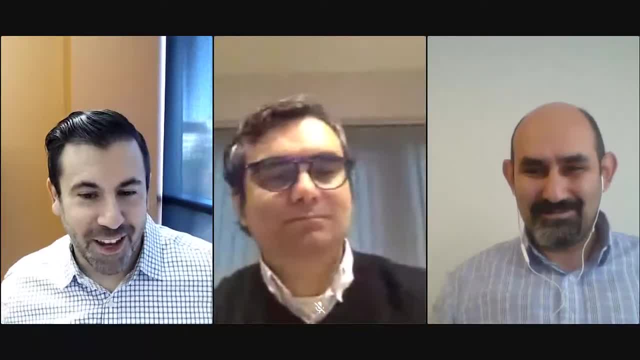 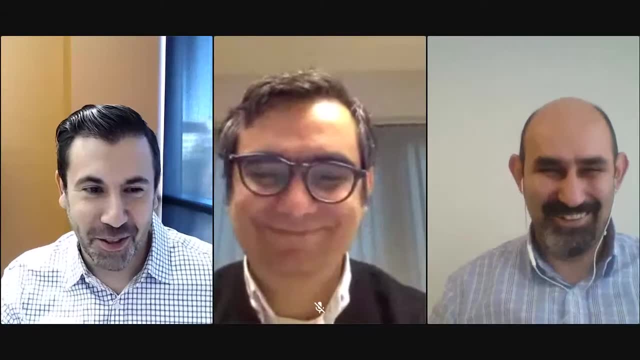 for the invitation to speak today. I really, really appreciate it. Thanks for that really kind introduction. You reminded me of a few things I'd even forgotten at this point, so that's always good to be reminded. Let me get the screen share up and running. 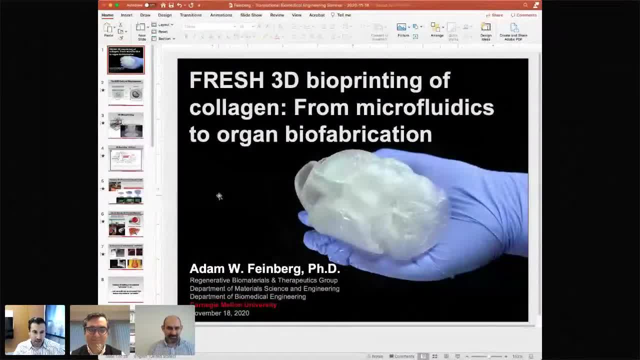 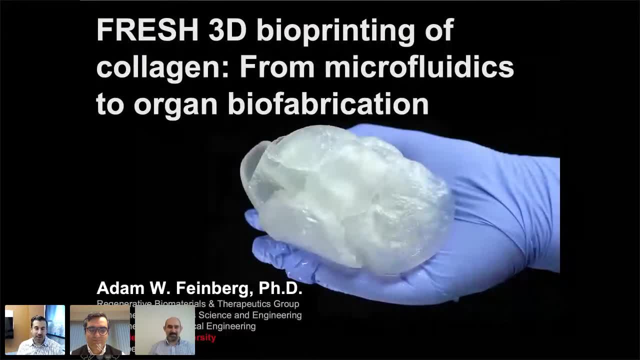 Excellent, Yeah, You see, Perfect, All right. Well, I really appreciate the opportunity to speak with you all today and share some of the work we've been doing in my lab at Carnegie Mellon University in Pittsburgh. We've been here about 10 years. 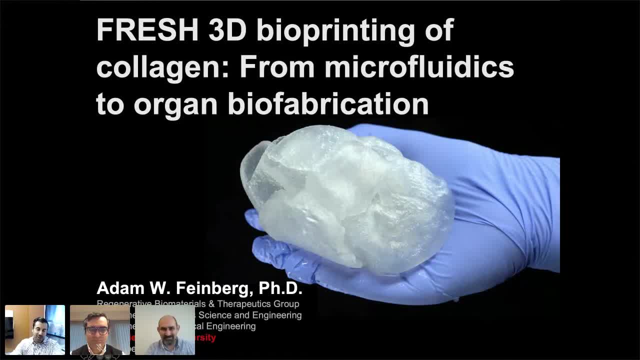 and really we focused on a lot of things. as was mentioned, kind of a key focus, Thank you, is really: how do we build tissue, How do we create environments that are instructive to cells to help guide the assembly into more complex structures? 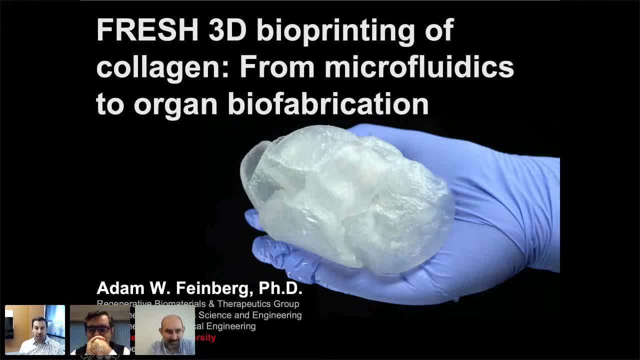 and ultimately get to the point where we can build tissues and then, one day, organs for a wide range of therapeutic applications. Fresh 3D bioprinting is one of the technologies that we've developed To do that, which I'll really go through in this talk. 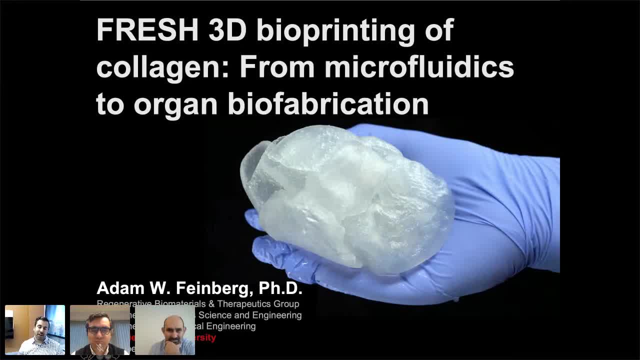 and kind of describe how we got there, where we're going and some of the new things that will be hopefully coming out soon. And then, you know, as was mentioned, we've also got a startup. I'm also CTO and co-founder of Fluidform. 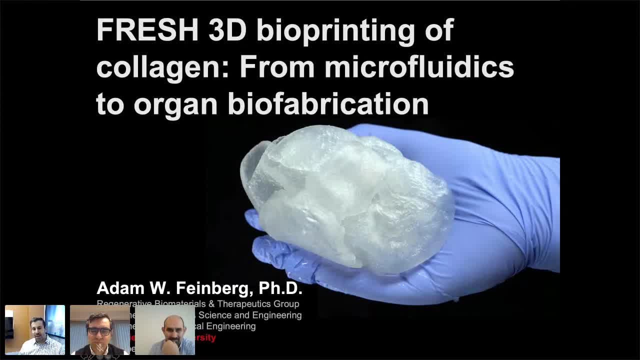 which is commercializing the technology, So that is one of my conflicts, which I'll cover at the end. So, obviously, please, you know, just want to be very transparent. So what you see on this very first slide, though, is really one of the culminations of this vision. 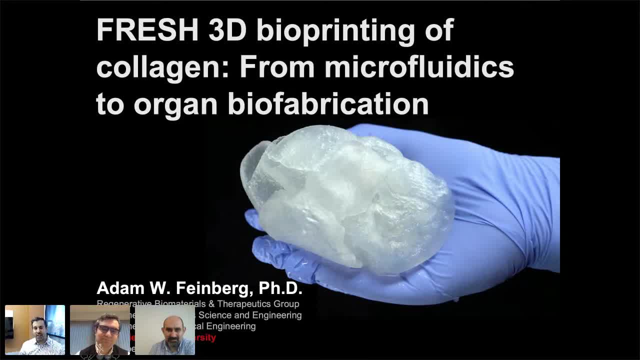 which is to be able to 3D bioprint, Bioprint biologic materials and, one day, cells at the scale of full organs, And this is a paper that just recently came out in science, or, sorry, in ACS: biomaterials, science and engineering. 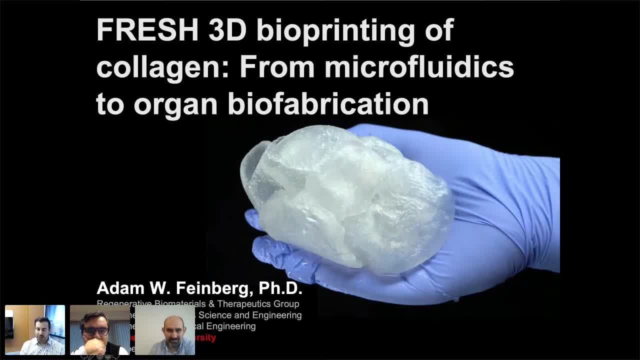 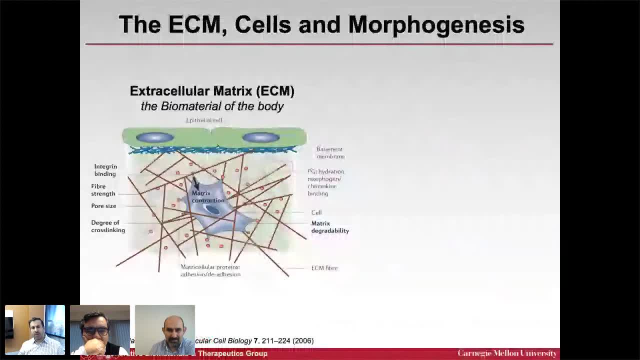 where we've actually printed an alginate heart scaffold- no cells, with scaffold at full organ scale, which I'll talk about how we got there throughout this talk. But before we do that, I kind of want to take a step back and kind of talk a little bit more. 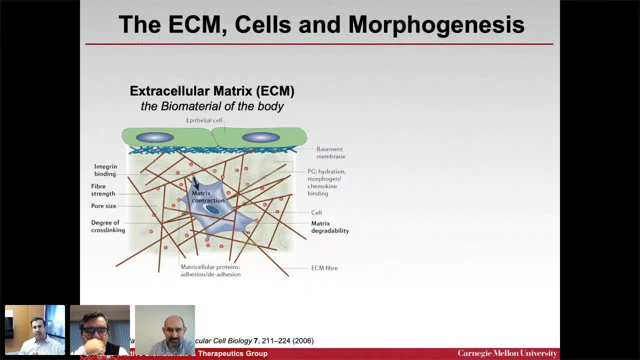 about the big picture, about what we're talking about. So we think a lot about the ECM- extracellular matrix, We think about cells and we think about morphogenesis. When you want to talk about biomaterials, what are the biomaterials of the human body? 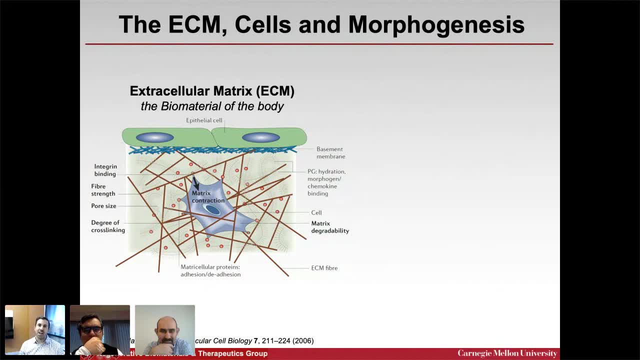 Well, for really almost every tissue and organ. that's the extracellular matrix. This is, you know, by mass, predominantly collagen, but also includes a wide range of other proteins and molecules, things like laminins and fibronectin. 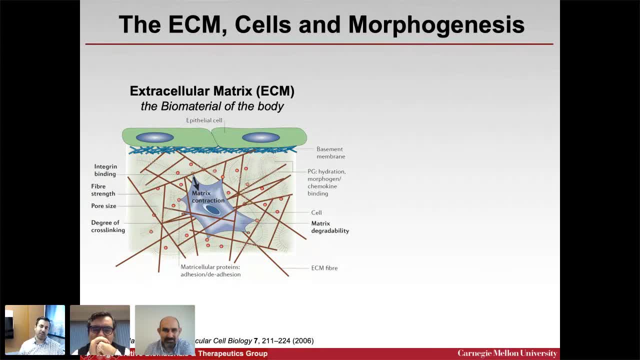 which is a very important protein. You have proteoglycans, you have things like hyaluronic acid, You have growth factors that integrate and immobilize into the ECM And cells are uniquely really built to both secrete and build the matrix and remodel that matrix. 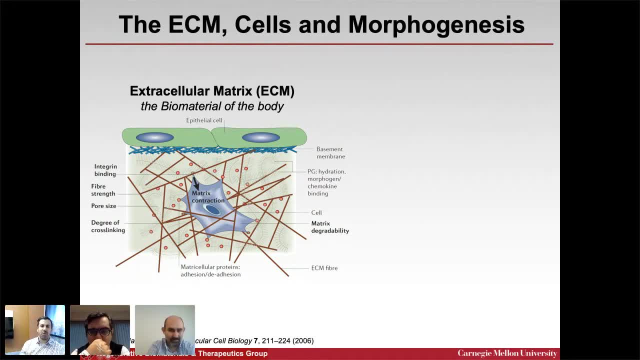 And so we really look at how can we use the extracellular matrix as a biomaterial in the same way that the body does. We feel like if we can use the extracellular matrix as a biomaterial, if we could do that, then we could really start to rebuild tissues in a way. 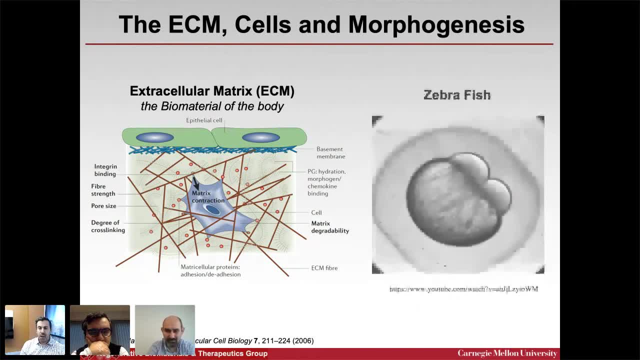 that hasn't been possible to date. We're also really inspired by embryonic development, And so this is a- this is just a phase image in the dish of a zebrafish embryo, And what you're looking at is basically that larger dark brown area shown here is the. 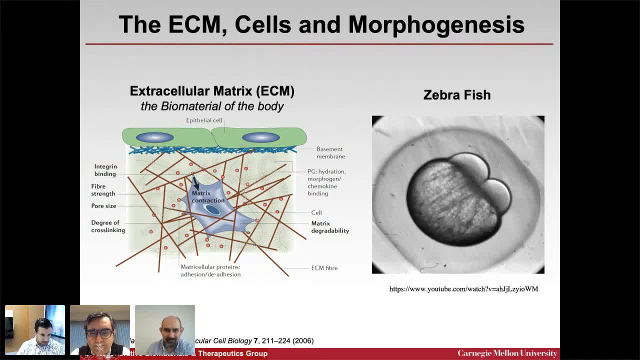 and let me see if I can't turn on the laser pointer. Yeah, so over here, this is the yolk sac, and then this is the fertilized egg after the very first binary division, And what I want to show you is the zebrafish developing over the first 24 hours. 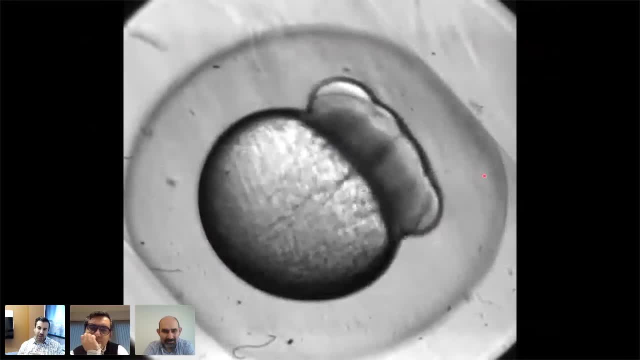 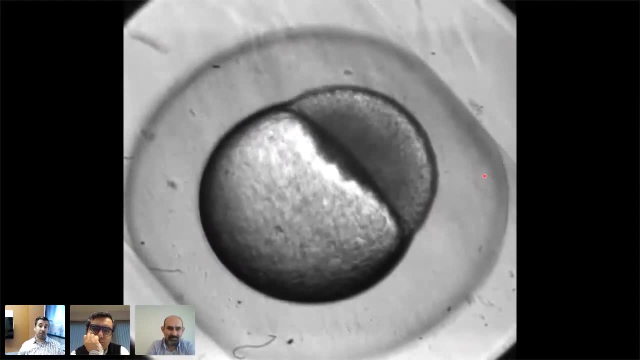 So I'll play this video. What you're seeing now is those two cells are dividing into smaller and smaller cells through binary division Because, remember, the initial fertilized egg is actually a really large cell. So the first thing you do is you get these divisions. 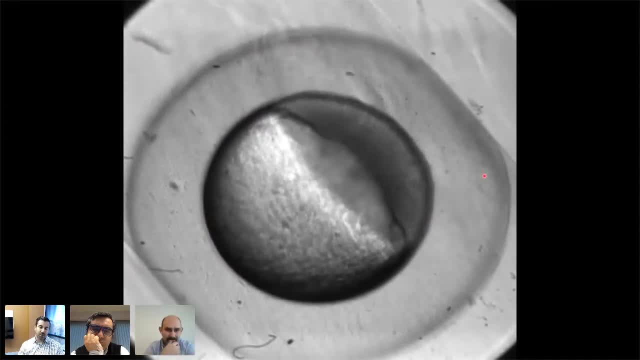 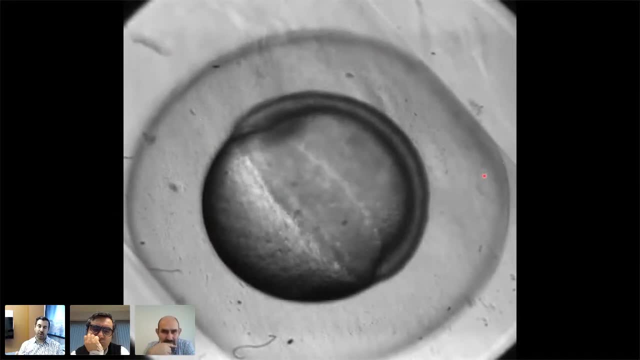 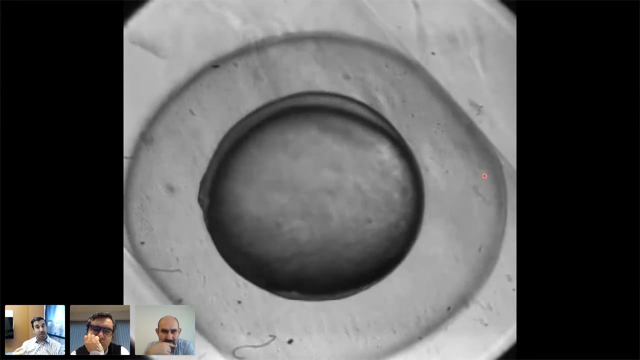 And then, as it happens, and the cells get smaller and smaller, they start to migrate around this yolk sac, almost like migrating around the outside of a balloon. Now, as they contract against the yolk sac, they generate mechanical tension and that allows the cells to start to organize and pattern into the, into, basically, the animal. 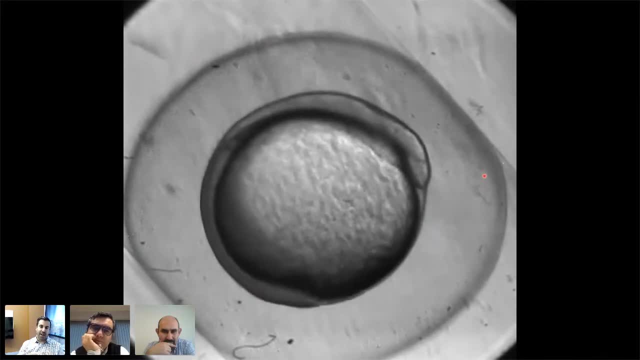 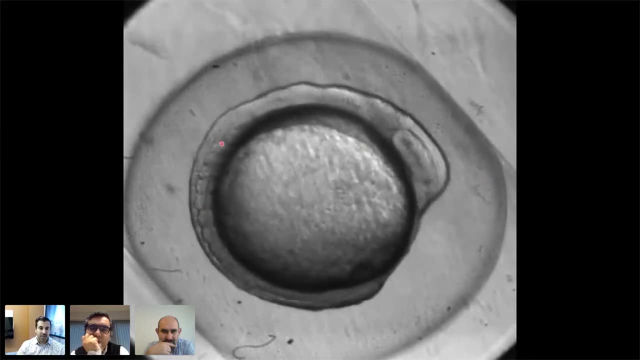 Now, as the cells are dividing, they're also specifying and differentiating, but they're also secreting and assembling the extracellular matrix at the same time, And at this point we can start to see some of the somites forming here that'll form some of the internal organs. 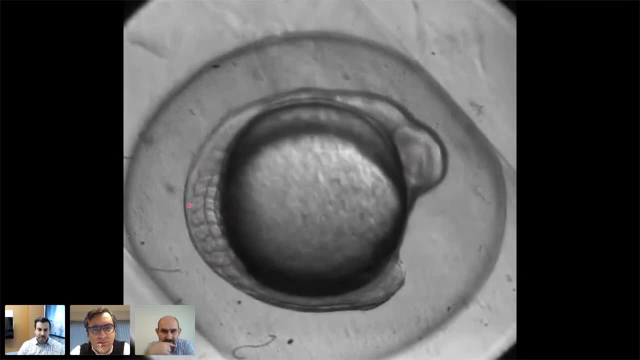 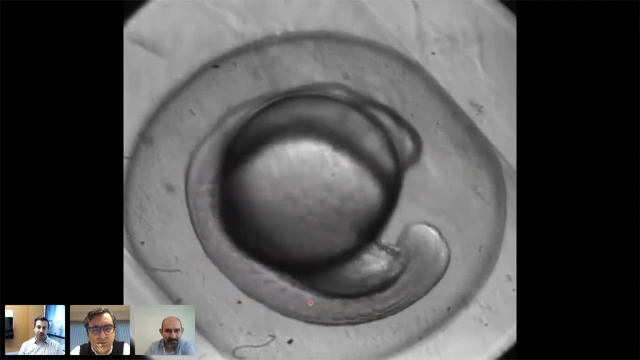 You can see the eye is quite visible here. And then, as soon as the skeletal muscle forms in the tail here, you'll actually see the animal start to twitch as that, as that muscle tissue becomes active. And so this is all happening in 24 hours. 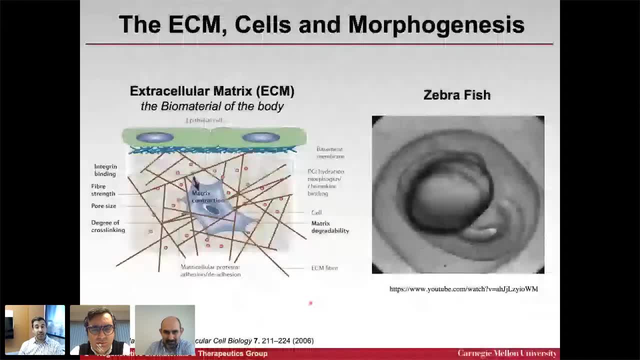 This is the. the zebrafish takes about three days to undergo development, So we can think about this as roughly like the first trimester Uh of perhaps, human development, And I think what's really interesting here is that, again, this started as a single cell. 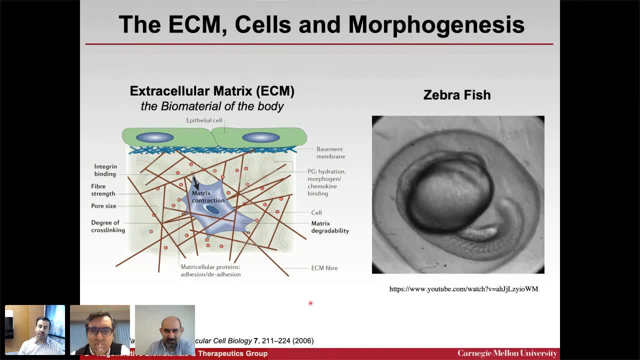 And as the cells divide and secrete matrix, they build all of the structure. This is all genetically encoded right. This entire process is based on the on the DNA that drives the instruction set for this entire process, And so what we want to do when we look at developmental biology is extract engineering design principles that we can then use outside of normal development. 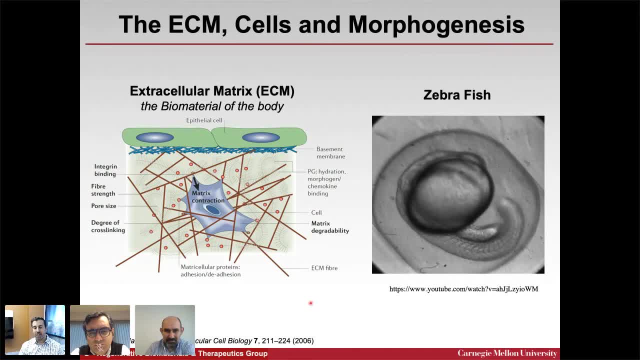 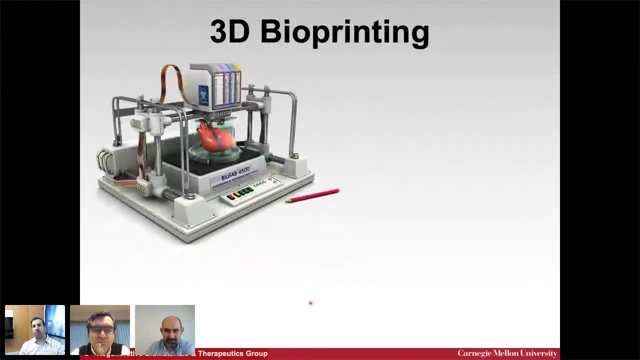 more in the synthetic context, But to build these tissues, again inspired by embryonic development. but but how do you do that? So this talk is focused on 3d bioprinting as one way to get us there, And this is actually a cartoon, an illustration, if you just Google 3d bioprinting, but it really shows the basic concept that you have basically your normal 3d printer, right? 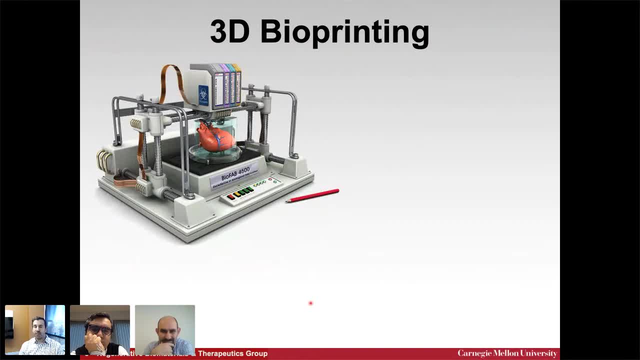 A three axis machine that has a cartridge for for cells, uh, for for biomaterials. Uh, you have a CAD design, uh, perhaps Based on MRI imaging of a person, say unique heart structure, and that you can hopefully just print, print or press print. 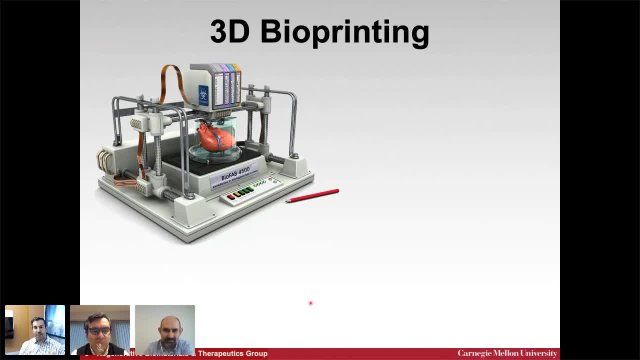 And the whole thing is printed layer by layer over time. So that's the vision, right, And the idea is that you can hopefully precisely place cells and biomaterials anywhere in 3d space exactly the way you want that to recreate the structure. 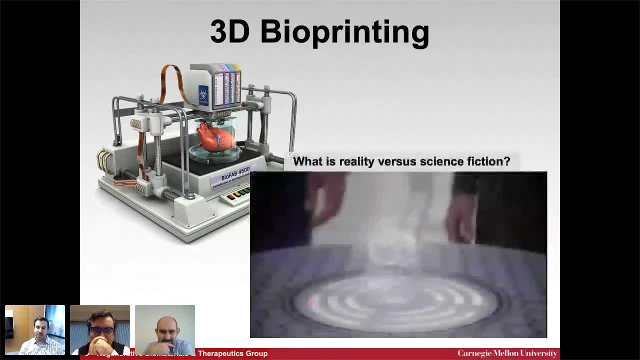 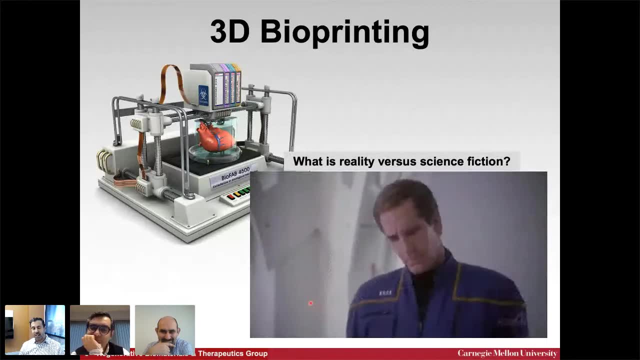 That's the vision. I think it's been a little bit overhyped, In fact. I think sometimes, um, it's hard to tell what's reality versus science fiction, So I always like to show this. This is the image of the uh, of the replicator from start from Star Trek. 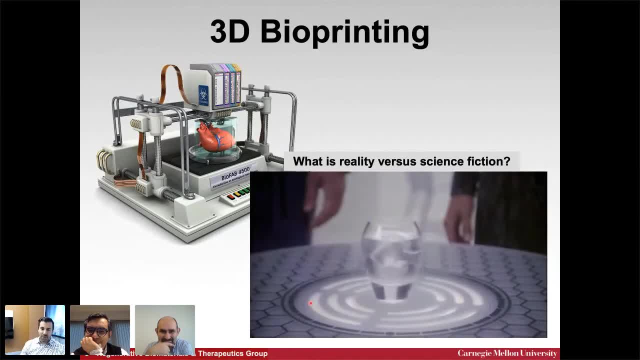 And if you remember the replicator, typically it was what they use to create food. um, uh, from, from you know, a molecules that magically assembled. But even in Star Trek, um, you very rarely saw, if ever, uh, actual living tissue being created in this process. 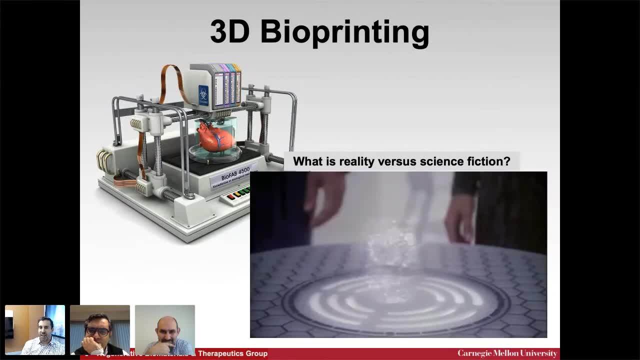 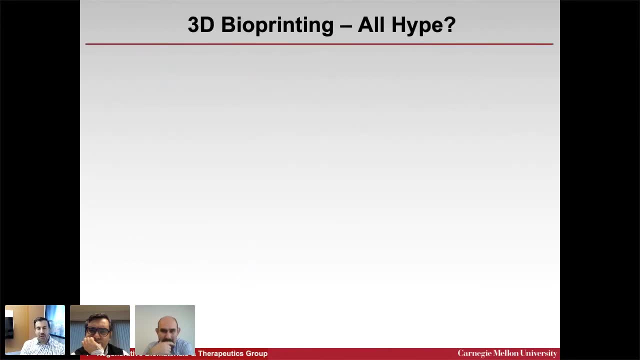 And I think that speaks to, even in science fiction, I think- what the challenges are of creating a functional living tissue. Um, I also like to uh show this: hype curves. I think it's important to understand 3d bioprinting as an emerging technology. 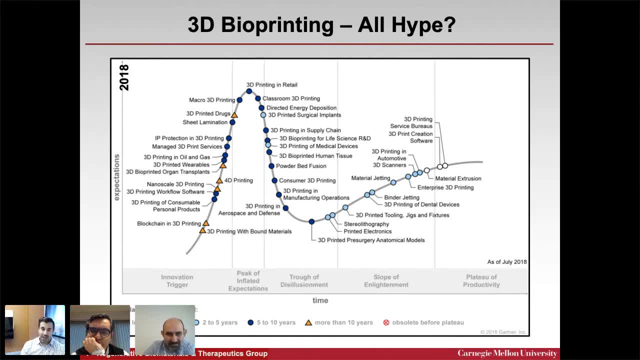 It's incredibly exciting with a tremendous potential. uh, you know otherwise we wouldn't be working on it, but we're still very much uh in a hype uh period. right, If you haven't seen these hype curves before- and this one happens to be from 2018, there's an innovation trigger. 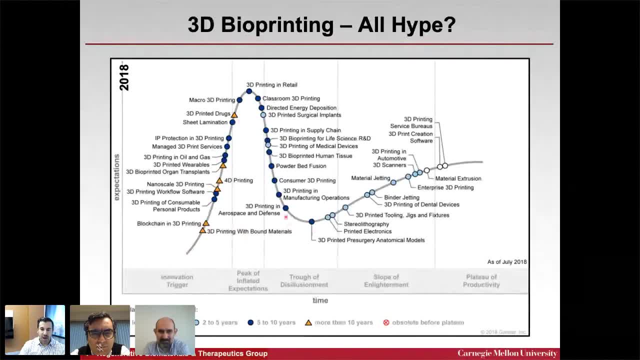 There's a peak of overinflated expectations. There's this trough of disillusionment and then a slope of enlightenment and then a plateau of productivity. So A lot of new technologies go through this, and this is all of 3d printing. 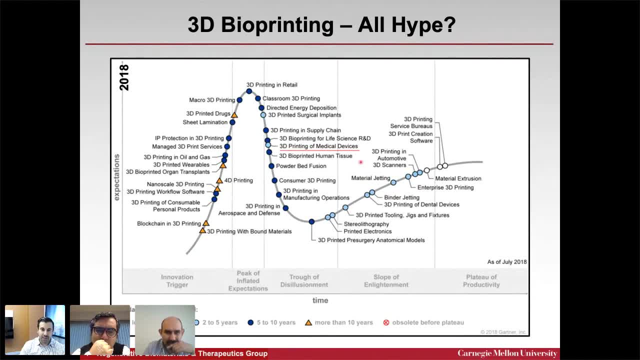 But if we look at bioprinting, you know, 3d printing of medical devices is right here. uh, still on this high curve. the 3d bioprinting for life sciences of human tissue and then also organs and transplants. 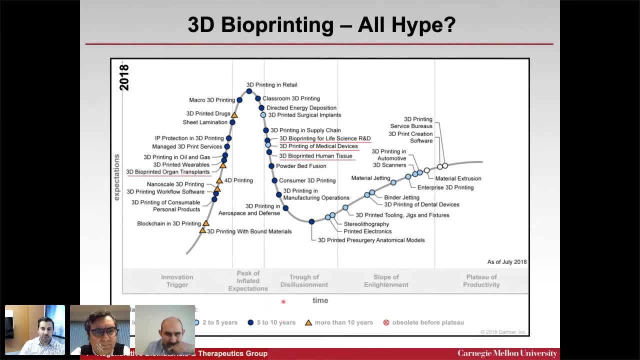 And then these little uh icons actually indicate how far off they are. So you know, medical devices- two to five years are actually already here now. So medical devices have started the transition, but things like uh, bio Printing of living tissue is still in this five to 10 year timeline and and um, bioprinted organs are are more than 10 years plus. 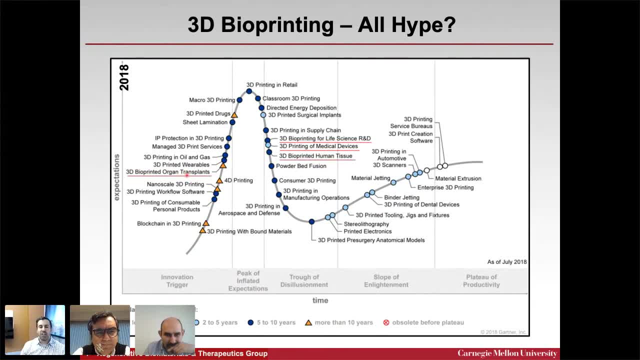 And I think this is all accurate, Um, I think it is our job as scientists in the space to be, um you know, enthusiastic champions of this technology, but also responsible in the sense of being realistic about what we can achieve when we, when we can achieve it, and really being rigorous with our scientific process. 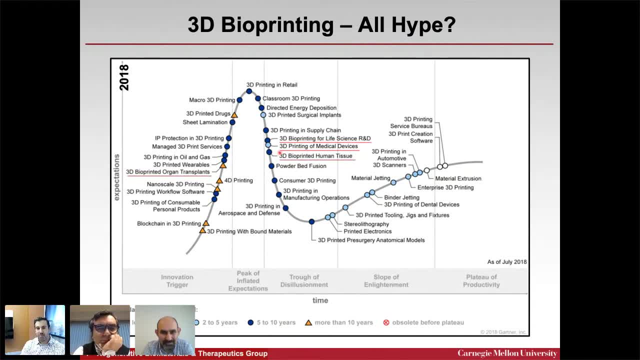 And so, uh, I just, I just like the kind of frame where I think 3d bioprinting is because uh it, it deserves all the excitement that has been kind of allowed it on, uh, on it, but it's also a technology that still needs many years of development to reach that, that promise. 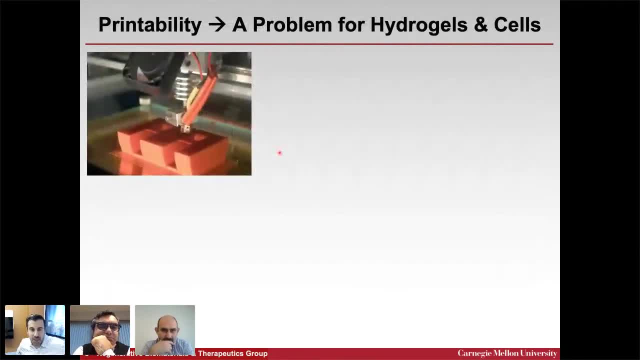 So I want to kind of get into exactly what we've been trying to do in the space of 3d bioprinting and why. and what we've really been trying to address is is: is this problem of printability specifically for hydrogels and cells? 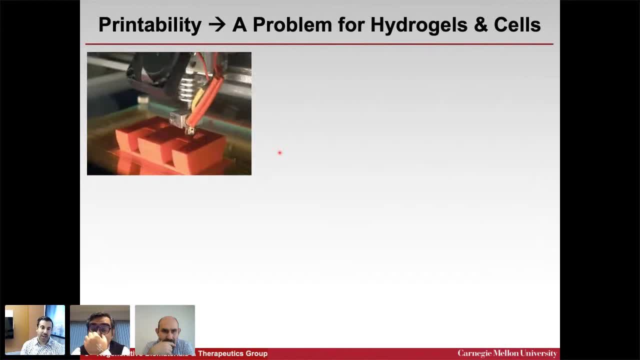 So if we look at a normal 3d printer shown here in the upper left Slide, This is your normal plastic printer that many of you are familiar with, And the reason this works is that it it obviously prints layer by layer by layer, but by extruding plastic and then letting it rapidly solidify, it becomes very rigid and solid. 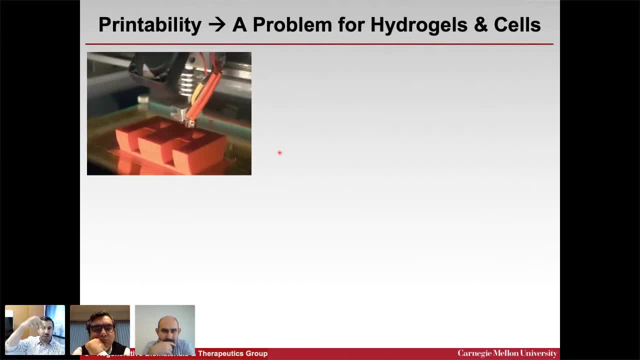 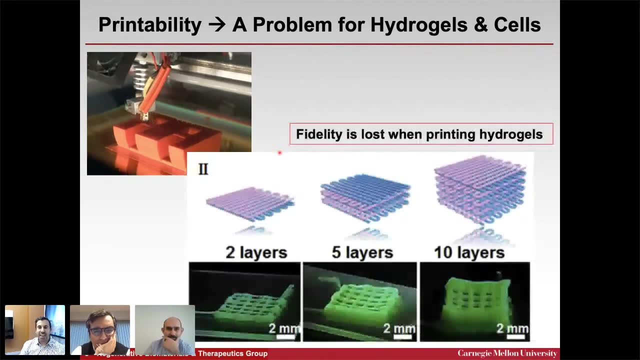 It's stable in 3d space. that makes it very straightforward to come down and put another layer on top. uh, because the layer below it is stable. Now, that is not the case with many hydrogels and cells, because these are materials that have a very low elastic. 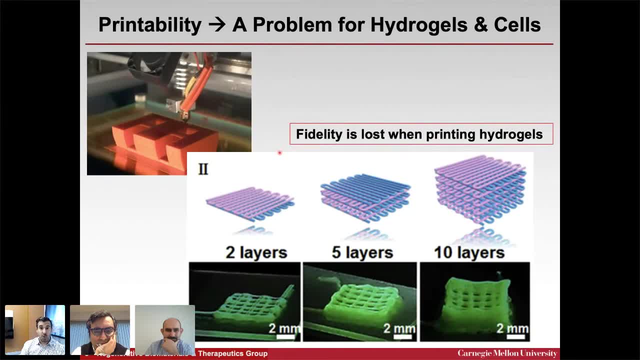 Modules, Uh, they typically are not able to support their own weight in air. and shown here is some hydrogel printing. As you try to print additional layers, uh up, uh. that is really, really difficult to do. You lose fidelity because when you put down a layer, it moves. 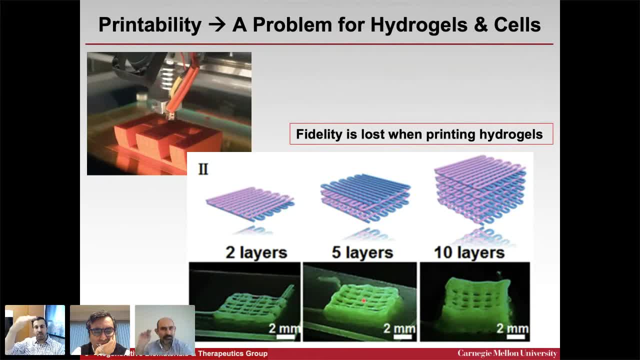 And so it's challenging them to put the next layer on top, And as you build layers, that just increases your error. If you also have living cells, they have the potential to actually move on their own too, And so that's a whole nother layer of difficulty. 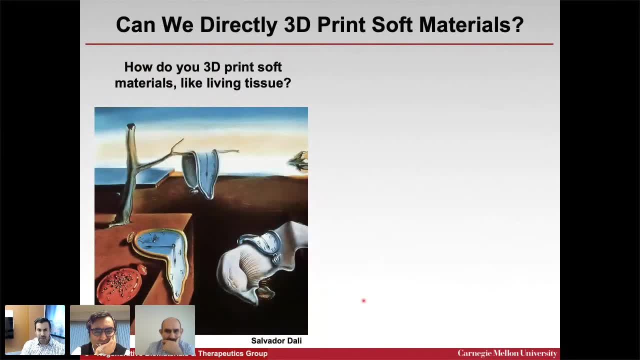 So how do we print Hydrogels And cells? Um, I like to kind of also kind of talk about this challenge with the Salvador Dali painting, which shows these kind of deformed clocks, and the problem of trying to build a complex living biologic system out of soft materials that move. 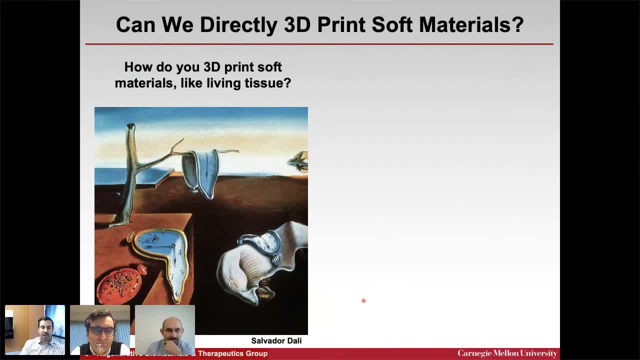 Is that you at least have to hold everything in place during the assembly process, even if that system is deformable and moves after the assembly process. So the analogy I use is: imagine you had a pocket watch that you disassembled. uh, you had all the 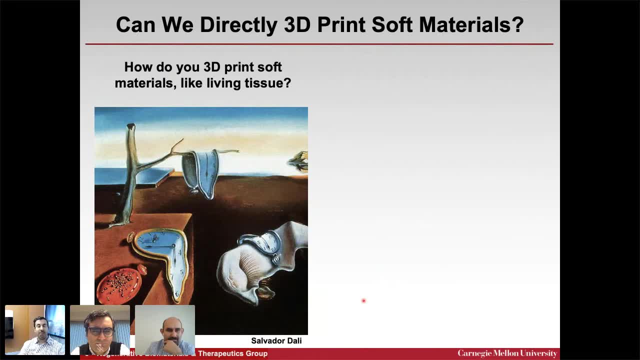 Gears and springs, uh, laying in front of you And your job was to put that pocket watch back together. I think most of us could start to figure out at least how some of those gear assemblies fit back together, uh, to rebuild that watch. probably not the whole watch, but we could understand how pieces go back together. 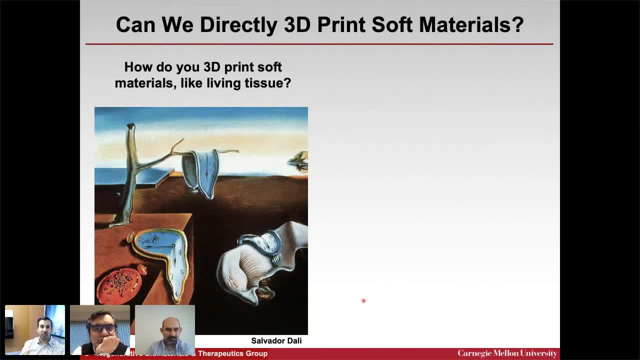 But now imagine you had to build that watch, and all those gears and springs are soft and flexible and floppy and they didn't hold their shape. How can you possibly rebuild a gear assembly with materials that don't hold their shape Right? And so, again, we're dealing with materials. 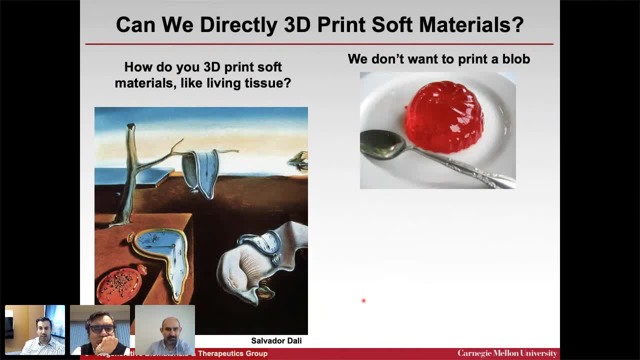 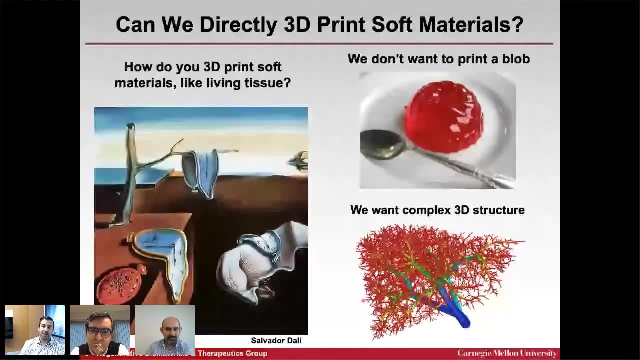 They're very much have the the mechanical properties of something like jello which is easy to make into a block or a mold. but that's not what we're trying to do. We're trying to turn it into something complex like, say this: this uh CAD model here of of liver vasculature. 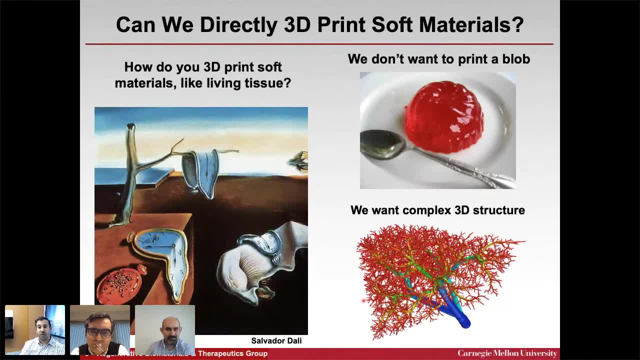 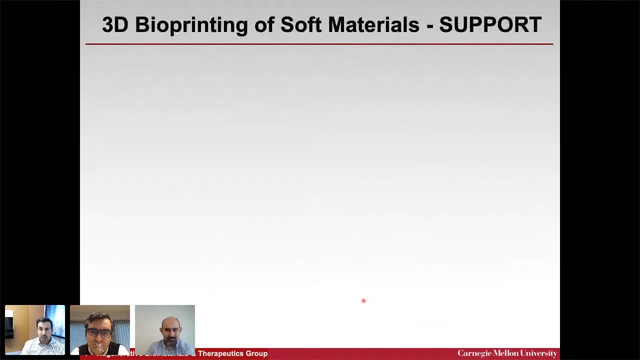 I think we can all appreciate that if we tried to make something complex like the jello mold uh into something like the liver vasculature, it would collapse under its own weight. So so how do we do that? So my lab is by no means the only ones working in this space. 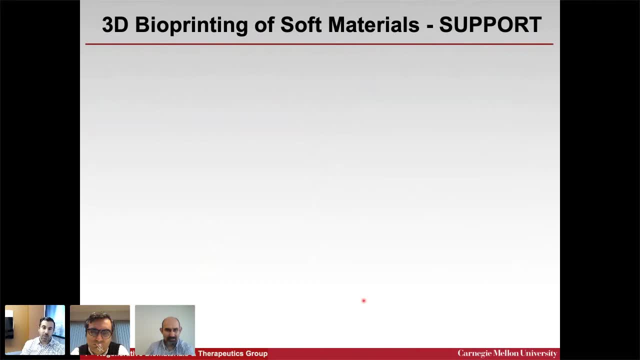 There's obviously many labs doing Amazing work really across the globe. I just got to highlight a few, obviously in the interest of time, Uh, but there's a couple of different strategies. So this is work from Tony Atala's lab at wake forest, where they're trying to print soft hydrogels. 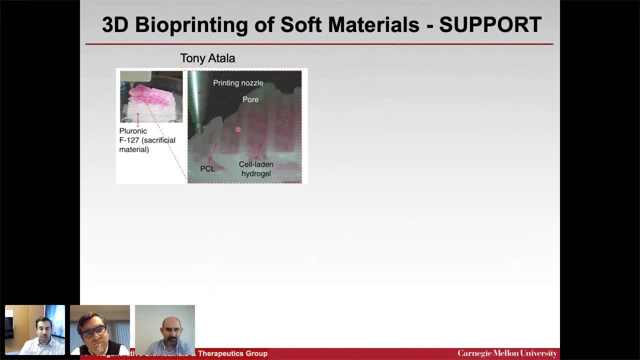 And the way they do that is they print a PCL frame shown here, kind of like the lattice you would see uh, or scaffolding Like you would see on the outside of a building as it's being constructed. that PCL lattice uh is basically provides mechanical support and the hydrogel, the cell late. 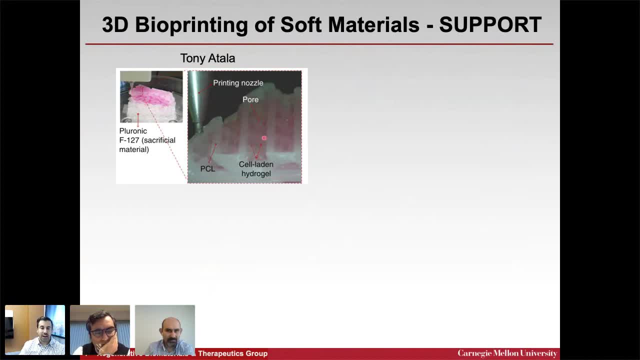 The hydrogel. It's basically extruded inside of the pores, inside of this PCL lattice, And this is one way to create a rigid support material that can hold up a softer hydrogel, And they've used this and published it in in in nature, uh uh biotechnology and other high impact journals. 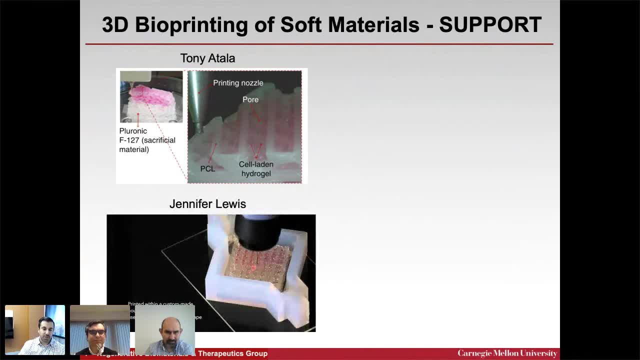 Uh, this is some work by Jennifer Lewis, who's really pioneered this approach of using a sacrificial chloronic filament uh, which is relatively straightforward to print. Uh, that's shown here, printing a large uh kind of a cube of of of this lattice structure. 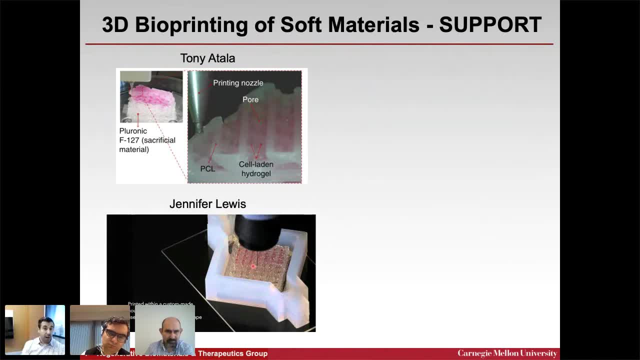 Uh, of of this lattice structure, Uh, and then they can cast a hydrogel around that And then, uh, using a, a temperature, a thermal reversibility of the fluoronics, actually wash, dissolve and wash out the fluoronics, which leaves a vassar like network inside of that hydrogel cast around it. 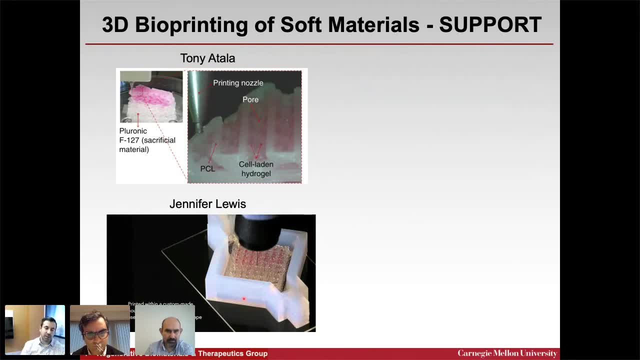 And they've really done pioneering work, creating larger, vassarized structures with this approach. Um, you know publishing, you know advanced materials and and uh, science advances in other high impact journals as well. And here's some additional work aboard. 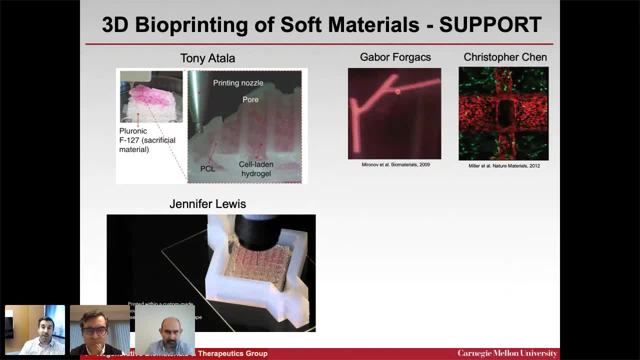 Forge acts. We've developed this cell spheroid printing. That really was the foundation of organ Nova, really the first uh, you know, uh, uh, uh, uh, large scale 3d bioprinting company. Uh, this is worked by Christopher Chen, where they had sacrificial sugar filaments, very similar in the idea to the work done by Jennifer Lewis. 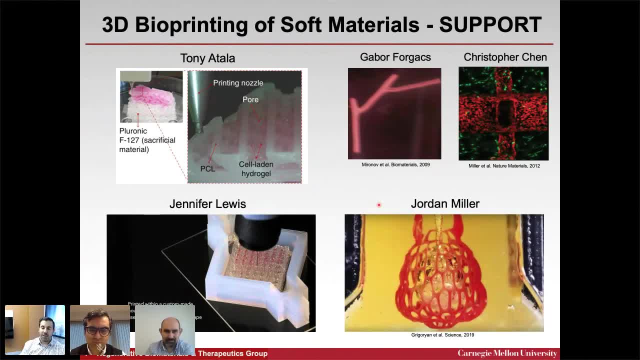 And very recently, Jordan Miller published last year in science using uh not an extrusion based technique, but a light based technique of 3d printing. uh that allowed creating a peg or a gel Uh block, but basically being able to pattern complex microfluidic networks inside, and had a very elegant example of an alveolar light structure. uh, that could do gas exchange. 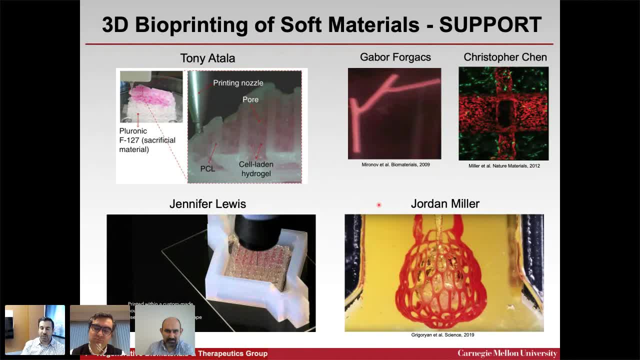 So these are all amazing examples of 3d bioprinting with soft materials, but these are all doing something slightly different than uh, than what we want to do. We wanted to be able to directly 3d bioprint the soft materials. 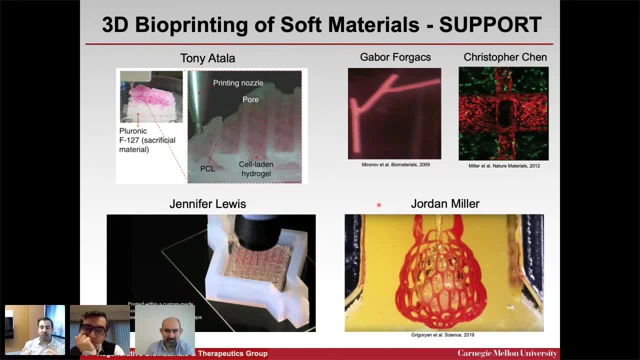 These are all kind of ways of getting around the challenge of directly printing these soft materials, Um in in different kinds of ways, right? So we really wanted to take that idea of the plastic printer. That's just directly extruding plastic. 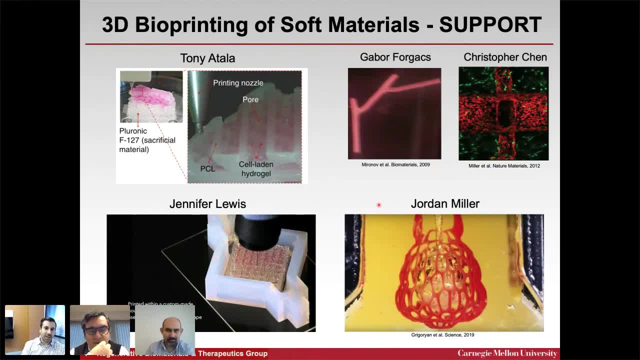 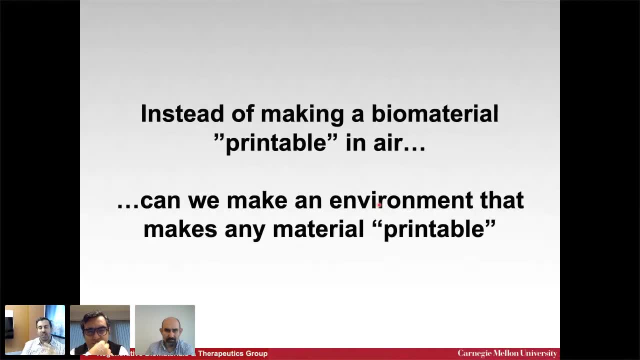 Can we do that with a hydrogel? Clearly that you can't do that in air, And so we took a different approach. So, instead of trying to make a biomaterial that's printable in air- which typically means modifying that material, making compromises- instead can we make an environment that essentially makes any material printable. 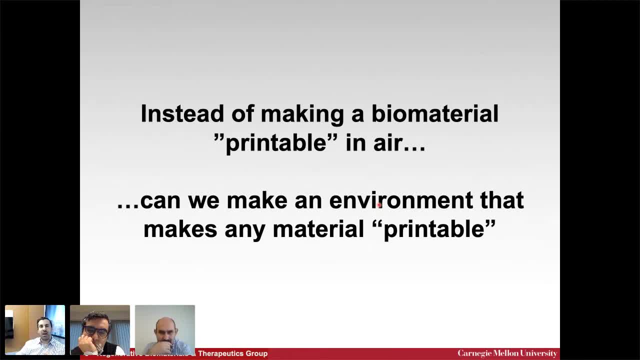 So, and another, another way of saying this is: let's decouple The printability from the biolink and put the printability into the environment, and then almost any material now becomes printable. So the way we do to do this is this: fresh 3d bioprinting. 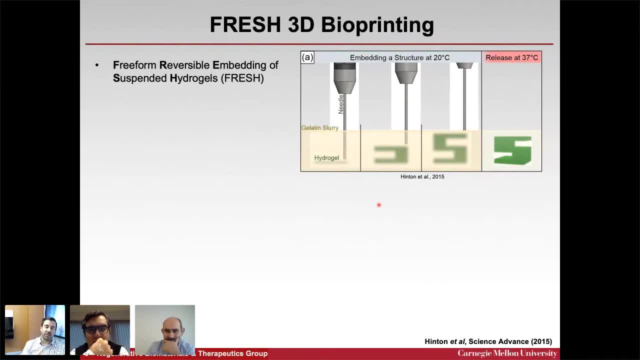 So fresh stands for free form, reversible embedding of suspended hydrogels, And really the most uh, uh kind of prolific example we have of this is using a gelatin slurry based support bath. And so if you look at this uh schematic, here we have the needle, we have a yellow to the yellow gelatin support material. here. 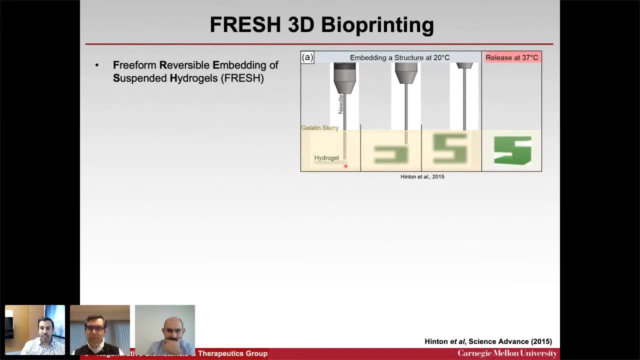 which is, Yeah, Actually a gelatin microparticle slurry. We can drop the needle inside uh and we print the second hydrogel inside of that support hydrogel. We can print the entire structure, and we do all this at room temperature and then we raise everything to body temperature to release the print. 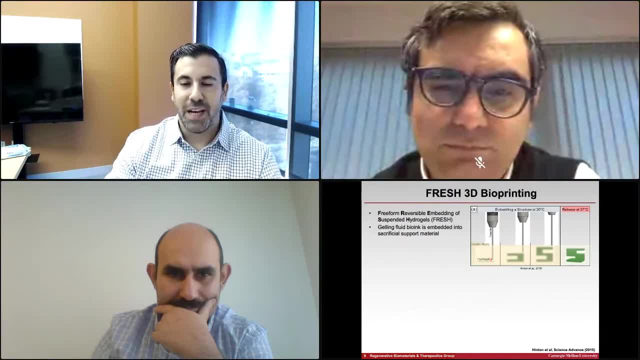 Right. So that means the gelling fluid biolink is embedded in our sacrificial material during the printing. The bath that we print into actually acts as a yield stress fluid, So it transitions from solid to liquid like that allows the needle to move through easily. 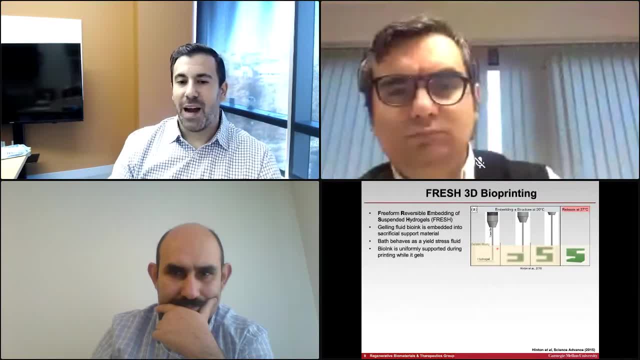 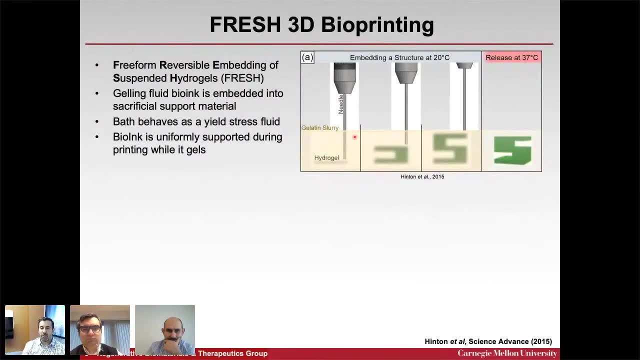 But whatever we print to stay embedded in place, this biolink is now uniformly supported during printing while it gels, And very often we have a cross linker in the support bath that helps drive that gelation process, And then, when we're done, we simply melt the support bath again at a physiologic temperature and releases whatever we printed. 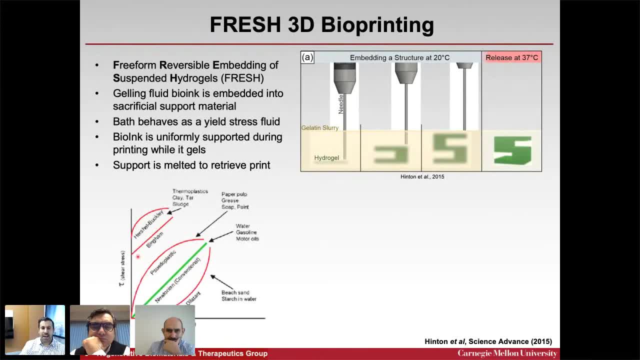 Really, the key rheology of our support bath is that it acts as a Bingham plastic. So if we look at this plot here of sheer stress versus sheer rates, uh, you see the Bingham plastic here and we basically need to hit a certain shear rate and then the support bath flows like a liquid. 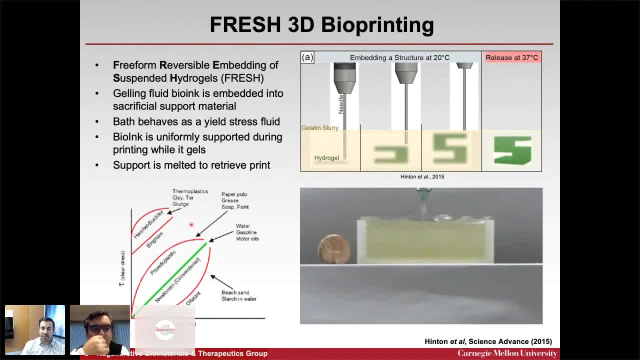 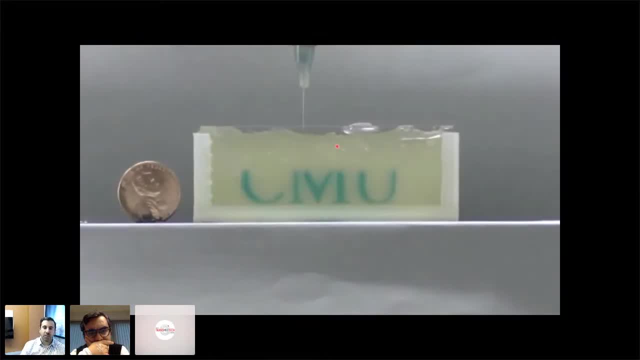 So I'm going to play this video just to show a real example of the printing process- uh, in a time lapse. But what you're going to see here is you see the needle, you see it's moving through that support bath, essentially with almost no resistance. 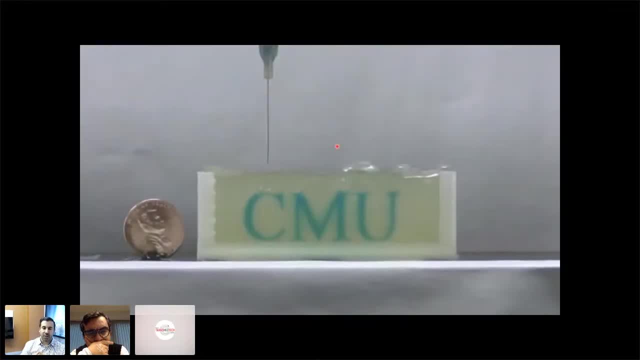 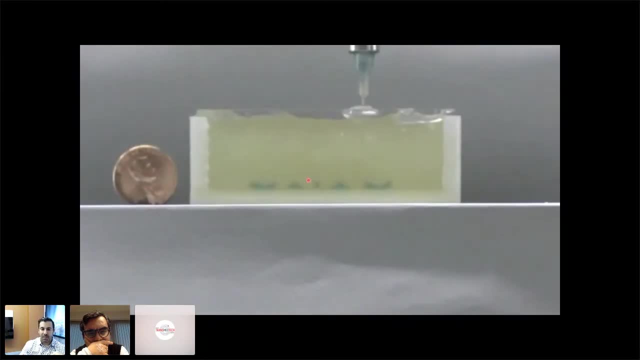 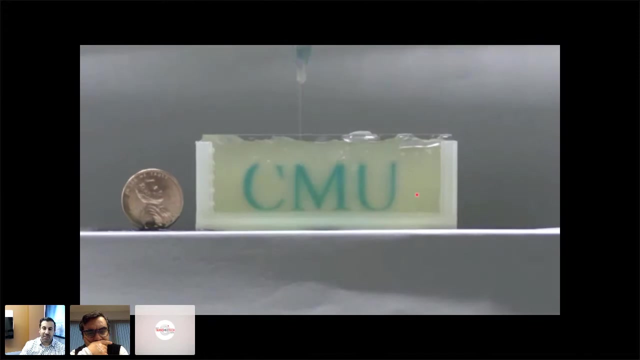 That's because as the needle moves, it generates enough shear force that the support bath flows around the needle as a liquid but then rapidly re-solidifies. But whatever we were printing stays embedded in place, Right, In this case we're printing an alginate, the alginate solutions- in the syringe. we have calcium ions in the support bath. 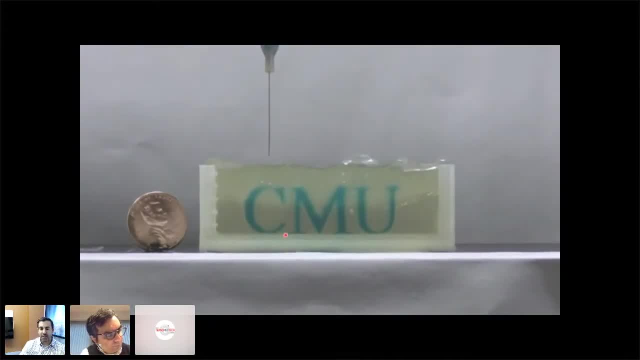 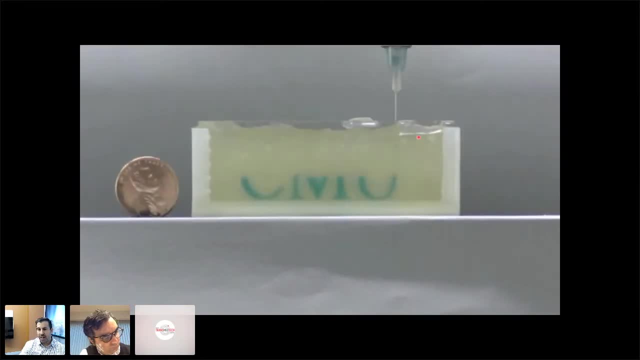 So as soon as that alginate comes out, it's immediately ionically cross-linked uh into a gel And then, when we're done, we're raising the temperature of the build platform. You can see the liquefication goes from the bottom up and it releases our prints. 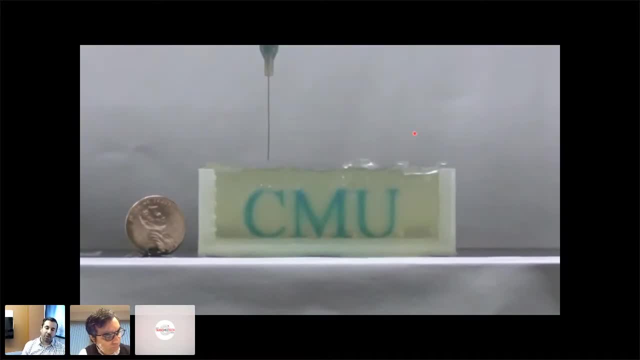 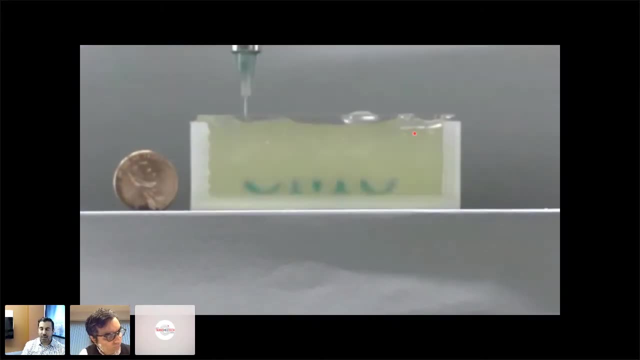 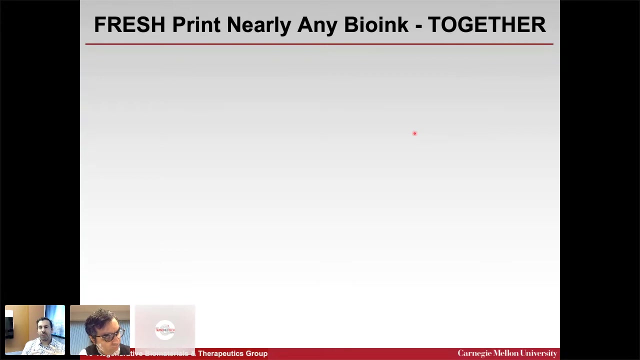 Again, we can do this between room temperature and body temperature, which is really a thermal range in which cells and most biologic materials like proteins have, you know, excellent uh, uh, uh tolerance. So you know, one of the exciting things with this approach is that we can fresh print, uh a really wide range of bio-inks, and most of these can be printed together if they have orthogonal or essentially non-interfering gelation mechanisms. 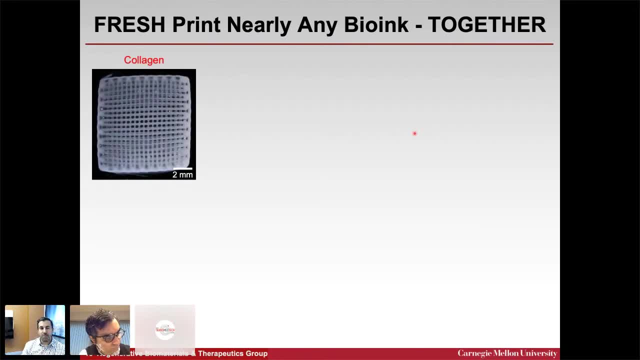 So, just as an example, uh, we can print collagen by printing an acidified collagen solution into the support bath. where the support bath is pH buffered- And I'll talk more about this in a second- We can print alginate, like I just showed, and alginate. 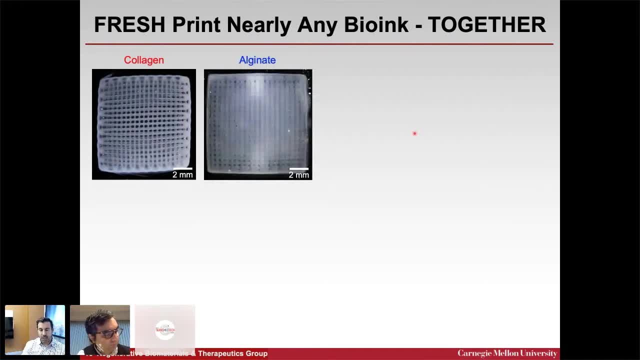 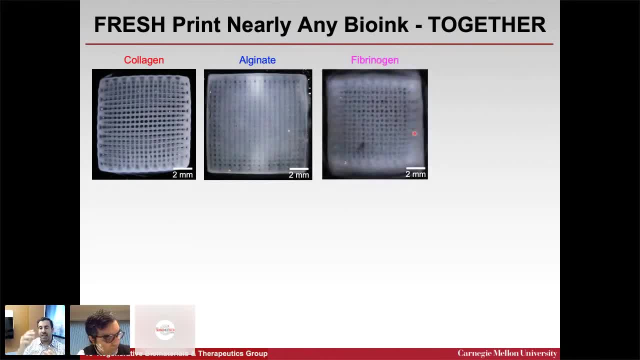 We can do enzymatic cross-linking by printing fibrinogen into our support bath where we have thrombin, and then thrombin will cross-link the fibrinogen into fibrin through an enzymatic reaction. Or we can use more traditional UV-based cross-linking where we, in this case, have a methacrylated hyaluronic acid. 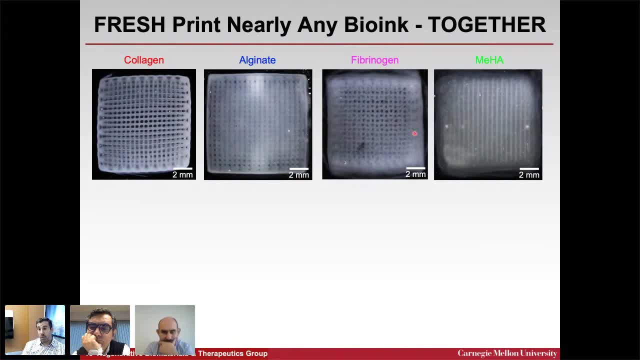 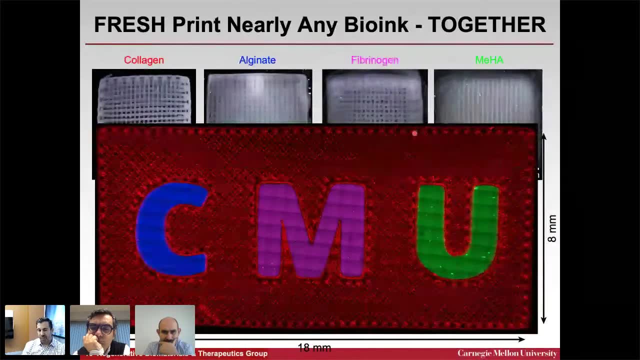 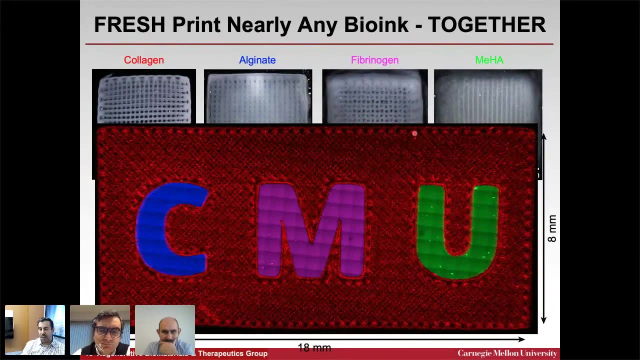 Uh, we print that into our support bath where we have herbicure and we have a UV light that drives photocross-linking, And this can all actually be done in the same support bath, in the same print, And just as proof of concept. you know here: uh, the red is collagen, the blue is alginate, the pink is fibrin and then the green is hyaluronic acid. 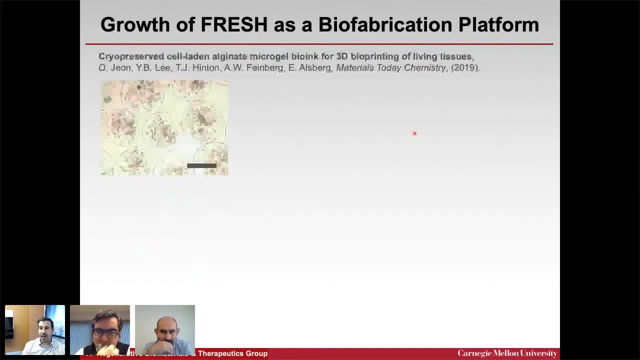 So we've been really excited that, uh, that Fresh has grown as a biofabrication platform- uh, a fair amount over the past five years since we first published this in 2015.. Uh, so this is an example of collaborative work with Edmund Alsberg's lab. 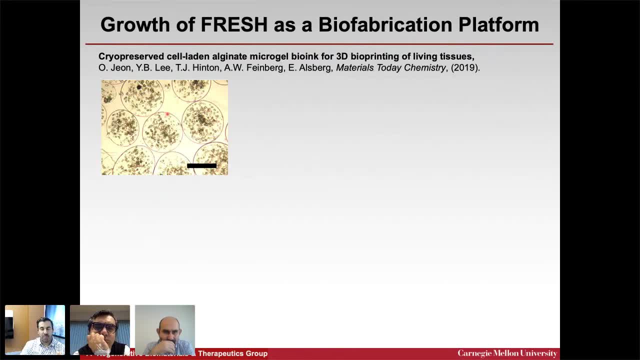 Uh, where he created these microspheres out of alginate that have embedded, uh, mesenchymal stem cells? Uh, these are alginate that are ionically cross-linked, but it's also methacrylated so they can be UV-cured later. 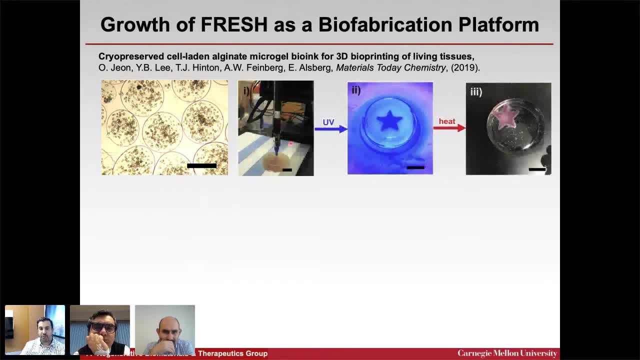 And so these can be cryo-preserved and thawed on demand fresh, printed into a structure and then exposed to UV to gel them into a structure. So it's this really cool: cryo-preservable UV, cross-linkable cell-based biolink. 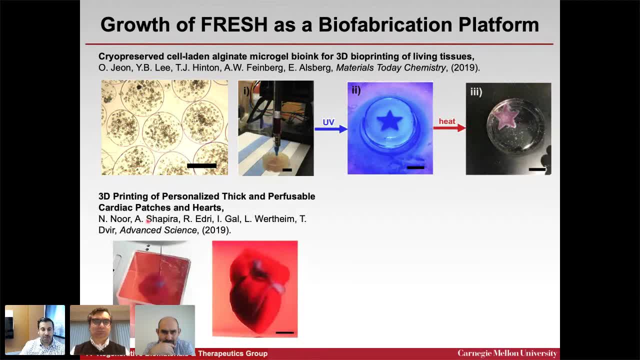 Uh Tal Daveer's lab at uh University of Tel Aviv- uh last year had a a nice publication using uh hyaluronic acid. Uh Tal Daveer's lab at uh University of Tel Aviv- uh last year had a a nice publication using hyaluronic acid. 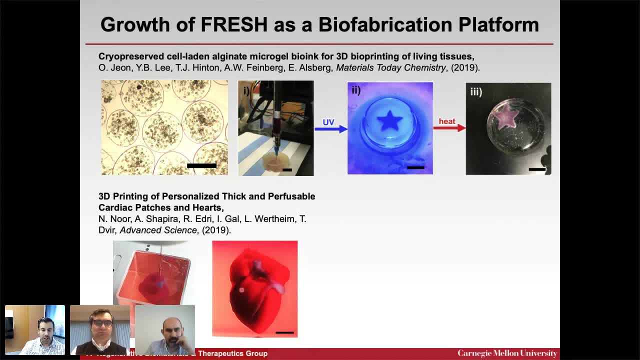 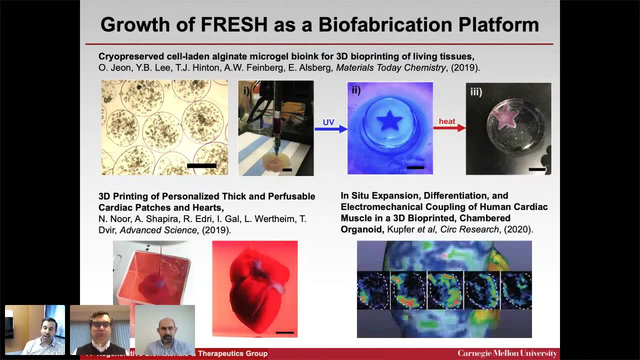 Uh Tal Daveer's lab at uh University of Tel Aviv uh last year had a a nice publication using an alginate-based support bath uh, where they printed a heart-like structure. Uh, and then just this year, uh Brenda Ogle's lab at the University of Minnesota in Cirque Research uh had another uh heart-based, uh fresh printed construct. 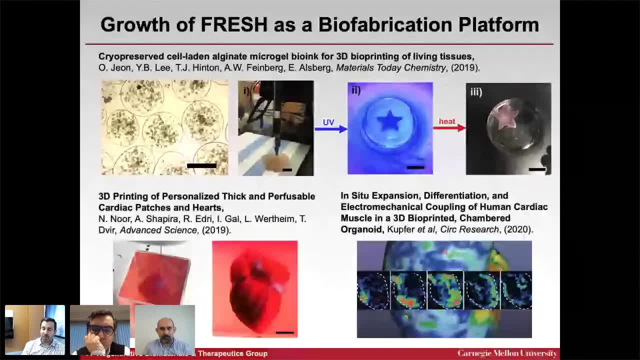 In this. in this case, we're actually to show a closed chamber that could generate pressure and PV loops. So really uh excited that these these labs have been able to uh take this technology and also be successful with it. 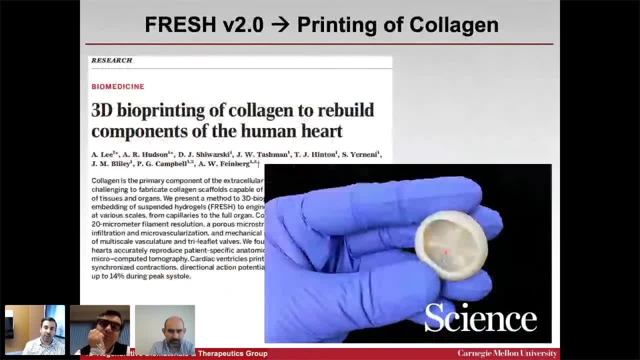 Uh, what I kind of wanted to talk about, though, is our- really our- latest results With fresh bioprinting. uh, it's published in Science again. about a year ago- a little bit more than that- I really focused on printing collagen, and we really wanted to focus on collagen, because it's really the foundational ECM protein, uh, in the human body, for every tissue and organ. 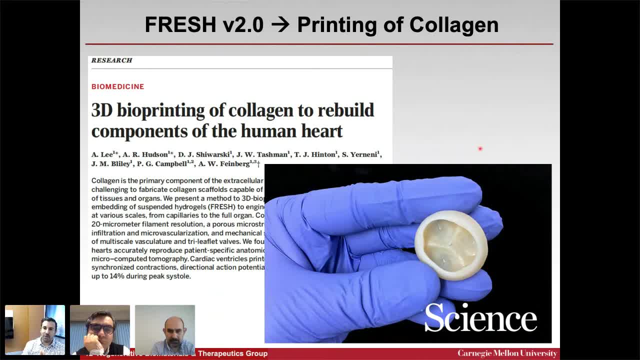 Um, and you know, we we figured if we could start to really print with collagen. uh, can we start to really print things that don't just have really cool structure, but can they also now start to demonstrate true biomimetic function? 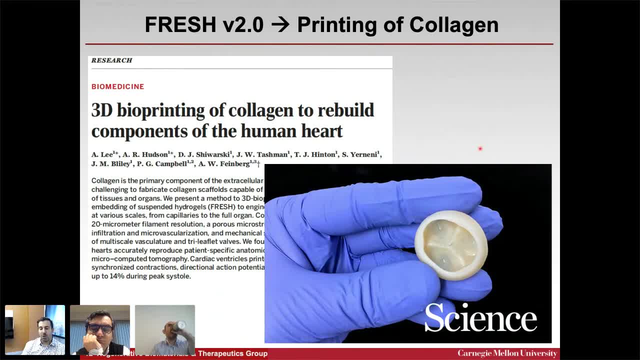 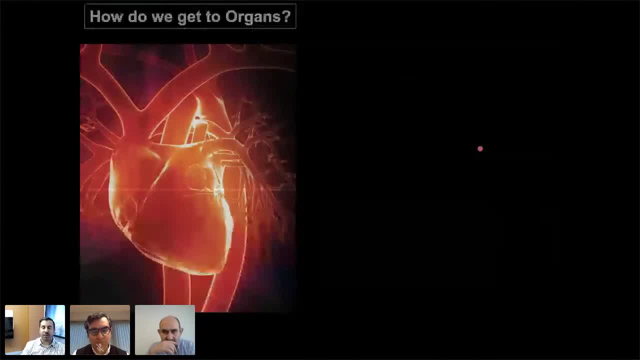 Uh, I think that's a really good question. Uh, so that they function in a way that's similar to the real tissue or organ. And so if we think about that goal and really trying to again move this towards organs one day, how do we get there? 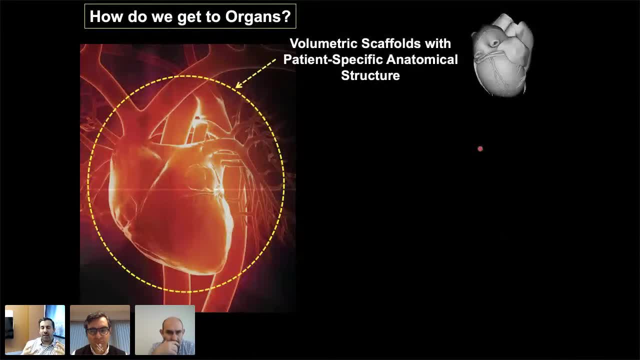 The key things we wanted to hit upon were: A- can we, can we print at volumetric scale? So really, you know, single to tens of cubic centimeters, really large structures, you know, at least for state-of-the-art bioprinting. 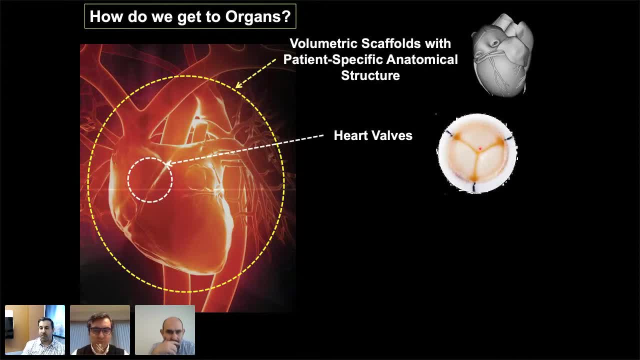 Number two: can we have mechanical function? We really looked at the heart valve to show this. Can we start to address this challenge of multiscale vasculature from capillaries on up to, you know, arteries and veins, And then, finally, can we do dense cellularized tissue? 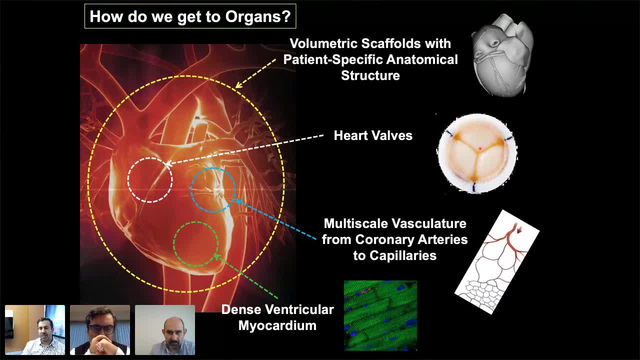 You know, one of the one of the challenges with a lot of bioprinting is that cell-laden hydrogels typically have a relatively low cell density of tens of millions of cells per ml. you know, along with the biomaterial to get printability. 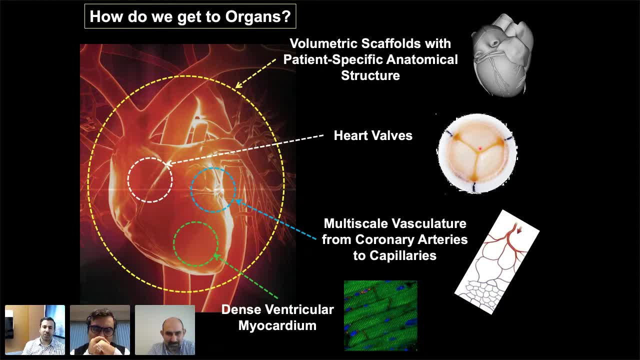 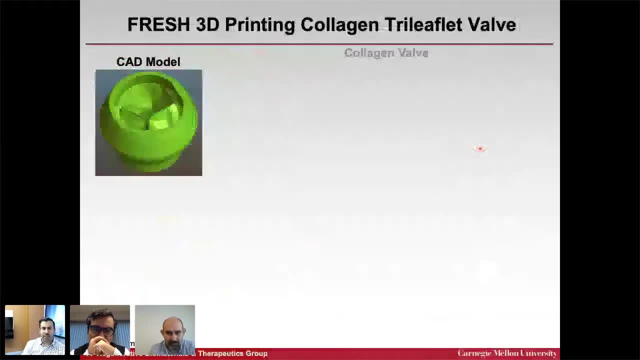 But real tissues, muscle tissues are not as mobile tissue, liver tissue, other tissues have extremely high cell densities, hundreds of millions of cells per ml. so how do we achieve that? so the first example I wanted to show here is of the heart valve. so this is a CAD model of a simple 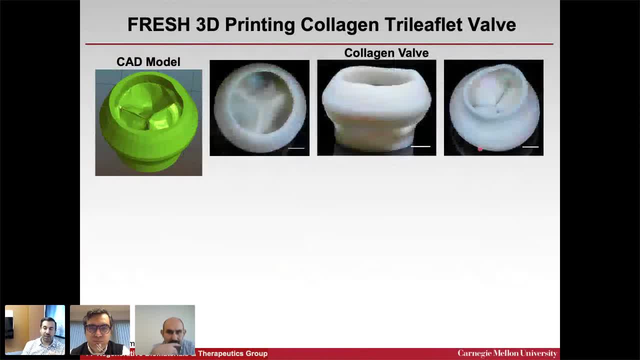 trileaf and heart valve, and what we did it was a 3d printed that at full, basically full adult scale, so about three centimeters in diameter, entirely out of collagen, and you can see that here in a couple of different views you can even see the build line. so again, this looks very much, maybe, like an FDM. 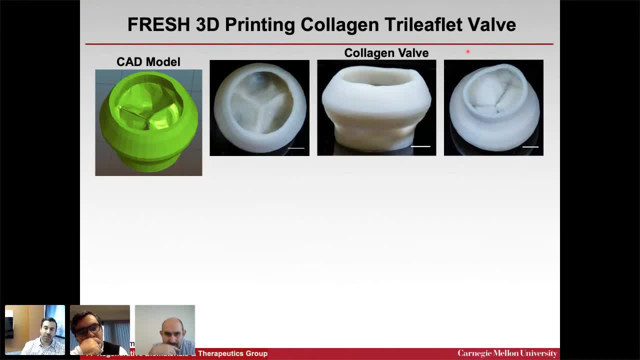 plastic print, but this is 100% collagen. now what we did was we tried to mimic the way collagen valves are used clinically, which is where they take a porcine valve, they strip away the cells, they decel your eyes, it, and then they fix it in glutaraldehyde. so we use the same process. we use basically the same. 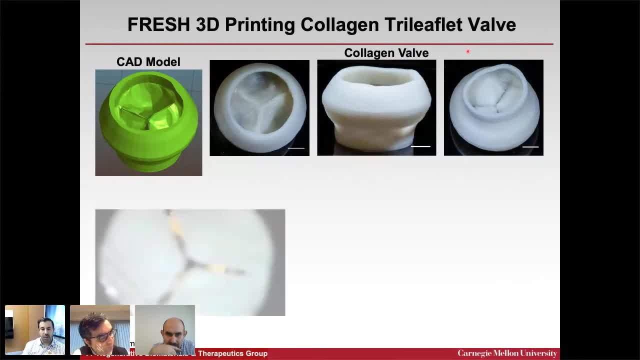 fixation process on our valve, basically to make it stronger. and while these have not yet been in vivo, we put this on a flow system that simulates adult flow rate and pressure, and then here it is being imaged with an endoscope, and so we were able to create these functional collagen based heart valves. 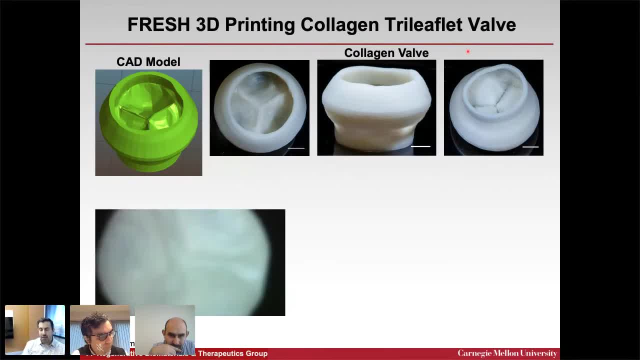 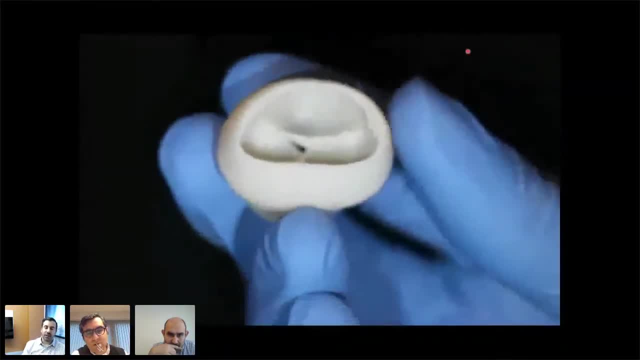 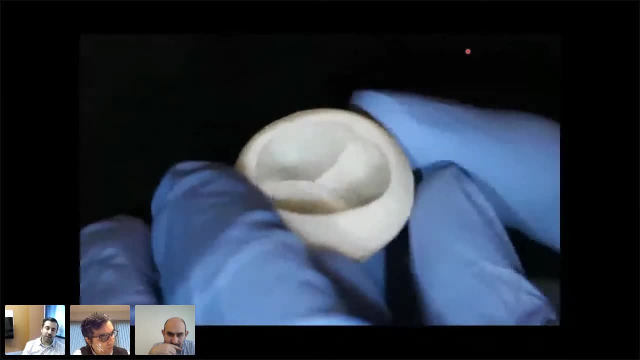 and and then, just to kind of give you an idea of what the the physical properties are, here's just a video of that valve being handled in air, and so this is again a really robust collagen based valve that we have full control on the, on the design, and so future work is going to be looking at improving the. 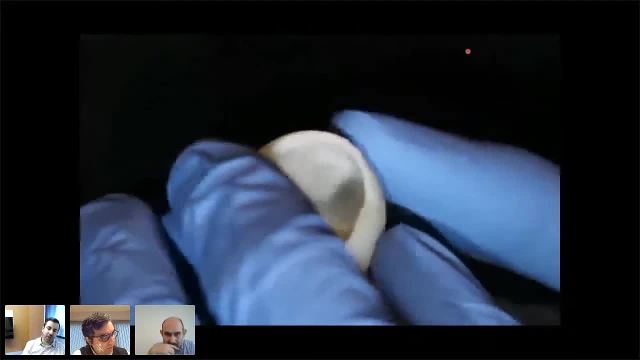 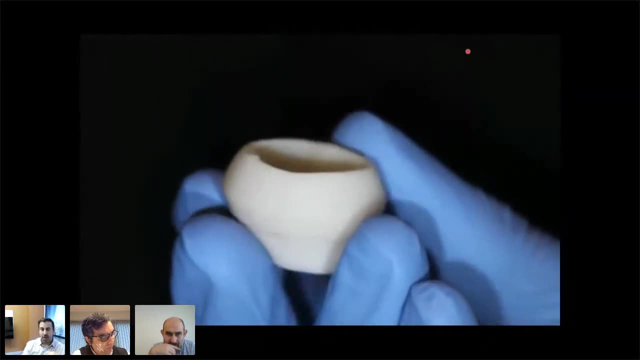 performance of this valve further and then getting this in vivo in a large animal model to look at the ability to actually function as a valve in the actual heart, and so that that's all on the on the on the slate for future work. the second thing I mentioned is actually creating. 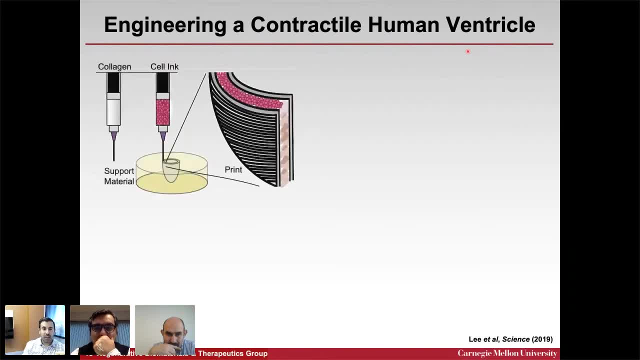 dense cellularized tissue that has some level of function, and so the way we did this was we had a to bio, basically a to bio anchor biomaterial system. we had one syringe that's just just collagen and another syringe that's a cell based ink. 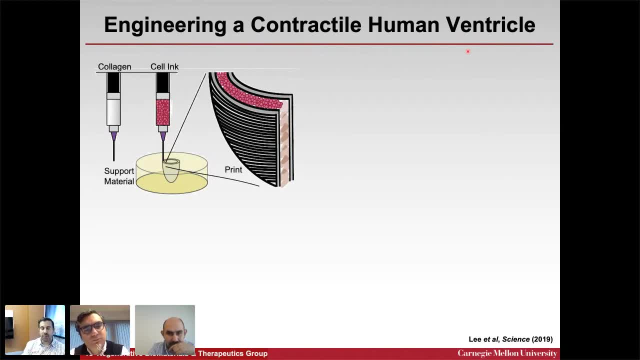 that has cardiomyocytes. so these are human stem cell derived cardiomyocytes and fibroblasts at a very high density of about 300 cells per ml. and what we did was print a simple ventricle like model, like kind of like this open ellipsoid where the outside and inside shell are collagen. 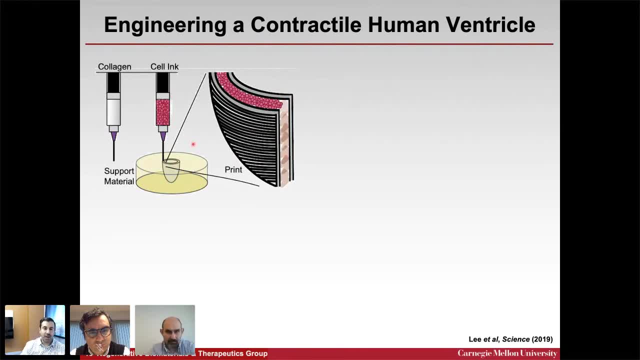 and then in between is a layer of these cardiomyocytes and fibroblasts. as I mentioned, the collagen is actually printed by having an acidic collagen that is rapidly neutralized. but we did separate these because we need to have a very high density of collagen and we need to have a very high density of. 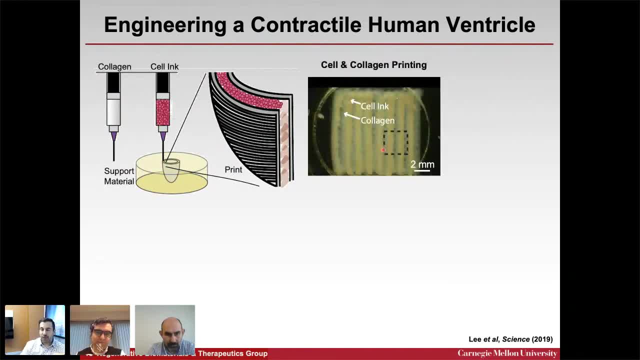 cells that have functional muscle tissue, and so one of the first things we did was actually print this cell ink and then those colleges collagen ink next to each other, to make sure that we could neutralize, using our buffering system, the collagen very rapidly and that that would not the acidic, the acid and the. 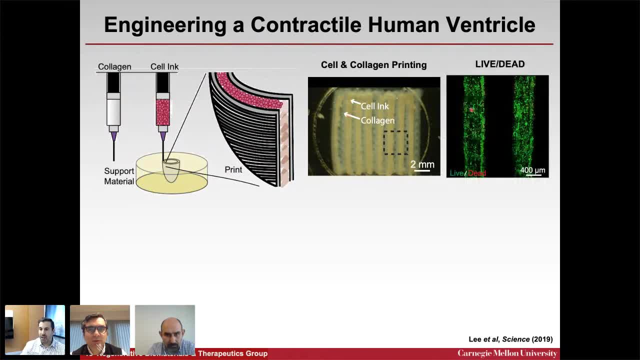 collagen would not damage the cells, and indeed it does not. here's some live dead where we can see high cell viability. we then here's the simple model of this ellipsoid of this ventricle. it's really about a simple model of this ellipsoid of this ventricle. it's really about 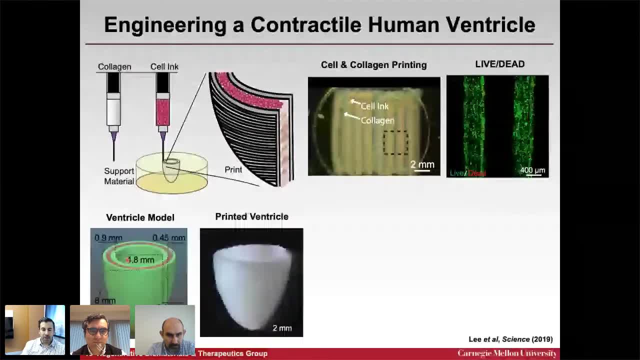 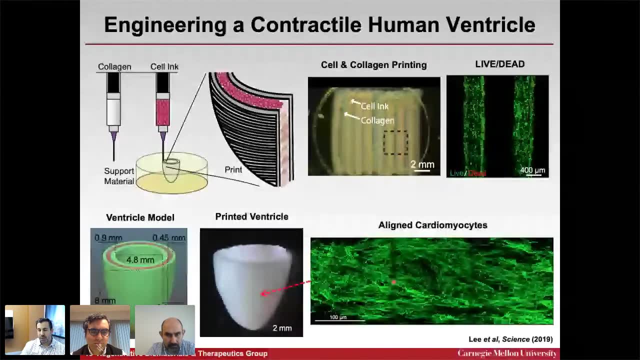 the size of the end of the pinky. here it is printed out of the collagen and cells and then here is actually a staining of the cardiomyocytes in this wall of this ventricle, stain for the sarcomeric alfactinin, and we can. 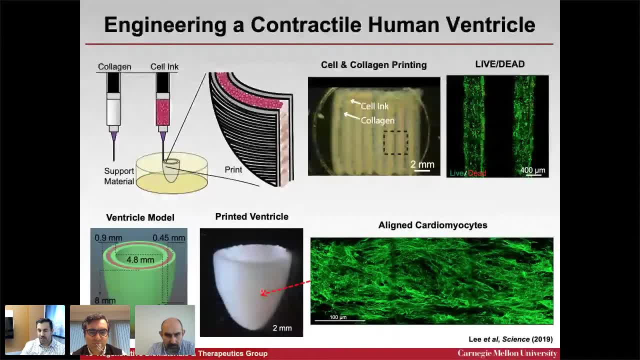 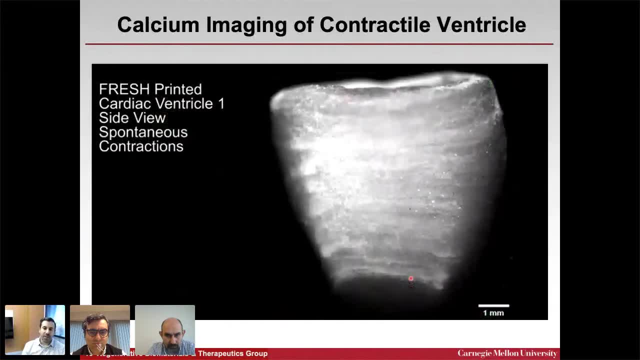 actually get a general direction of alignment in the print direction, which is really cool, so we can control cell alignment through some of our printing technology. so look at function. what we did is we took this, these ventricles. we then looked at them under the stereo microscope. 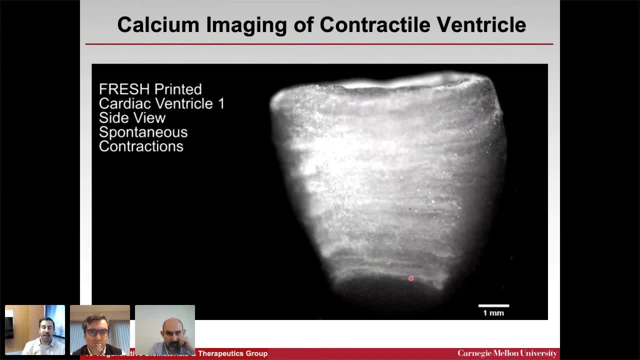 under fluorescence using a flow for calcium sensitive dye and for muscle cells, when, when the cells contract, calcium rushes into the cell and that's actually visible as an increase in brightness. so if I play this video, what you'll actually see is this wave of electrical activity that propagates. 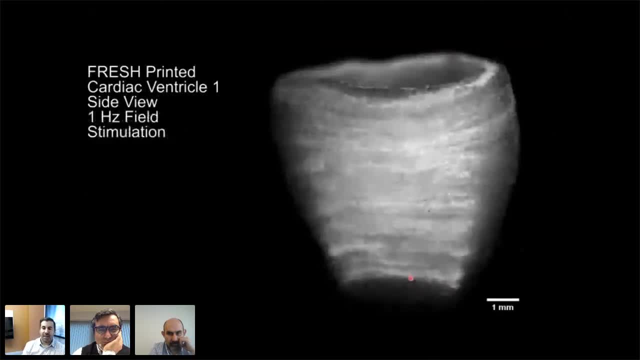 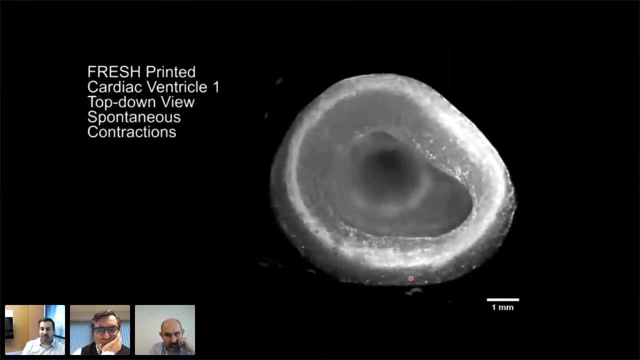 spontaneously around the ventricle. that's spontaneous. and here it is actually under field stimulation. so we have some platinum electrode wires outside the field of view and they stimulate the heart at a constant rate. now we're gonna, we're gonna flip and look into the ventricle from the top and again, this is 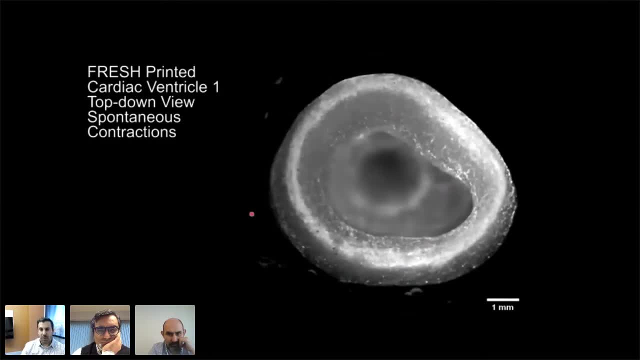 spontaneous. you can see the wave of activity again going around the ventricle. we're then going to pace it and then actually what's happening during pacing is: do the synchronization, we actually have wall thickening and decrease in interior chamber volume. this is actually the first time anyone have. 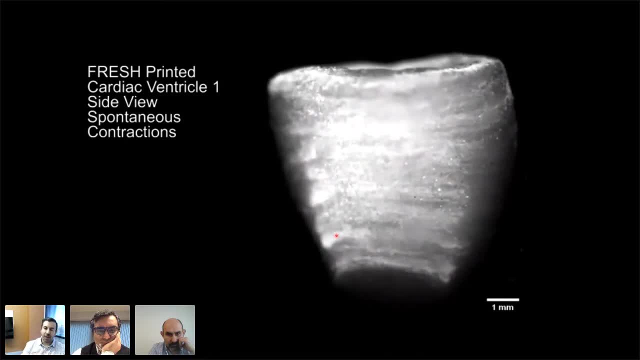 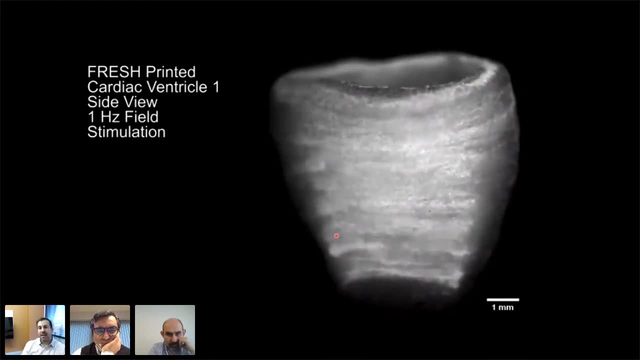 been able to achieve wall thickening in one of these engineered ventricles, and that's really exciting, because that's the same way the heart actually functions. and so, even though we're far, far below the level of function of the actual ventricle, we can at least start the function in the same way in terms of wall. 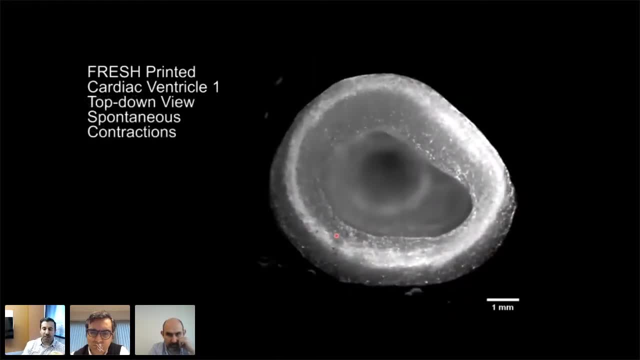 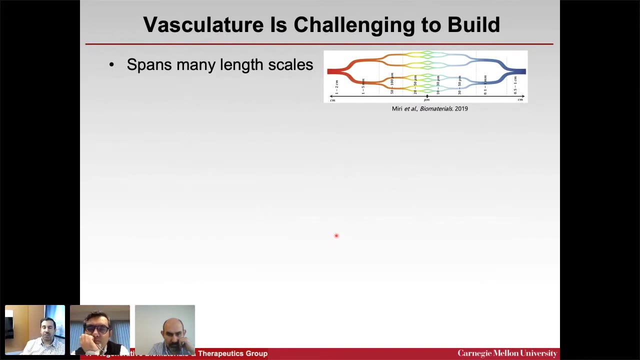 thickening, and so we're really excited that, again, this obviously can be improved much further than where we are are in this video, and we're already doing that building kind of these improved ventricle models in the future. the next thing I wanted to touch upon was basically vasculature and really 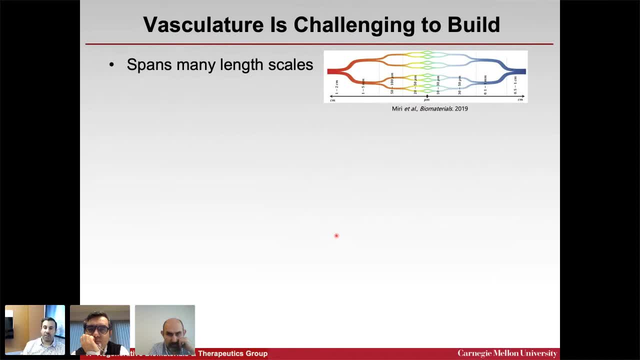 this challenge of trying to build a vasculature across length scales right. as we know, we go from arteries and veins down to capillaries. we're talking about, you know, vessels that are many centimeters in diameter, down to vessels that are really, you know, maybe even as. 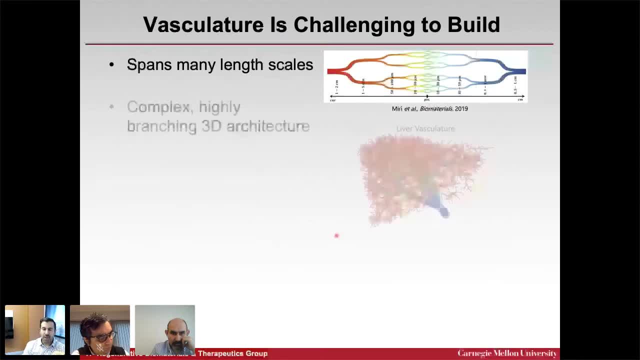 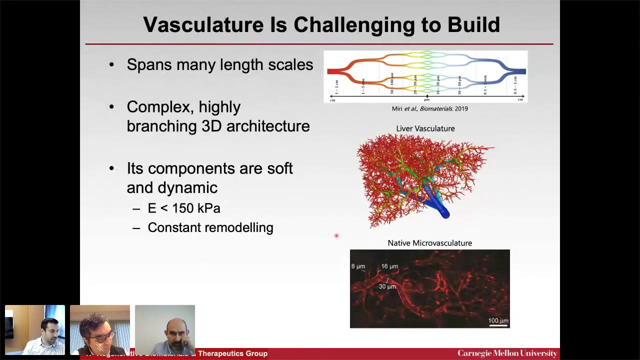 small as five microns of diameter. so how do we do that right? we also have this complex three-dimensional architecture, right branching architecture. how do we, how do we rebuild that? that's really difficult as well. and then obviously the materials are soft, they're constantly remodeling and obviously all this needs to be created in a system that's 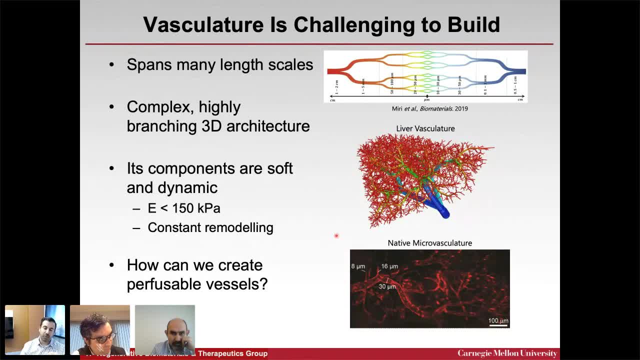 perfusable, right? so the pressure drops between levels of branching really needs to be correct for this whole system to become perfusable and to function properly. so those are some pretty high bars, I think the hits. so how are we approaching this? how are we tackling this? so you know, I think there's a 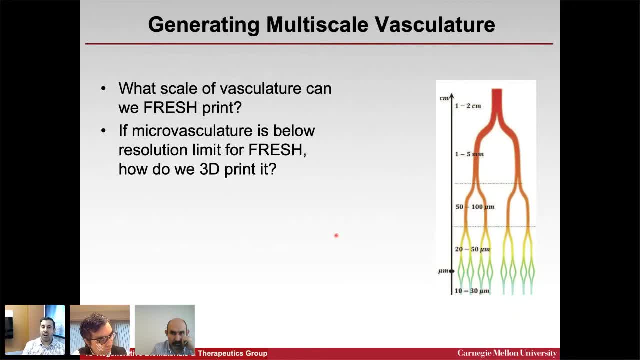 fundamental question about what do we need to print and then what can biology do for us? so what scale can we fresh print and then what can we do to get it to be a very good printing system? if microvascular is required below the resolution of fresh, do we need to print it, uh, or do we? do we? 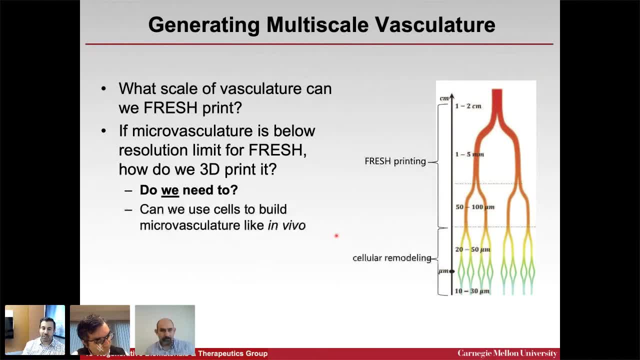 do we uh not need to print it? in other words, can we rely on, basically, cells to build the microvascular for us? and so that's really what we're doing. we're fresh printing from about 100 microns on up to larger scale and then we're really relying on cell-based uh processes and 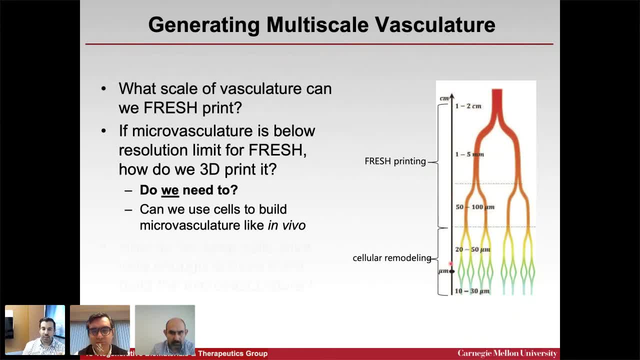 geogenesis to basically build the microvascular for us, uh, and, you know, also trying to address the challenge of how do we keep cells live long enough to have this microvascular actually be built. so i'm going to want to show you kind of two examples of how we're approaching these different 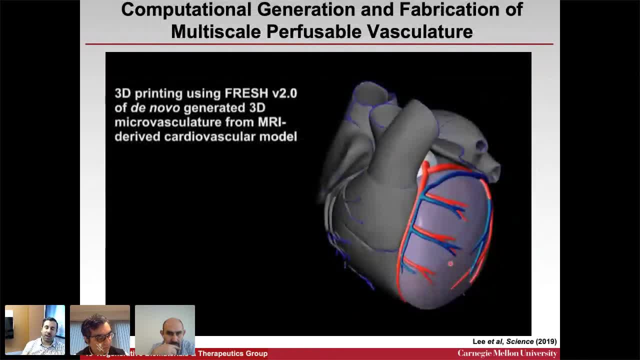 length scales. so the the first is really the, the level of printing the baths, which are directly, or at least ambassador, like three-dimensional branching networks. what you see here is an mri image of the human heart. you see the left ventricle and purple, and then you see: 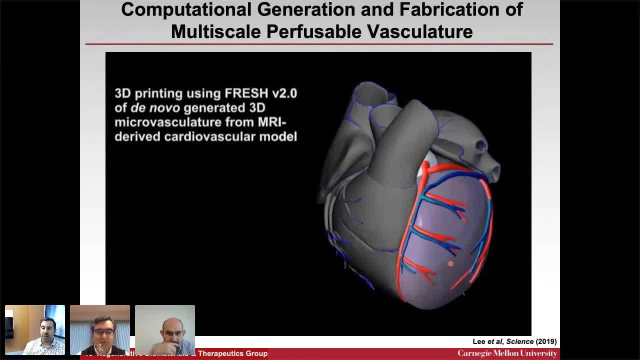 the coronary arteries and veins and red and blue respectively. now you know, mri is really exciting because we can get a patient-specific model of the anatomy. but clinical mri has a resolution of voxel size on the order of about a millimeter and a lot of the vasculature is below that. 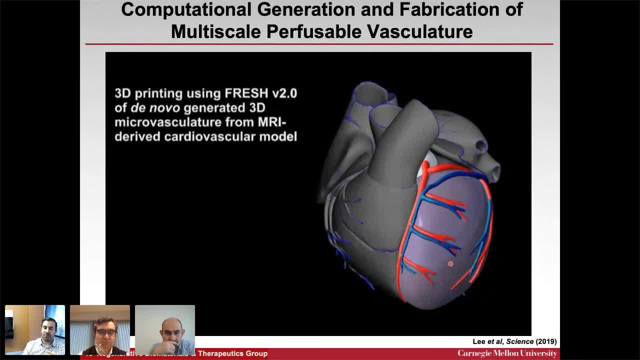 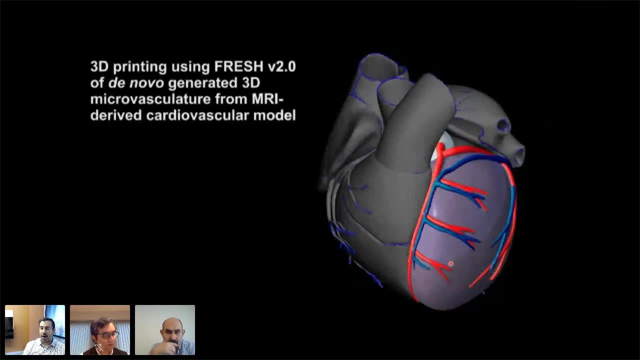 so how do we recreate a vasculature that we can't image? so what we did is we decided to use computational methods to generate vasculature and then try to print that and then perfuse it. so again, as i play this video, what you see here is this, this mri image, this segmented image. you 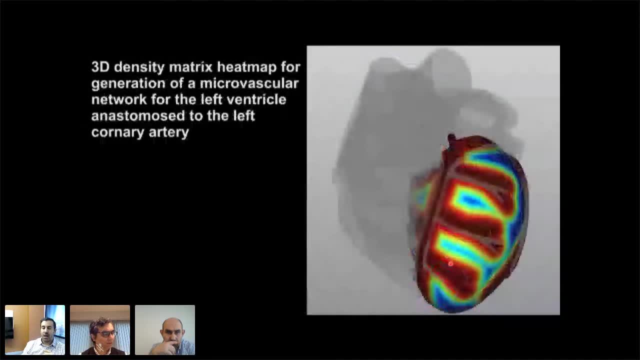 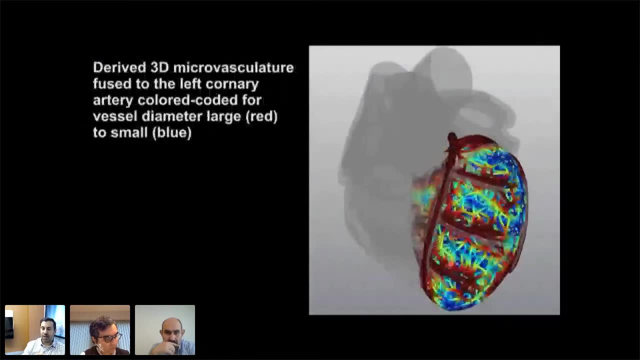 see the left ventricle. we're going to then focus on that left ventricle. what we're doing here is creating a distance map where red is near the artery and blue is further away. so we're looking at just the arteries now. we then created a vascular network using a voronoi lattice. 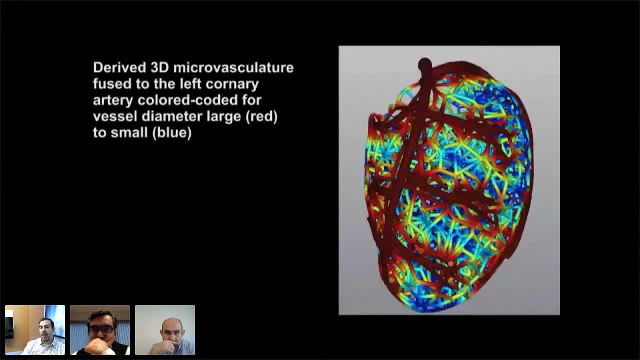 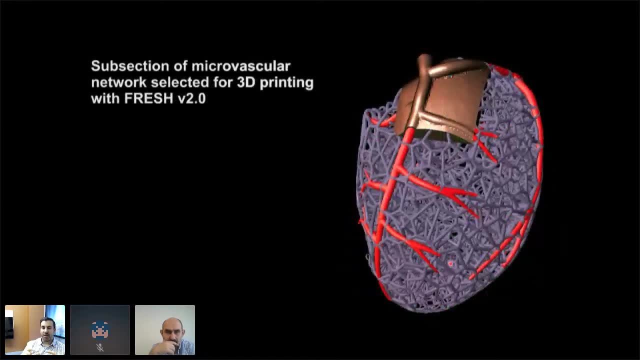 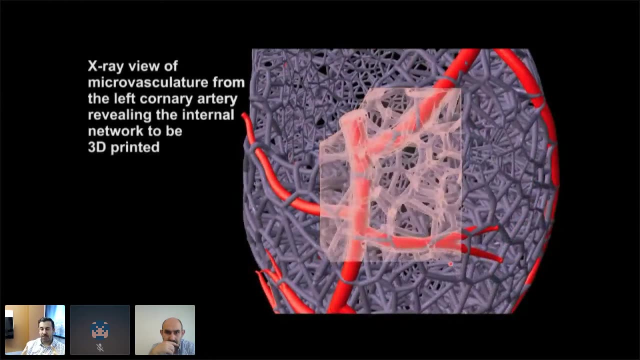 structure where the, where the vessels get uh uh smaller and branch more of the further you you get into the arteries. we're then going to focus on a segment of this, a whole ventricle. uh, this is where the root of the coronary artery is, as well as some of the surrounding vessels where, basically, it's. 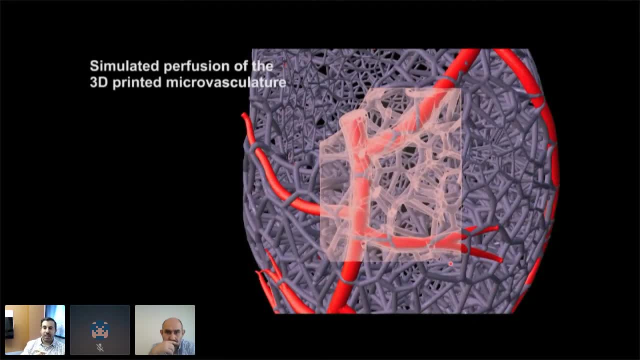 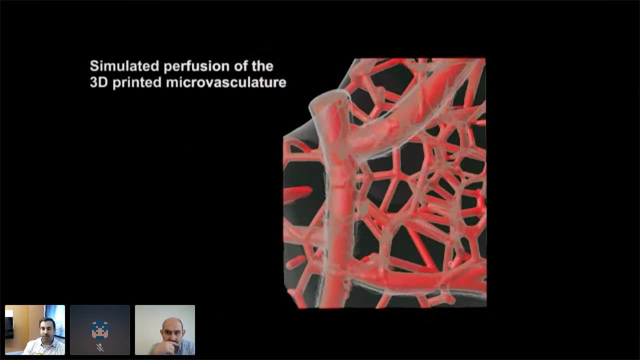 about two by three centimeters. we're going to basically isolate just that. um. so the red here is the, the image by the mri, and then now these smaller vessels is what we computationally generated. we're going to take that, create an sdl and now 3d print this entirely out of collagen. 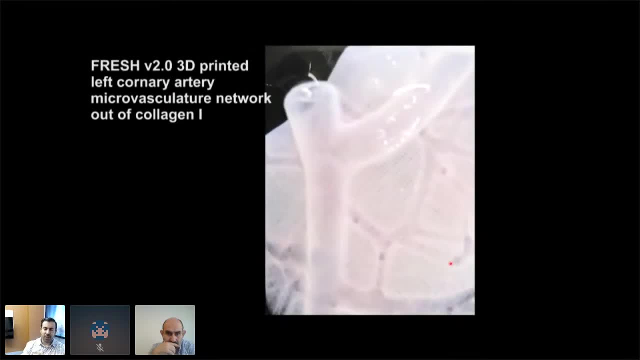 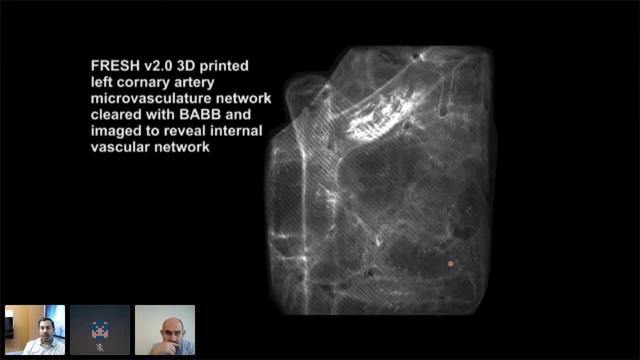 type 1.. so we're going to take that and we try to image it using fluorescence, but you know it's hard to see a lot of the internal structure. so what we did next was actually to clear this, uh, clear the collagen so it becomes optically transparent, and so what you're seeing here is a real-time perfusion. 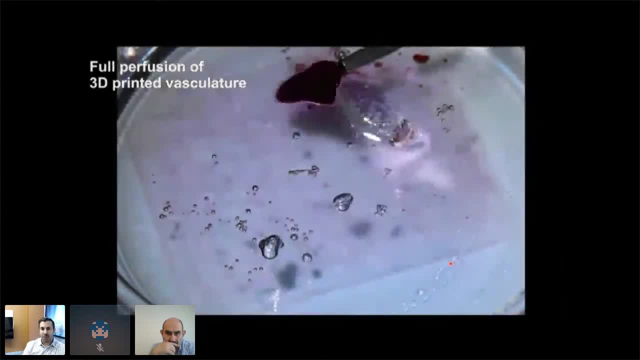 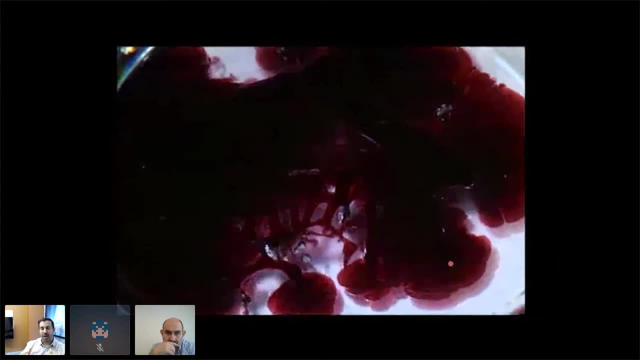 video of a blood substitute into this multi-scale network, so into the root here: larger vessels, smaller vessels. now it's actually leaking out the periphery because again, this block was kind of just cut right out of the whole ventricle. so those vessels are open. but what you'll see us do now is 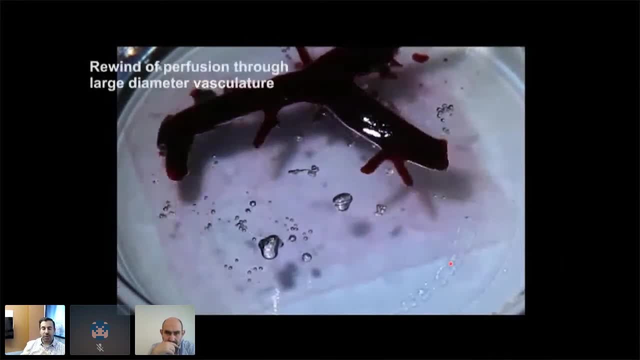 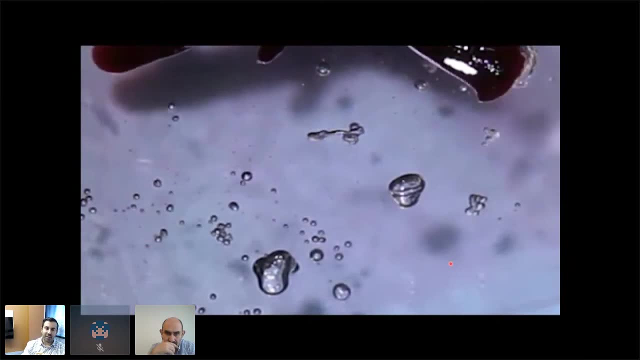 kind of move this video forward and backwards in time so you can kind of see again this interconnected multi-scale branching network be perfused. and if we zoom in here just on the very center, you'll see some of the smallest channels being perfused and the smallest one right in the center actually goes. 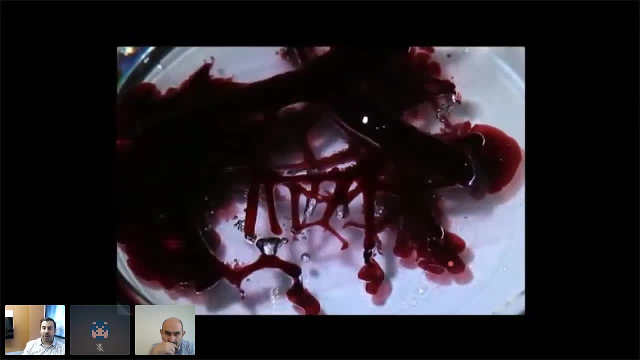 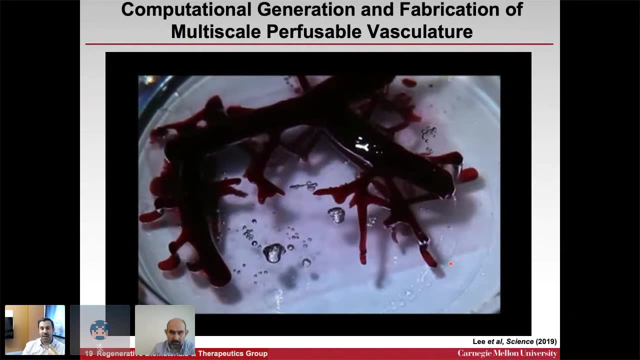 down to a 100 micron diameter. so again, this shows that you know, with fresh we can really start to build these multi-scale vasculatures, uh, at least vascular-like networks. these are not yet cellularized, but, you know, entirely within a collagen-based ectoplasm. 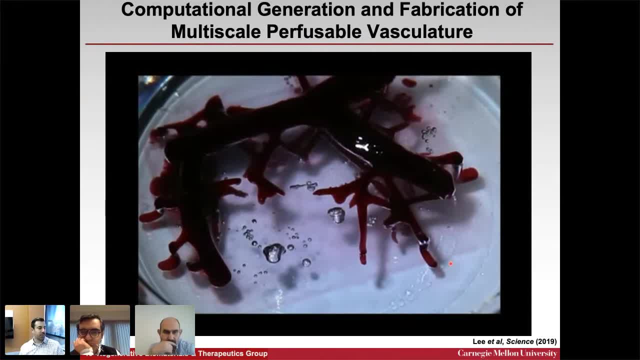 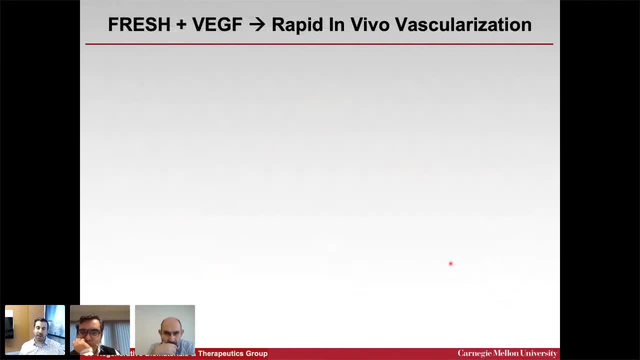 system. so this is what fresh can actually print directly. so what about going smaller? so by going smaller, as i mentioned, we're really looking for cells, endothelial cells, pericytes, other cell types- to help build that vasculature for us, and so the way we looked at this was to: 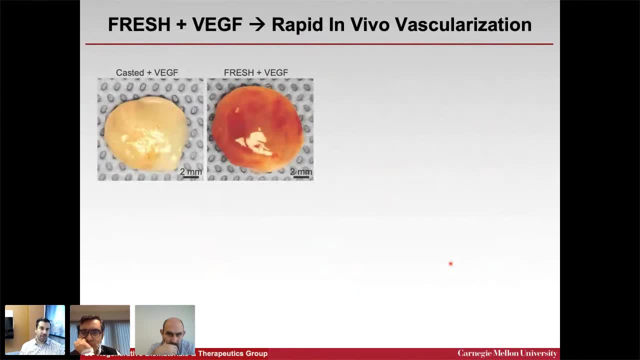 take a disc of collagen about a centimeter diameter loaded with vegf and also some pdgf, and either cast that into a disc shown on the left or create a disc the exact same size but fresh printed, shown on the right right. and these were both, uh, implanted subcutaneous in the mouse for 10 days. 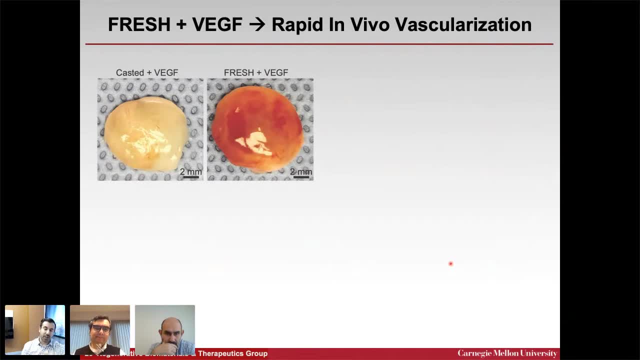 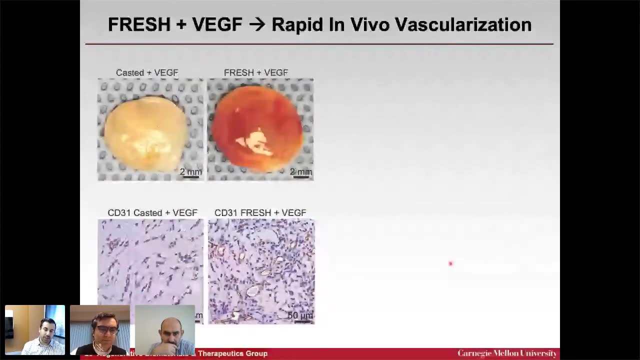 you can see just by gross examination that the fresh printed construct has much more vascularization. when we do cross sections and stain for h, e and also cd31 for the endothelium, we can see that we get cell infiltration in both, but only in the fresh printed construct at this. 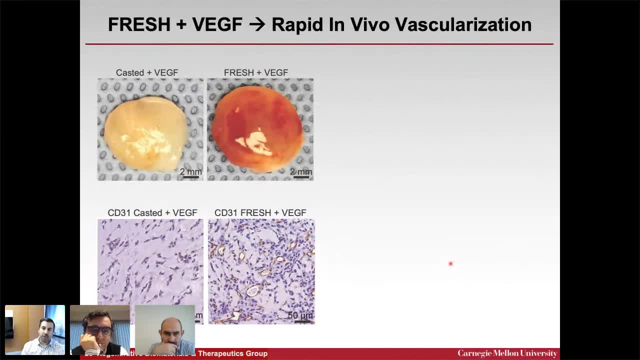 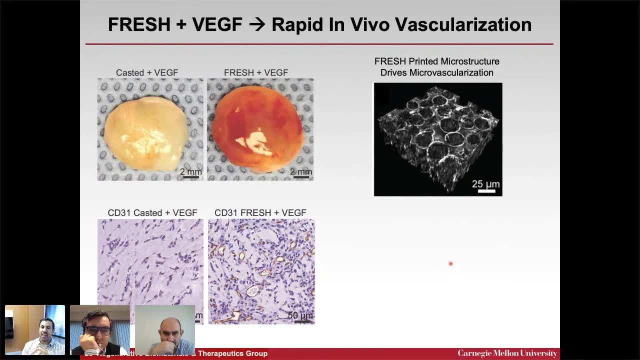 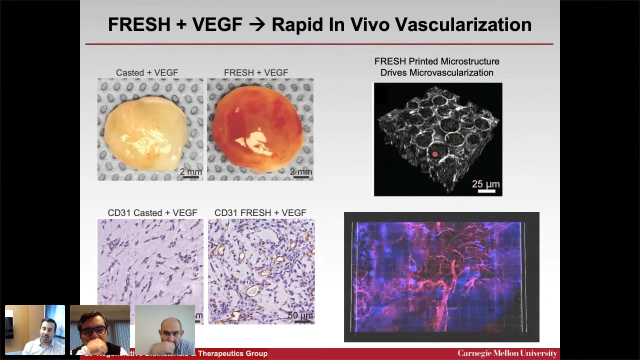 time point do we have robust vascular ingrowth? the reason for this is actually by purposely adding these extra diazepam and to the process of making all these different mass- misschien in this case we also added a few- becomes lectin stained, And this is the construct that we removed and did some whole mount imaging. 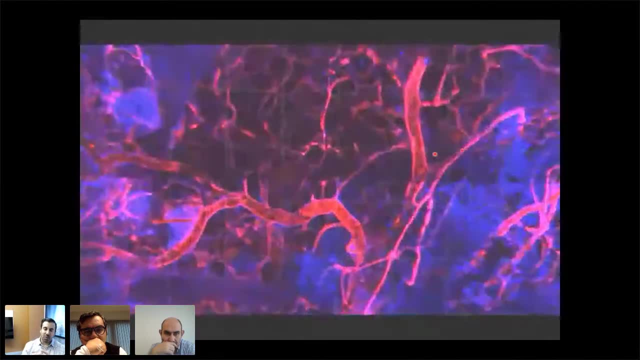 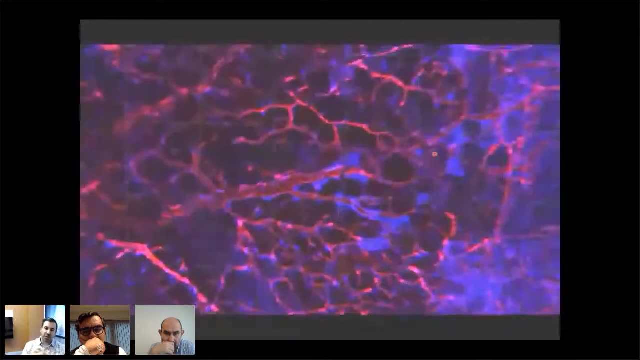 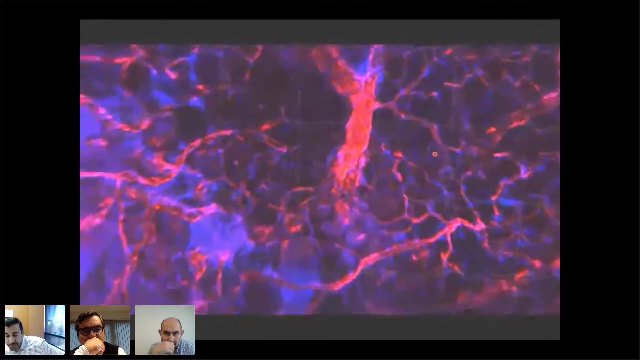 on And you can actually see this robust bastardization, with some larger vessels up to about 100 microns in diameter, which again matches up with about as small as we can print down to these capillaries that go as small as five microns in diameter. And so again, 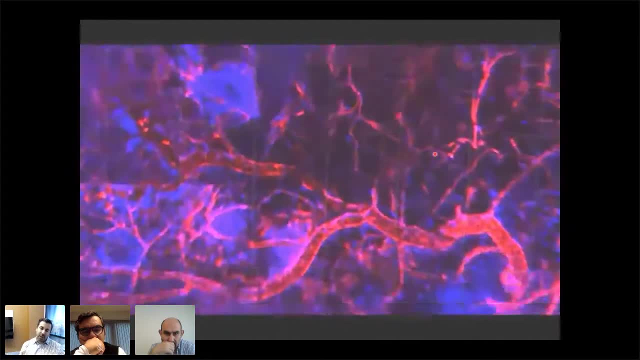 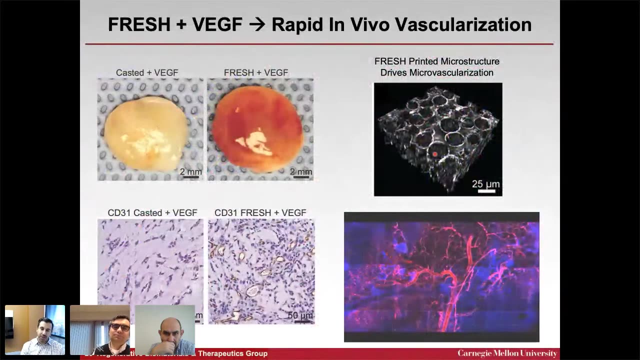 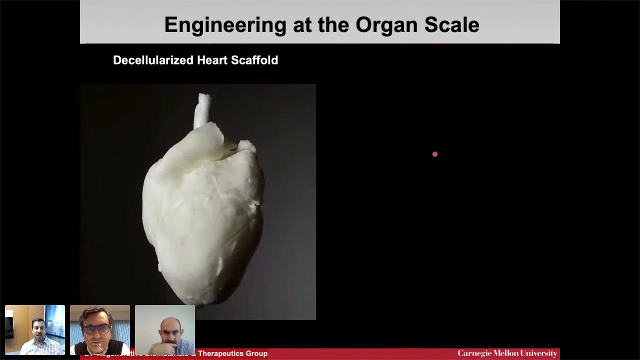 while we have not yet figured out how to marry these two levels of bastardization up directly within a single print. that is ongoing research in the lab right now to do that, But kind of shows the potential of the technology at both different length scales. And then, finally, I want to talk. 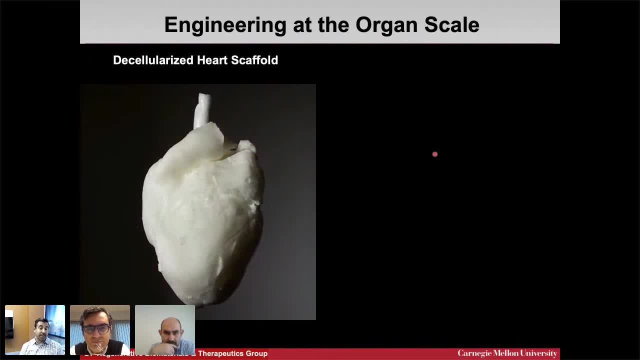 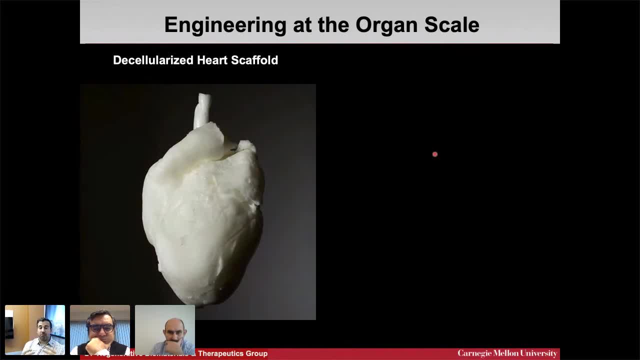 structure in 3D space and you put the right cells back, you start to really rebuild complex tissue. We just saw that. decellularized organs, however, have a lot of challenges with recellularization, especially as you go bigger. So the vision was then to be able to take MRI. 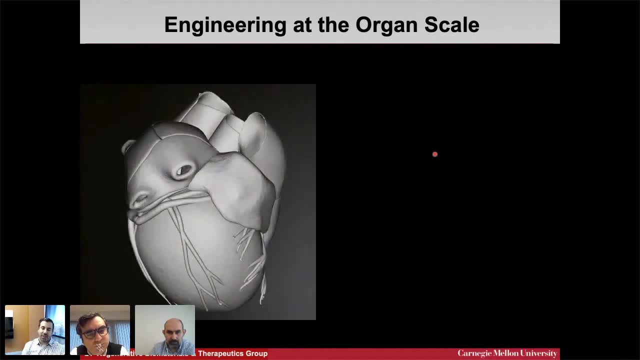 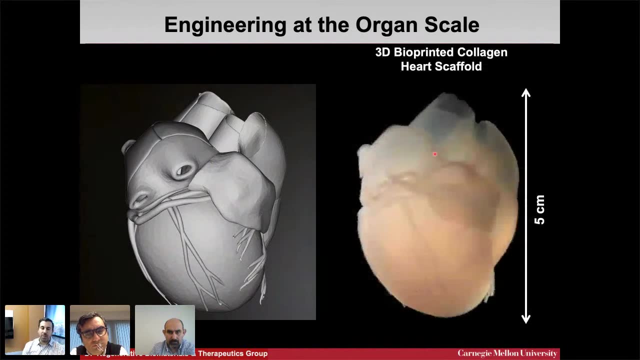 images and use that to directly fabricate ECM-based scaffolds that were like decellularized organs. So we're not all the way there yet by any means. But this is one example where we took the adult MRI segmented heart image on the left and we printed that not at full adult. 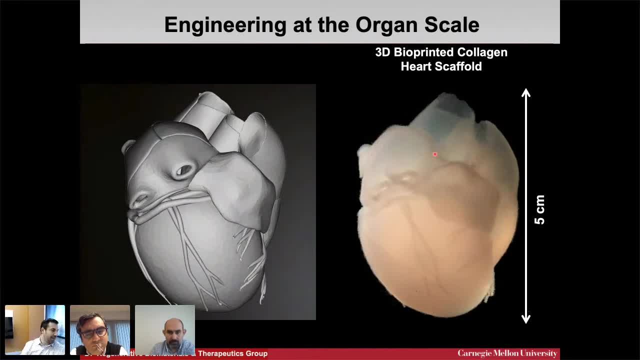 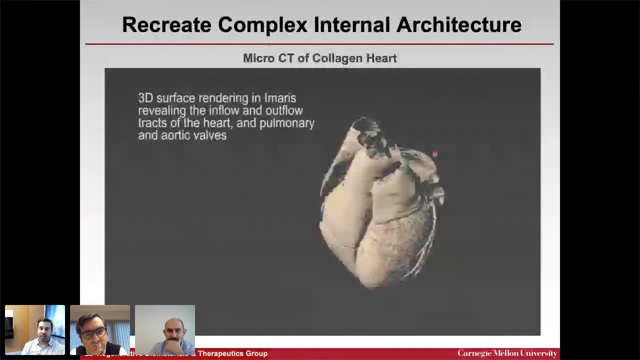 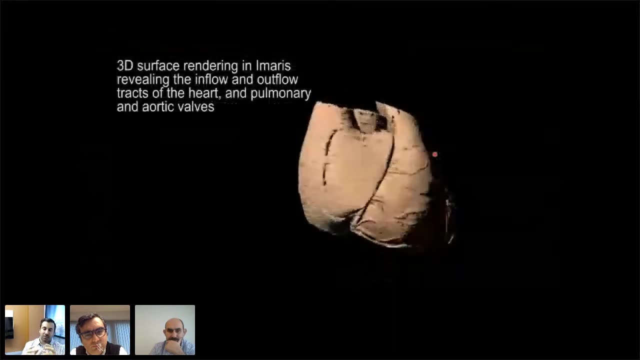 scale, but at neonatal scale, So about five centimeters top to bottom, entirely out of collagen. We were able to then take that heart and actually run it back through the micro CT And I'll play that video here. So this is the heart that we printed And again in the micro CT. 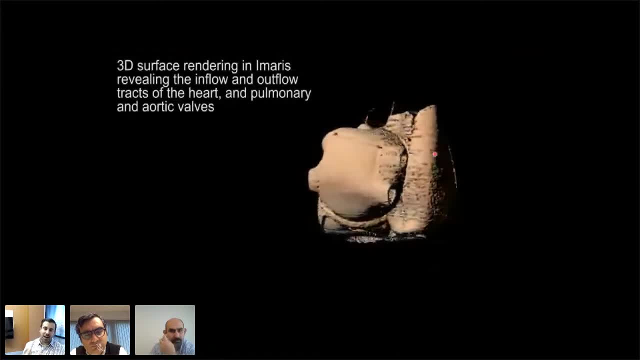 it looks like there's some holes in the wall of the heart. That's actually just more of a contrast issue, just because those areas are thin and didn't really resolve very well. But as we rotate this heart, you can see, we can really recreate almost all of the detail that is in the MRI image. 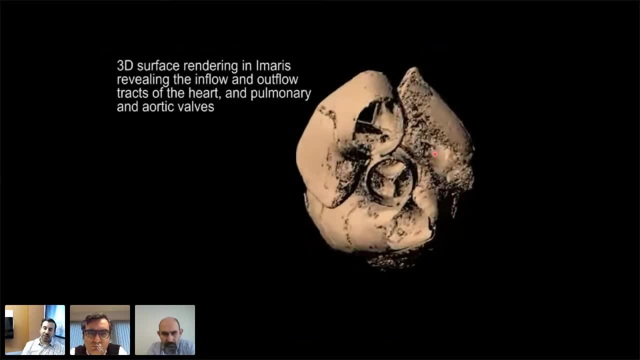 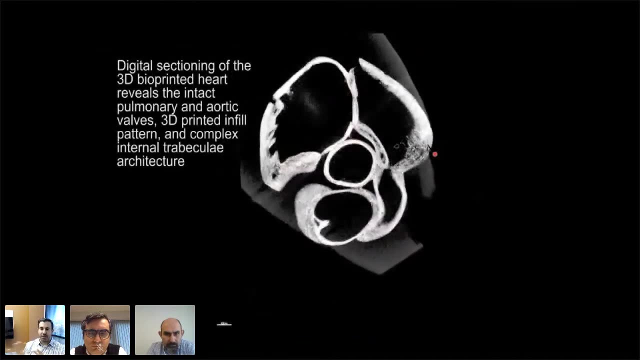 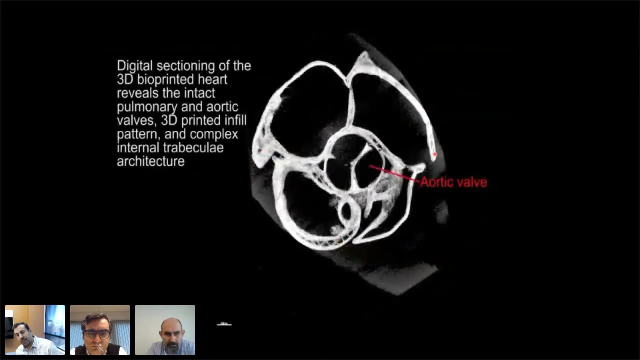 And now, as we look down into the main arteries here, we're going to actually go slice by slice and you'll be able to see now the different internal structure. So you see here the left and right atria, the pulmonary valve, the aortic valve, And then, as we move deeper, 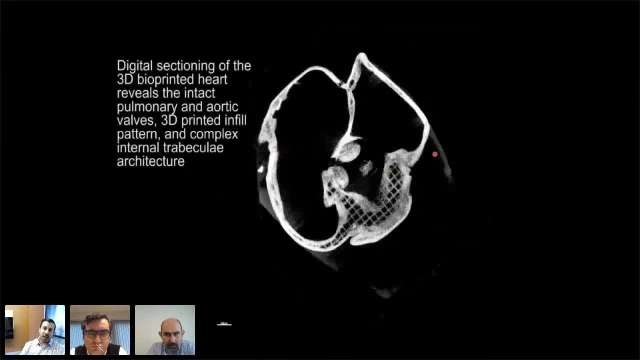 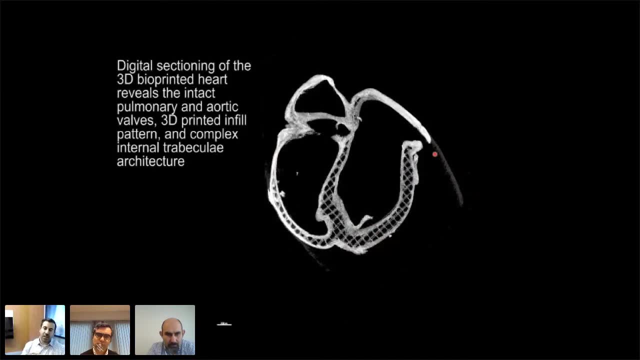 into the heart from top to bottom, you'll see first obviously the pulmonary valve, obviously this infill structure in the wall, but then also the left and right ventricle and the trabeculation inside, And so this obviously really points to our ability to really start to. 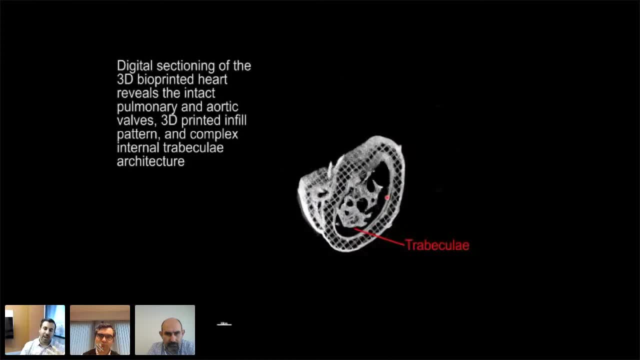 create complex 3D volumetric anatomic structure And again, while these are not yet cellularized, because that actually requires a tremendous number of cells that are still difficult to produce- the idea of producing the scaffolds itself is really starting to be addressed. 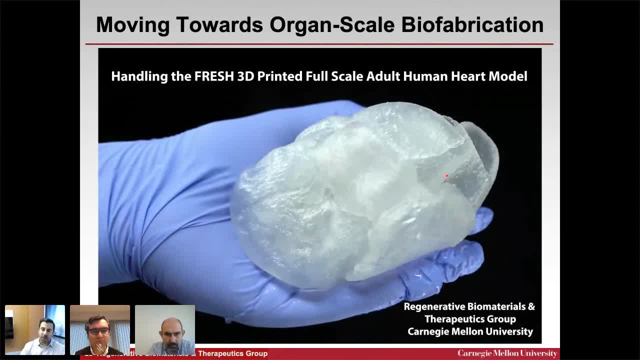 And we've kind of, really kind of, I think, taken this all the way now to full organ scale. as I mentioned on the very first slide, We just published this last week or the week before in ACS Biomaterial Science and Engineering. But as I play this video, this is again a full-size heart. 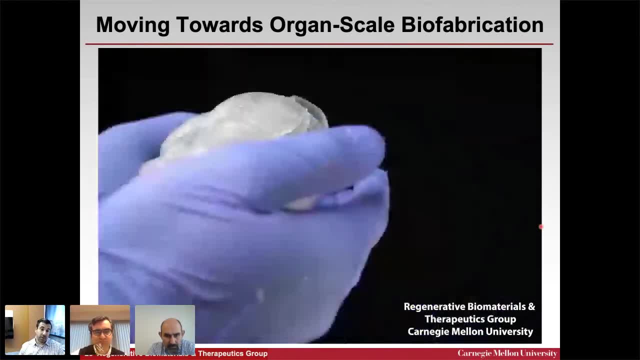 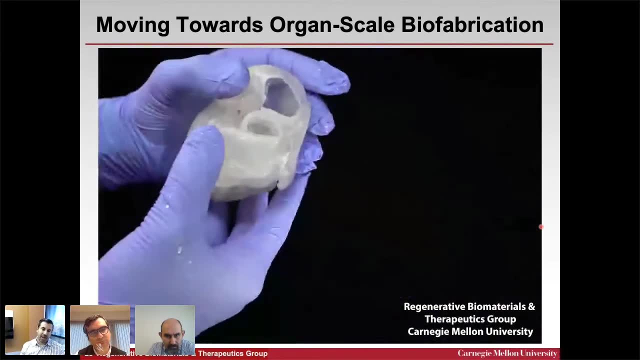 where we basically took a small bucket, if you will, filled it with our support material and printed the full-size organ. This one happens to be out of alginate. We showed that the mechanical properties can be tuned to be tissue-like and that you can also begin to think about suturing. 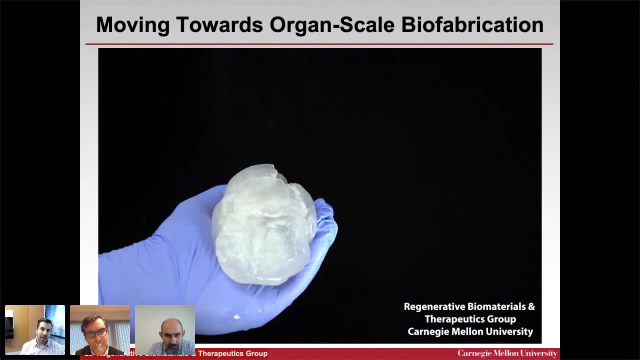 this organ, And so we've kind of, really kind of, taken this all the way now to full organ scale, hand- Oligenet in the form of this material and perfusing the vasculature, And so we think this is, you know, really quite. 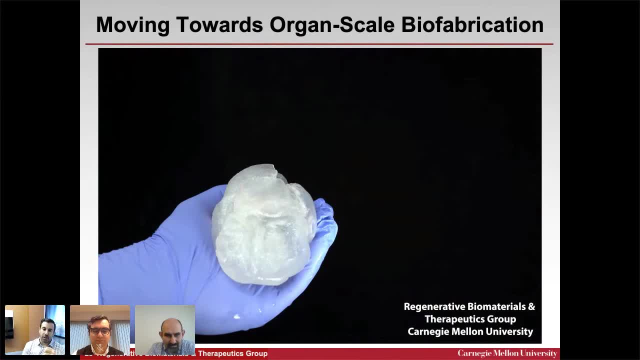 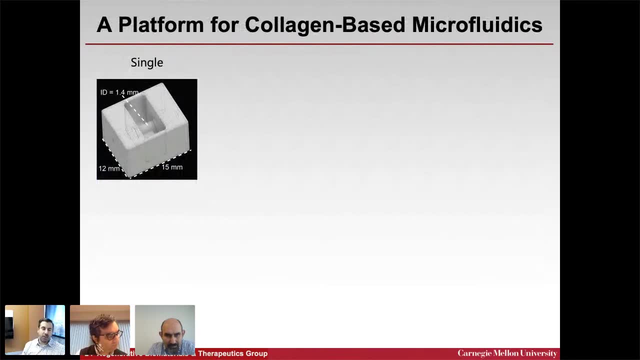 exciting in terms of thinking about how large you can go. And then you know. I wanted to talk about some of our work that'll be coming out in the near future, moving this more towards microfluidics again, since we can create. 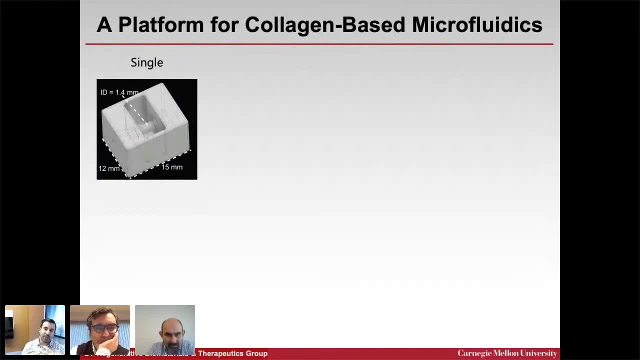 these vascular-like networks. You know, the idea that we can have a collagen-based microfluidic platform rather than a PDMS or a thermoplastic-based platform is interesting from the standpoint creating more realistic models. so here's just a few examples of some different structures. 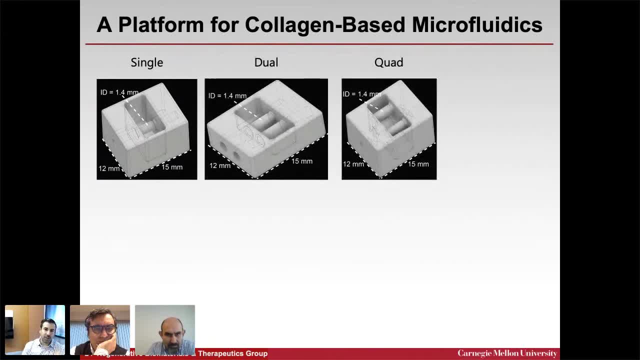 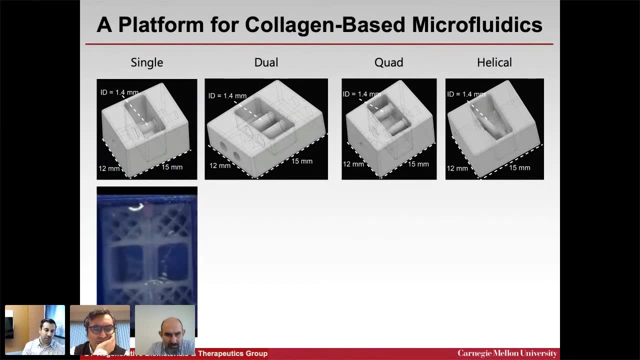 we've been building. here's just some different single, dual quad and helical channels. so again, these are very straightforward to print in our system out of collagen. we have these in these perfusion systems. uh, here you know, these are real. these are not quite microfluidic. you know the. 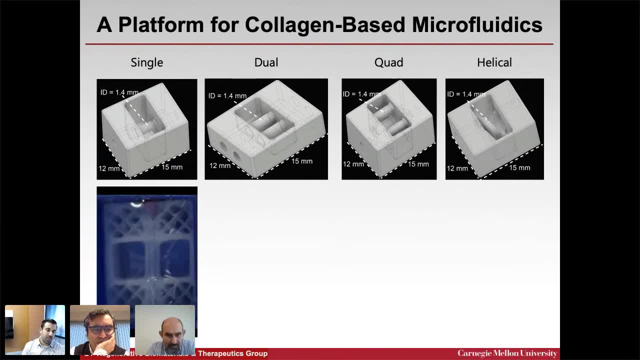 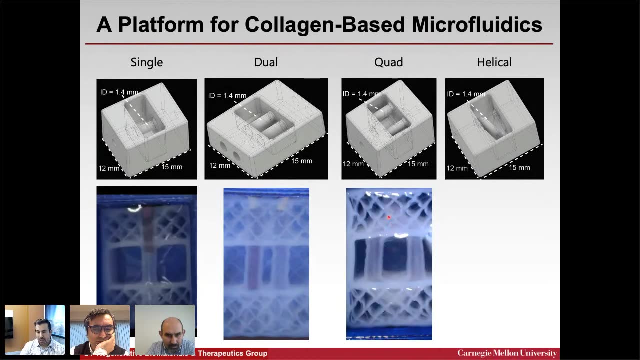 diameter here is about 1.4 millimeters internally. but again here's the single channel, you know. here's the dual channel being perfused. the wall here on these vessels is about 300 microns. here's the quad channel. so you can kind of see some of the branching we have in this area and as we play. 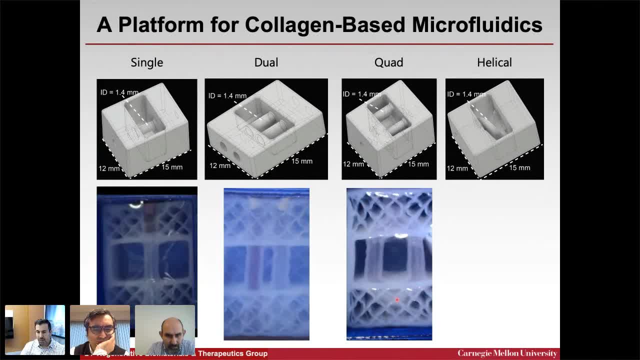 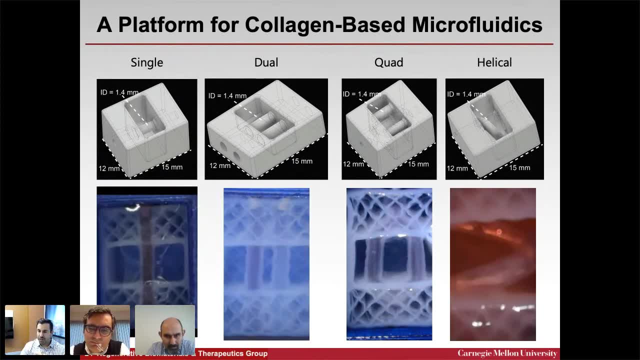 this, you'll actually see some of the bubbles that are perfused through as the perfusion starts. um, then we also have here the helical channel, so we don't just have to produce these simple linear channels. you know, we can be curved in 3d space really, however, and so the printing fidelity. 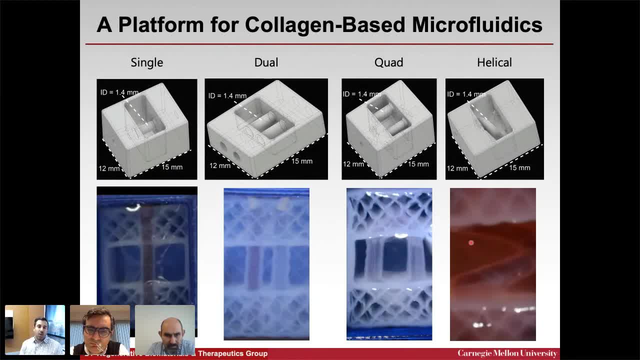 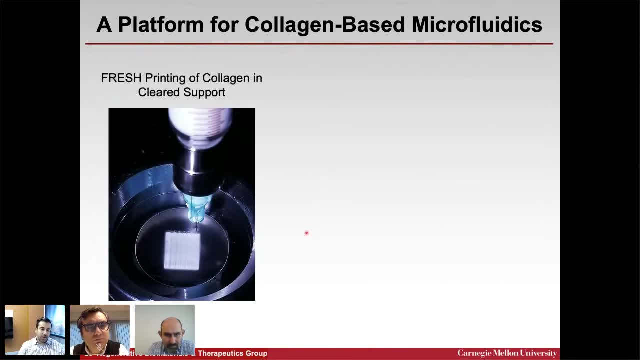 and the ability to print collagen-based systems that are essentially, you know, water tight. uh is quite good, and so, uh, we've also been improving the support bath. this is again some additional work that'll be coming out in the future. this is our transparent, fresh support bath, not a completely 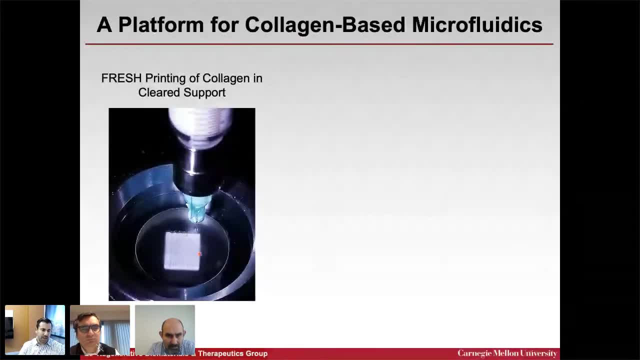 transparent, but pretty transparent where we've been able. uh, anyone who's used normal fresh knows that it can be a little bit translucent and a little bit hard to see through, but here is a straightforward collagen based device that we're printing, um we're uh, here's- it's actually a test piece to see, uh what. 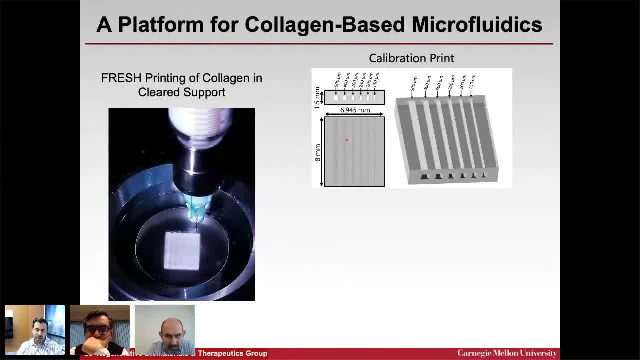 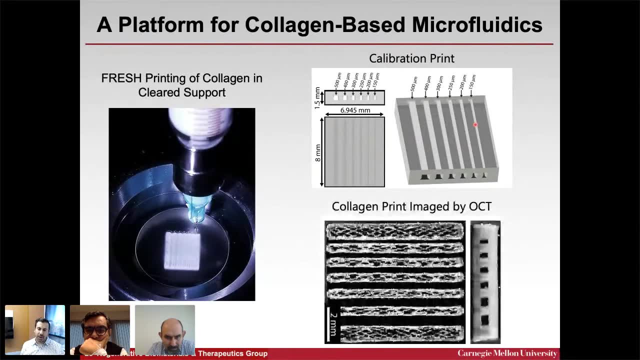 our resolution is that we can achieve. so it's this block, you know about a centimeter or square a little smaller, with 500 micron down to 150 micron with channels, and we've actually implemented an oct, so an optical coherence tomography imaging system, so we can get rapidly 3d images of our 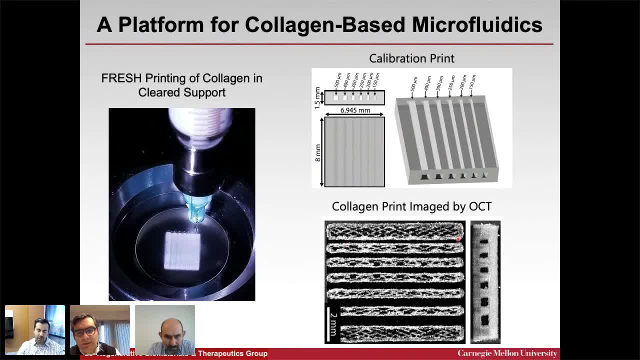 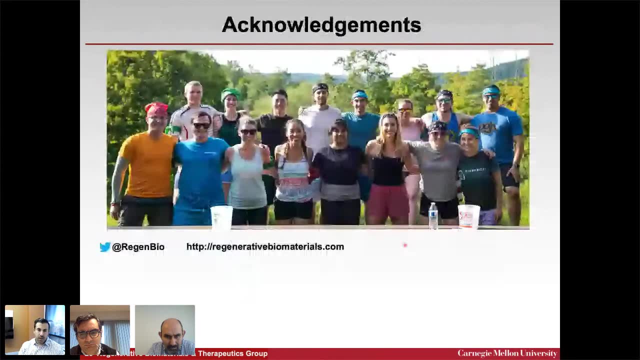 scaffolds as we're fabricating them, and this just shows you the routine, you know, resolution we can get here. this is 100 microns. you know, on our newer printers we can get down to about 100 micron with with really, really excellent fidelity. so, uh, that really, you know, highlights the work we've done. i want to really thank. 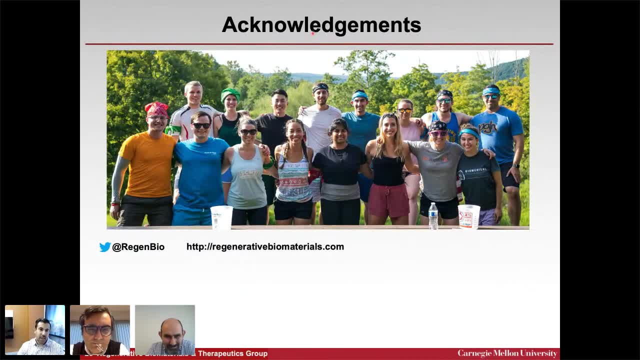 uh the folks in the lab that have made this all possible. uh, you know i have a really talented group. uh, josh tashman uh was key on developing uh the the cleared, fresh support and a lot of our students have been doing some of the micro fluidic printing. uh, andrew hudson did the valve printing. 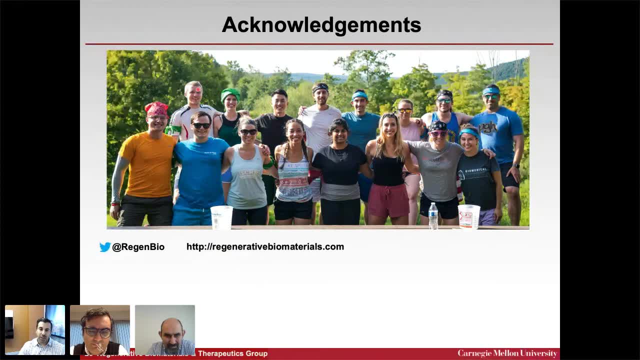 and has been doing those perfusion uh studies on some of the microfluidic work i showed uh. andrew lee, uh really drove the work on the 3d bioprinted ventricle. uh. dan shawarsky is doing, uh the work on the microfluidics, the oct uh in a number of other areas that he's contributing to. 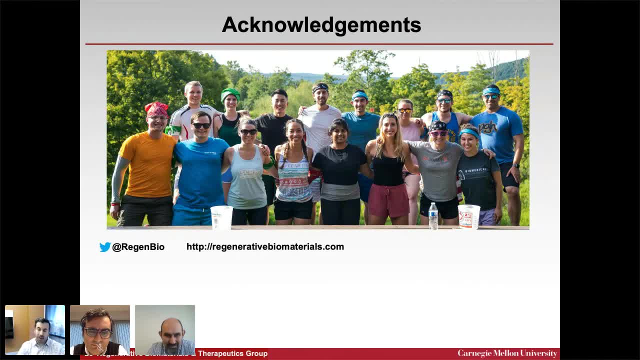 iman murtamati, uh, with a master student who's now at the university of maryland, who led the work on that full-scale bioprinted uh heart, um, and then obviously we have a lot of other talented folks doing work that i wasn't able to. 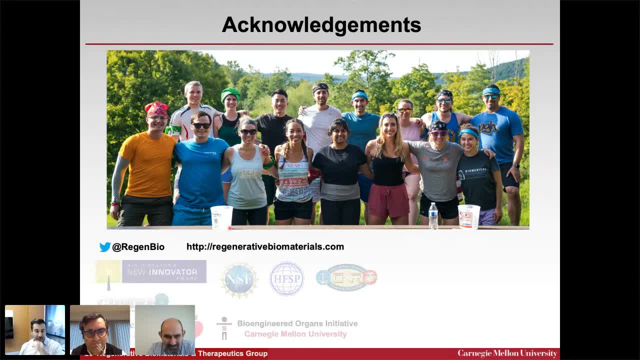 share. today we're on twitter and we have a website and i'd like to thank the funding support uh from nih, nsf, department of defense, american heart association uh, human frontier science program and then, obviously, the disclosures: uh, i am a- you know- co-founder and the cto at fluid form i'm also. 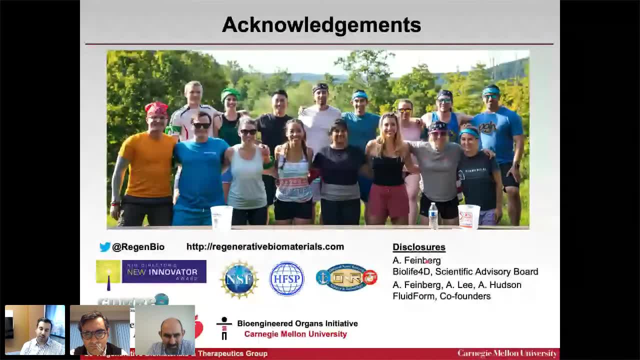 on the advisory board on biolife 4d, which is working on a bioprinted heart. i did want to, before i finish, cover two kind of things that i love to share. i think they're both exciting in different ways. the first is our 3d bioprinting open source workshop, so we actually have done all this work. 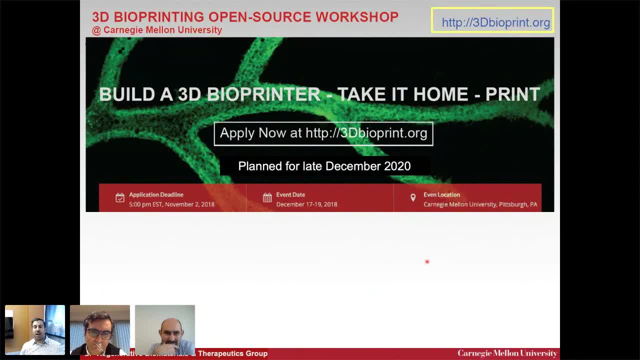 on desktop plastic printers that are open source. we created open source designs that basically turn them into bioprinters that we've published on, we've released to nih 3d print exchange and we also have a workshop we now run. we ran it in basically. 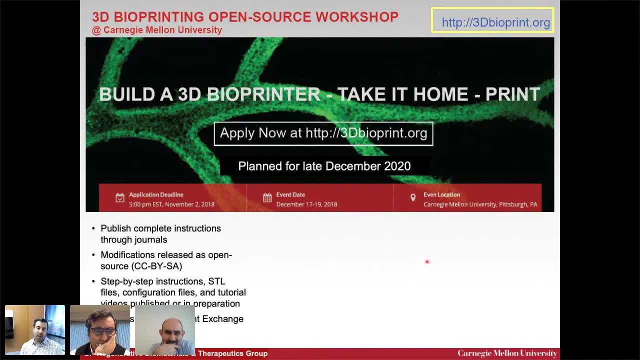 december of 2018 and 2019. we're not running it. this year, uh, we'll actually have a virtual workshop, uh, that we're going to be posting information about soon. that'll probably be in january or february. but basically, you can come to cmu, build your own open source bioprinter and take. 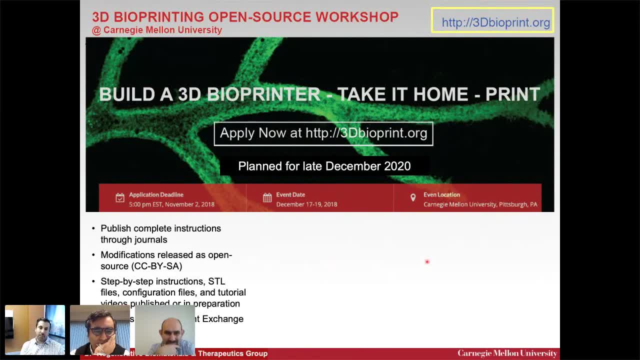 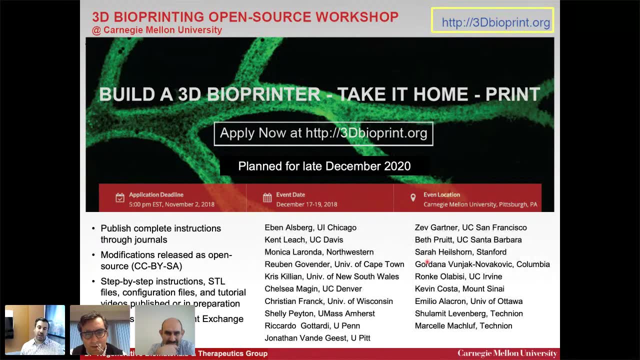 it home with you, and we've really seen this as another way of trying to grow the number of labs that can be successful in bioprinting. this is actually just a subset of labs that have either worked with our lab directly or attended our workshop. it's really been exciting, so we have 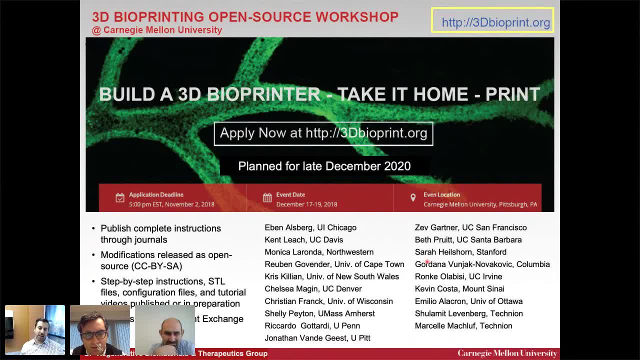 grouped some really all over the us as well, as you know, korea to, to australia, uh, to israel, to europe and the united states and all over the world, and so we're really excited to have this workshop and it's really been exciting, and so if you're interested, please go to this website. it hasn't yet. 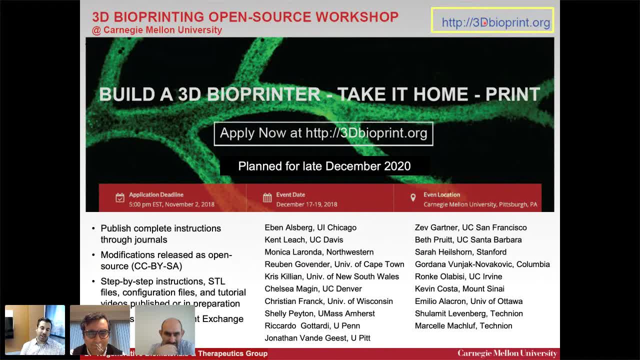 been updated, but it will be soon with information about our virtual workshop and then, hopefully, once covet uh is no longer- uh, you know, interrupting or uh really disrupting our lives, we'll go back to the in-person workshops here at cmu and then, as a final piece, if you're interested in, in fresh. 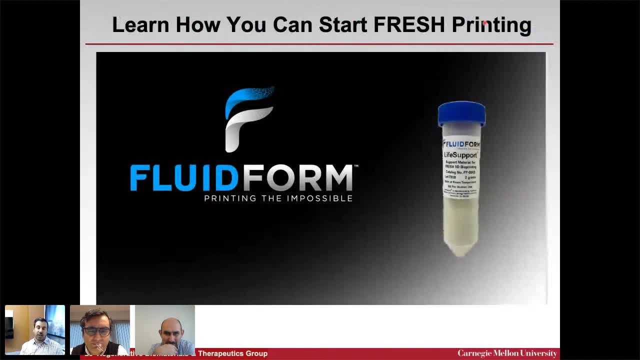 printing. you know fluid form. you know again, uh, this is the startup that's been commercializing this and it's been dabbed in our lab. uh, we've done a fair amount of research on this and you know, uh, the, the, the one quality, and the uh, the value of the material is. you know what they're good for. 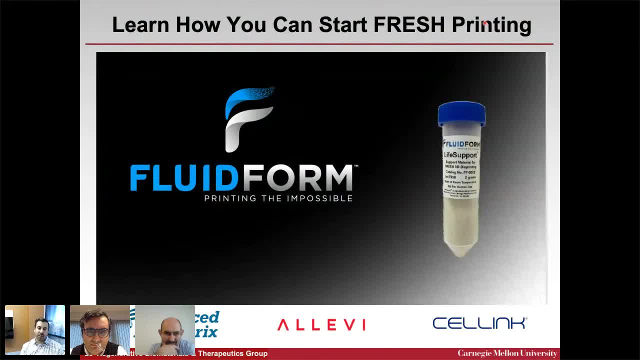 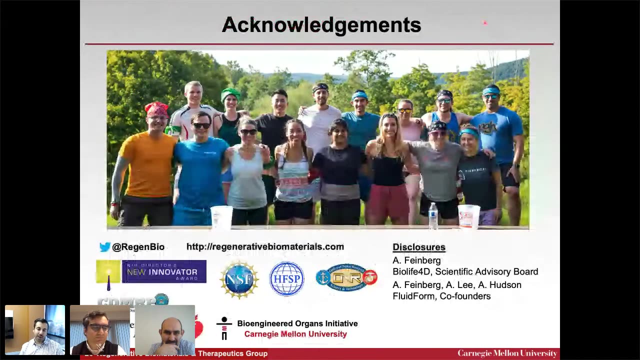 and you know if you're interested in doing that. uh, we've- we've partnered with advanced biomatrix, elevi and selen. they all resell this life support material. so please go to your favorite um either bioprinter company or supplier and- and you can, you can buy this to try it out. so 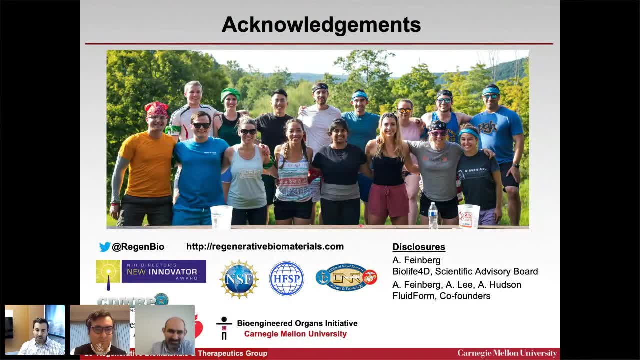 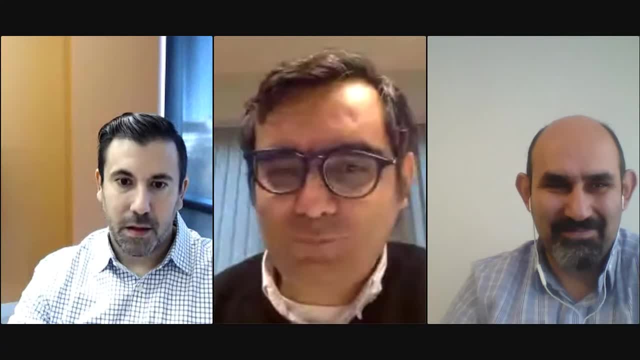 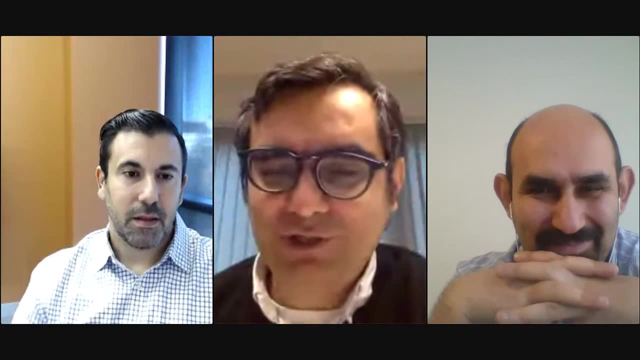 answer any of your questions. Thanks, I think I'll end the screen share now. Well, thank you very much, Adam, for your very, very nice presentation. You didn't see our faces, but you're all surprised to see your new technologies and new results. So very nice work. 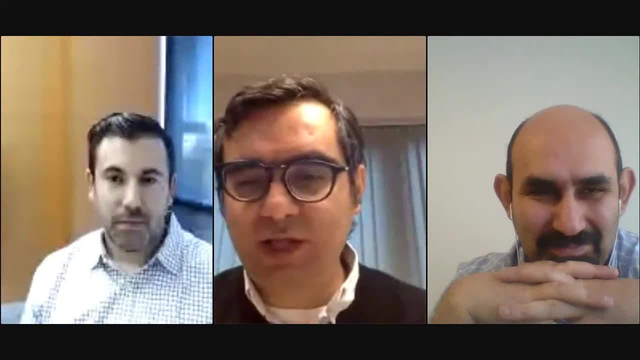 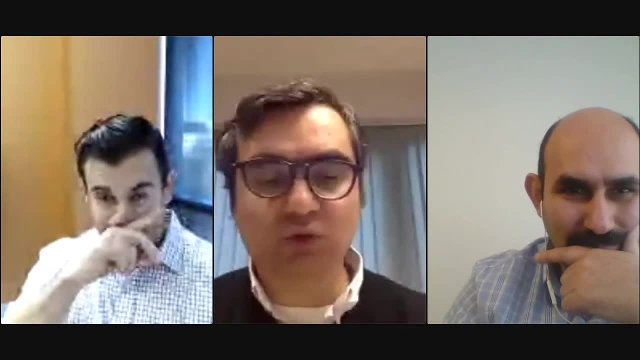 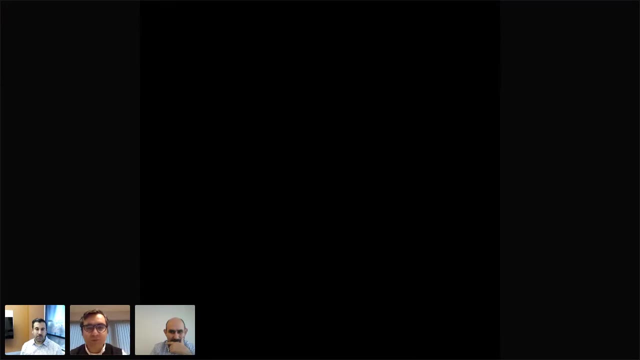 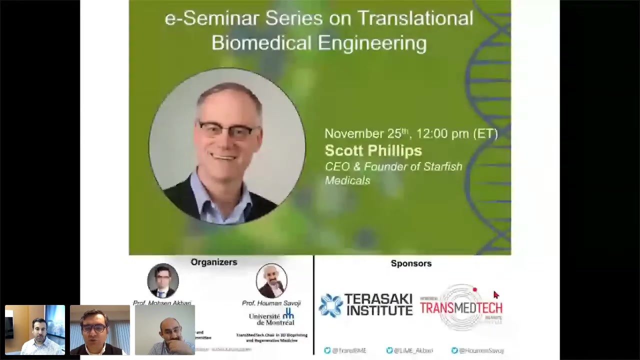 as always. So before we start the q&a, I would like to make a few announcements. First of all, our next speaker is going to be Mr Scott Phillips from Starfish Medicals, one of the largest biotech companies in Canada, So please make sure that you mark. 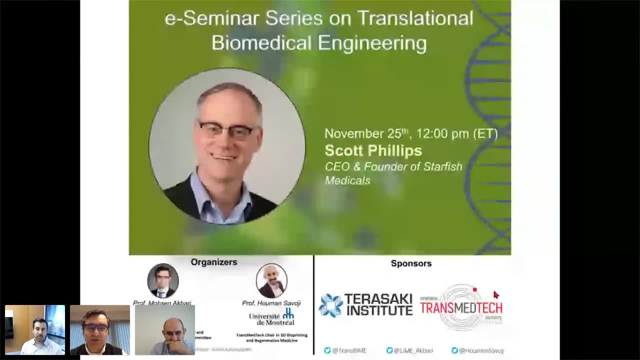 your calendar and and participate in his talk. I have participated in in his few of his talks and then it's, it's exciting, It's extremely inspiring. And then also I would like to thank again our sponsors and transmit Montreal, transmit tech, and then 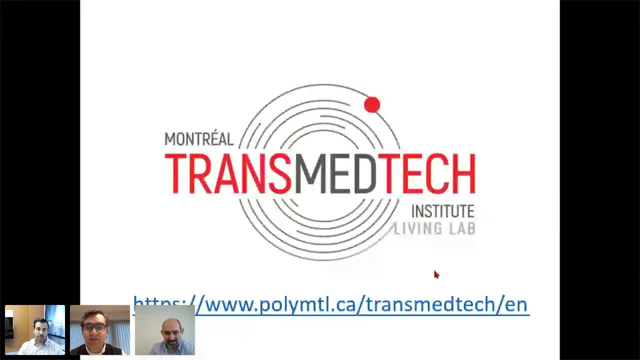 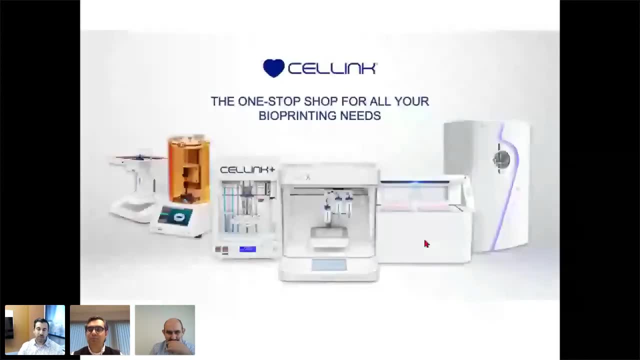 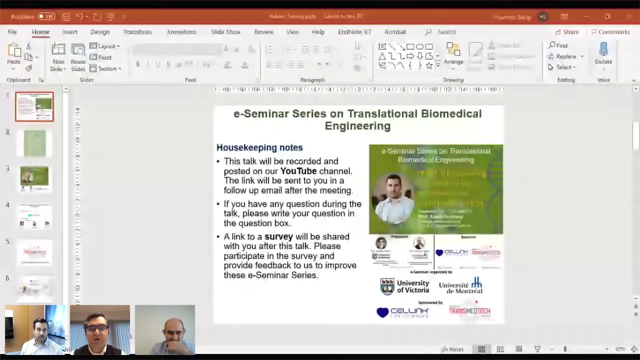 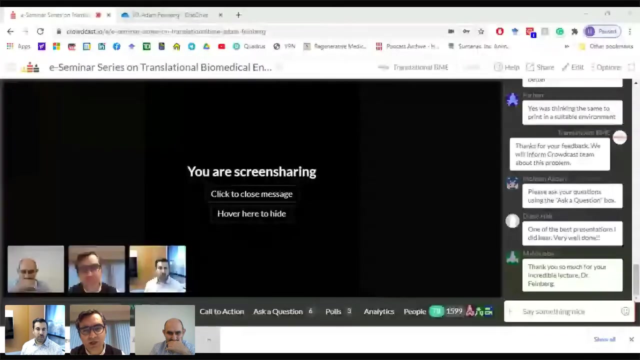 also selling for supporting this, this talk. So with that, I would like to start with the questions from the audience. So we have the first question. The first view question is from DS. I hope. I hope I pronounced or DS your name correctly, So the 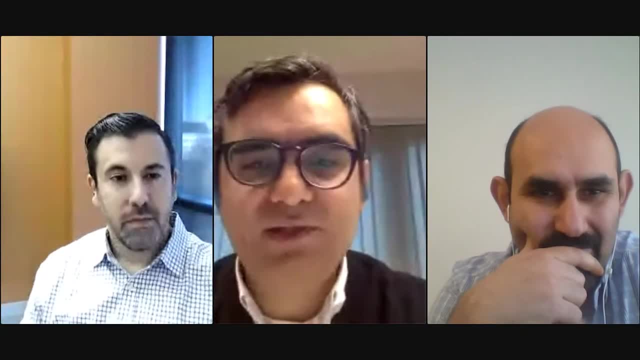 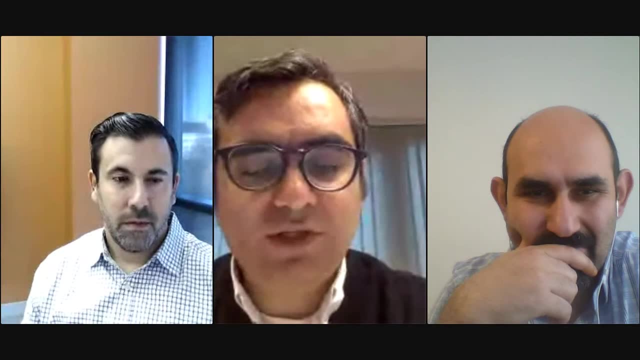 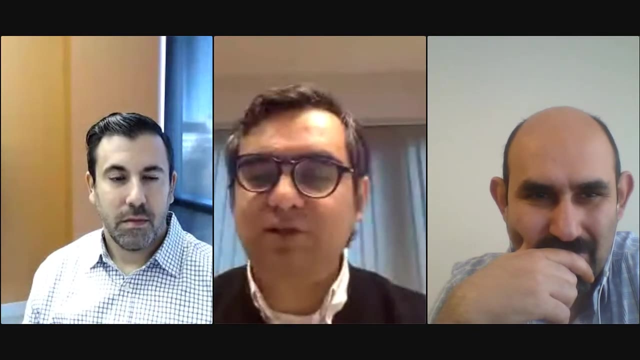 first question is about the sterilization of the heart valves that you- you have made. So is collagen. Is it possible? or let me just rephrase it: How do you sterilize the heart valves that you create before, Let's say, you want to implant them in the 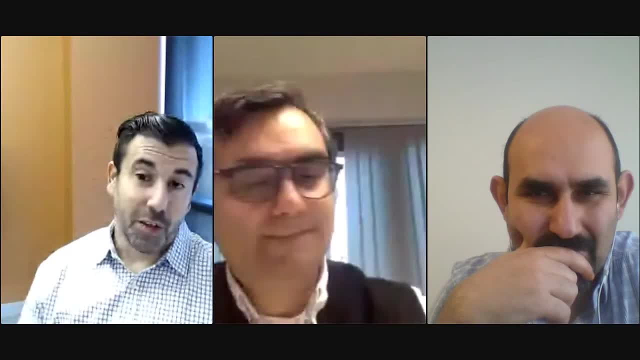 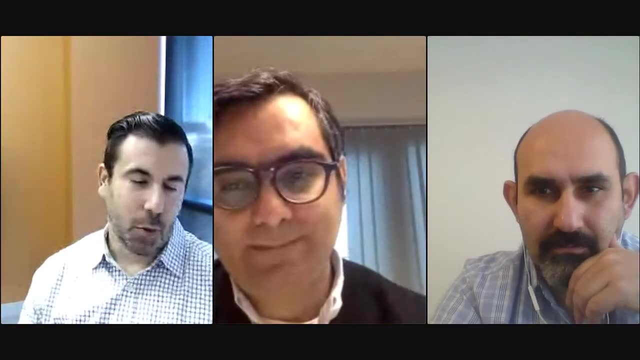 body. Yeah, so the heart valves themselves have not yet been implanted, but we have implanted other constructs, So you know just a. so there wouldn't really be much of a difference because they're still collagen. But really, first of all we produce. 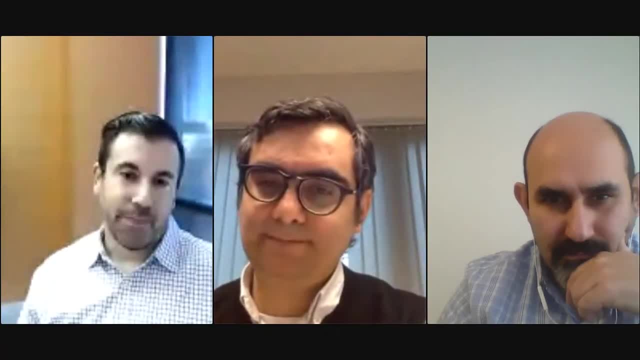 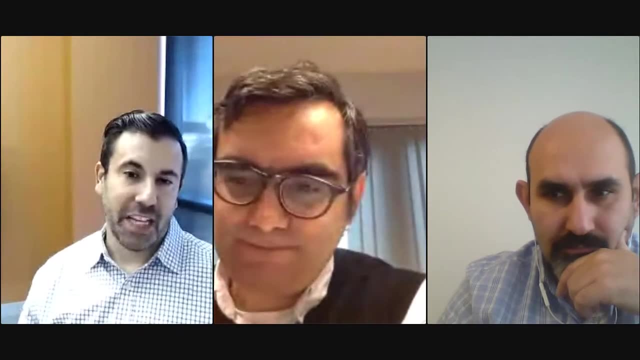 the support material under sterile conditions. Sometimes we make it ourselves. Actually, sometimes we actually buy it from the startup that we have, because it's already lyophilized and E-beam sterilized, So it's really great for cell based. So that's basically: you start with sterile support, you use sterile. 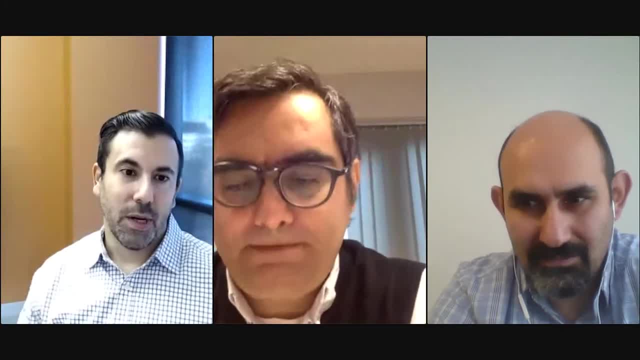 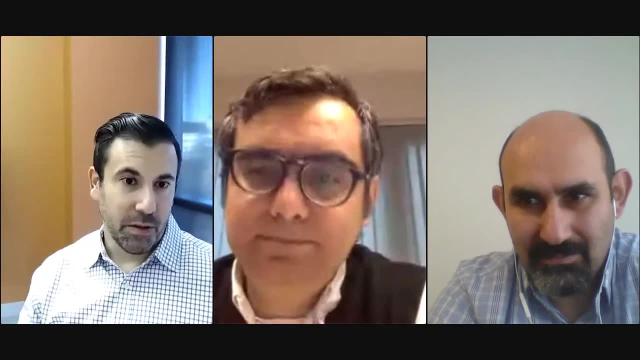 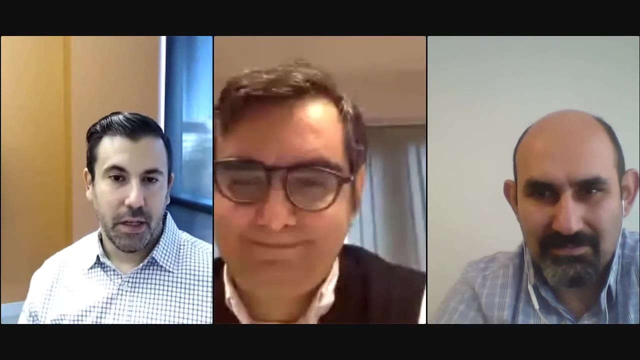 collagen. we do all the printing, the biosafety cap. So we've done that. We have done implantations, both subcutaneous in the mouse and then also a surface wound. We're doing for some volumetric muscle loss studies in a large animal model And we've used the 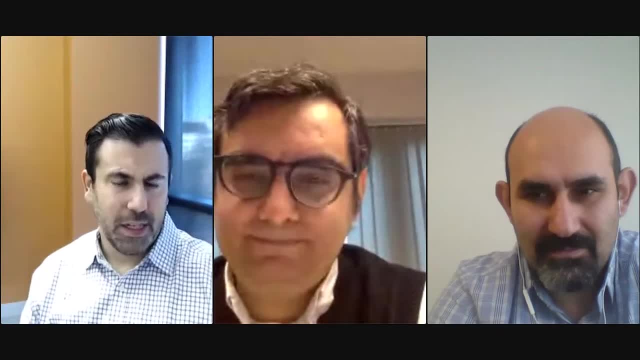 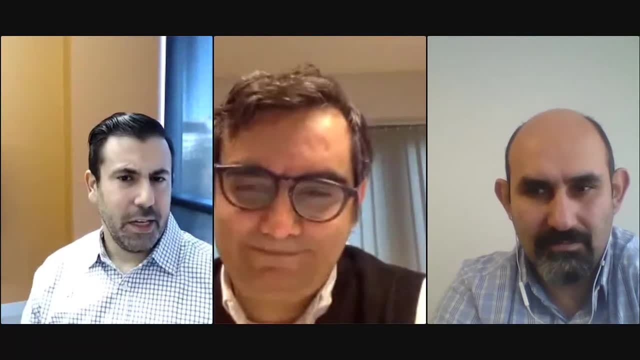 approach. in both cases I don't think we've had any infections yet. Obviously that is not as good as a post sterilization process per se, But you know it's actually difficult to sterilize collagen without altering its properties, And so 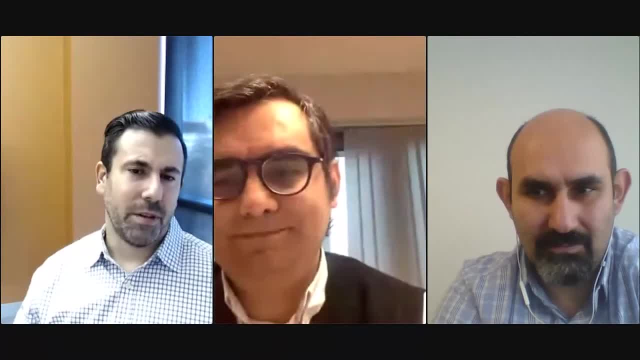 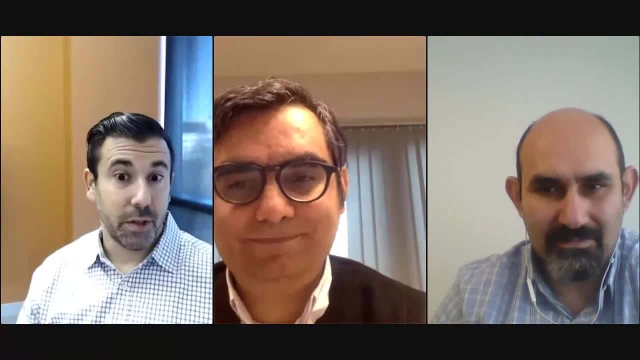 this is just a you know, a challenge, I think, with any bioprinted ECM or bioprinted ECM and cells- right you're, you're? there's not so many post sterilization processes available, So it's really about maintaining sterility during the 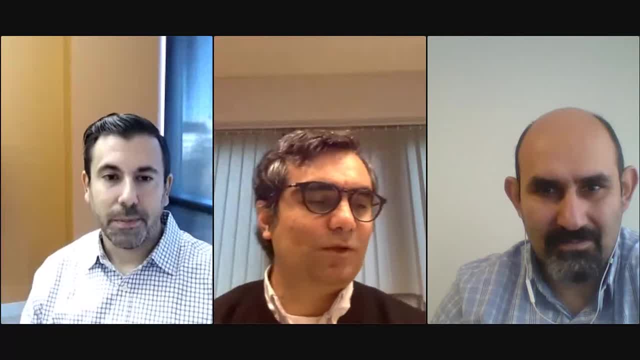 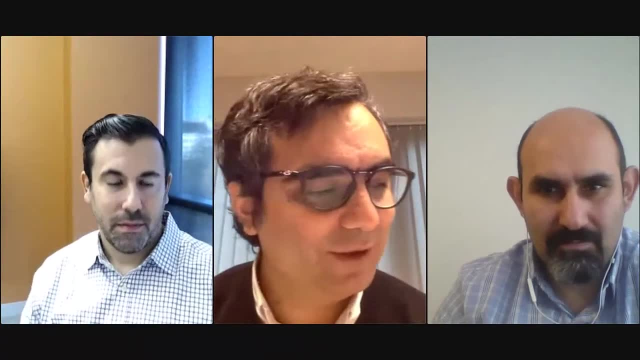 manufacturing or fabrication process. So yeah, I mean, I mean I agree with you. And then we're working on some of these uh sterilization issues with the high level gel that we're working with And we tried gamma sterilization and it's completely changed the you know. 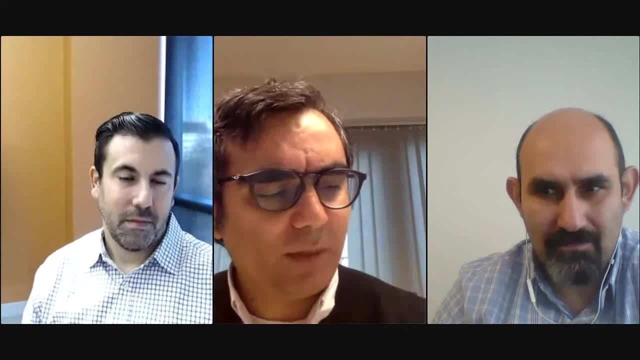 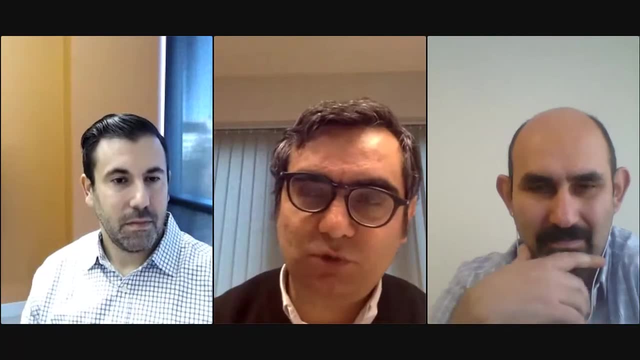 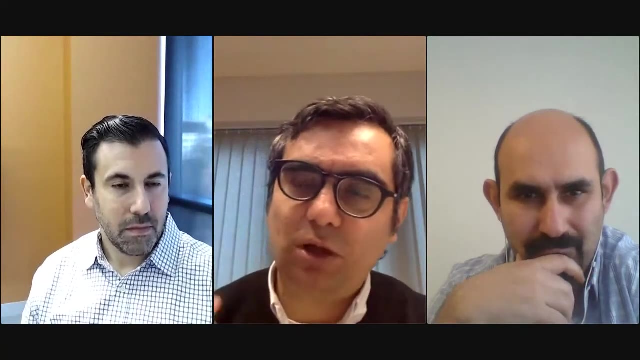 the structure of the gels that we were using. But I mean, I mean that could be a challenge, as you mentioned. Let's say that, like towards tomorrow, towards commercialists, or selling these heart valves to you know, or you know, to patients not. 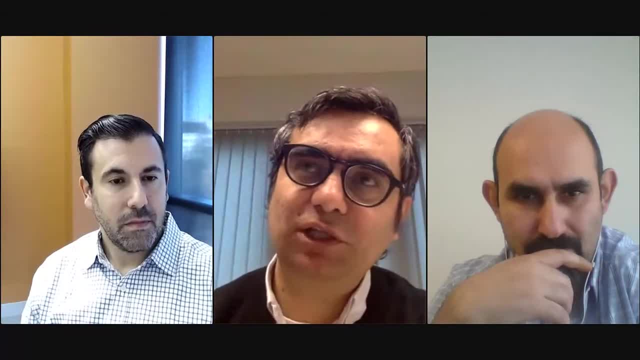 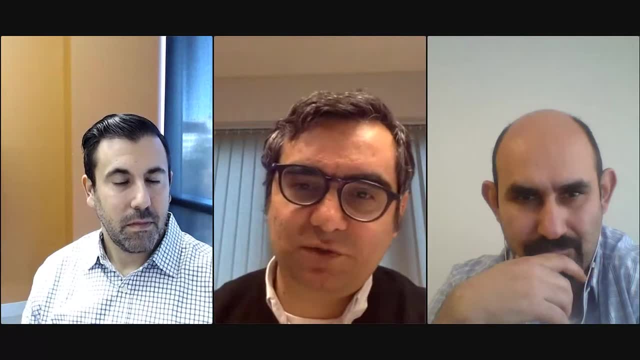 not to patients, But you're using them in patient because eventually, the ultimate goal is to make these heart valves, and then you know, giving it to clinicians so they can just, you know, place it in there, you know, implanted in the body, and then you probably 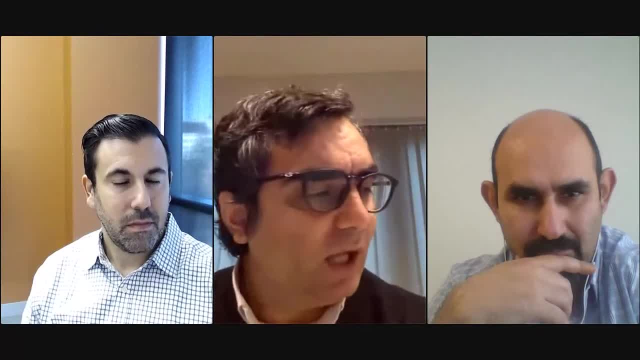 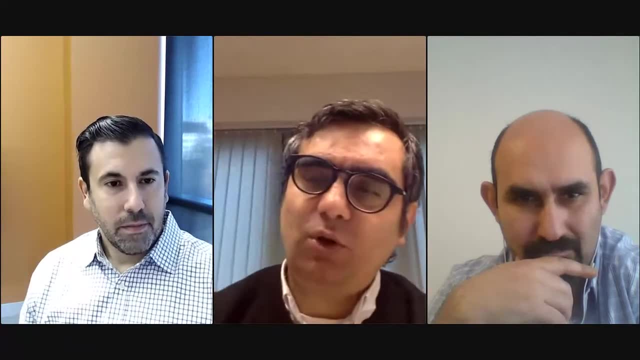 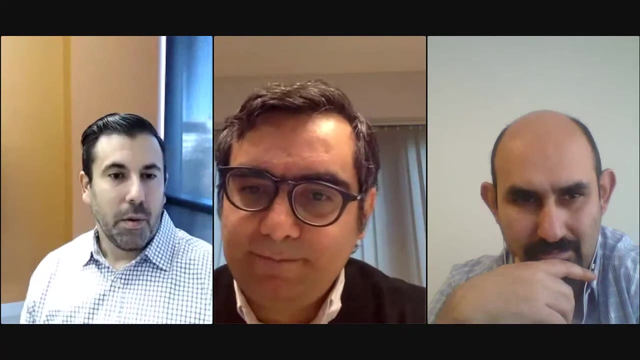 need many of these heart valves. So so, what are the challenges besides these sterilization approach that you see, Or what are the barriers against, you know, you know, bringing this into clinic? the heart valve technology Dr. Well, I mean I think the big, I mean there's, there's two 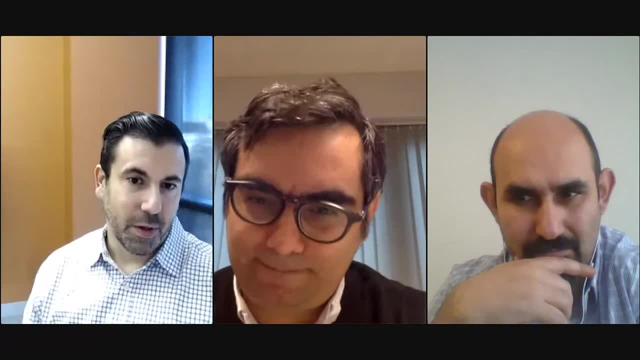 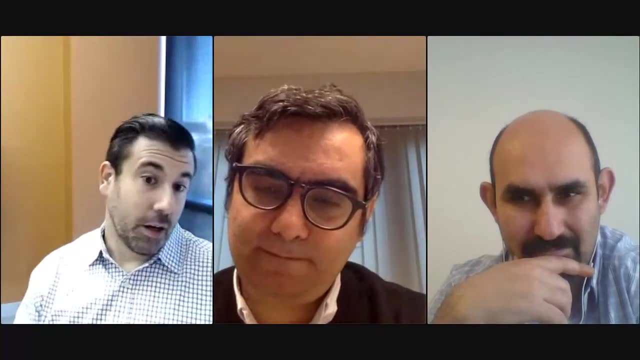 big issues with the heart valve. right is: can we get the mechanical performance that we ultimately need And can we get the biologic response that we want? Right, You know, because you know what we're trying to, I mean our vision. right is: 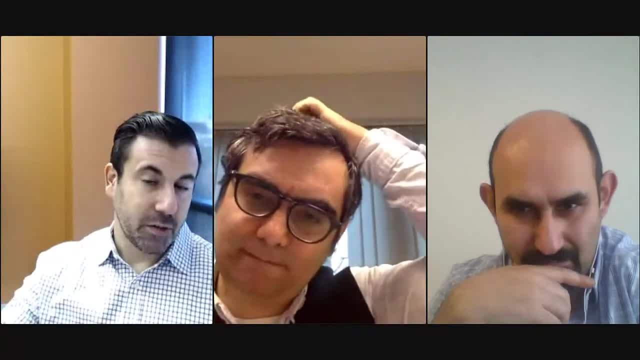 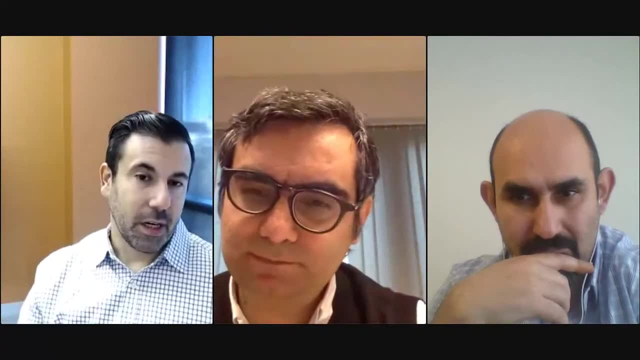 that we get the biologic performance of the current biologic valves, which is clinically. patients do not need blood thinners right? That's the big advantage. They can also be delivered through a Cherens catheter approaches endovascularly. 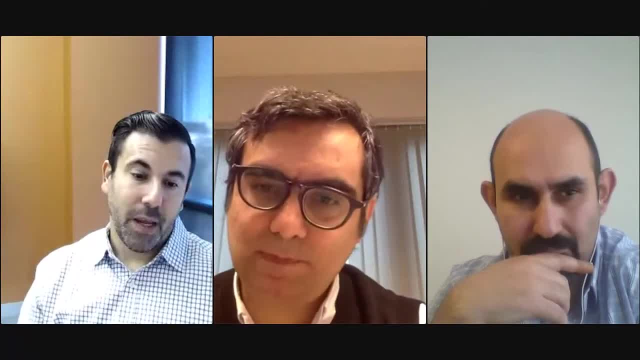 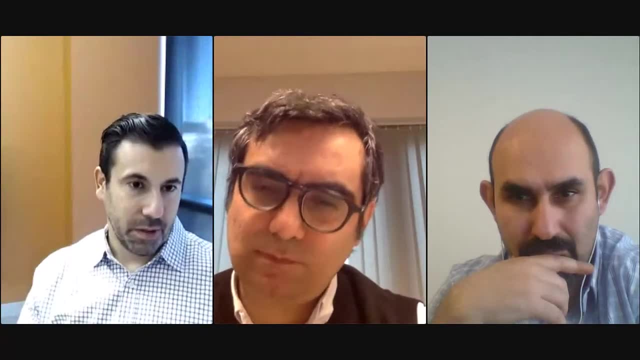 right, So that's also great. you don't need open heart. So we think we can. we can achieve that. I think we have some advantages there because we can tune the biomaterial we're printing right, So we can print collagen. but we can think about. 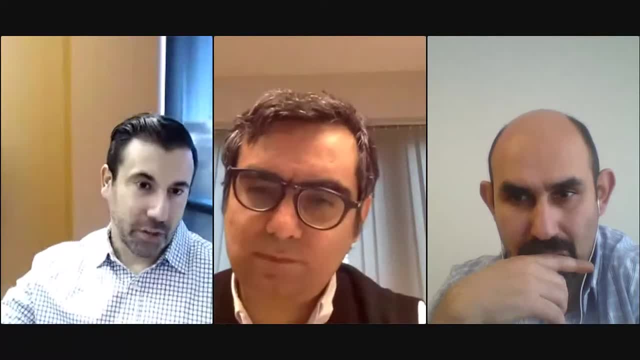 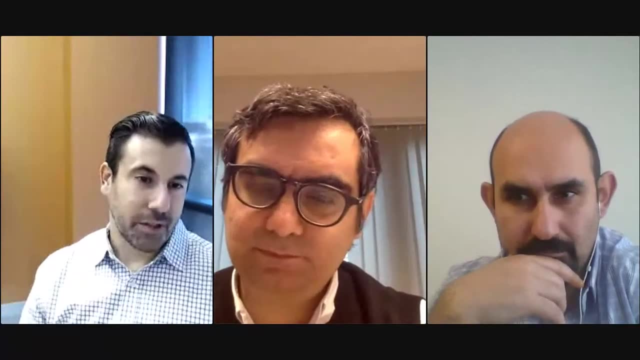 adding additives or other compounds that might slow the calcification, which is the major risk, right, We don't necessarily have to use glutaraldehyde, which is known to enhance calcification, So we have, I think, some options there to improve the material. Now, that's not our strong suit. 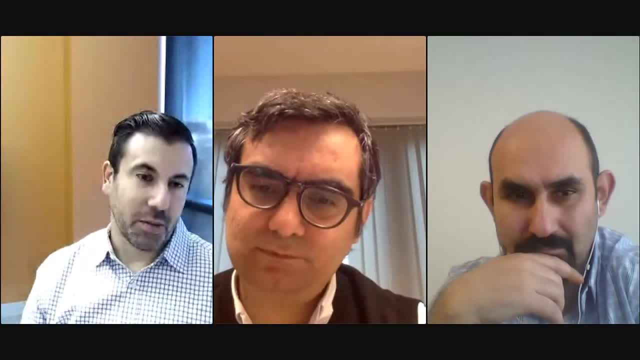 per se, like in our, you know in our lab, but you know working with other people. So you know that's that's, you know that's that's, you know that's a good thing, But we 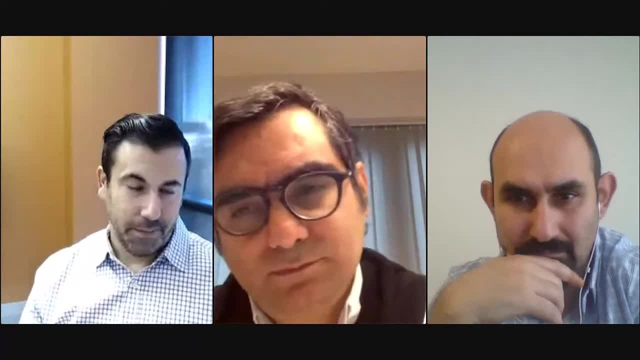 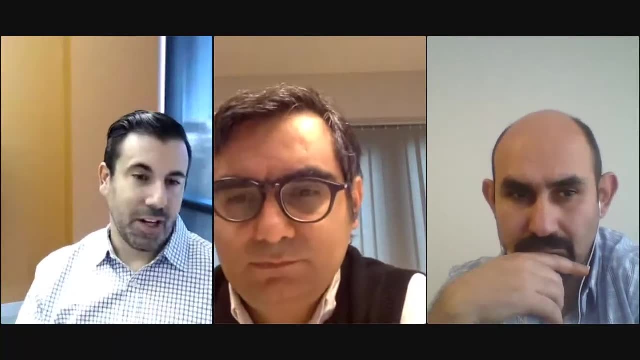 also like the idea that because we designed this in CAD, we can manufacture it to potentially better fit for transcatheter delivery. it better folds up right, Because you know otherwise people are trying to make other things work- that you 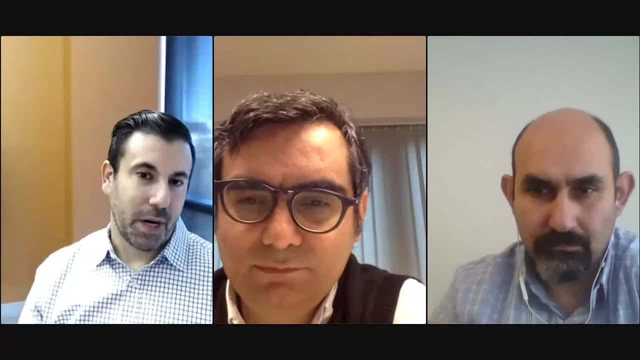 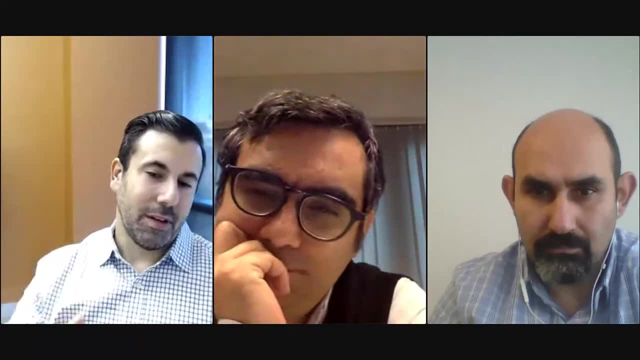 know are difficult to do, like an existing valve or whether using pericardium that you sew, which is another approach to doing this. We also think you know, in a more advanced valve you could potentially do a patient specific right, Because 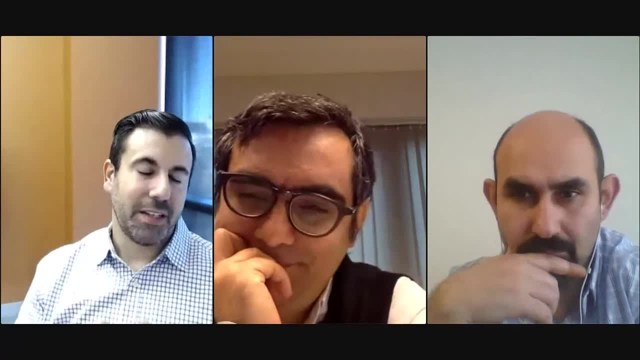 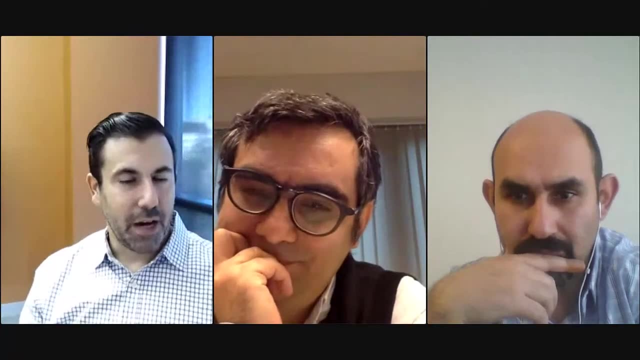 when you use a porcine valve or even the standard valve, it's a. it's not a one size fits all, but there are set sizes and not every patient, every patient anatomy is different. So can we think about in the 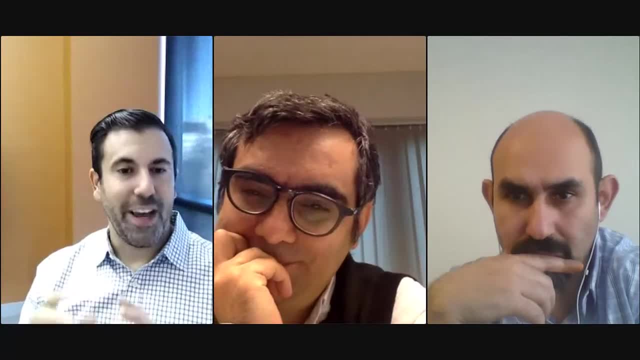 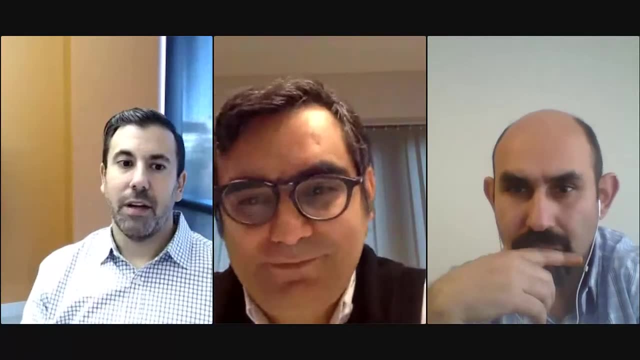 future using computational modeling to determine what's the optimum valve design for the best flow condition in that patient, which could also even help with things like calcification right. Can we actually then design a patient specific valve and then manufacture that, getting the 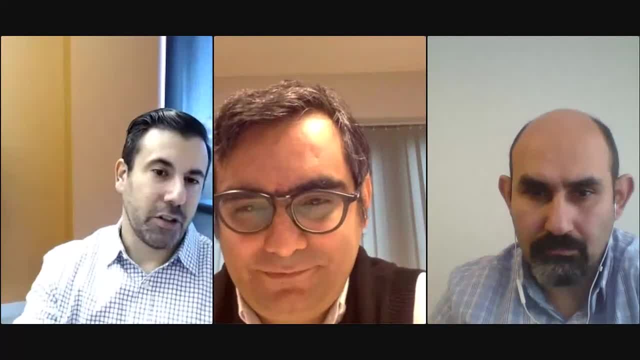 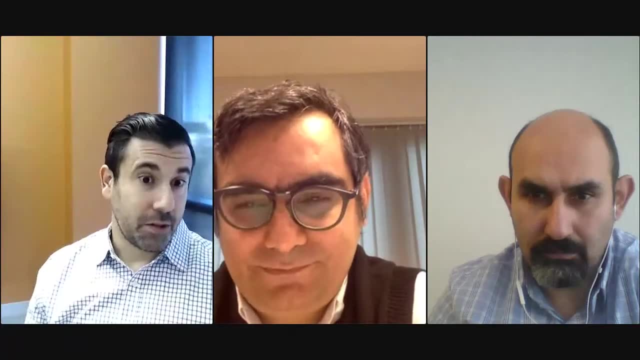 manufacturability you get out of the printing, but by making out of collagen you get that calcification Right, that collagen biologic performance right. That's the vision. Now achieving that again comes down to actually getting the right material properties, getting the right 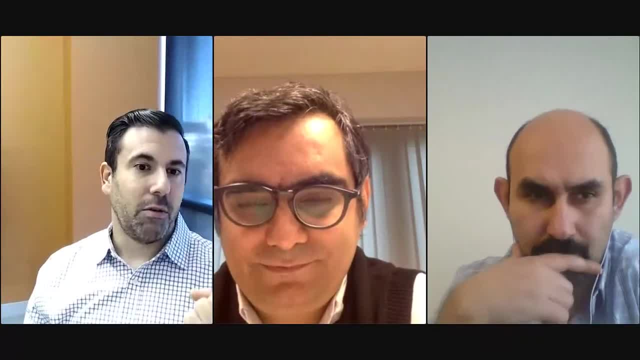 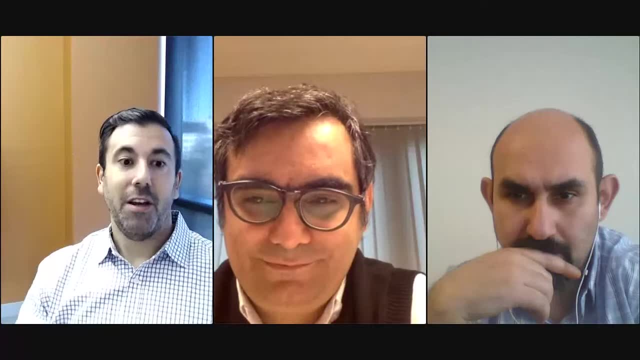 mechanical strength, actually figuring out, how do you, through a regulatory process, get a valve that is unique to each patient? because typically right you when you manufacture a valve, you do a lot of them and you take a subset for destructive testing. But that might be really expensive with 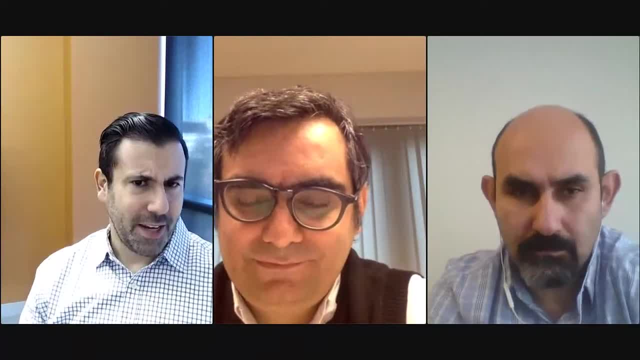 a patient specific valve to do it that way. So what kind of in silico testing can we do? You know what is the, what is the value? What is the value of the product, What is the value of the validation, quality control process from a regulatory? 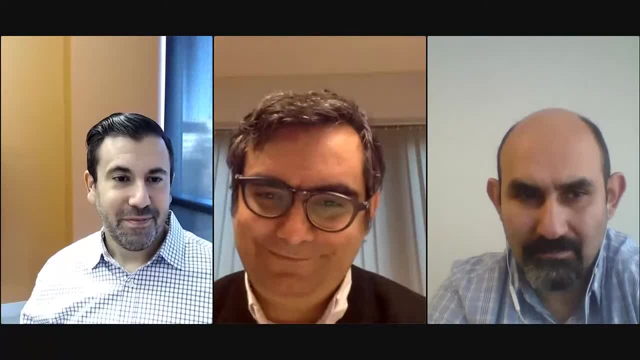 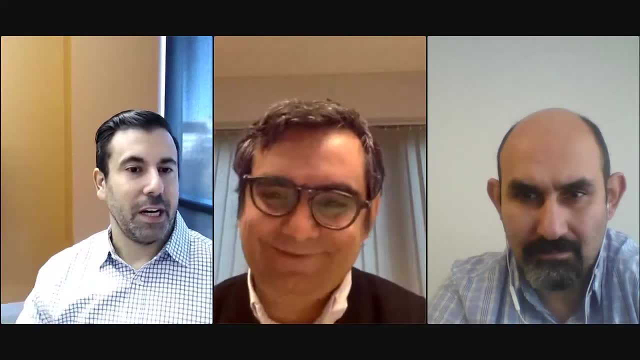 standpoint as well, that all needs to be worked out Right. That's why you know these things are going to take some time, But I think you know, I think we've all seen this field is accelerating in terms of what we can do And we're starting to. 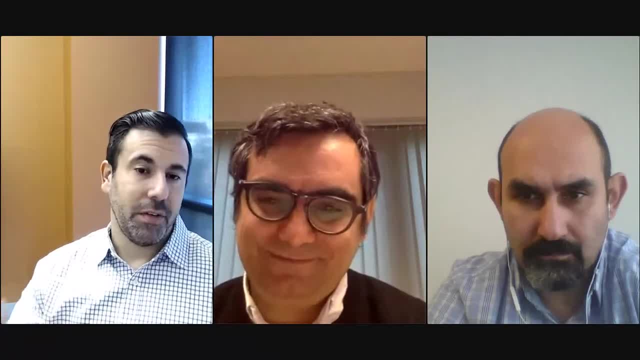 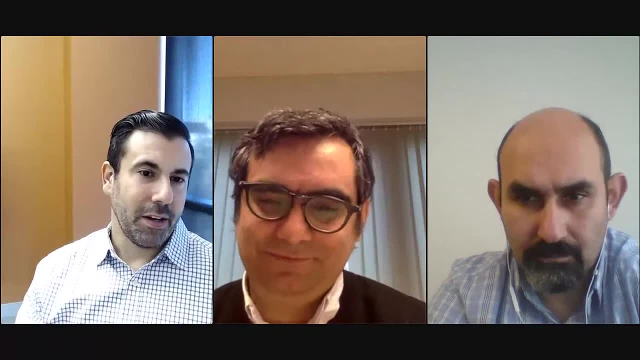 get the investment as well, right, Because all these technologies, I don't know it's if it's so much an if anymore, it's more of a when and a lot of the when is a financial. there's a lot of. you know what are the? 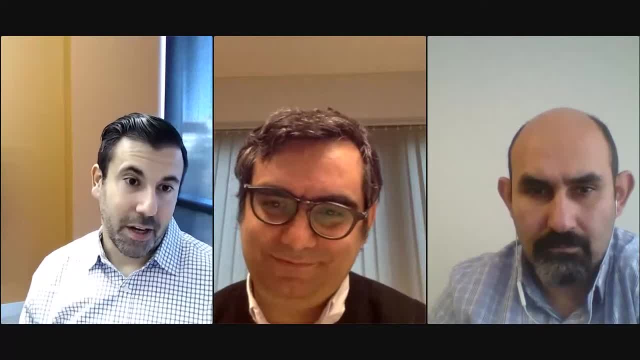 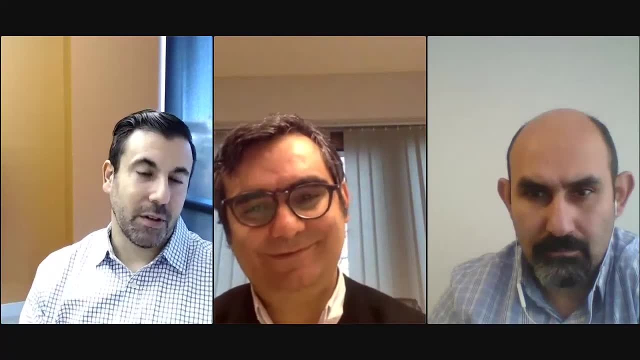 resources that are being brought to bear to translate some of these technologies. I think that, then, is answered by what's the profit, You know, what's the commercial right, profit driver, the market size right for these, for these devices, And so I think we're still searching for that torch. 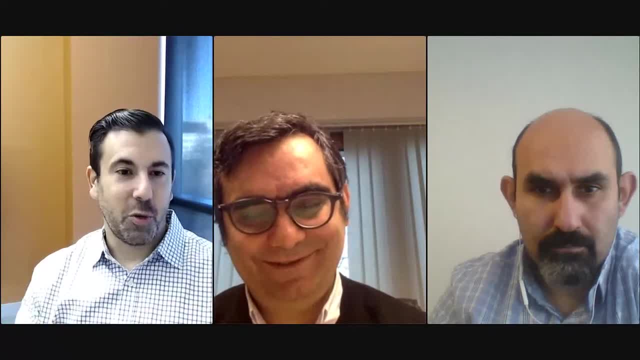 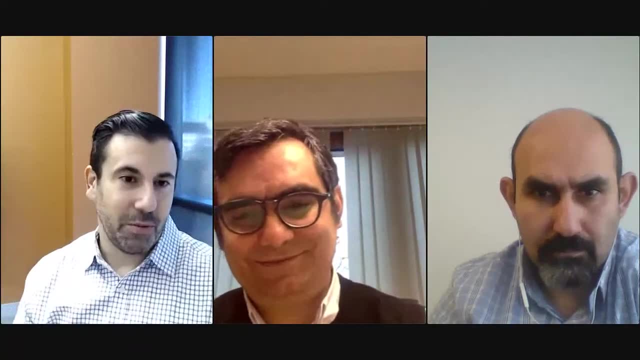 bear like what's the first thing that kind of is? the is the sweet spot of like: oh, bioprinting is a killer advantage, right, But there's also a large enough market, right, and we can make them cheaply enough. And then the? 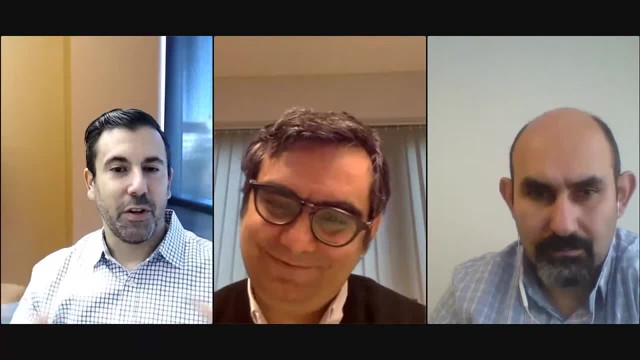 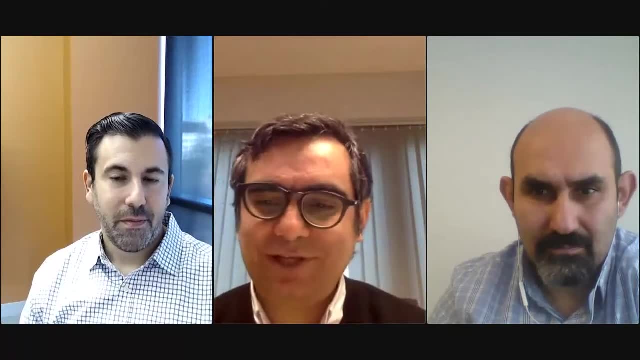 regulatory hurdles are not too high. I think we. I don't think the field is quite got in there, But I think we're rapidly converging. Okay, that's great, That's good, That's promising and encouraging. That's that's awesome. But along the same, 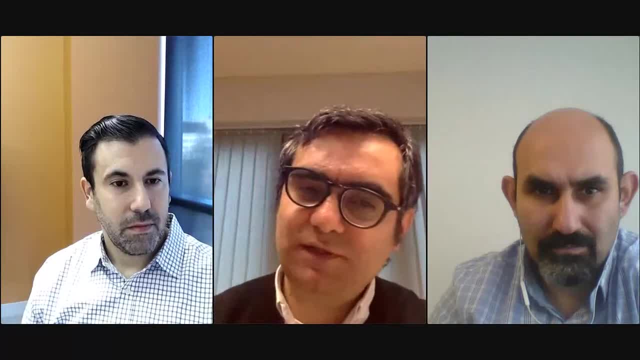 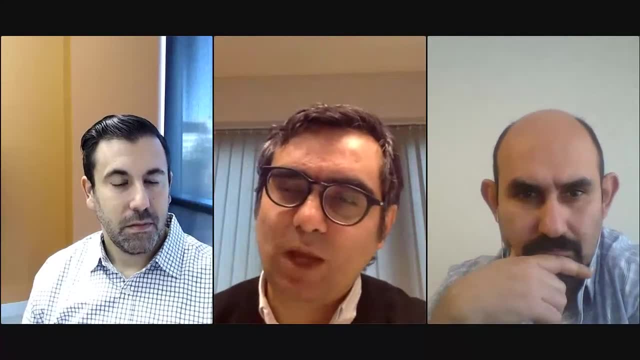 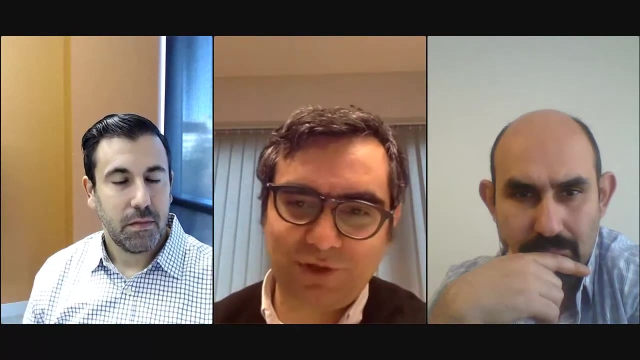 direction. Do you see these technology, especially the fresh bioprinting which enables creating complex tissues? Do you see them being used by clinicians in the operation room? So they, they put, they have this print, They have this printer in the room, They have all the MRI. 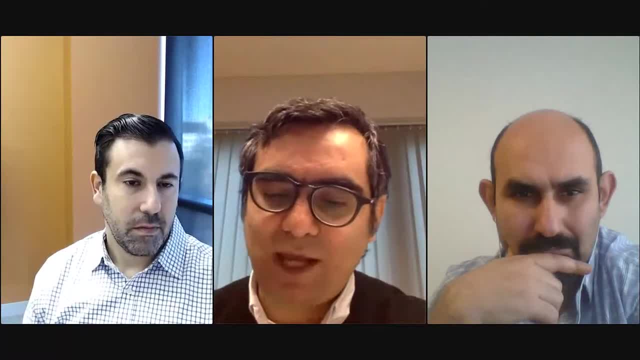 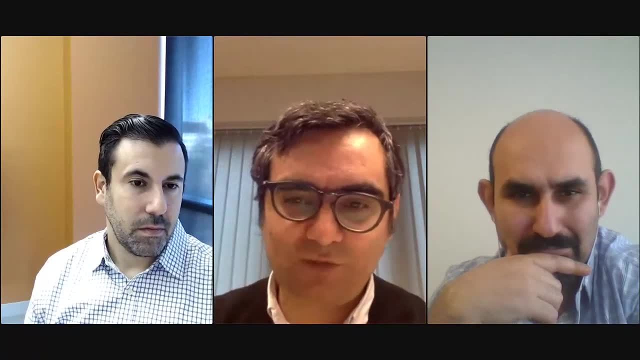 images from the same patient that they're going to like operate, And then, while they go or prepare the patient, they'll just hit, press, you know press print, and then they print the heart valve and then take it from the bath and then put it in. 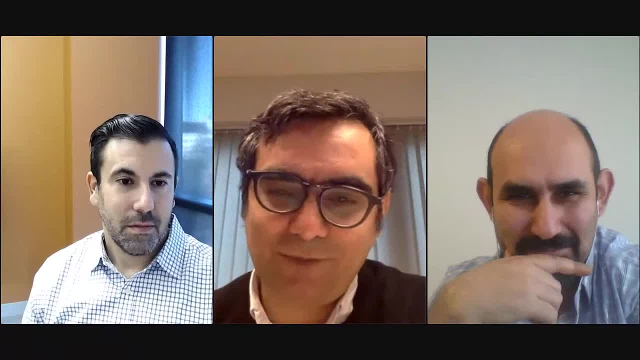 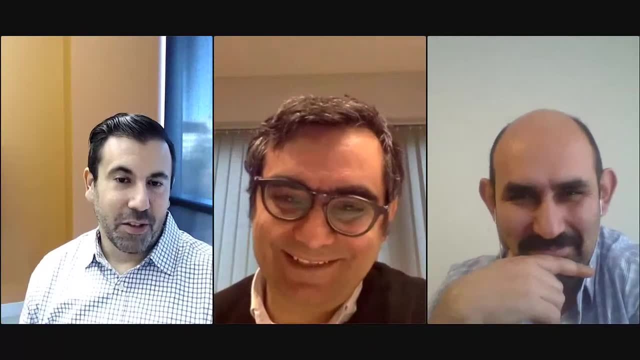 the look or implanted in the patient. Is that something that you envision happening anytime soon? Not anytime soon, I do think that is a potential option, I think one you know. one of the advantages with with medical imaging is that we don't necessarily need to have it as 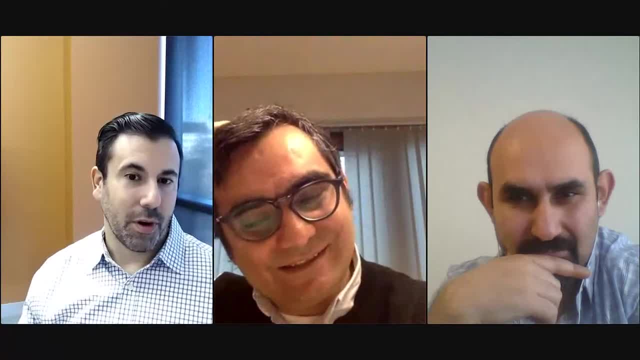 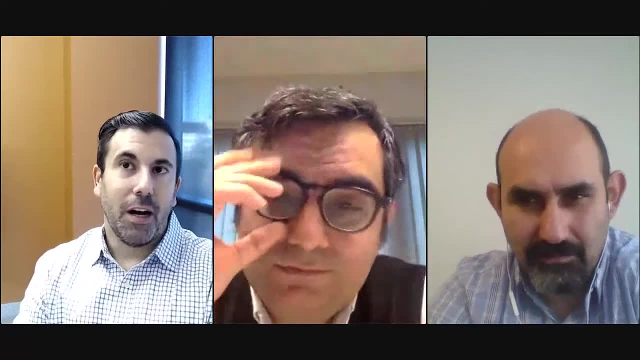 that acute of a process right which might open up more kind of manufacturing options And, again, like sterilization options, other things we might be able to do. But you know, I have always thought that the idea of in situ, like in the 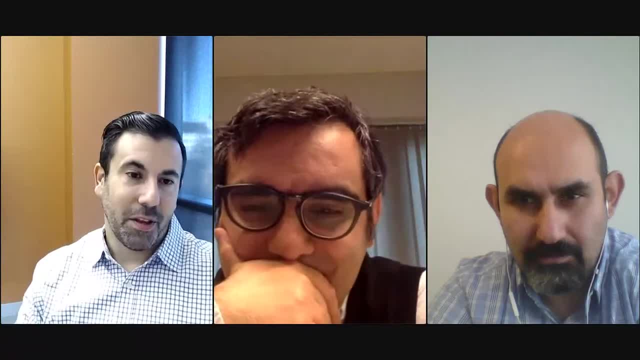 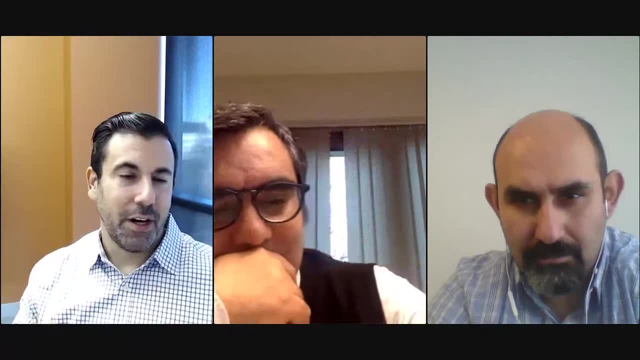 patient printing is pretty interesting. We're not working in that space, But I thought that that's really kind of an interesting idea as well. But you know, you know, I think you know, outside of a very acute, like immediate, you know, surgical need we have. 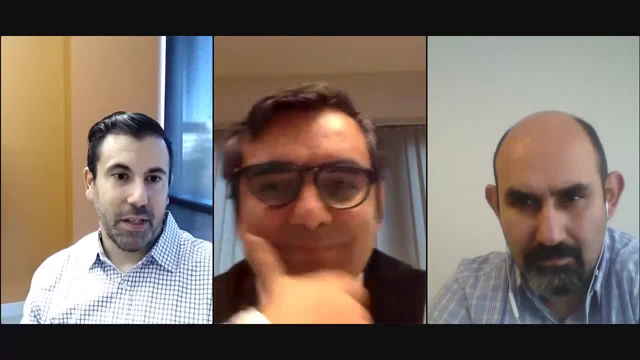 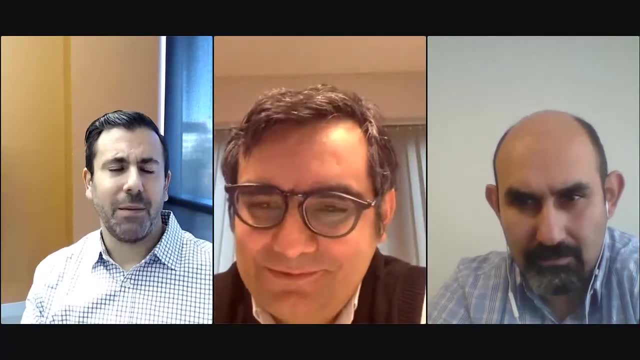 time. you know. you know one of the problems, as we all know, with 3d printing: sometimes is time. So right, if you're printing with cells, it's a huge issue. right, Because cells have a pretty limited viability window and suspension, which is 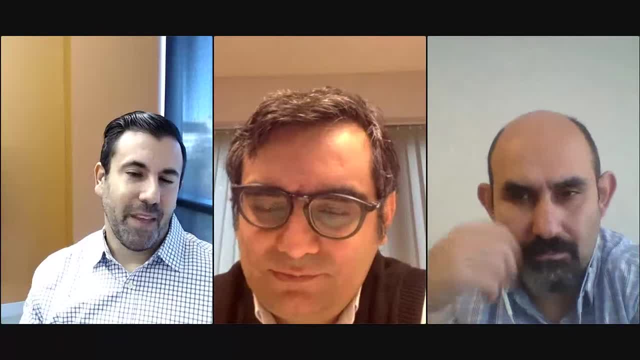 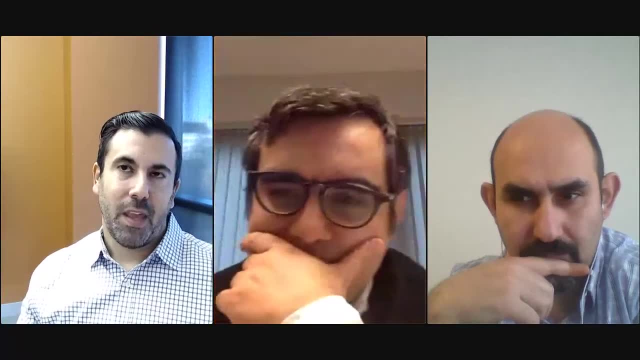 how we print them. It's a few hours, you know. you know two hours, four hours, maybe a little longer. there's some tricks we can do. varies by cell type. So how do you solve that? And we're looking at. 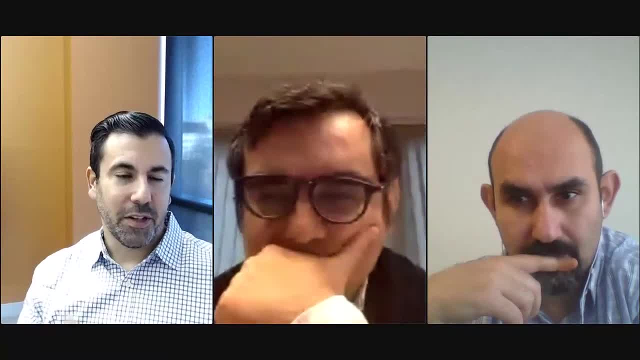 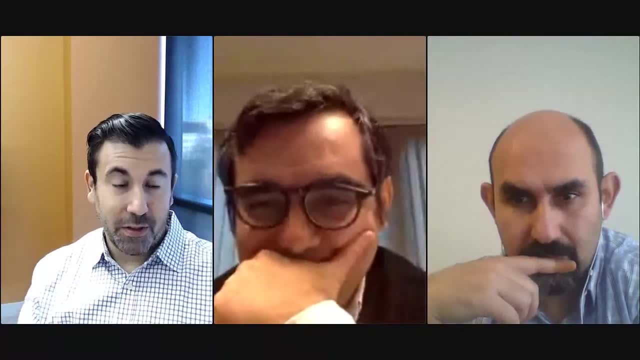 different ways of speeding up printing. you know that is an issue with size, but also obviously, with extrusion right. the finer the resolution, right, the more time it takes to fill up the same volume, so the longer the print, And so I know. 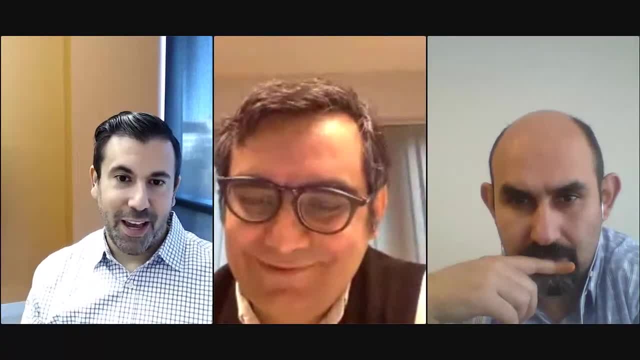 a lot of people are always excited about: oh, what's the best resolution you can get? Well, I'm like, I don't know. in our system we got down to 10 microns. That's great. I would never print a scaffold at 10 microns because I don't need. 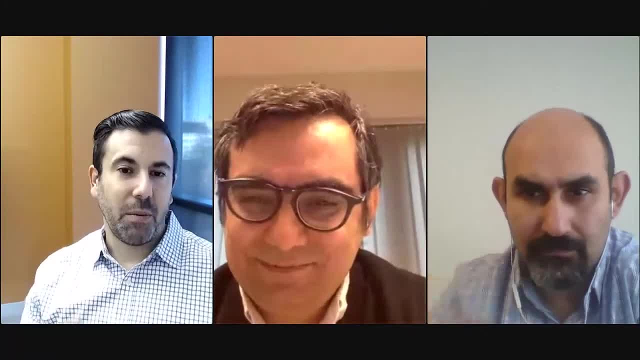 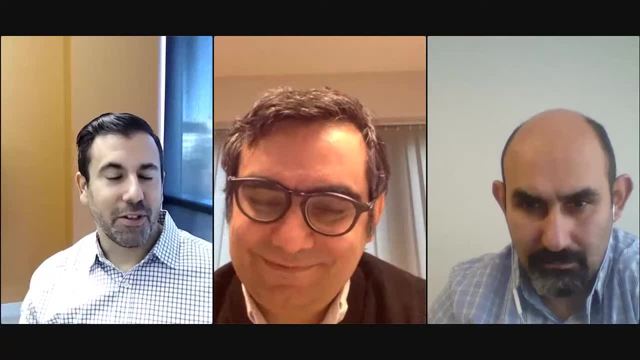 to. it takes too long And that resolution is probably not required for a lot of applications, Right? So I think you know there's all these parameters, that that that matter, But you know, for example, we're, we're. 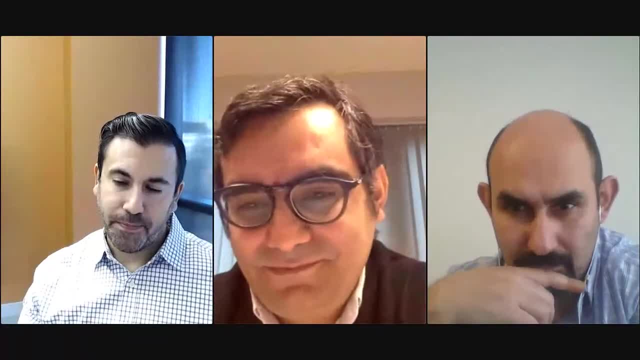 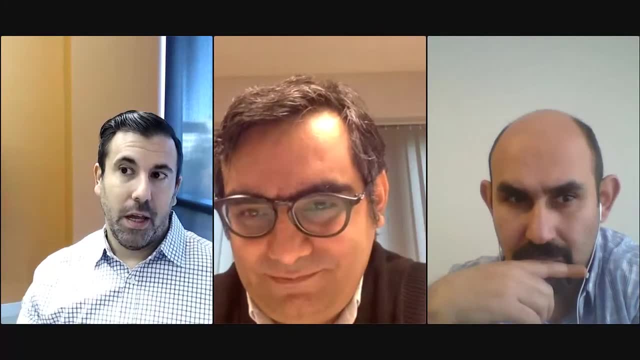 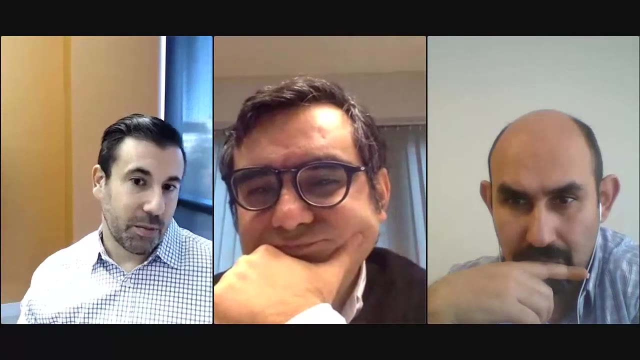 printing scaffolds right now for volumetric muscle loss. that are the habit on the order of 10 to 20 milliliters of bio ink, so pretty big Right. so about 10 to 20 cubic centimeters of volume, And you know they take about eight hours of print. the 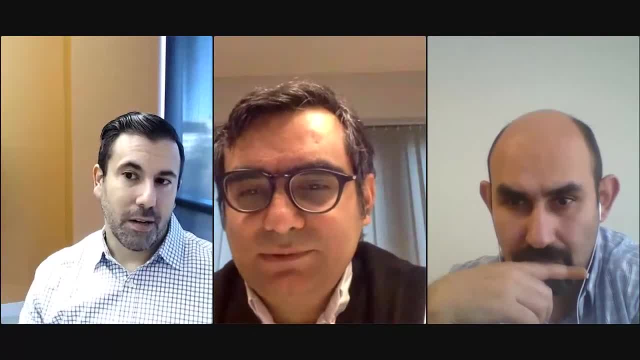 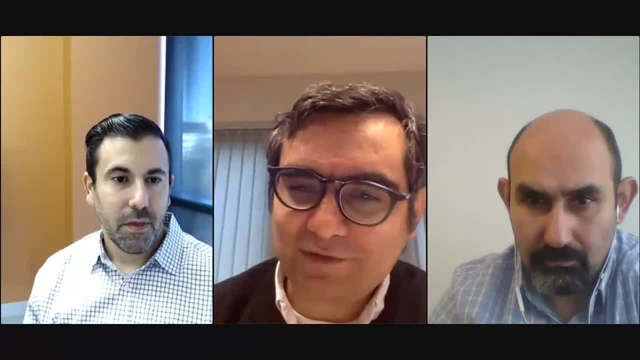 lot of things that we need to do, And so you know there's a lot of things that we need to do, And so you know there's a I see. So how long did it take to print those hardvowels? 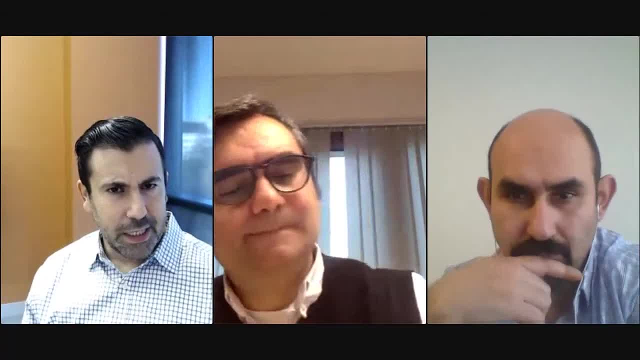 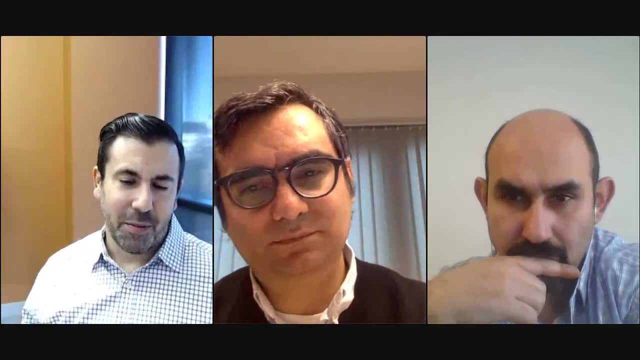 The hardvowels, I believe, were a couple hours. Uh, hmm, Not, not that long. Again, It's a little bit of a resolution game. Um, you know the, the collagen I always tell people and this shot does more. 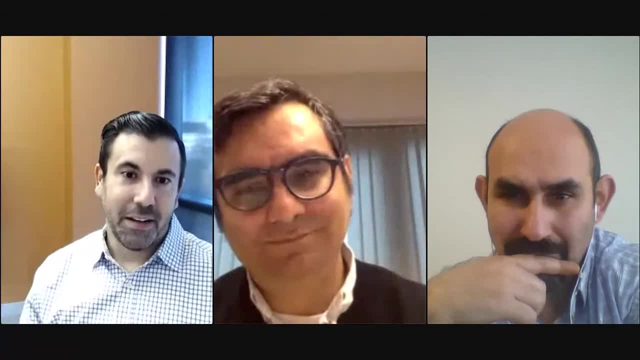 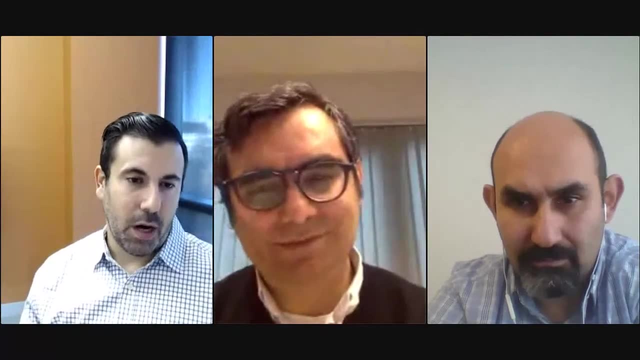 than anyone else. that collagen is actually the easiest thing we have. now the print like it works so well Using this pH neutralization in this approach. We get better quality resolution, So it kind of works best when we use it like this. Yeah, we get better quality resolution like this. 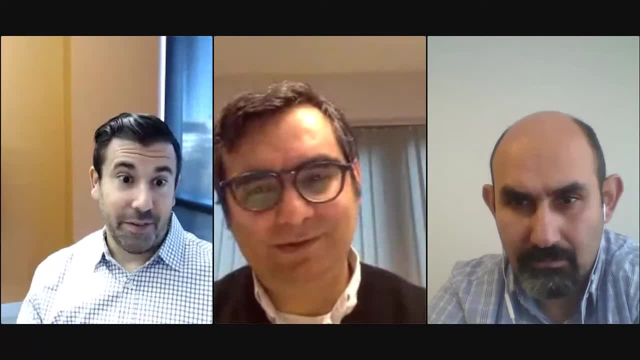 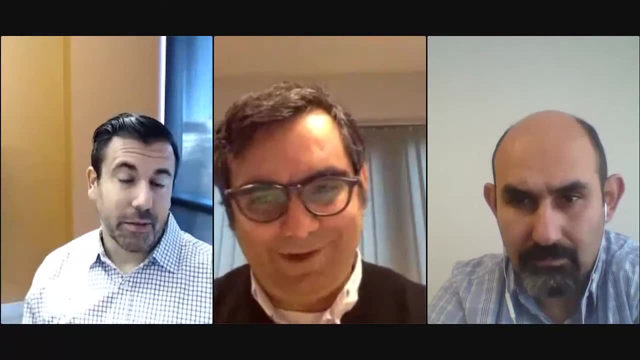 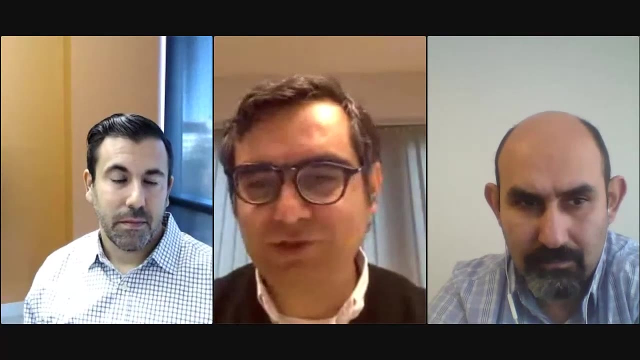 fidelity out of the college in printing, then we actually do out of anything else, yeah, and and that, and so you know we're really excited by because hopefully that helps a lot of people. yeah, yeah, okay, okay, that's good, that's promising, I mean in terms of time, because time has, as you mentioned, I mean it's always especially. 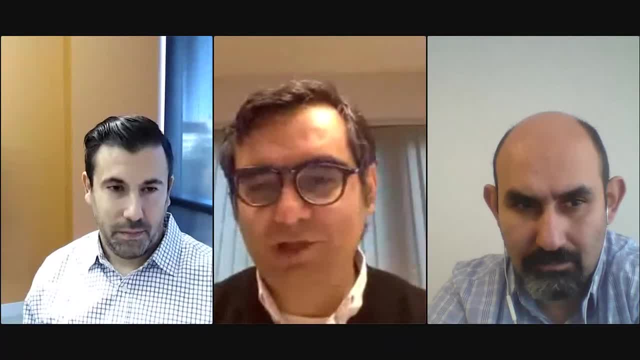 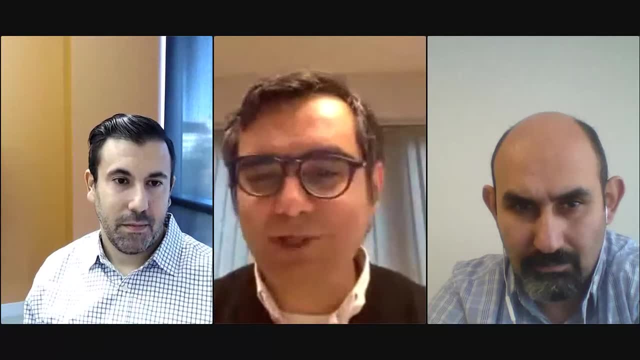 when it gets bigger, the the construct gets larger than it takes. it takes a few hours to print and but I'm sure that there are, they will be. I mean, many smart people are working on the in the field of 3d bioprinting. I'm sure you. 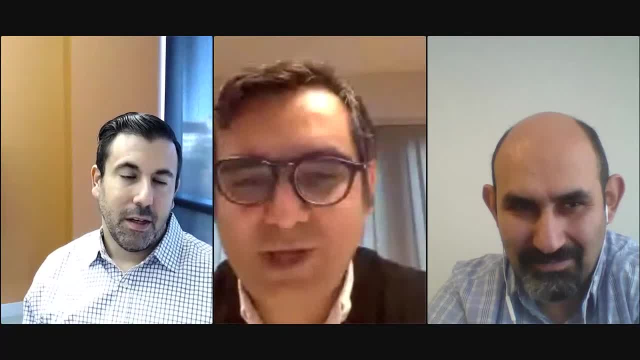 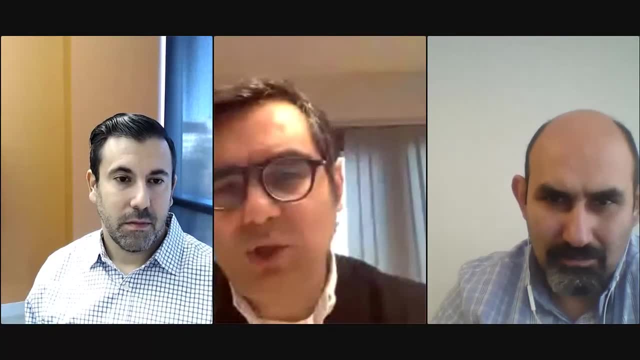 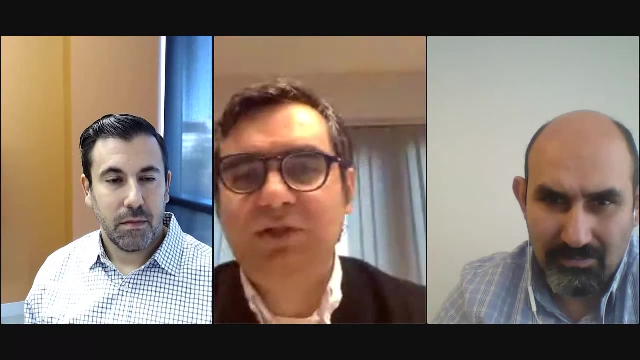 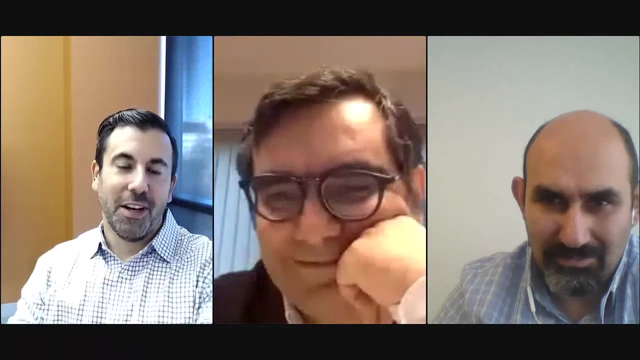 will find basically a solution to that problem. so the other question is asked by Marinus. probably we already covered part of it, but the question is about the main challenges of using fresh method in 3d bioprinting of soft materials, the main challenges. I mean, it was right we developed the solve challenges, but you 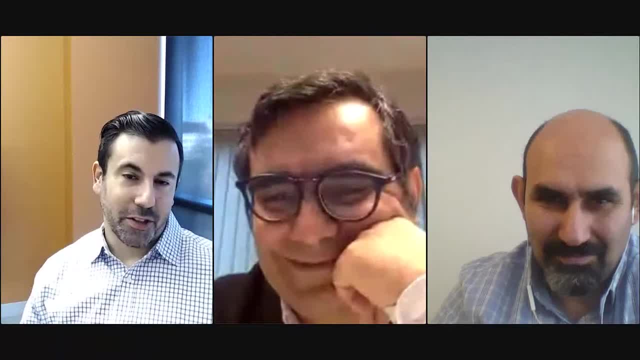 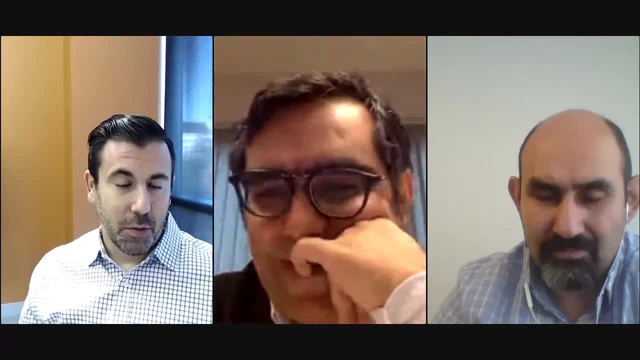 know, like any technique, it has its pluses and minuses, right, I mean, that's just technology, right? so you know it's it's temperature sensitive, right? so you print at room temperature, you raise it, the body temperature to melt the support. now, we did it, we did that. intentionally because it's an extremely gentle release right, and so we found that if things- there's a lot of different support bass that have now been been developed out there, they all have their own advantages, but we haven't seen anything that's as gentle of a release and maximizes kind of viability. 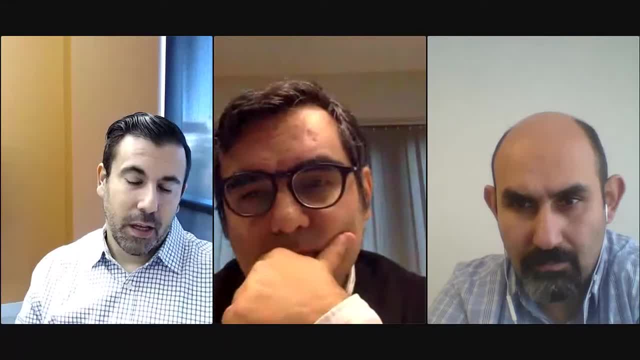 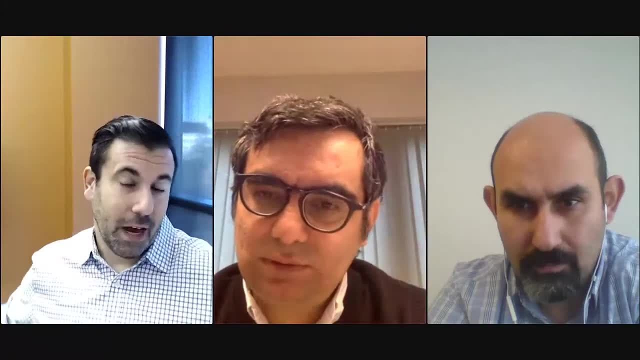 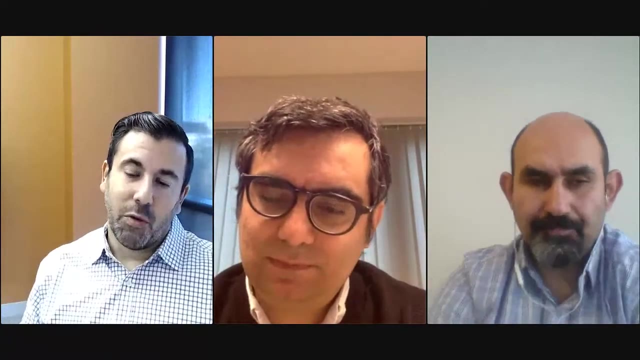 instructional integrity. like, like the gelatin does so. but you know, if you need that's that structure, that support material, to be around longer, you know, obviously you go in the incubator, you melt it, so it's not there for that purpose. you know we've also had some issues producing the support bath over. 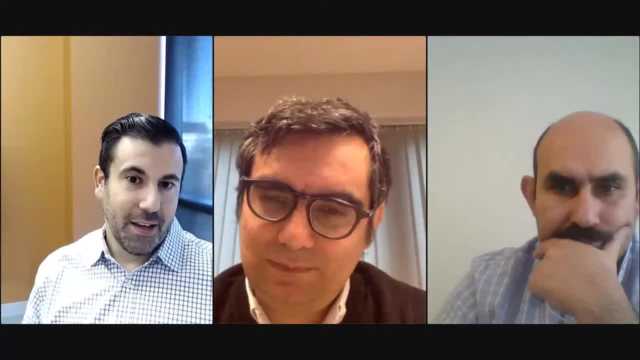 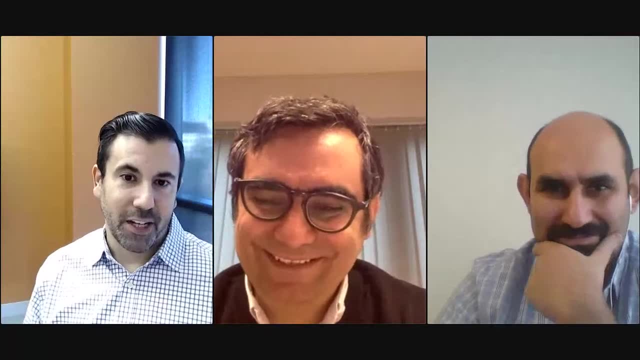 time, because it turns out that the gelatin that you buy is so incredibly, incredibly variable- lot, a lot like it's the worst thing out there from almost any bioreagent we've used- and so We really had to get really deep in the weeds on a specification for the gelatin. 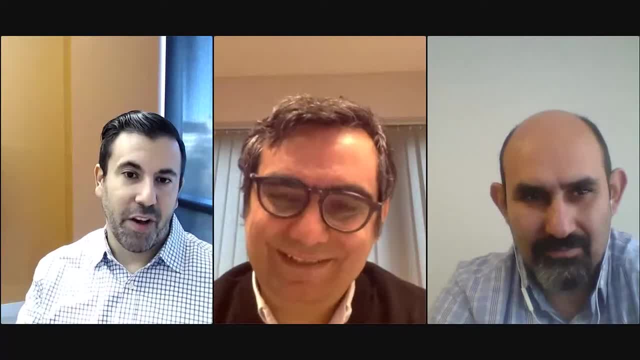 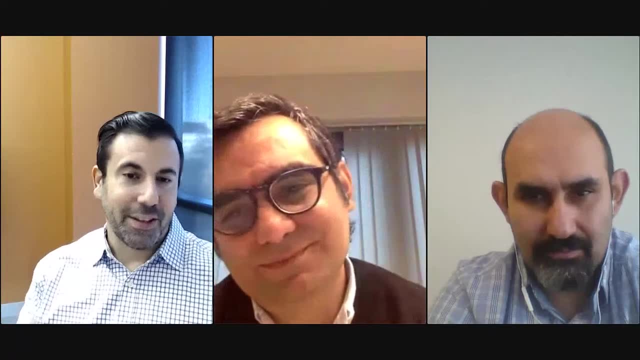 Yeah, you know, far below what you would ever see on a normal manufacturers label. Yeah, to be able to effectively get good support material. You know, that's actually one That's that's like, that's the kind of thing They're like: the company solves, right, the company solves that. so no one, if you want to buy it. 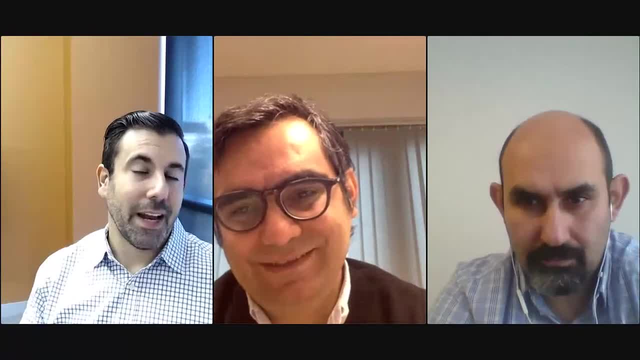 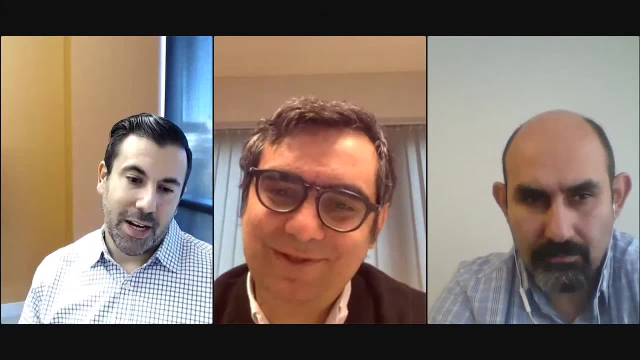 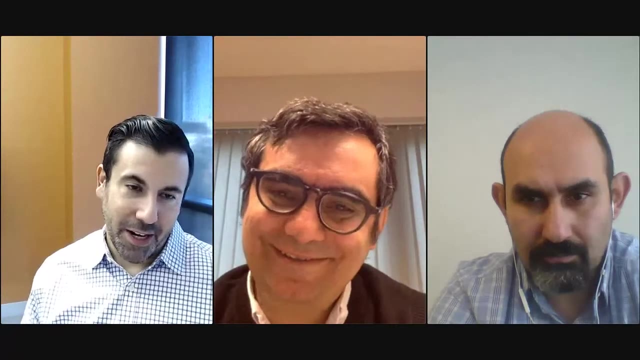 You never have to worry about that again. But it that has been a challenge that we've largely addressed at that point. But that's always been difficult and I think that probably holds for other support baths That better out there. But you know, you know we're mostly leveraging the advantages of it. right now There's not too many. 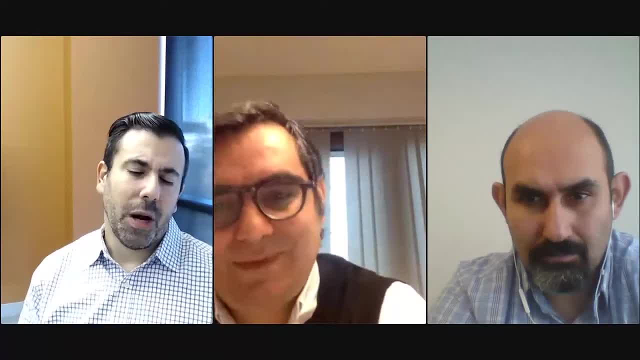 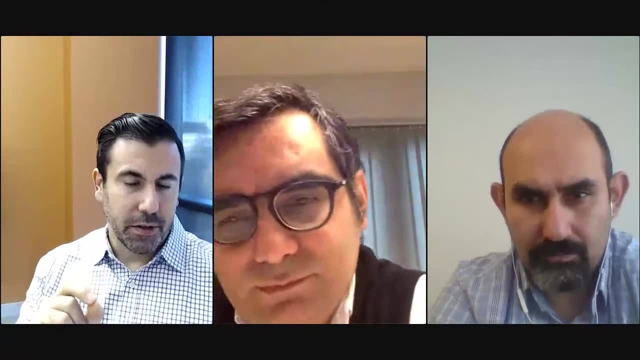 Too many disadvantages beyond kind of the obvious. what you see. Oh, I would say another one is that you know we're the. the support bath is made of micro particles. Yeah, So those micro particles can actually, if you look in our science paper- I didn't. 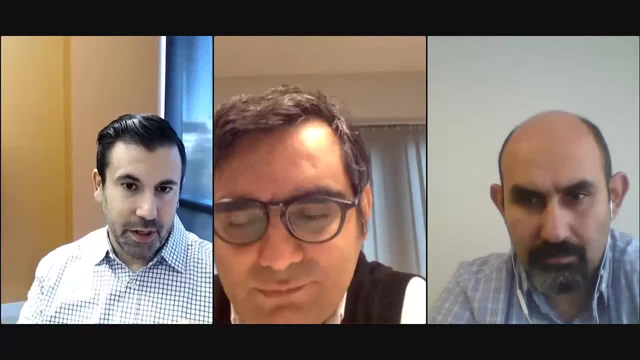 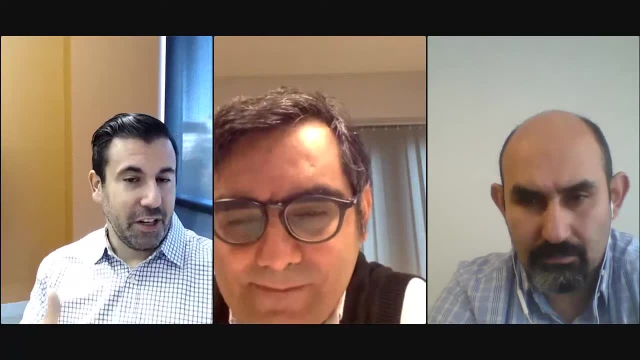 Show any images of it in the talk, but you can see little dimples on our filaments, Yeah, where those micro particles were. so that might be an issue for some printing. Like I said, we actually turned that into an advantage because we for our micro vascular ization work. 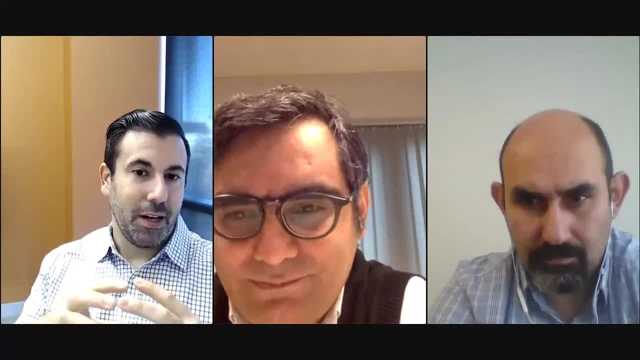 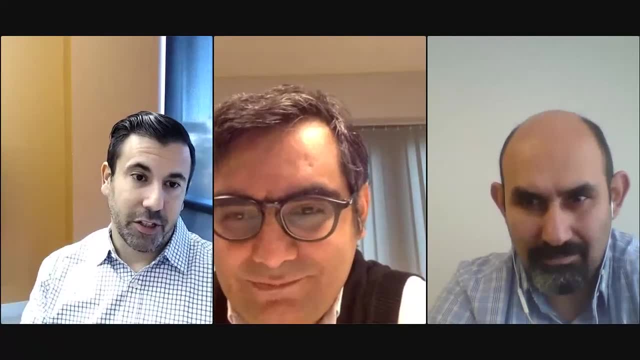 We actually incorporate those micro particles and purpose Into the prints, and so when we dissolve the gelatin support bath, we have these little micro pores And it's actually turns out to be great for cell infiltration. But I think that's, like most things, right. it can be a feature or a bug, depending on how. 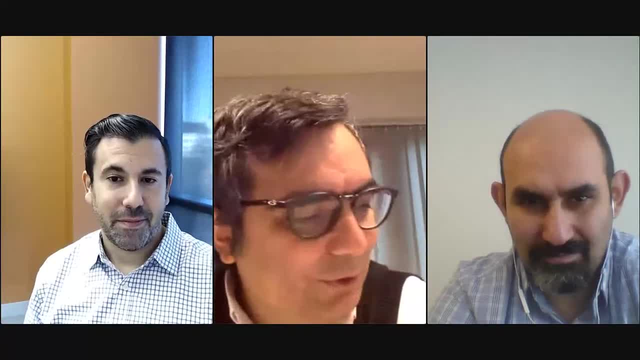 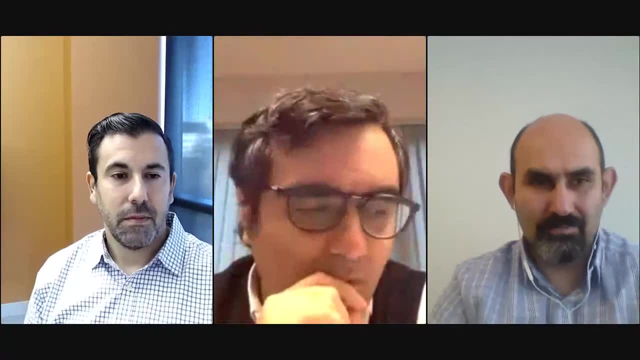 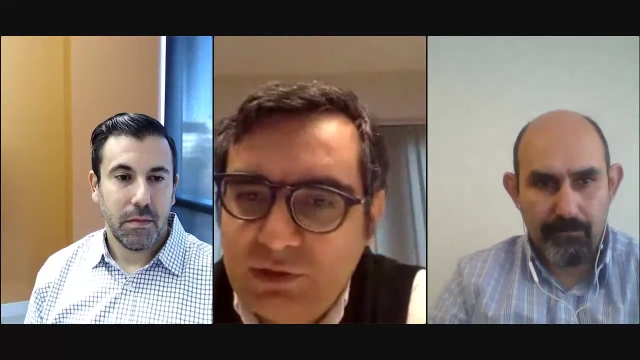 You how you look at it. So yeah, yeah, cool. So I just have one more question about the challenges. So do, have you faced any issues with the Premature Across, thinking of the ink at the tip of the needle Using this method, or you, you, you don't. you didn't see that as an as an issue. Yeah, the only time we see that. 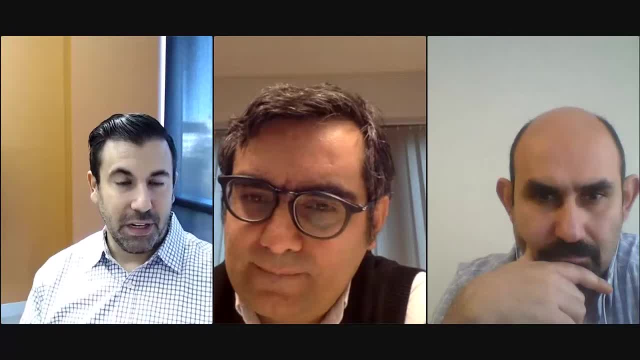 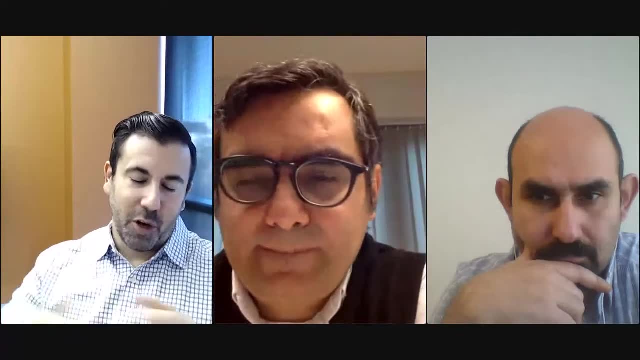 is When we are doing multi material and we switch nozzles and we stop extruding out of a nozzle right and so what? and so we- We we show pictures of it in some of our papers- but that we've basically developed a system when, when we're done printing, we put it into a 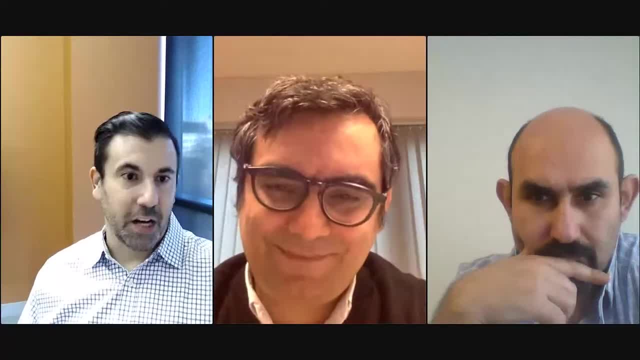 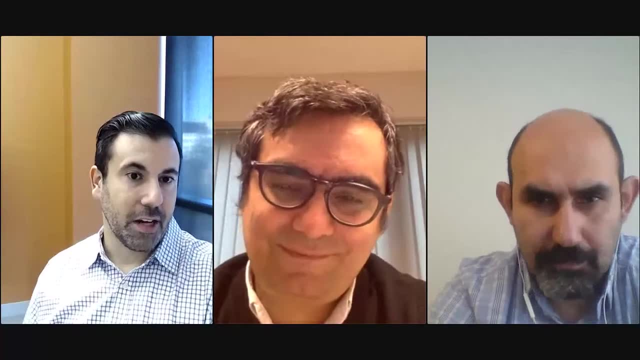 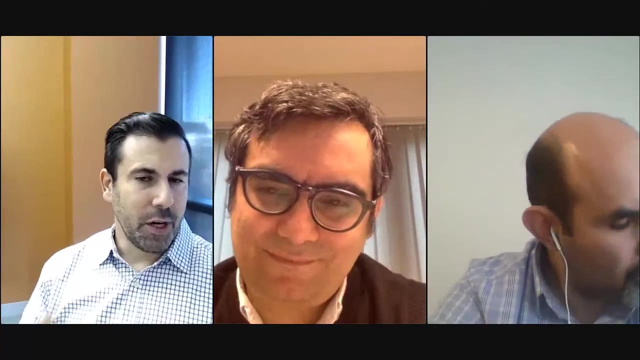 DI water bath. the other need: the needle that's not printing is hanging out in the DI water bath and That basically dilutes enough of the cross linker that when we go back to start printing again it hasn't clogged up. but you know, There's one thing that we do with our printing typically and we don't use a pneumatic. 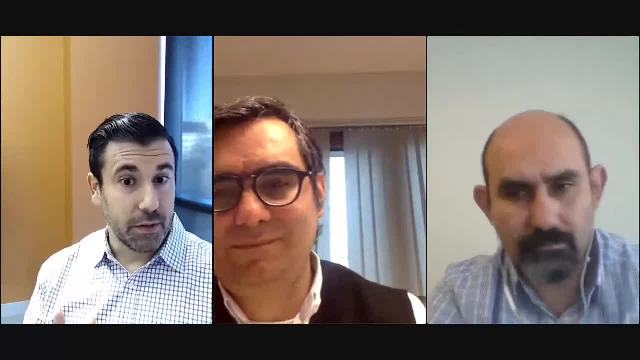 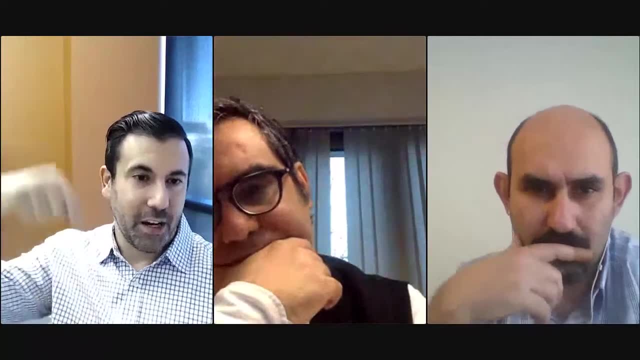 Extruder. we use a direct lead, screw driven, plunger driven, Syringe based extruder, and so it's constantly retracting and so you have a lot of mechanical movement back and forth. I think that probably helps prevent a gel clog as well. So, yeah, Yeah, I agree. 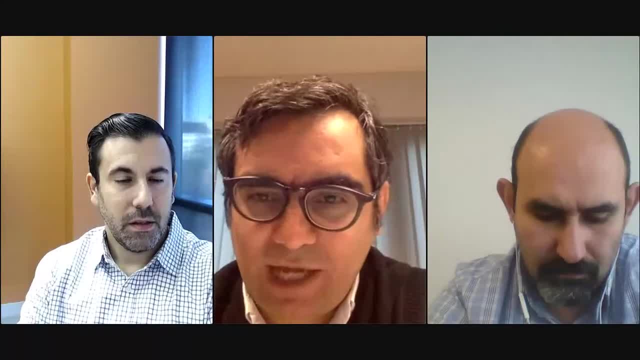 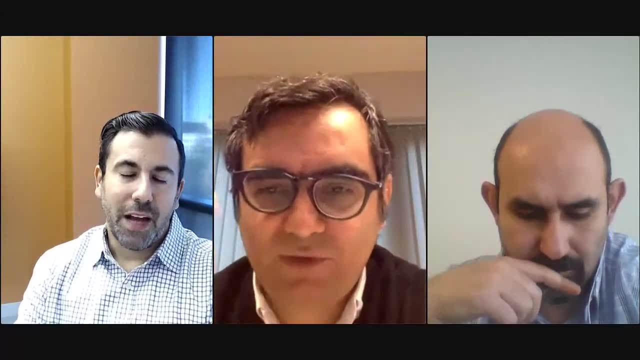 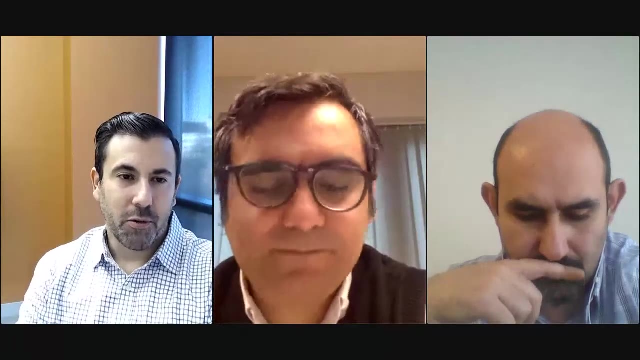 Because there was a little bit worried about alginate. They were the alginate ones that you print, because alginate will be in contact with calcium chloride and then there might be some diffusion from the calcium. but but We've like never clogged a nozzle. I mean, we definitely on occasion have clogged the nozzle, but it's actually quite, quite rare. 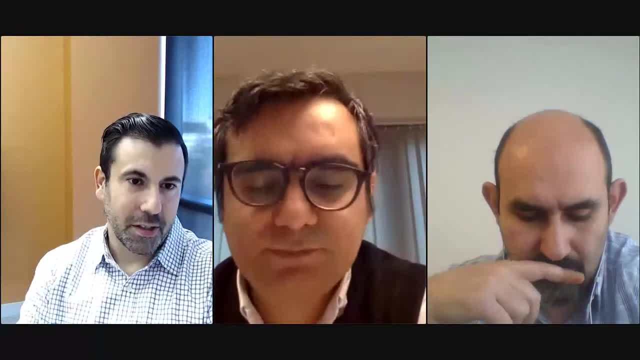 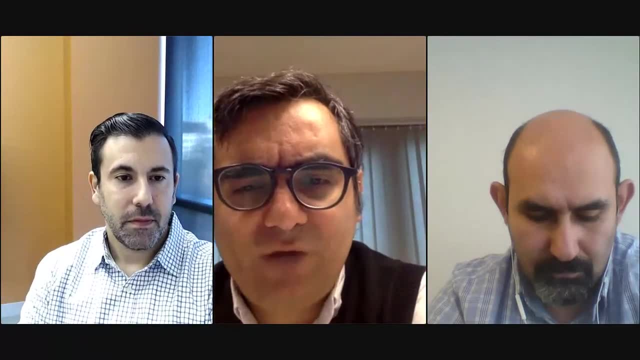 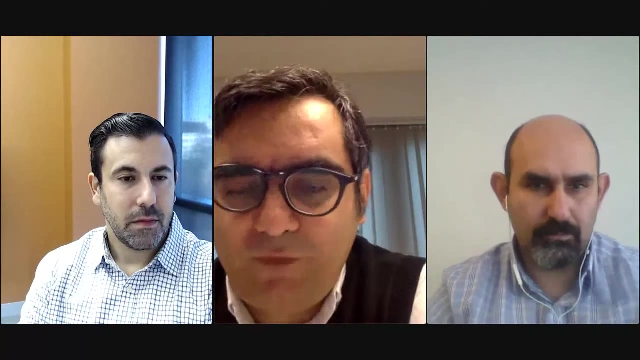 And if we're printing at a high enough speed as well. that tends to this all that. so, yeah, brilliant. so the other question is from From this again, I mean, I don't know if I pronounced his or her name correctly, So how did you synchronize this? spontaneous contractions of myo 2?? 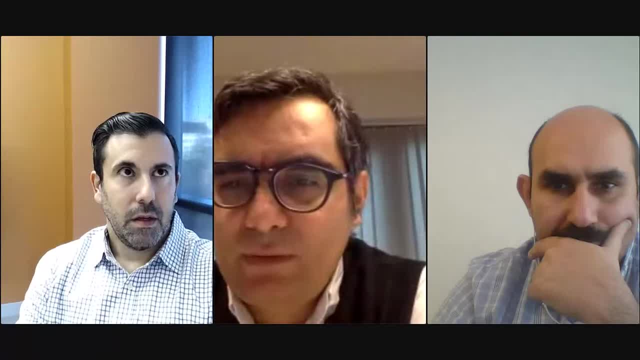 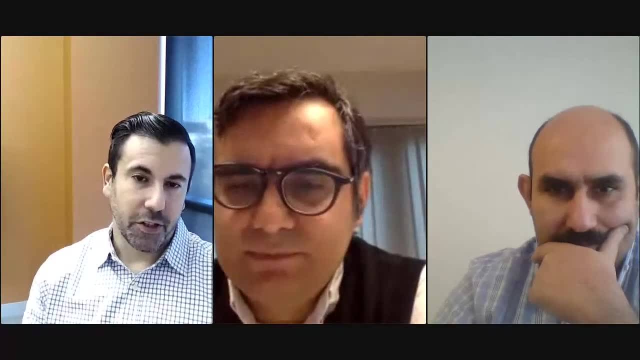 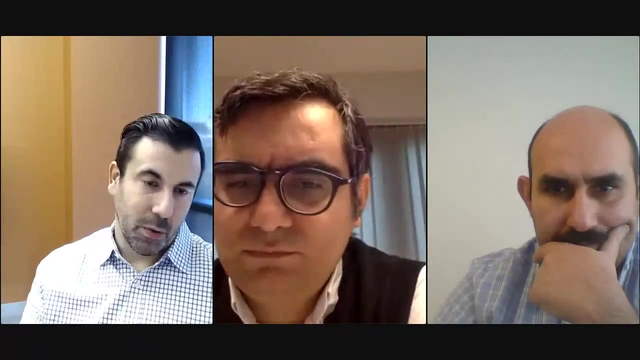 sites in the heart valves. so the myocytes were the ventricle, but i'll talk about the ventricle that was the cellularized one. but um, that's uh just field stimulation. so outside of the view of that video, there are two platinum wires in the solution and we basically send a square uh wave. 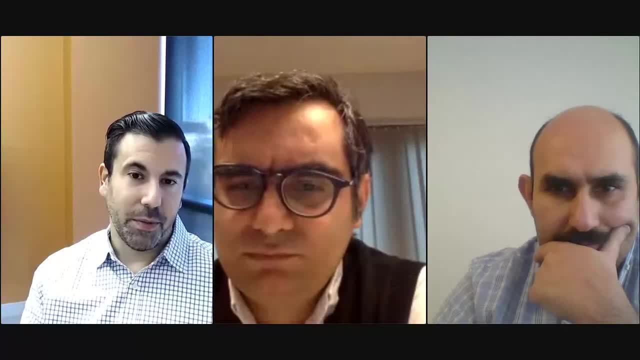 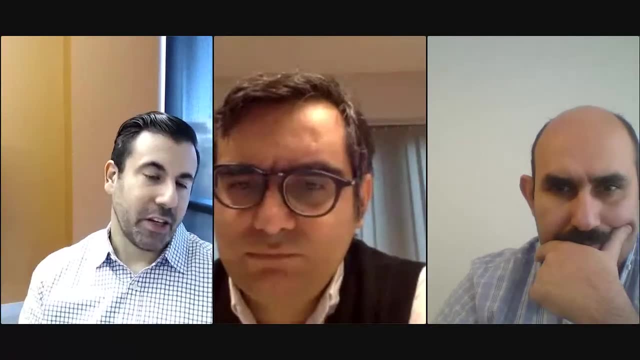 of voltage across them. it's kind of like when you get, when you've seen someone uh ever like defibrillate the heart, where you send a large shock to kind of synchronize the heart to contract at once. that's essentially what we're doing, so it's a it's a pretty common approach to get. 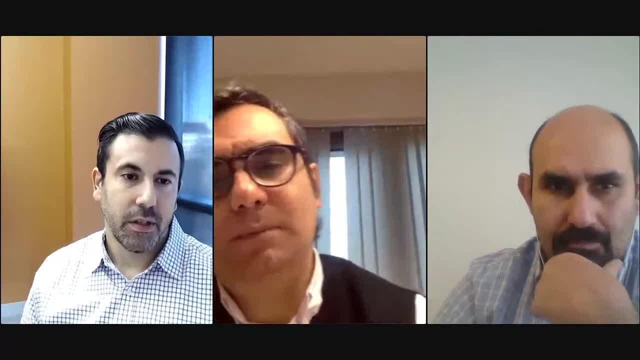 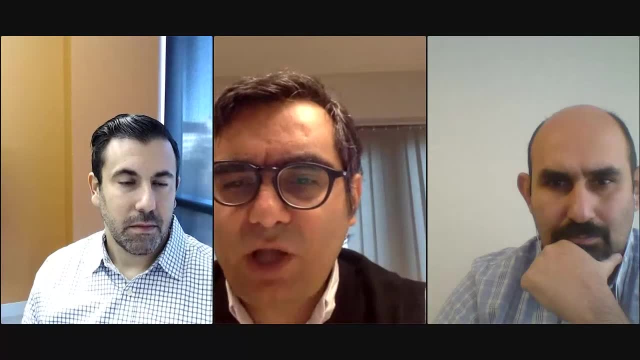 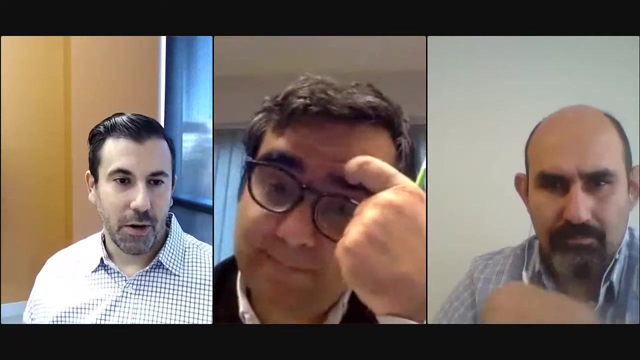 synchronized contraction and engineer cardiac tissue. the other question is from mark freer. so can you comment on the maturation state of your bioprinted ventricles? meaning, does it show positive force frequency? uh, well, so for that tissue we we didn't measure force, so i have no. 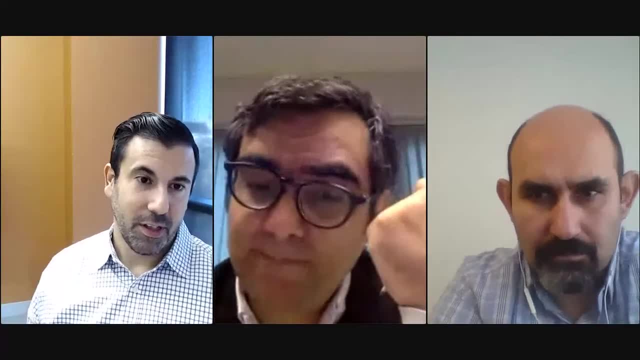 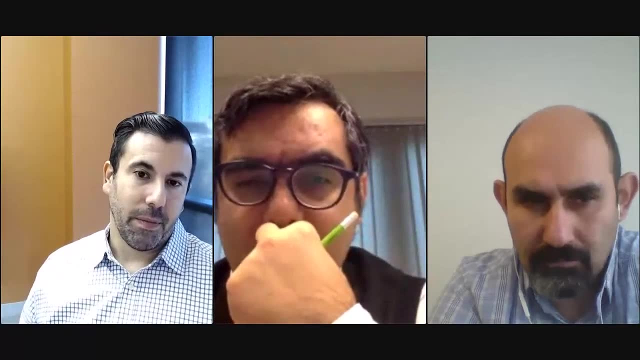 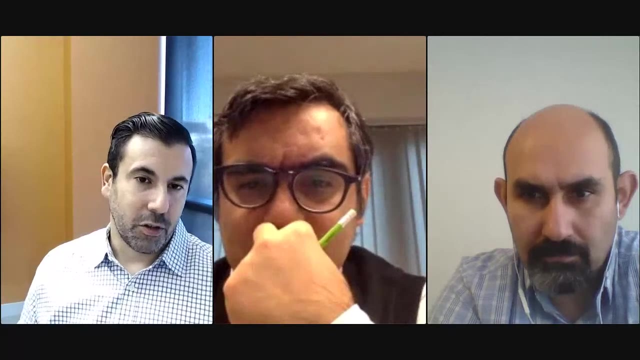 answer? my guess is that they're. they're relatively immature. um, uh, we've got another paper that's actually up on bio archive right now. um, that's not bioprinting, but it's actually. we developed a little engineered tissue construct where we actually look at loading and using tunable mechanical loading to try to. 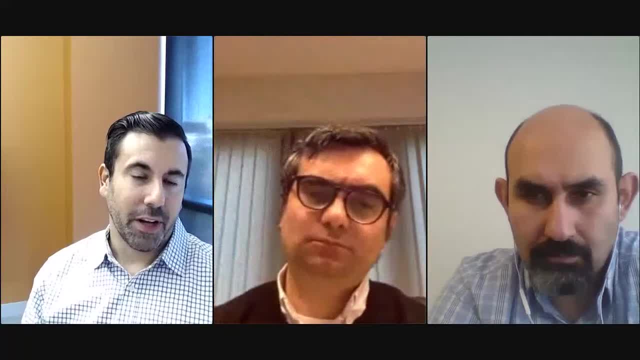 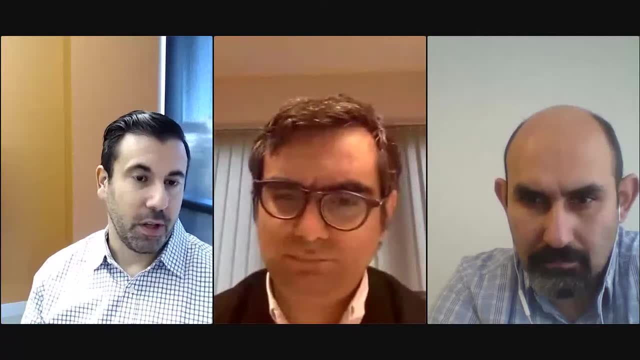 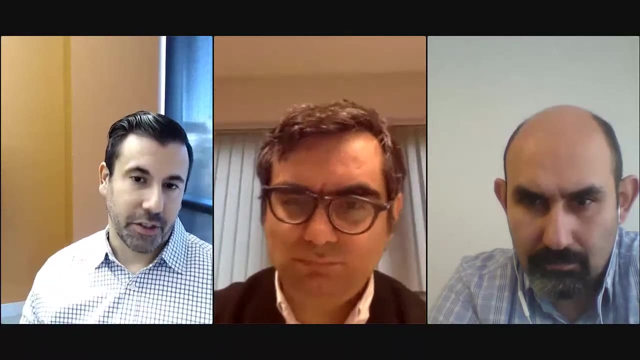 drive some functional maturation where we can look at force frequency relationships. so i know that loading is important and this construct we created because this is open ellipsoid: we're not controlling loading. the next generation of this system that you'll see from us is a closed chamber system. 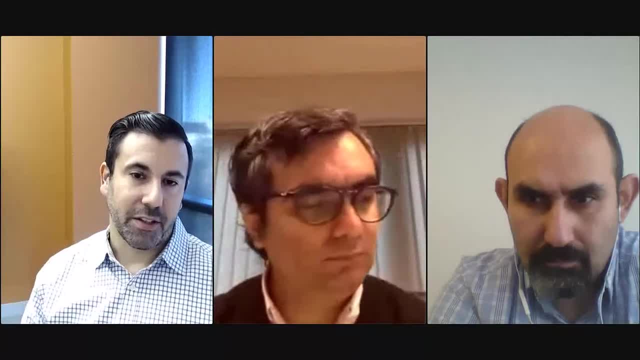 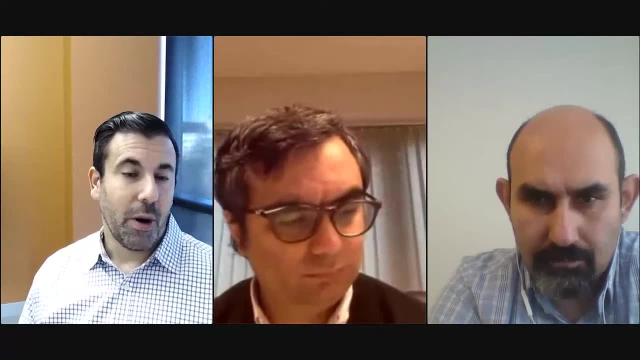 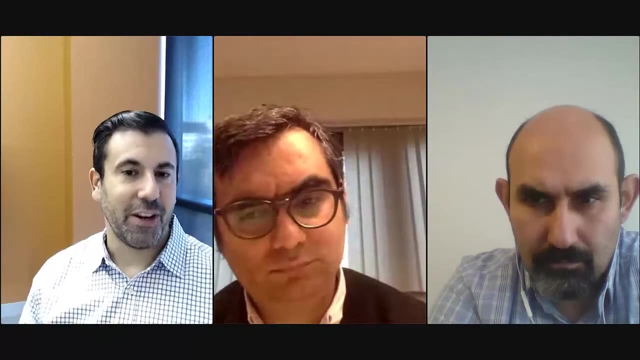 right with valves so that we can actually pressurize the system and actually, you know, put in a pressure uh catheter transducer and do some of that work. so i don't know the answer. my guess is that these are immature. um, it was really hard just to make that ventricle like to figure. 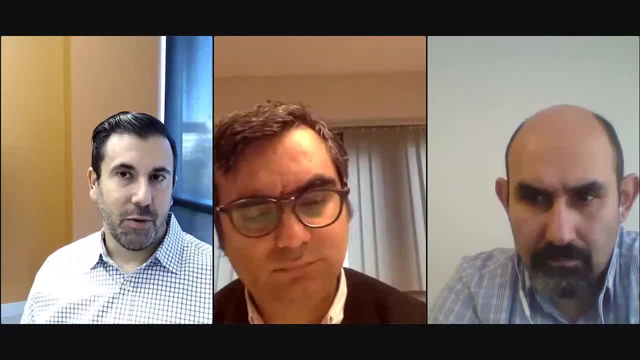 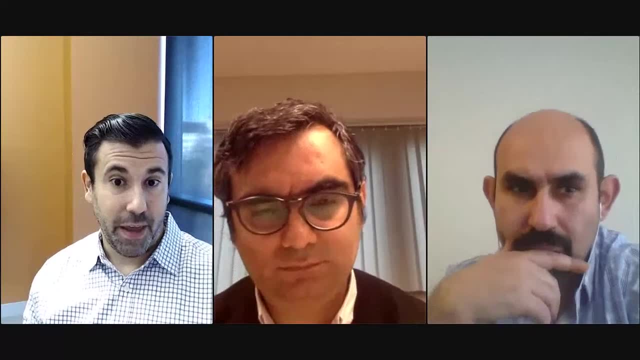 out how to do it. um you, you may notice that we obviously we printed the collagen and the cardio separately. we went through a lot of different design iterations before we hit upon that. we realized, you know, for a long time we were printing cell-laden hydrogels because, honestly, 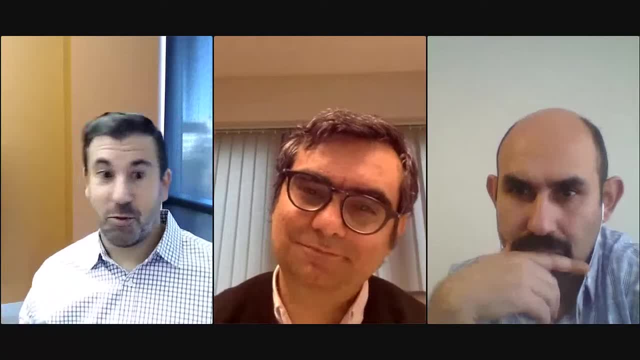 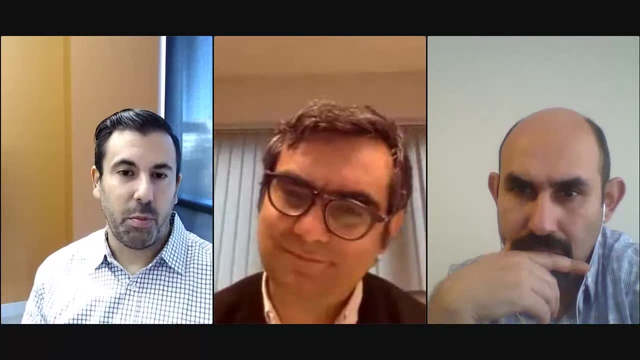 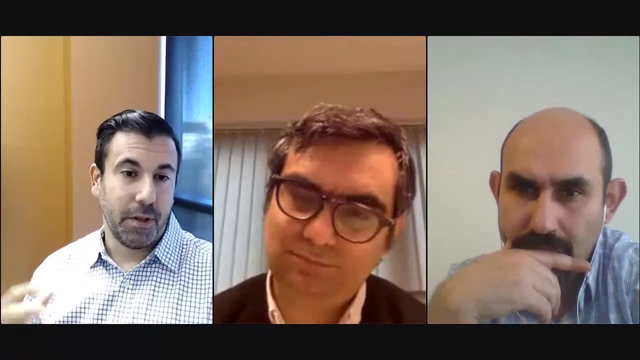 everyone in the field prints cell-laden hydrogels. that's just what you do. we realized the density of cells was so low and the quality of tissue we're getting out was so poor. like we need way, way, way more cells. yeah, how do you do that? you either print higher density or you need your your cell-laden. 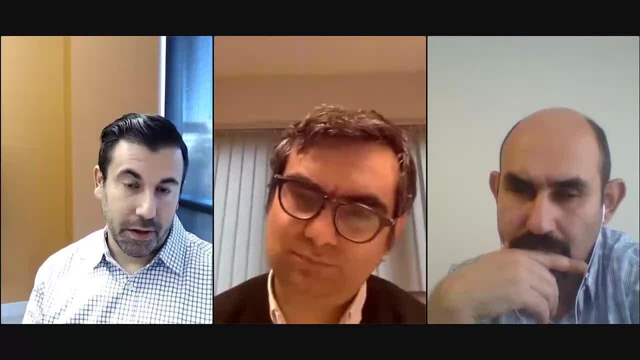 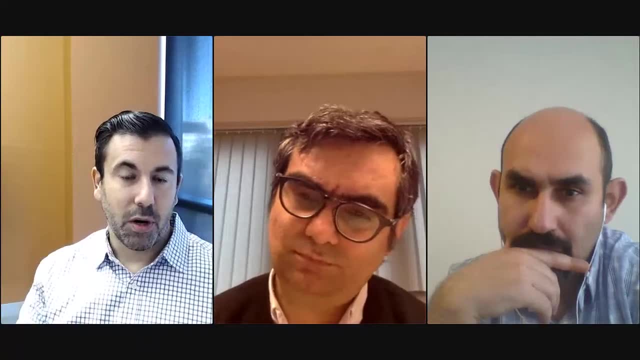 hydrogel to compact, to densify. it's got to be one or the other. we went with the high density bioink by doing that and kind of using the collagen as a separate ink to create more of just like a supportive shell. that's how we got to a tissue that at least could contract the right way. 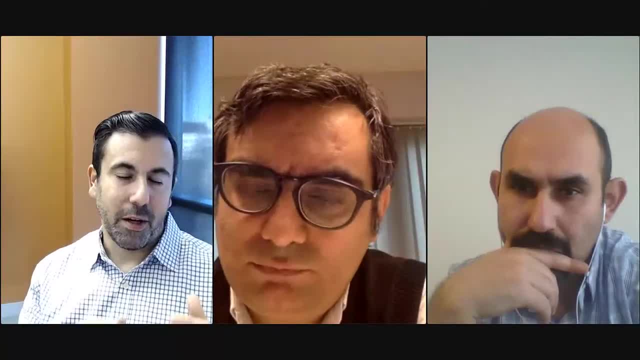 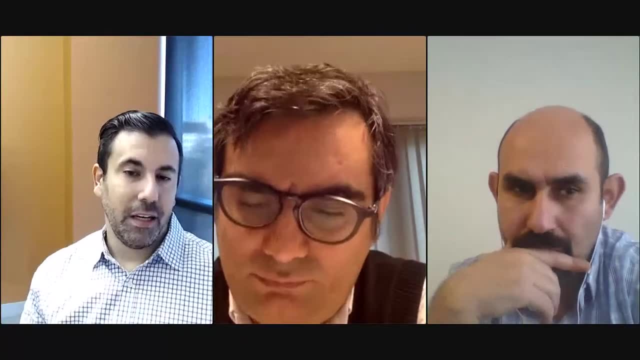 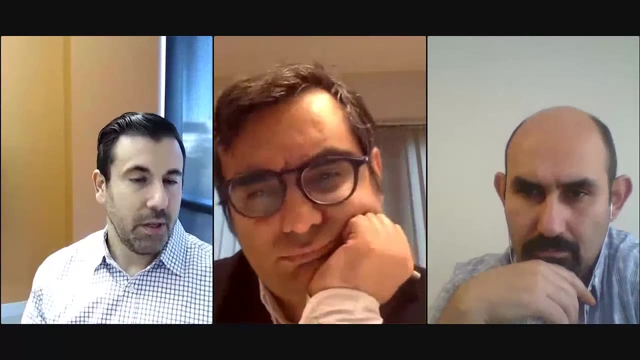 you know. but again, as many people know, you know it's, you know es or ips derived human cardiomyocytes tend to be quite immature. my guess is that these are quite immature, you know, the conduction velocities we were getting were only about one centimeter a second. two centimeters a second, that's. that's quite slow. so again, a lot of room. 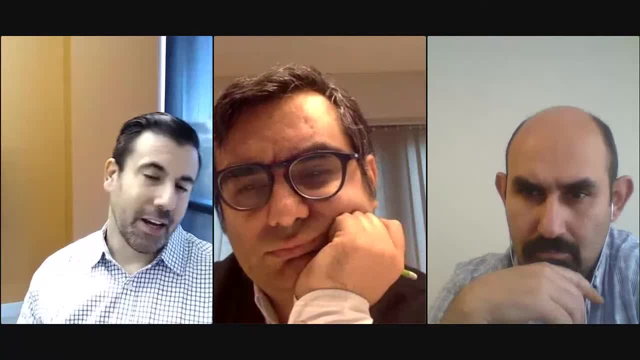 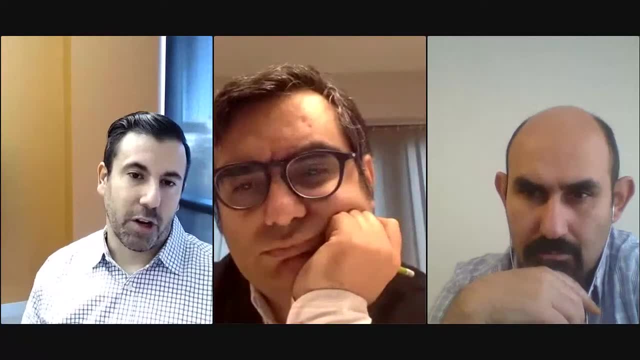 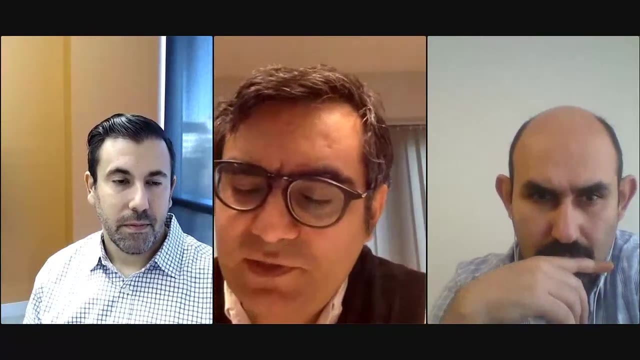 for improvement we're actually really excited to to try again, or the devices we're building next to, to do some of this, this mechanical loading, uh, to try to drive some of that structural and functional maturation. that's it. that's it, great, great. and then, uh, speaking of high density cell, 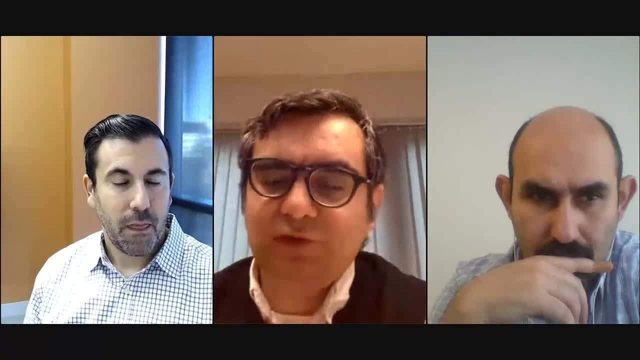 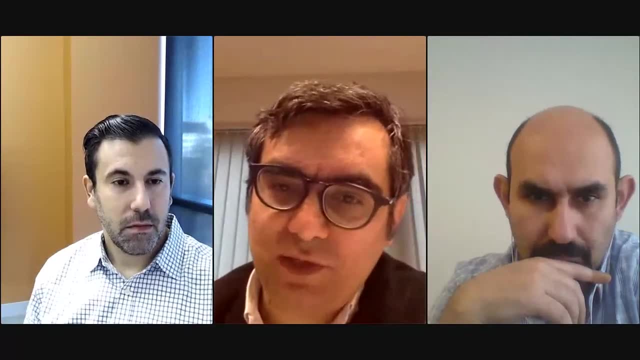 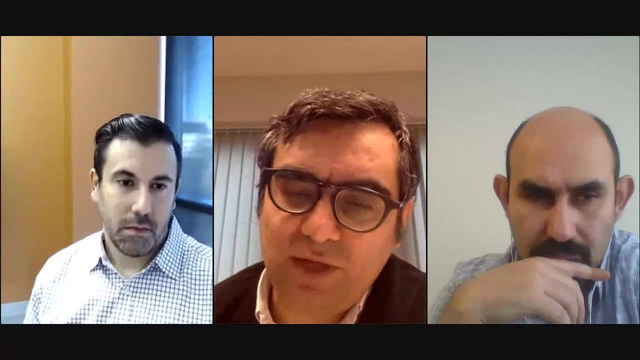 printing. have you? i mean, i mean you have the results, but before that, have you faced, uh, any issues with the shear stresses being applied to these cells during the printing process? and how do you, how did you fix the issue? if you had any problem with that? yeah, i mean our problems. 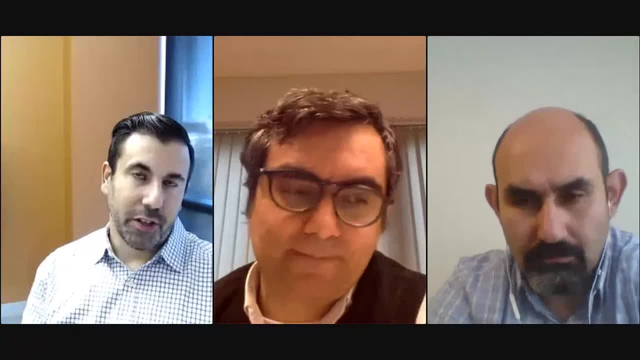 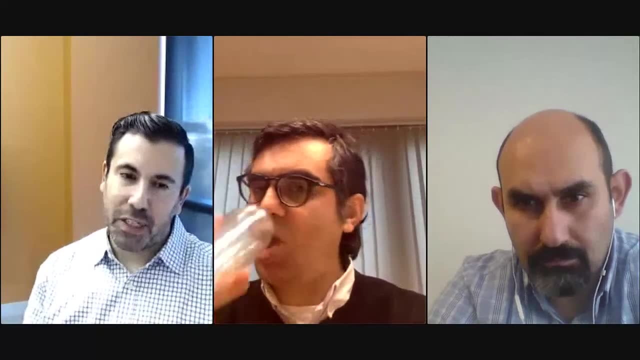 were primarily around. well, there's a couple different problems, you know. one is just um, you know, if not the nozzles too small. obviously, the smaller the nozzle, the higher shear stress. i believe we were using nothing smaller than 150 micron diameter nozzle right, or we have a essentially 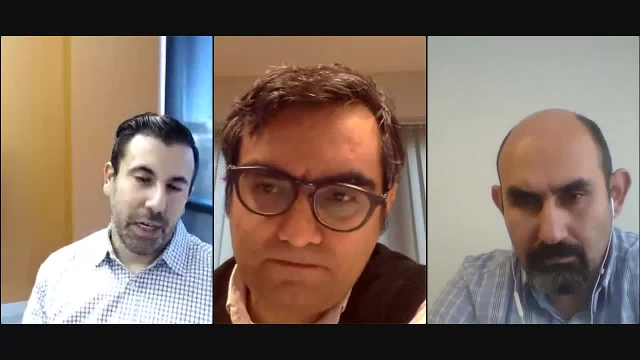 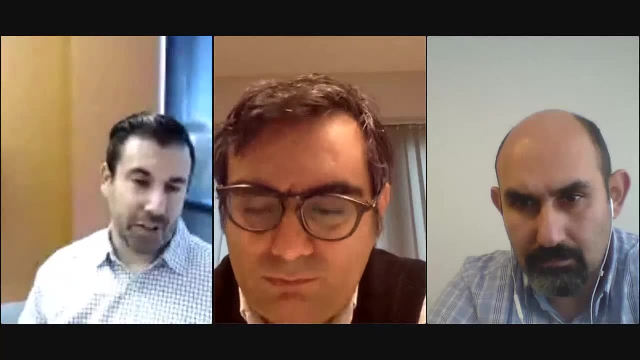 a resolution limit with the cell printing um. also, you need to make sure that when you have a high density cell bio ink, like we're using, it's really a cell slurry. it's basically, if you've ever pasted cells and made a cell pellet, you basically have a cell pellet with just a little bit of a very little. 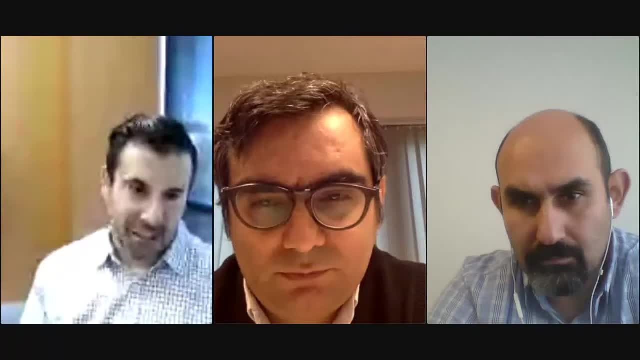 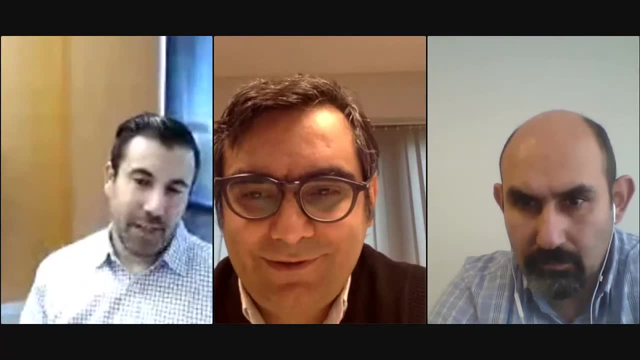 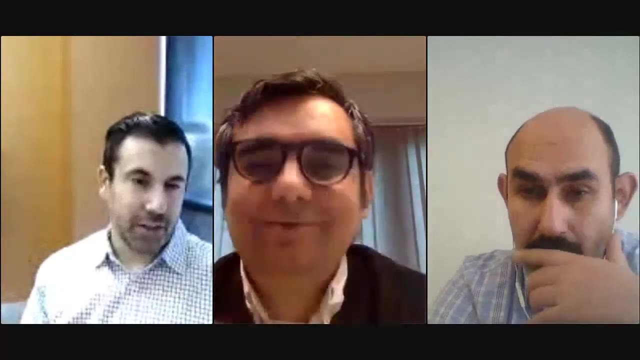 bit of extra liquid. yeah, the cells cannot stick. if they stick, then they become bigger and the shear goes up. so, uh, we actually have a paper we're working on um where we're using both uh temperature inks to slow down the cell, cell interactions, to both uh improve that and also prolong the working. 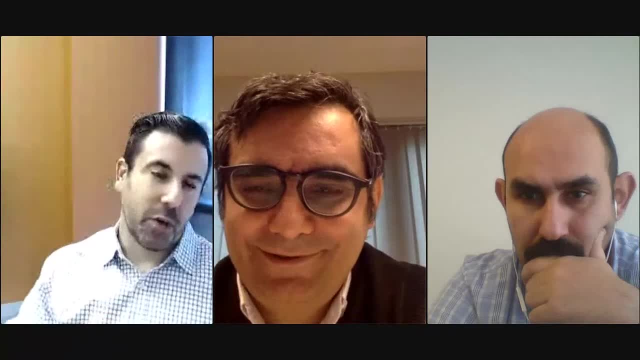 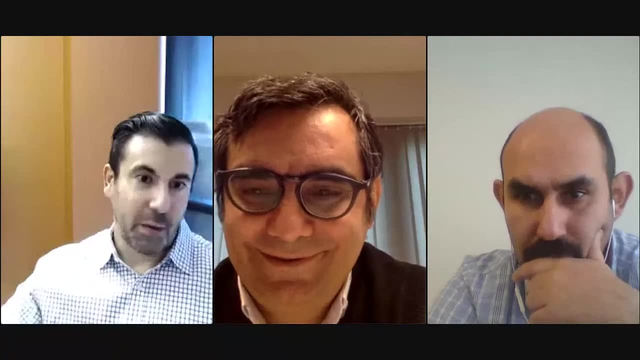 window, uh, of the cell link. so you know, instead of two hours can we stretch it out to four hours? it's still not game changing. uh, you know, if we go from like two hours to a day, that would be game changing. but we can at least go. we can kind of double the working time, but it also decreases. 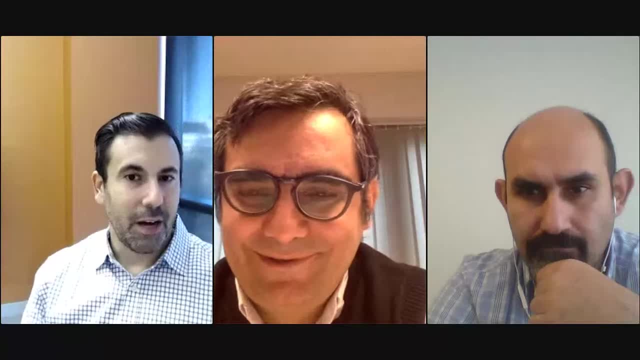 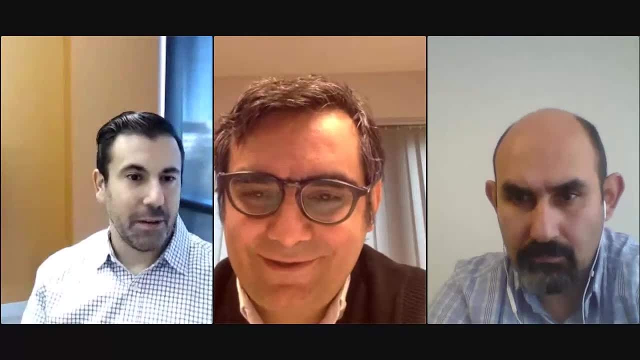 the shear stress, and so you know, uh, but you know, obviously it's like it's obvious, things like interfering with cat adherence, interfering with integrins, the way that the cells stick to each other. if you can slow that down, you know, not in the way that damages the cell, but just enough transiently, you can get some advantages. so there's, there's. 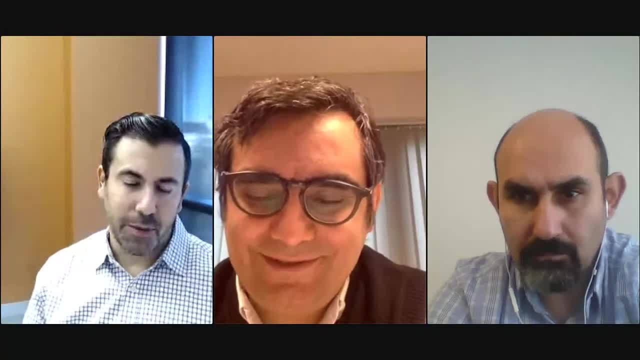 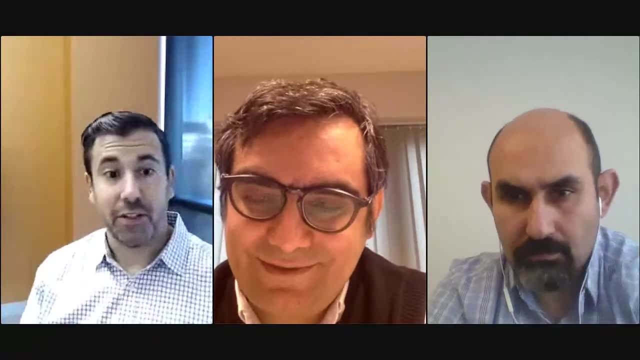 multiple issues. but yeah, shear stress is a killer. you know there's other groups that have developed bio inks that are meant to actually just better shear, or sorry, shield the cells from the shear stress as well, and so you know that's interesting, uh, as well, i think. i think there's still a lot of. 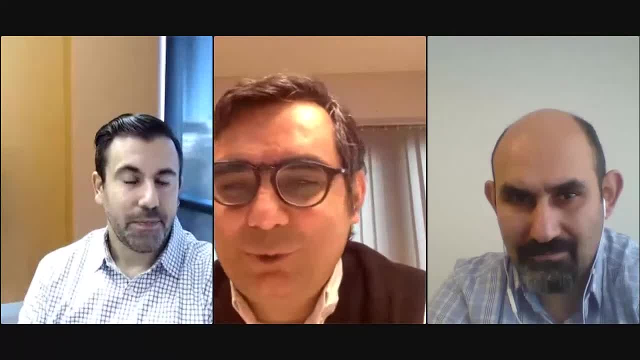 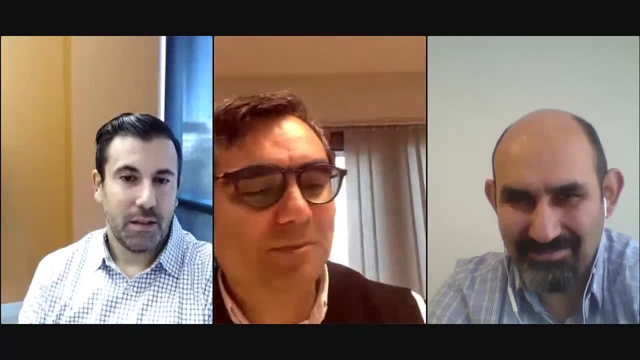 improvements to be made there, though overall so well. i would love to to read about your other tricks in in the paper that are coming out, because this is very interesting and exciting and i'm looking forward to that paper. and, uh, have you ever thought about maybe encapsulating the cells? 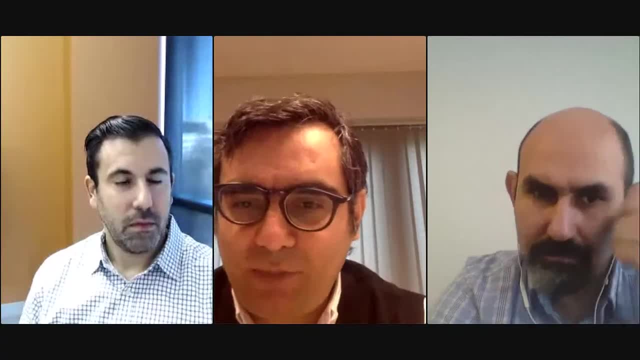 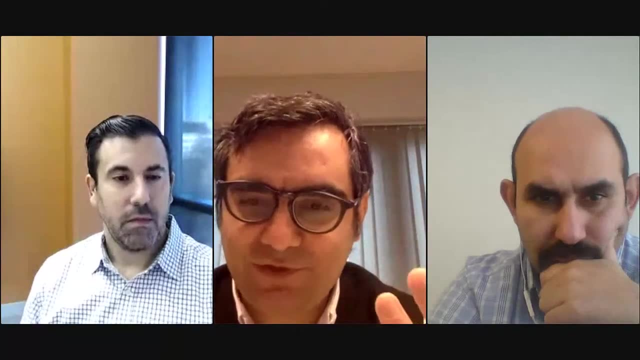 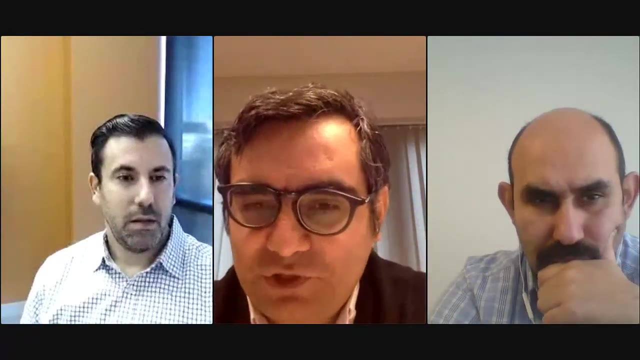 you showed some of the work with evan uh and then but but are you planning to use those hydrogel based micro particles so you encapsulate the cells in those hydrogen micro uh capsules and then print them as a way to avoid uh the effect of shear stress on them and the cells? 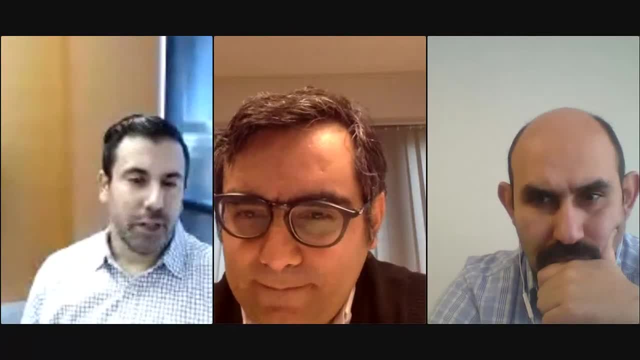 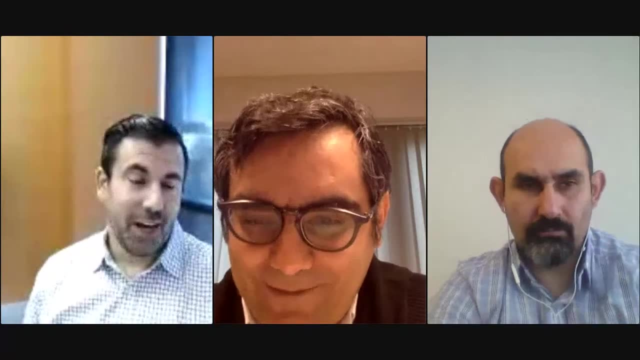 i think we're. we're still trying to figure out what, and i think that this is like the field is trying to figure out what is the best thing to print. yeah, i don't think there's an answer. yeah, it's probably also application dependent. yeah, like what are you trying to make you know also? 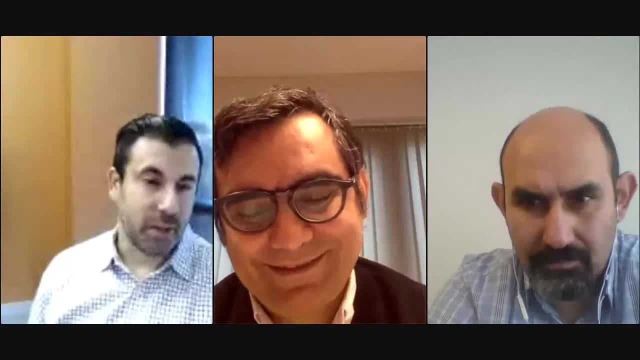 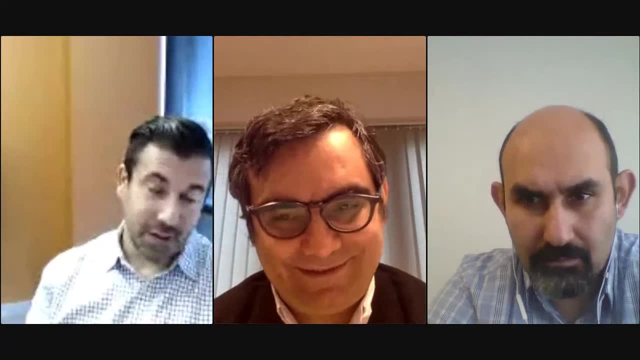 when we think about speed, those bigger cell spheroids or those encapsulated cells are also really interesting from a speed standpoint. yeah, because they're bigger. right, we have a bigger nozzle. whatever we're printing, we print faster because we've got a bigger nozzle and then we're. 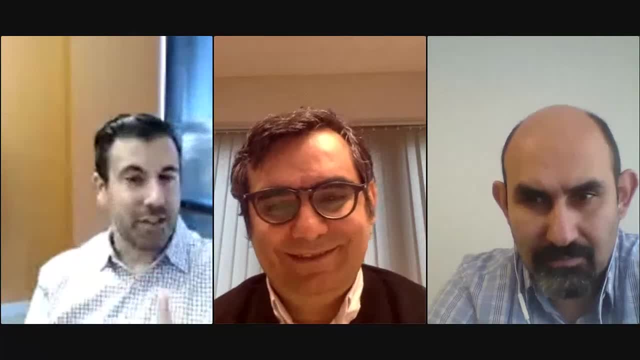 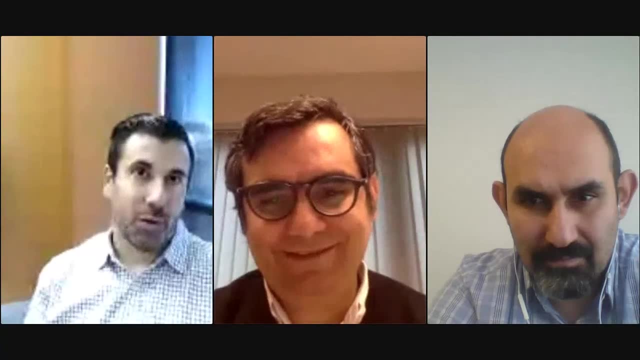 so that's another way to try to achieve. so we are trying to balance these different concerns and i think you know so we're not specifically using that, but we do have a project where we're- you know not where- we are trying to figure out: is that cell slurry? is that better than cell spheroids like? 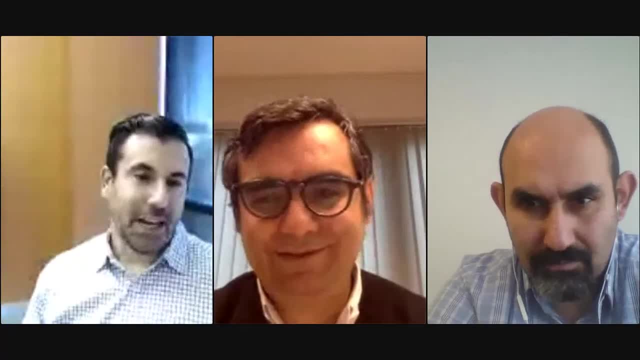 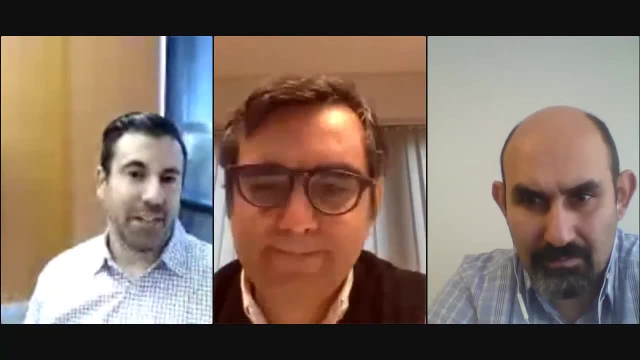 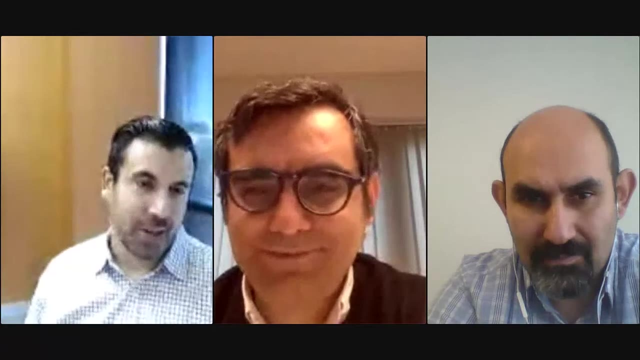 what's the right thing to be printing, and i think the answer is: we're really going to ultimately just want to have a toolbox where, for whatever we're actually trying to make, there's probably an ideal answer. uh, for that, for that approach, um, depending on size and speed and complexity of the tissue and so forth, well, great these. 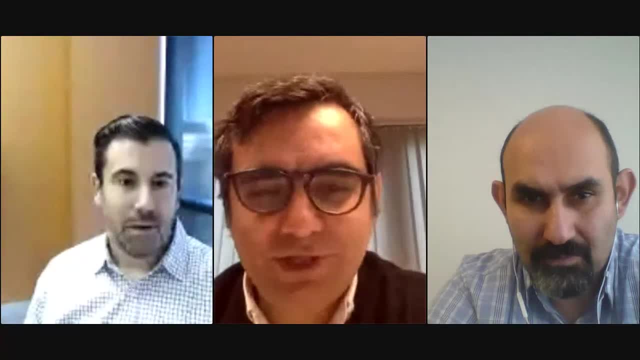 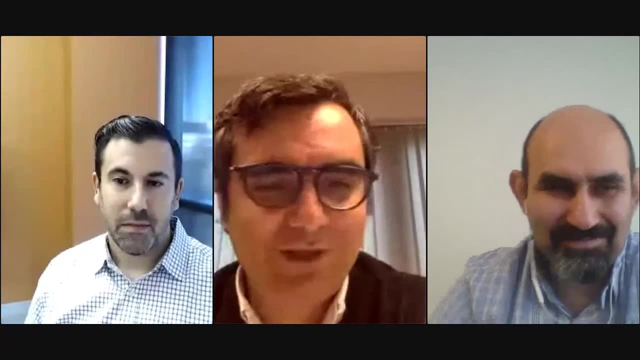 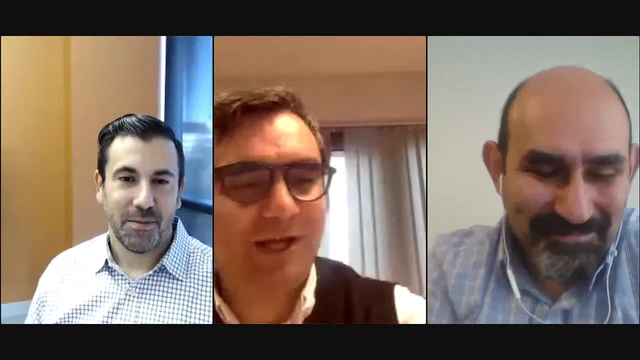 are great, uh uh projects, uh, for the future of 3d, fresh 3d printing. so i'll let human ask a few questions, if he has, because i know he is. he is in this field, he knows more than me about cardiovascular tissue engineering and he uses bioprinting, so i see that he's going up and down. 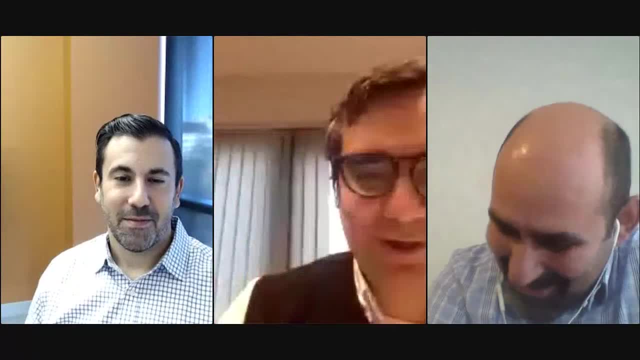 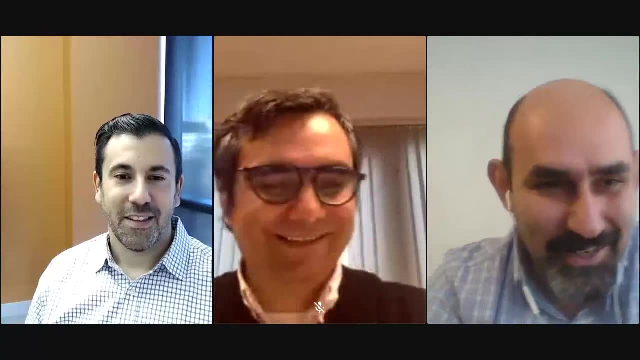 to ask questions, so i'll let him ask a few questions before. uh, yeah, i think that's it. this is the end of the video. i'm really looking forward to seeing what you've seen from this presentation. Thank you before I. thank you so much. thank you, Adam, for for the nice presentation. I. 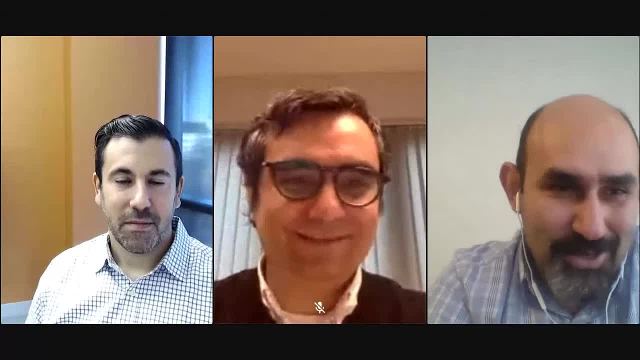 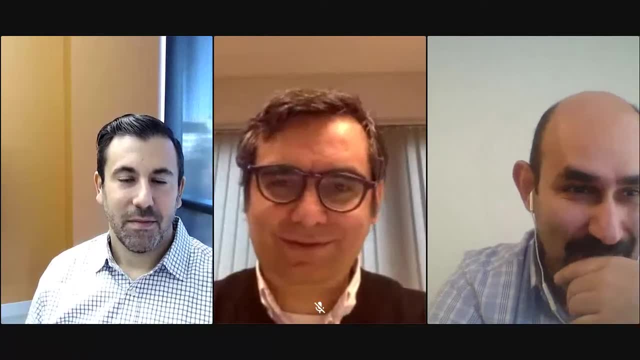 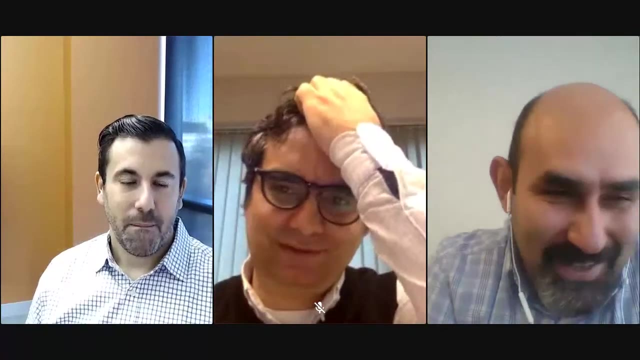 have been following your work since you started the fresh TD by printing, by publishing ACS by material science and technology, the first PDMS printing, you know, in so like, and after that science advances paper and then science papers. so it's really like exciting to see like this technology. I mean this technology. 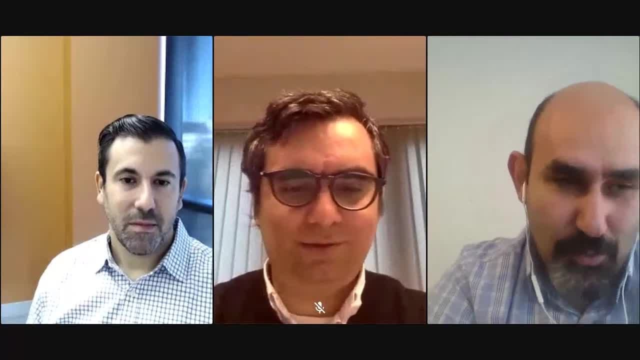 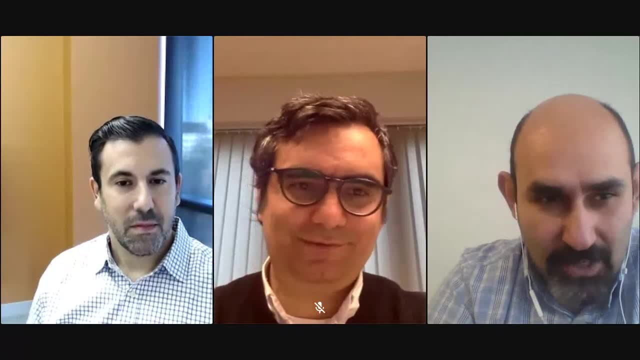 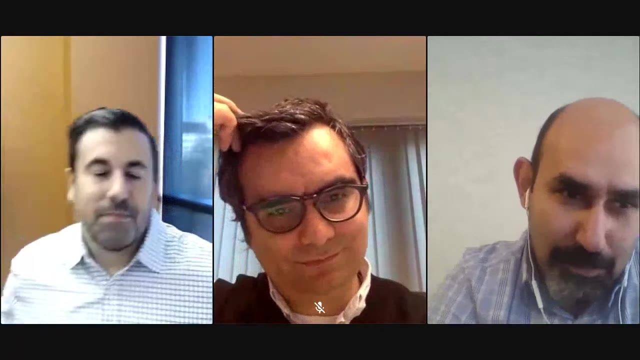 is growing fast, so like, as you mentioned. so there is no way. I just want to like clarify this: there's no way to print cells with collagen, since collagen is acid, right. so we, for the heart valve, we should always, you know, have the scaffold printed and then later on see that with the cells, right, because we do also fix. 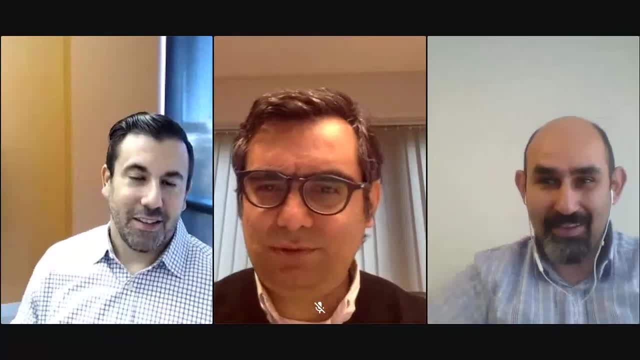 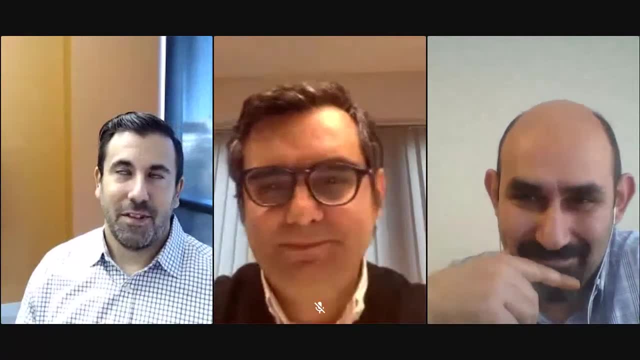 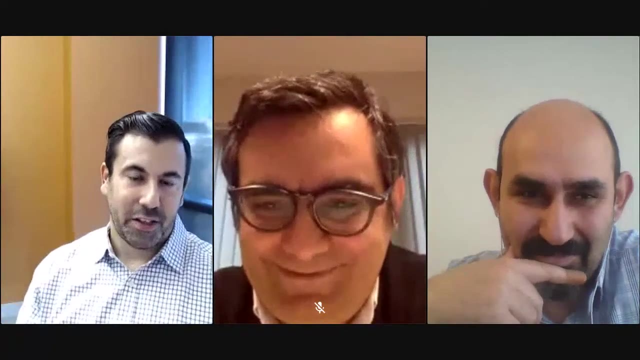 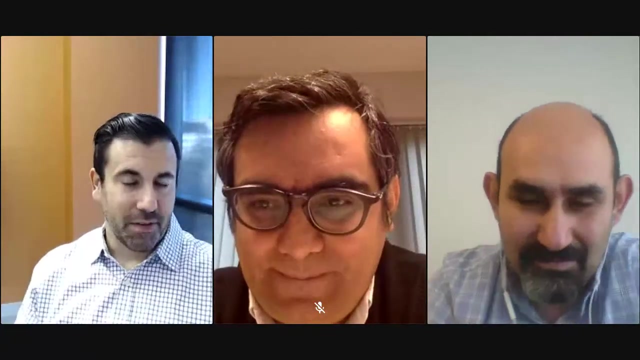 that with the cells, right. so I think that's one of the things that I would like to hear from you about is the presentation of the. so at the end of the printing right. well, so the, the collagen printing that we've published is is the acidify collagen. there are ways to print cells and collagen together, if you would. 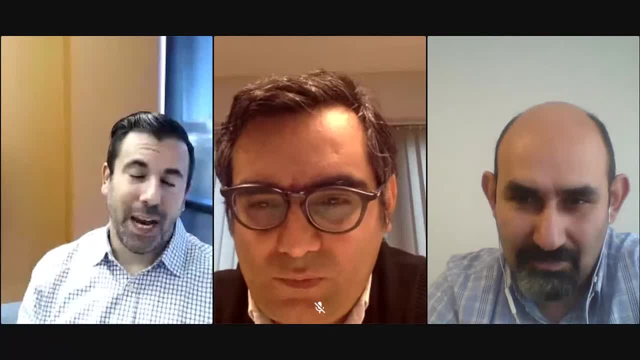 want, but you have to obviously use a different gelation mechanism than pH neutralization, right? we found that it's very easy to print cells with collagen- right? we found that it's very easy to print cells with collagen- right? we found that we got excited about that because the quality of the collagen that comes 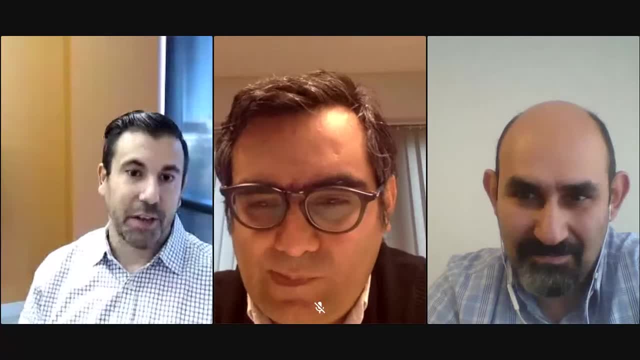 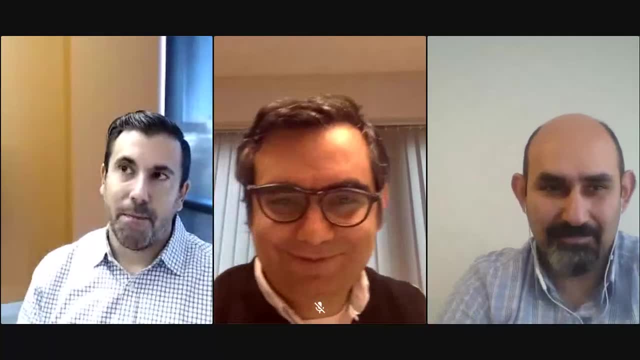 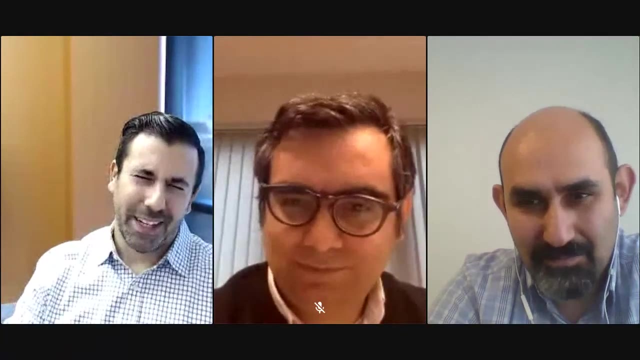 out of that process is pretty phenomenal. it actually allows us to create things like durable heart valves, which is typical. it's tough with our needles, right but, and actually to give you an idea of like how far we can take that you know that valve, I think, was printed with like around 24 make per mil. collagen. we're pushing that close to a hundred make per mil collagen. now, right, and so the mechanical properties are even much, much better, even before you do an additional cross like it. but those materials are actually brick wall, like that's a brick wall to a cell, like collagen at that density properly. 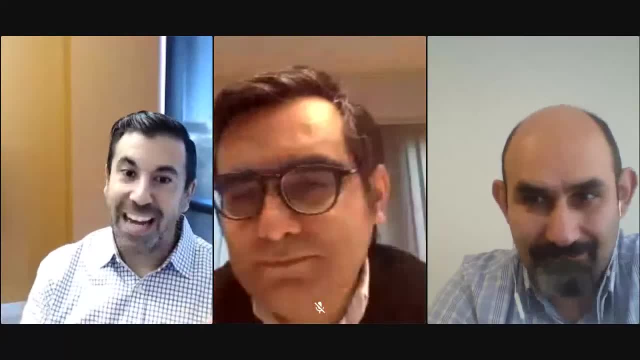 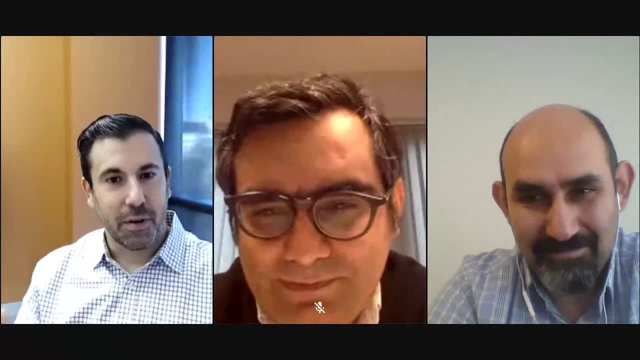 assembled at that concentration, like cells are not getting through that anytime soon. so so really just depends on what you're trying to do. so that might be interesting for printing more of like a cartilage, where you would want a low density of cells, maybe embedded in collagen, and there's some ways we're. 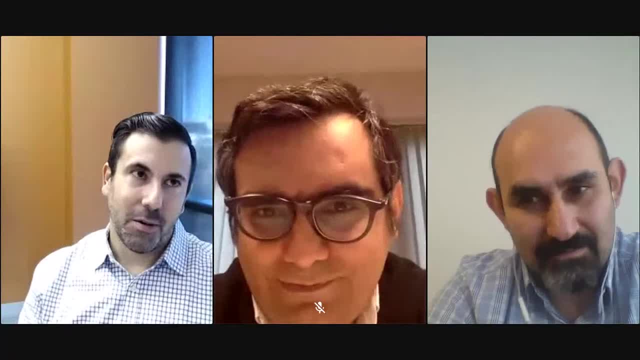 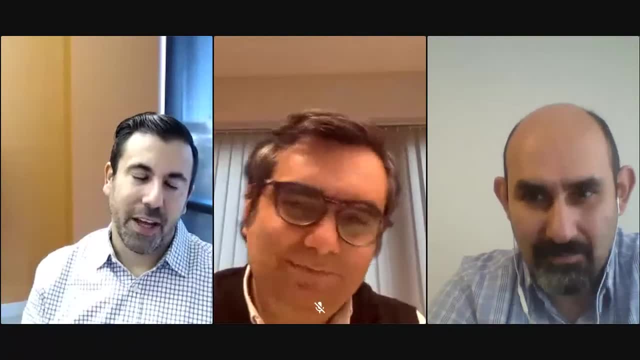 thinking about trying to do that, but otherwise, you know. you know the collagen is different. we are mixing in the collagen with some other bio inks, like that cell based bio ink that we're printing with hundreds of millions of cells per ml. actually that has fibrin in it. so that's how we gel. 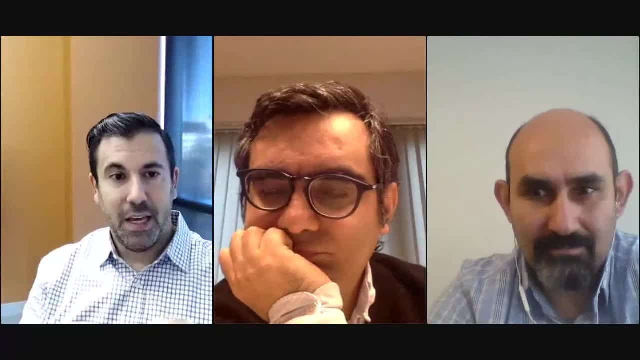 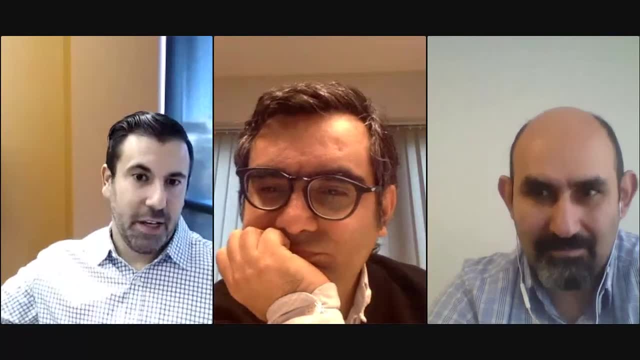 that there's fibrinogen in there, there's thrombin in the bath and it just. it holds the structure just long enough so that once you put in the incubators the cells can spread out and connect and stabilize themselves. but I think we all know like fibrin is a really weak gel. it's not going to be able to get out of the gel, especially compared to collagen at similar mass. right, you know, we use collagen at maybe 10 make per mil. we typically use fibrin much, much higher. so but yeah, there are ways to again get the collagen as the, as the matrix, but you, you can't use this acidified approach to do the gelation. you, you could use them a. 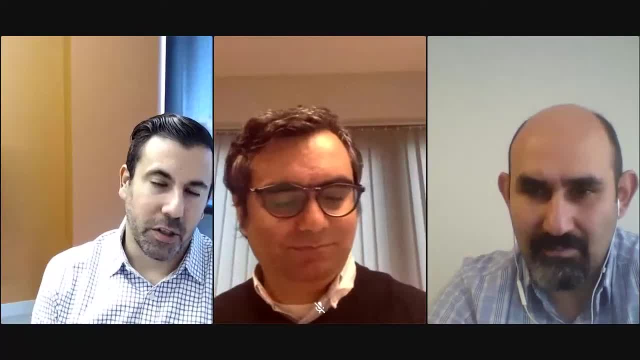 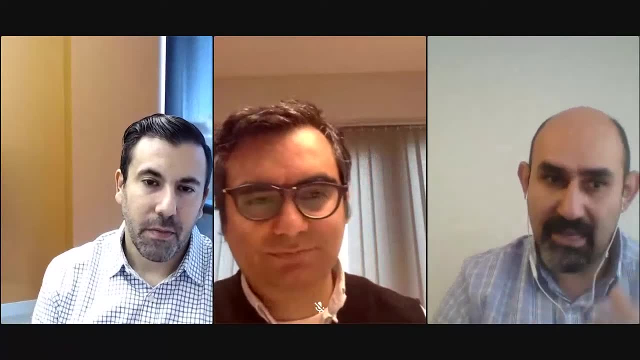 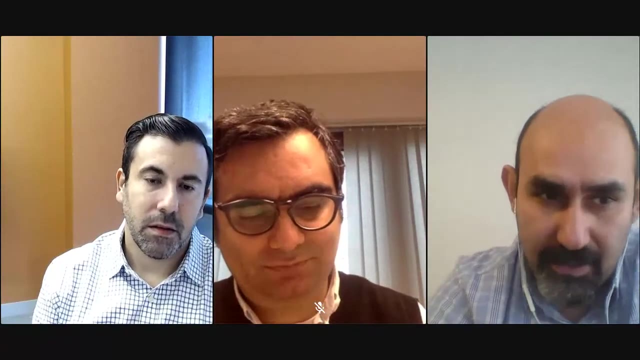 fact related. you could also do some thermal based approaches if you timing right. so and the other thing is the fixation and the fixation is the fixation. I mean if you have the cells and you fix the cells to increase them, fix that the construct to increase the mechanical property with glutar guide, so that will. 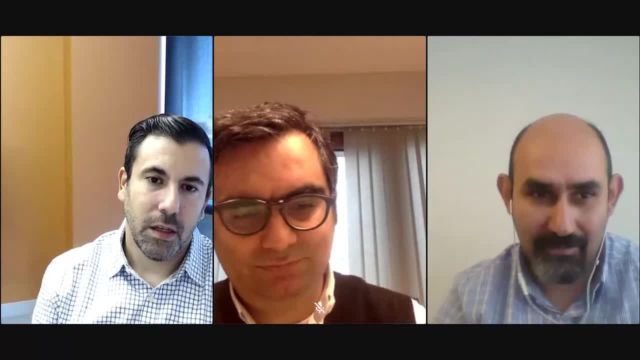 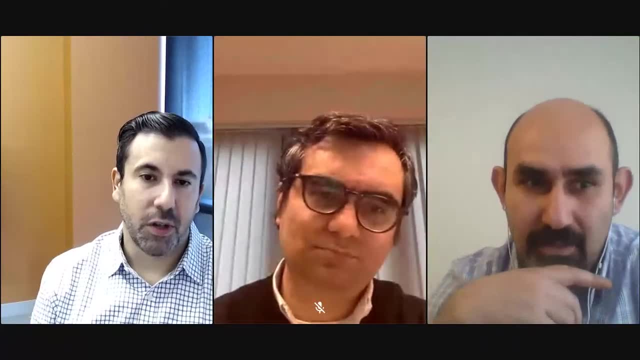 also is kind of bottleneck or limitation, and yeah, exactly so. our fixed valves are not meant to actually be like regenerative, they're actually more of like a medical device, really just like normal porcine valve. it's just: can we, can we make them better by, you know again, matching patient anatomy. 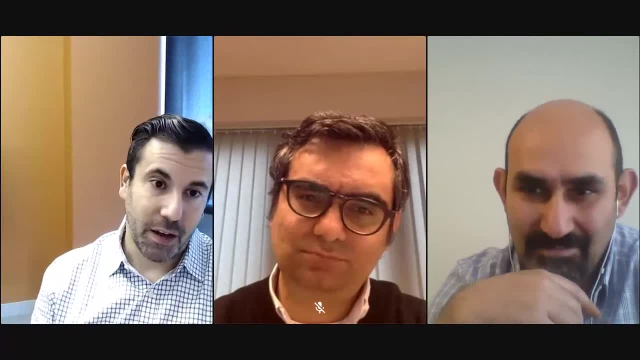 optimizing the fluid mechanics right through the valve, making sure that it's right through the valve, making sure that it's right through the valve, making sure right through the valve, making sure that it's right through the valve, making sure it may be easier to fold for transcatheter delivery. those kinds of 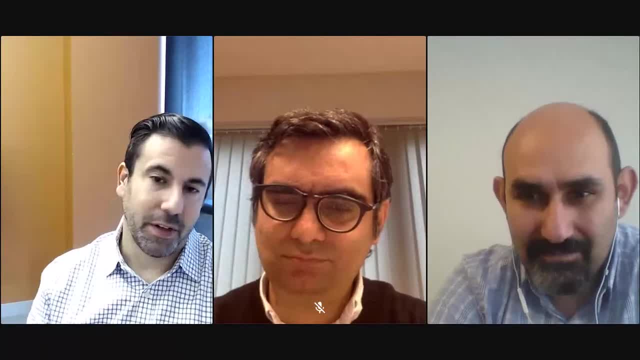 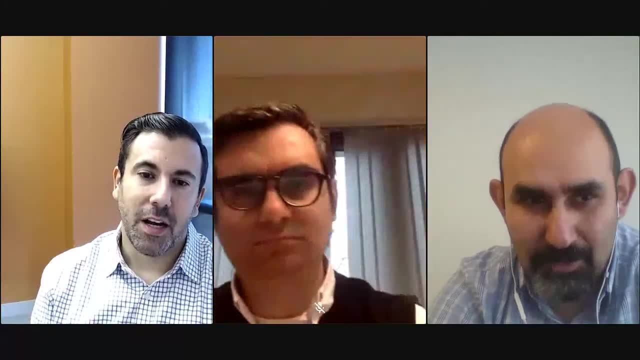 it may be easier to fold for transcatheter delivery, those kinds of things. for a regenerative valve, you would definitely you can't cross like it. things for a regenerative valve, you would definitely you can't cross like it and in fact you know it would be a very different kind of device. but even with and in fact you know it would be a very different kind of device. but even with that, I think you, you ask the question of like, how would you even want to sell that? I think you, you ask the question of like, how would you even want to sell? 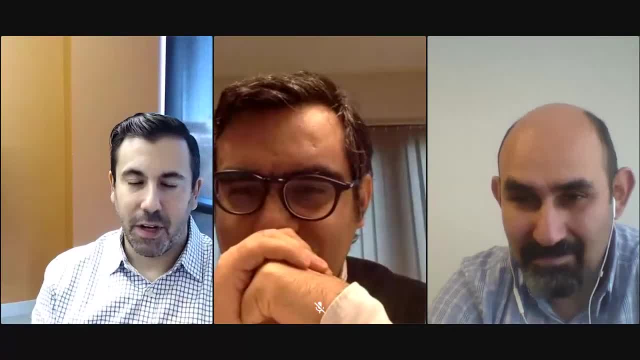 your eyes a regenerative valve right? you might think that, if you know, do you your eyes a regenerative valve right? you might think that, if you know, do you need to end of the allies the surface, because maybe that can happen once. you. need to end of the allies the surface because maybe that can happen once you. 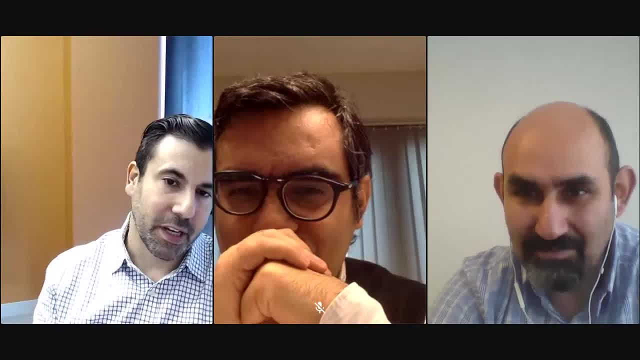 implant it. but for valve interstitial cells, do you need to print those into implant it? but for valve interstitial cells, do you need to print those into the construct? I think those are questions we have with a lot of the the construct. I think those are questions we have with a lot of the. 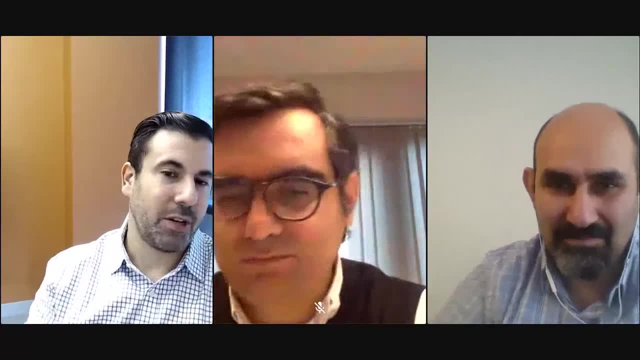 tissues we're trying to create, right. how do we? how do we create them? what do we tissues we're trying to create, right? how do we? how do we create them? what do we want to print as we go? what can we maybe see later or if it's going to be? 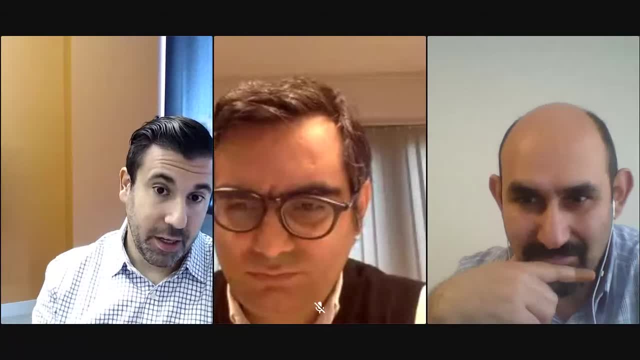 want to print as we go, what can we maybe see later. or if it's going to be implanted in vivo, what can it actually recruit from the host from a implanted in vivo? what can it actually recruit from the host from a cellularization standpoint? because you know the reason our bigger hearts are. 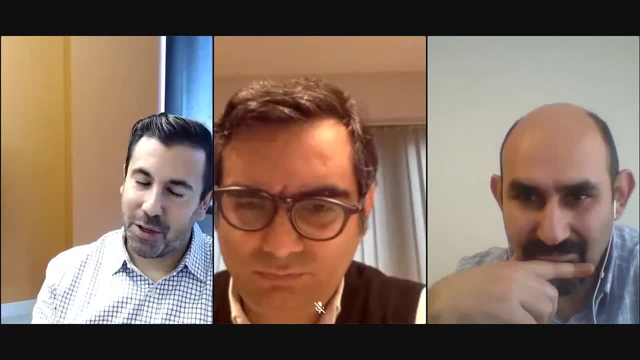 cellularization standpoint, because you know, the reason our bigger hearts are not cellularized. is that, hey, it's it's, we don't really have enough time to not cellularized is that? hey, it's it's. we don't really have enough time to print it that big. but it's really just hard to get enough cells right. the, the. 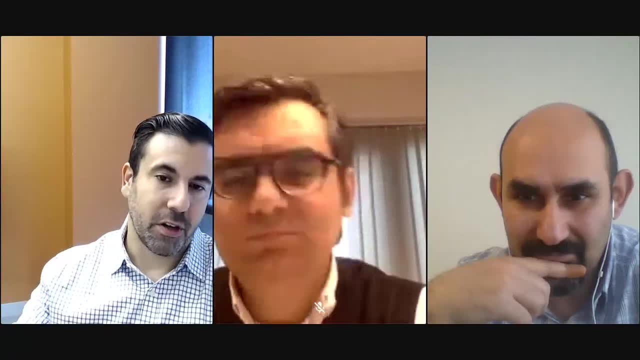 print it that big but it's really just hard to get enough cells right the the. the cost of doing IPS derived human stem cell cardiomyocytes is very high. so for cost of doing IPS derived human stem cell cardiomyocytes is very high. so for me to generate billions of those cells for a construct is basically just not. 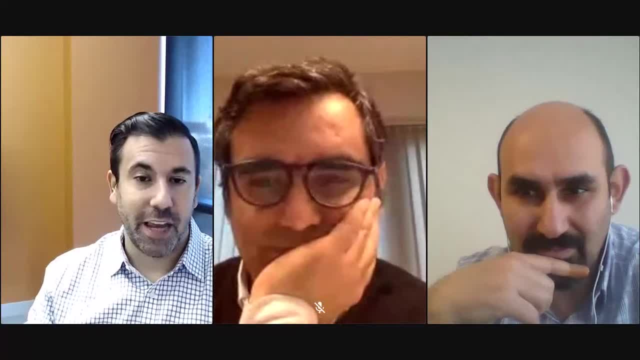 me to generate billions of those cells for a construct is basically just not feasible at today's cost and scale and ease of production. so that'll, I think, be feasible at today's cost and scale and ease of production. so that'll, I think, be solved right. there's a lot of folks working and sell stem cell based you. 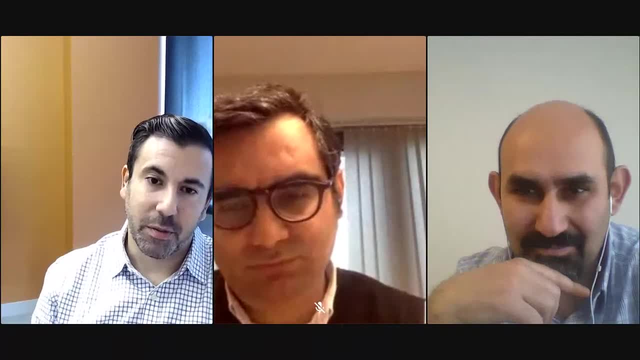 solved right. there's a lot of folks working and sell stem cell based. you know expansion technologies, but today those are some of the limitations. great know expansion technologies, but today those are some of the limitations. great know expansion technologies, but today those are some of the limitations. great. thank you so much, and maybe one more. 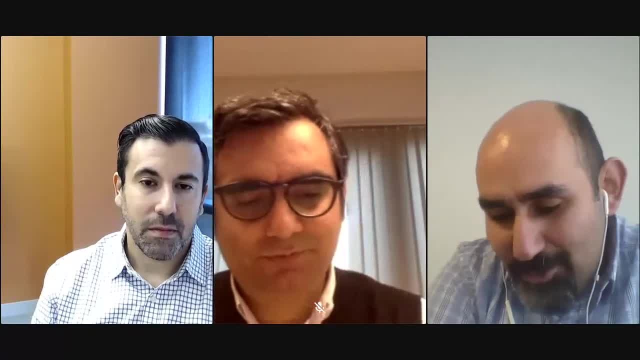 thank you so much and maybe one more. thank you so much and maybe one more. question about like a heart ventricle. so question about like a heart ventricle. so question about like a heart ventricle. so how far we are from you know, having a. 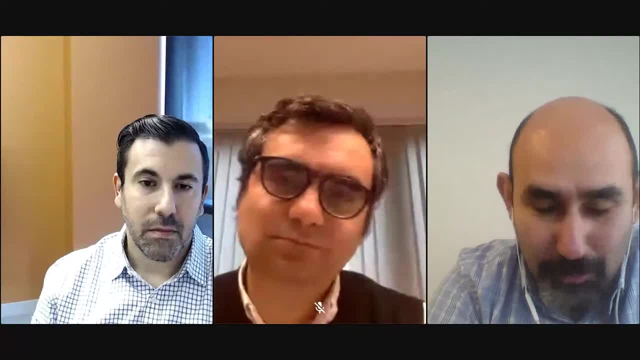 how far we are from you know having a. how far we are from you know having a heart ventricle pumping the fluid out of heart ventricle, pumping the fluid out of heart ventricle, pumping the fluid out of. so you didn't measure the output, but I 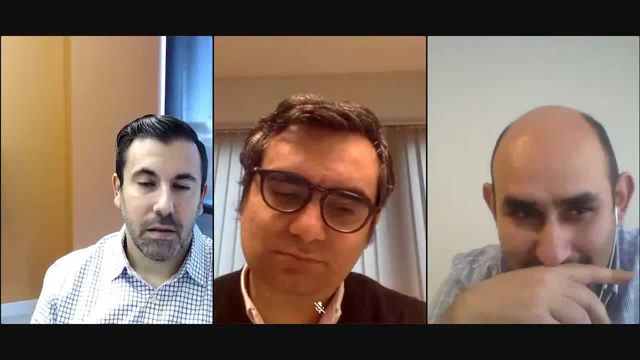 so you didn't measure the output, but I. so you didn't measure the output. but I know that some people do it, but how far know that some people do it. but how far know that some people do it. but how far we are from that to have the bioprinted. 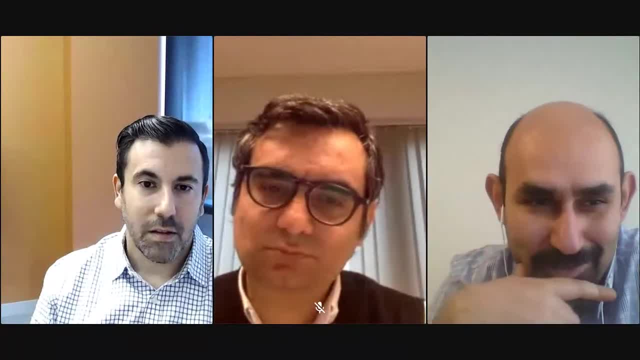 we are from that to have the bioprinted. we are from that to have the bioprinted heart ventricle pushing out or pumping heart ventricle pushing out or pumping heart ventricle pushing out or pumping out the fluid. we're not too far from. 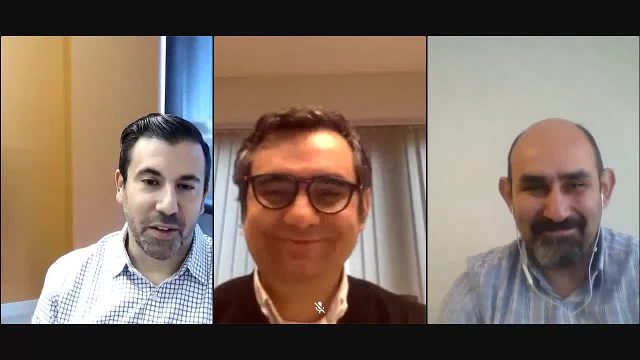 out the fluid. we're not too far from out the fluid. we're not too far from that. yeah, I wouldn't be overly that. yeah, I wouldn't be overly that. yeah, I wouldn't be overly impressed by the flow rates. yeah, we're impressed by the flow rates. yeah, we're. 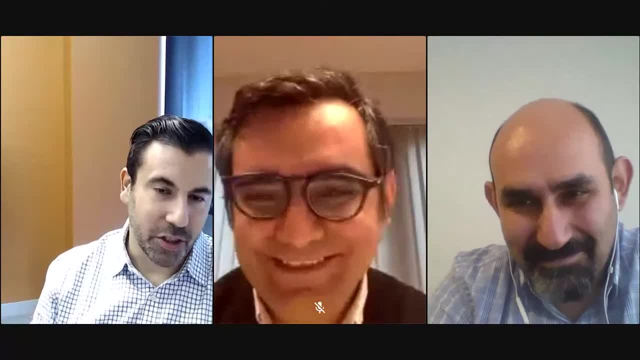 impressed by the flow rates. yeah, we're not too far from that, at least like. not too far from that, at least, like. not too far from that, at least. like basic proof of concept being shown. yeah, basic proof of concept being shown. yeah, basic proof of concept being shown. yeah, we're not too far, too far from that you. 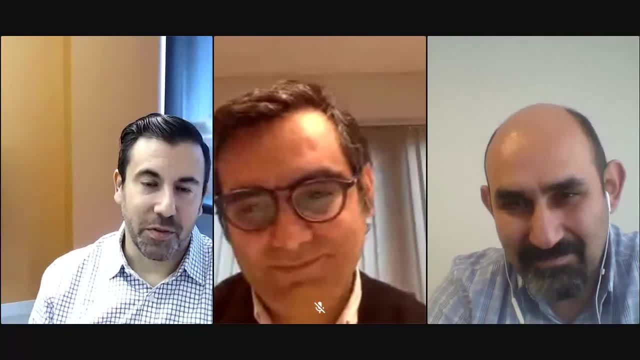 we're not too far too far from that. you we're not too far too far from that. you know we're really. I mean that's that's know we're really. I mean that's that's know we're really. I mean that's that's, you know. that's a nice proof of concept. 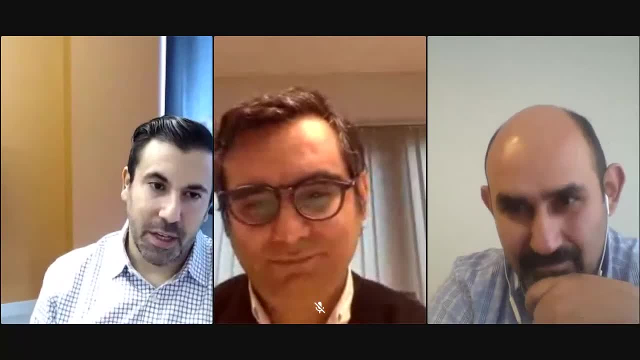 you know that's a nice proof of concept. you know that's a nice proof of concept we're really interested in once you have. we're really interested in once you have. we're really interested in once you have a closed pressurized system control, a closed pressurized system control. 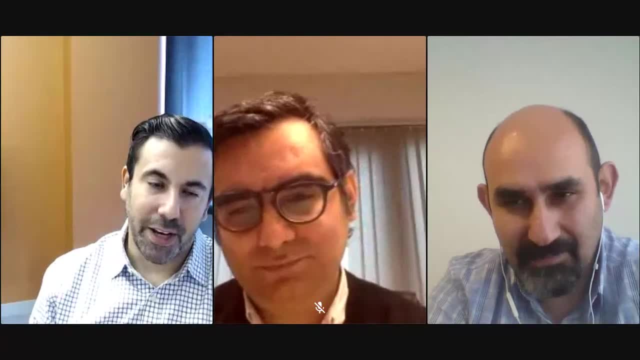 a closed, pressurized system control preload and afterload right. can we preload and afterload right? can we preload and afterload right? can we start to use that to help drive the start, to use that to help drive the start, to use that to help drive the? the structural and mechanical maturation of 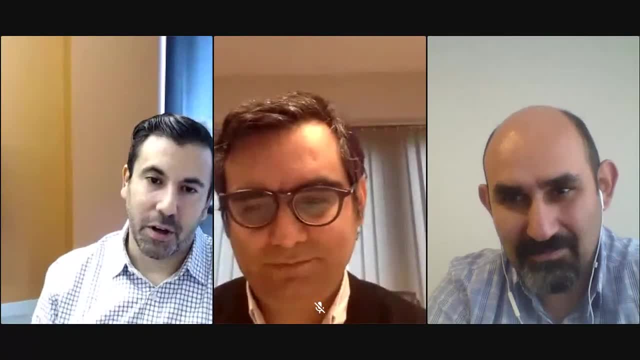 the structural and mechanical maturation of the structural and mechanical maturation of the of the IPS or derived. you know the of the IPS or derived. you know the of the IPS or derived. you know cardiac tissue. so that's really kind of cardiac tissue, so that's really kind of. 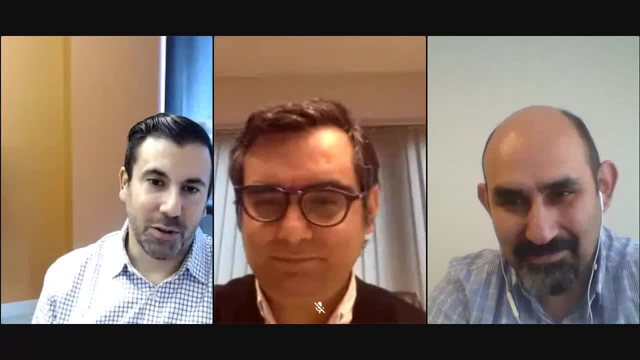 cardiac tissue. so that's really kind of what we're we're focusing on. it's like what we're we're focusing on. it's like what we're we're focusing on. it's like, now that we have these tools, we can. now that we have these tools, we can. 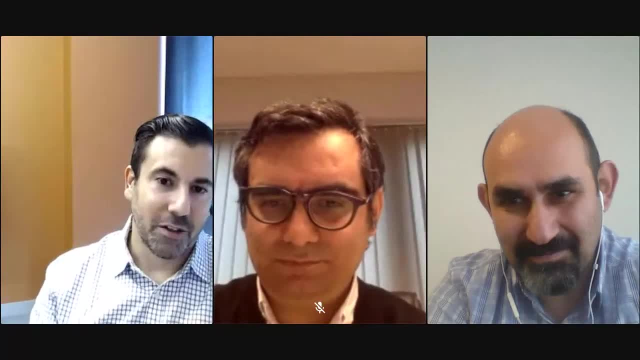 now that we have these tools, we can actually do the more of the science of actually do. the more of the science of actually do, the more of the science of like trying to understand what what we like, trying to understand what what we like, trying to understand what what we need to do to build better muscle. you. 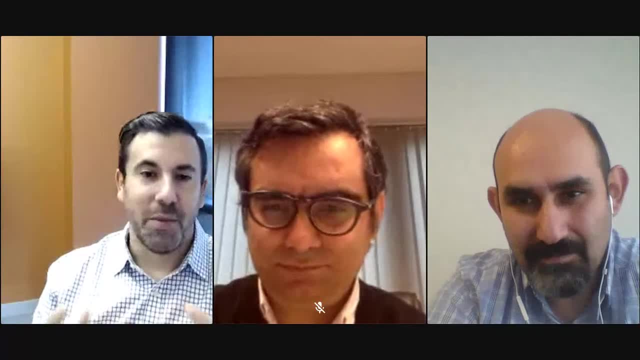 need to do to build better muscle. you know, there's obviously the there's know, there's obviously the there's know, there's obviously the there's, there's the matrix, there's the tissue, there's the matrix, there's the tissue, there's the matrix, there's the tissue stiffness, there's the the stress and 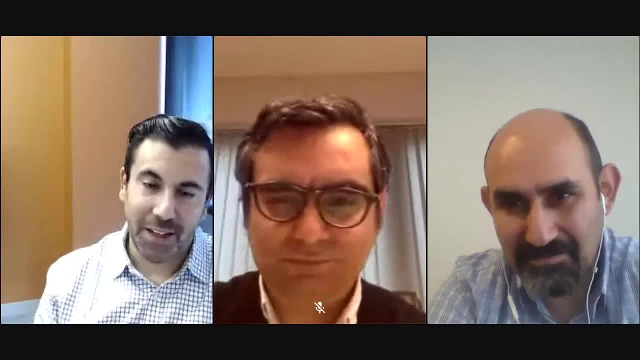 stiffness. there's the the stress and stiffness. there's the the stress and strain on the tissue. there's the strain on the tissue. there's the strain on the tissue. there's the different cell types. there's things you different cell types. there's things you different cell types. there's things you can add to the media. there's- there's a. 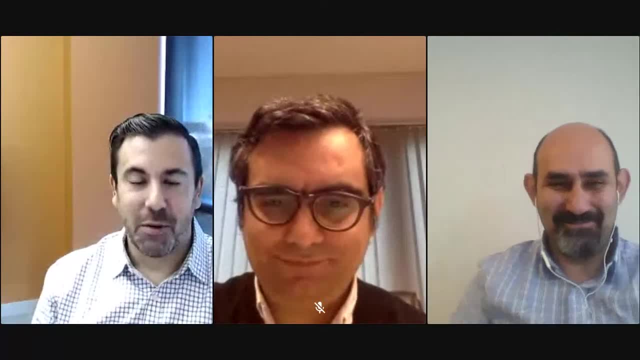 can add to the media there's. there's a can add to the media. there's. there's a lot of stuff. so we're really focused on lot of stuff. so we're really focused on lot of stuff. so we're really focused on building a test bed so we can start to. 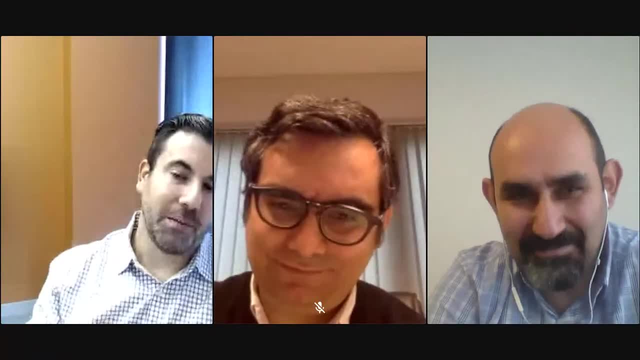 building a test bed, so we can start to building a test bed, so we can start to to understand some of these things, so I to understand some of these things, so I to understand some of these things. so I think that's, that's a, it's important. I. 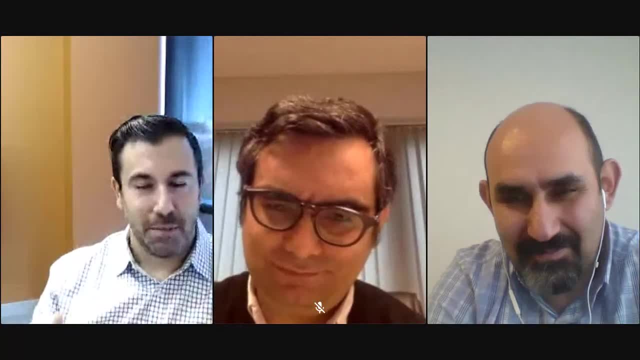 think that's, that's a it's important. I think that's, that's a it's important. I think the, at least from our standpoint, to think the at least from our standpoint, to think the at least from our standpoint, to build a test platform. you know, pause a. 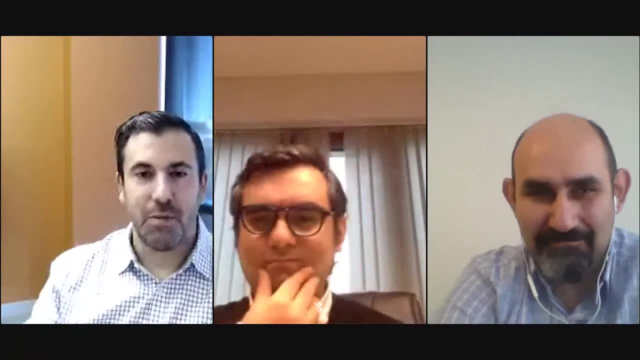 build a test platform. you know, pause a. build a test platform, you know, pause a little bit. do some basic science and little bit do some basic science and little bit do some basic science. and hypothesis testing: better understand hypothesis testing, better understand hypothesis testing, better understand what's going on and then hopefully then 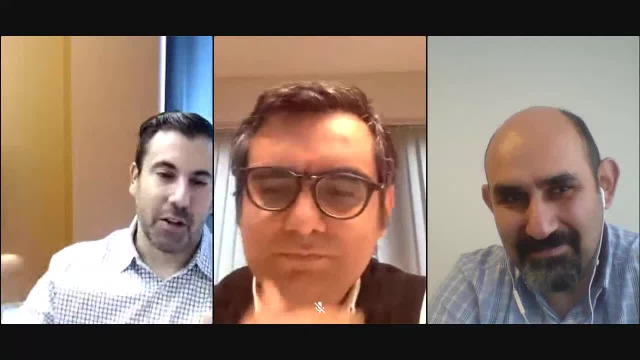 what's going on and then hopefully, then what's going on and then hopefully then take those lessons and then move that to take those lessons, and then move that to the next larger scale of constructs, the next larger scale of constructs, the next larger scale of constructs. so, yeah, very exciting. so just before I 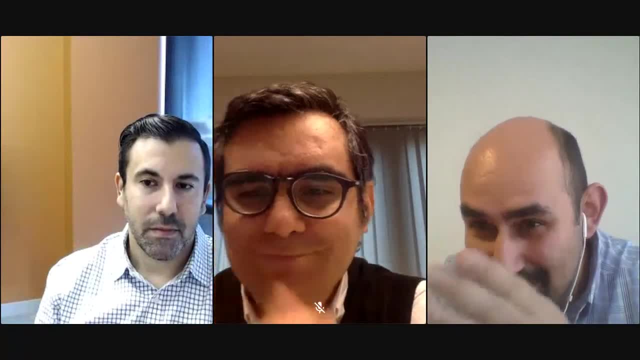 so yeah, very exciting. so just before I. so yeah, very exciting. so just before I pass the most and I see lots of nice pass the most, and I see lots of nice pass the most. and I see lots of nice comments, nice comments in the chat box comments. nice comments in the chat box. 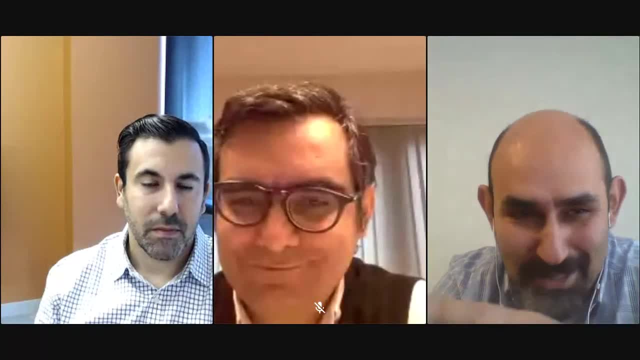 comments: nice comments in the chat box about your talk and participants are about your talk and participants are about your talk and participants are really excited about your talk and also really excited about your talk and also really excited about your talk. and also we got many question in the Q&A box. 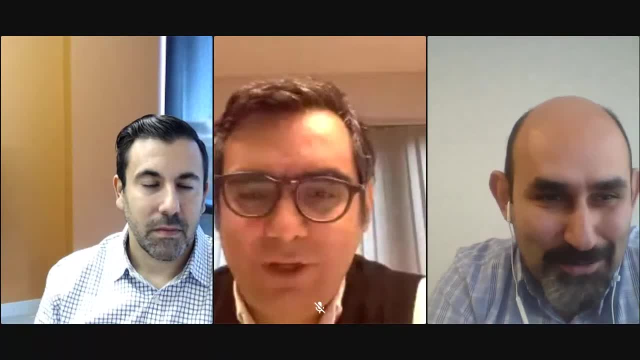 we got many question in the Q&A box. we got many question in the Q&A box that most them probably can moderate, that most them probably can moderate, that most them probably can moderate. thank you so much sure, yeah, well for. thank you so much sure, yeah, well for. 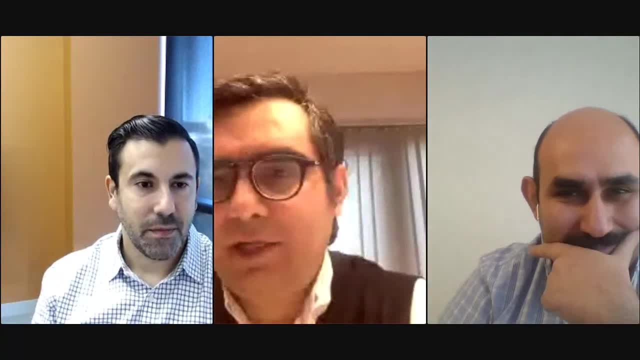 thank you so much. sure, yeah, well, for sure, again it's. it's very exciting and sure again it's. it's very exciting and sure again it's. it's very exciting and interesting to see that a multi. interesting to see that a multi. interesting to see that a multi disciplinary approach in which 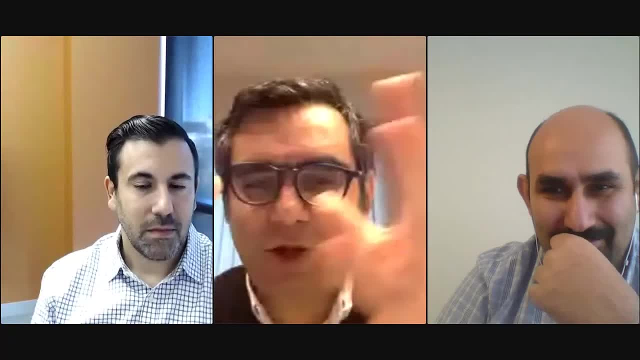 disciplinary approach in which disciplinary approach in which engineers, cellular biologists, material engineers, cellular biologists, material engineers, cellular biologists, material sciences they've come together and then sciences they've come together and then sciences they've come together and then develop this amazing technology that develop this amazing technology that 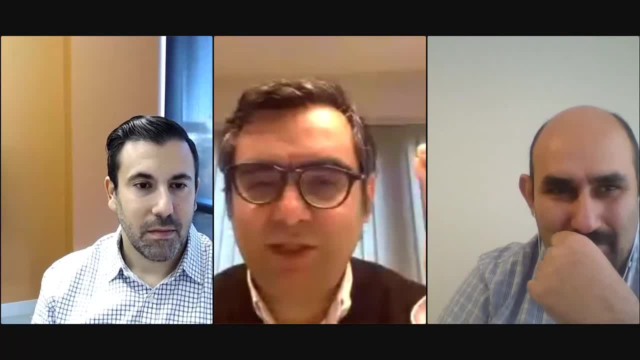 develop this amazing technology that, hopefully, at some point it will solve, hopefully, at some point it will solve, hopefully, at some point it will solve the issue that ever like that. we have the issue that ever like that. we have the issue that ever like that. we have right now a big clinical issue of 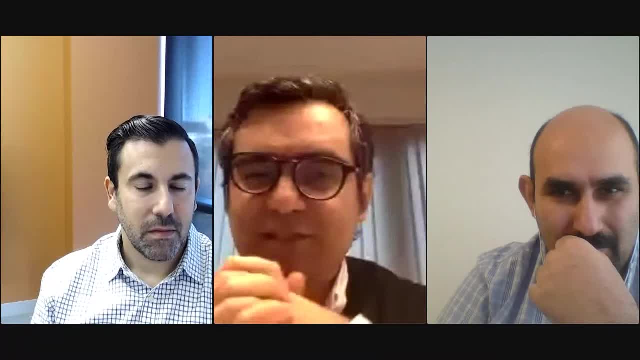 right now, a big clinical issue of right now, a big clinical issue of basically organ transplantation: heart basically organ transplantation, heart basically organ transplantation. heart transplantation is a major challenge and transplantation is a major challenge, and transplantation is a major challenge, and then a major clinical challenge, and then 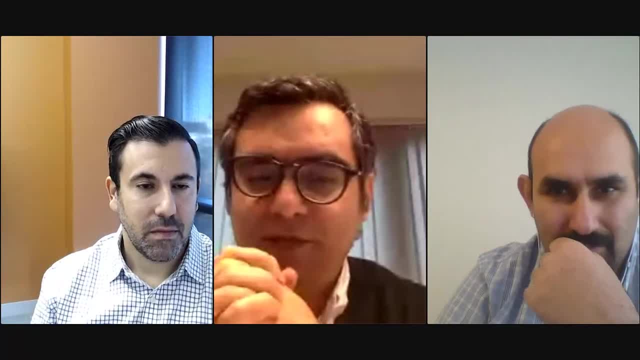 then a major clinical challenge, and then then a major clinical challenge, and then at some one point, I'm very optimistic at some one point, I'm very optimistic at some one point. I'm very optimistic that, with, with all the efforts that that, with, with all the efforts that 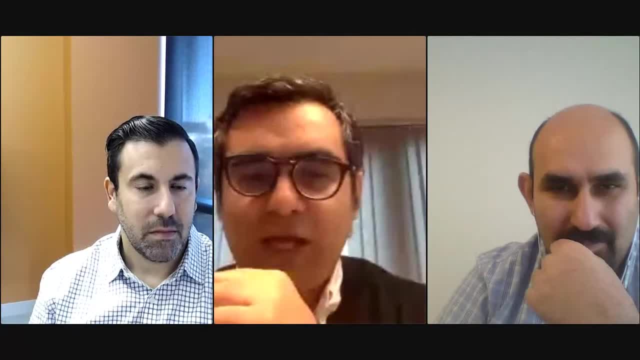 that, with with all the efforts that researchers such as dr Feinberg and researchers such as dr Feinberg and researchers such as dr Feinberg and others are putting into this technology, others are putting into this technology, others are putting into this technology. at some point we will have these beating. 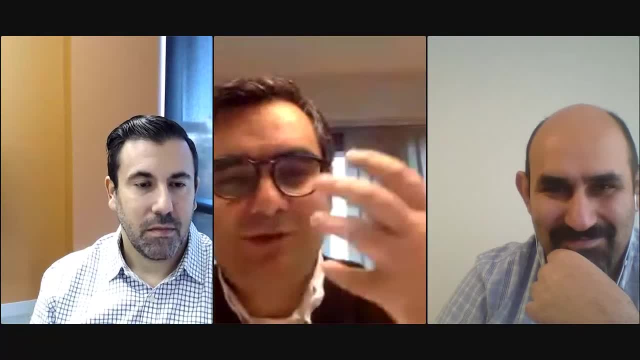 at some point we will have these beating. at some point we will have these beating hearts from like patient cells derived hearts from like patient cells derived hearts from like patient cells derived from patient cell built in a in a lab. from patient cell built in a in a lab. 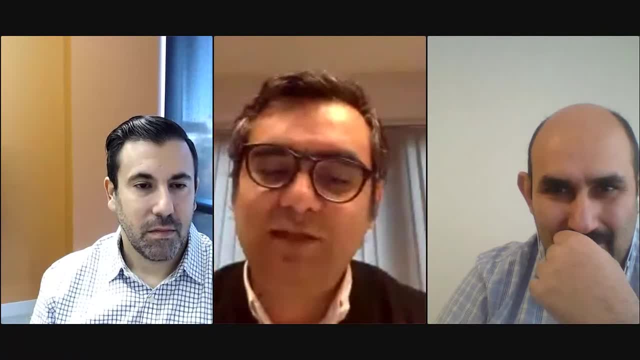 from patient cell built in a in a lab and that they can be implanted in the and that they can be implanted in the and that they can be implanted in the inpatients and save their lives. so it's inpatients and save their lives. so it's. 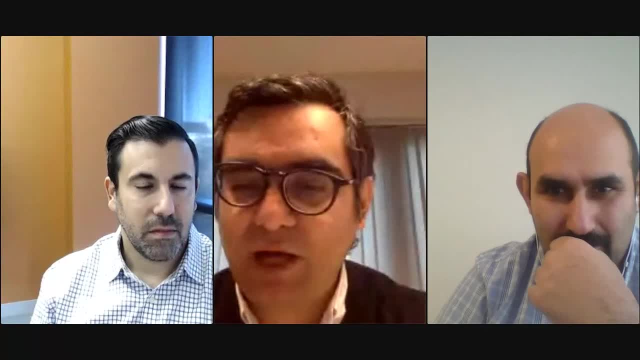 inpatients and save their lives. so it's it's amazing how, how the technology is. it's amazing how, how the technology is. it's amazing how how the technology is moving forward and I would like to ask moving forward. and I would like to ask moving forward and I would like to ask another question from the audience, which 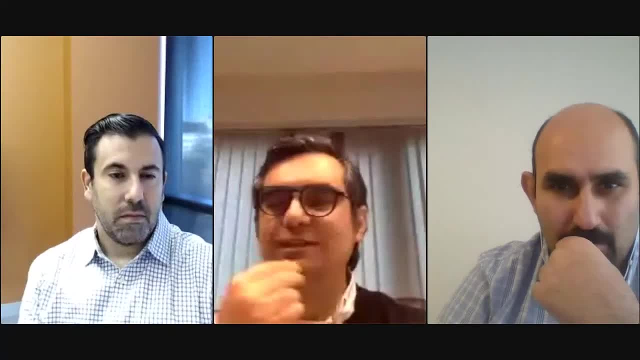 another question from the audience. which another question from the audience, which is from Mayim, and then she's she is is from Mayim, and then she's she is is from Mayim, and then she's she is asking about the types of hydrogels that. 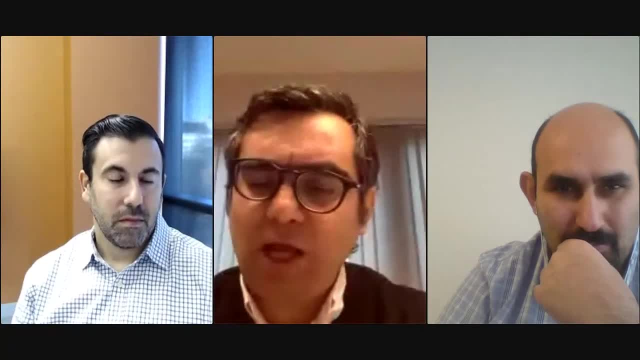 asking about the types of hydrogels that, asking about the types of hydrogels that you're using for in fresh by printing. you're using for in fresh by printing. you're using for in fresh by printing. what are they? when you want to choose a, 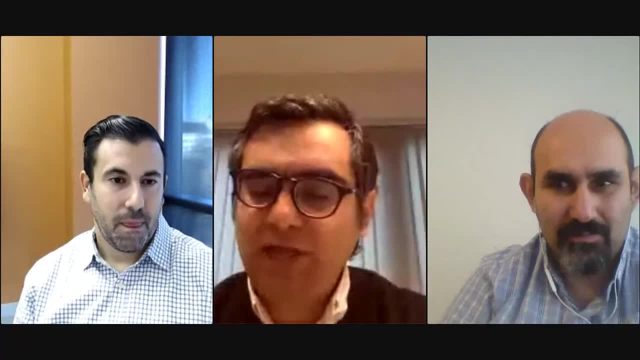 what are they when you want to choose a? what are they when you want to choose a hydrogel or design a hydrogel? how? what hydrogel? or design a hydrogel? how? what hydrogel? or design a hydrogel- how? what kind of characteristics are you looking? 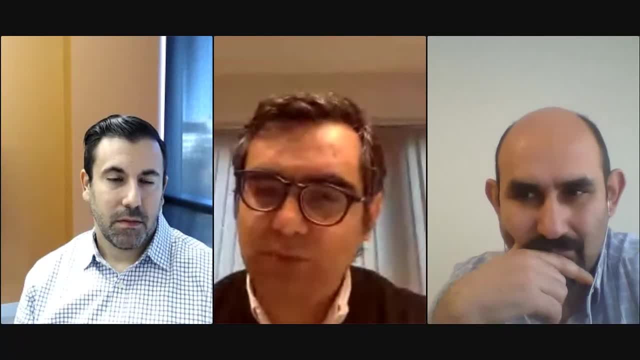 kind of characteristics are you looking kind of characteristics are you looking for for this particular printing, for for this particular printing, for for this particular printing approach? yeah, it's a really good approach. yeah, it's a really good approach. yeah, it's a really good question. so you know the things that. 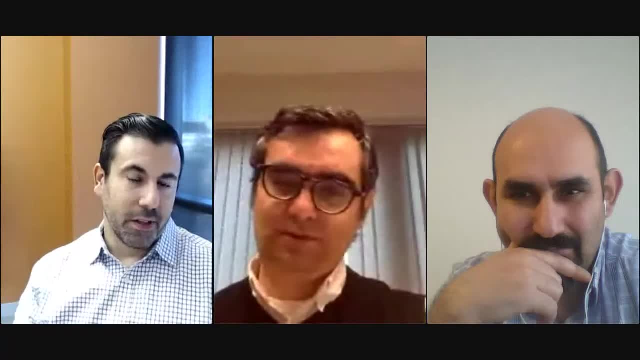 question. so you know the things that question. so you know the things that work best. you know that are hydrogels work best. you know that are hydrogels work best. you know that are hydrogels. are things that when you extrude it is, are things that, when you extrude it is. 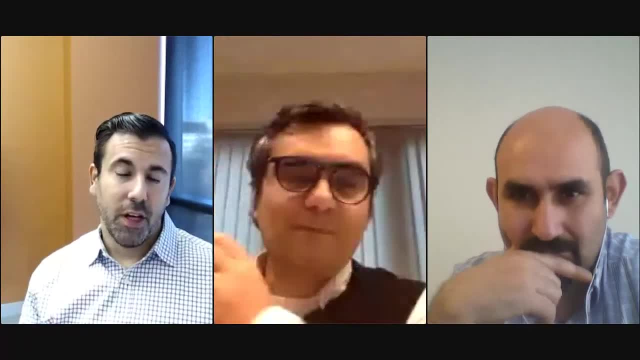 are things that when you extrude, it is gonna gel rapidly through some mechanism. gonna gel rapidly through some mechanism. gonna gel rapidly through some mechanism that you control, otherwise it'll just that you control otherwise. it'll just that you control, otherwise it'll just diffuse away, right. so that's really the. diffuse away right. so that's really the diffuse away right. so that's really the major thing and I think what's been nice major thing and I think what's been nice major thing and I think what's been nice if we've shown that it's, you know it. 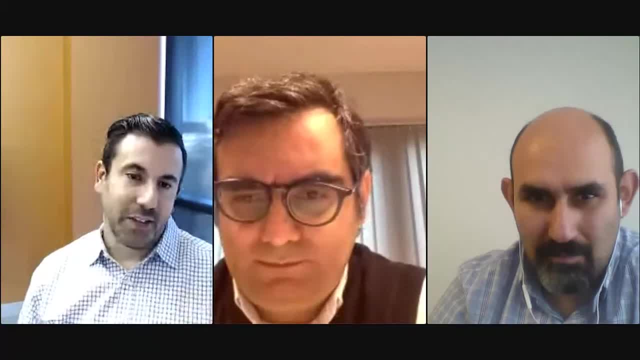 if we've shown that it's, you know it. if we've shown that it's, you know it could be. you know pH driven, you know could be. you know pH driven, you know could be. you know pH driven. you know ionic enzymatic UV actually, you know as. 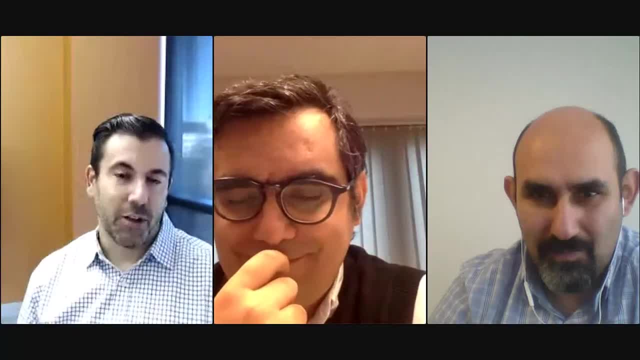 ionic enzymatic UV. actually you know as ionic enzymatic UV. actually, you know, as a little teaser. we have a collaborative, a little teaser. we have a collaborative, a little teaser. we have a collaborative paper with lab of Sarah Hileshorn at. paper with lab of Sarah Hileshorn at. 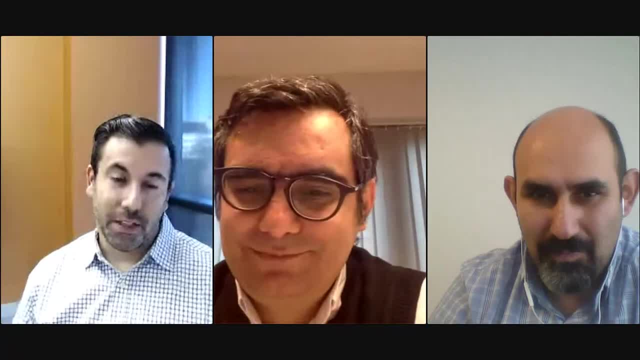 paper with lab of Sarah Hileshorn at Stanford University. that will that's Stanford University. that will. that's Stanford University. that will that's accepted and hopefully we'll be out. you accepted and hopefully we'll be out. you accepted and hopefully we'll be out, you know, in a matter of weeks, using a click. 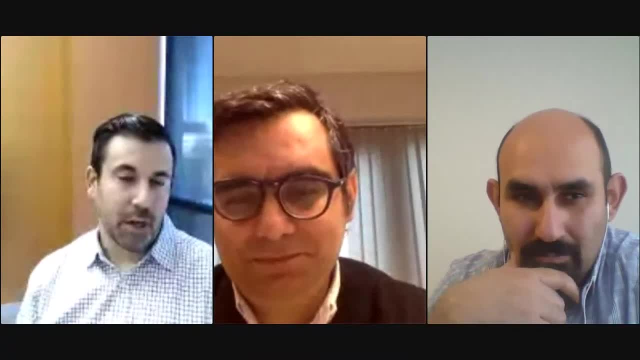 know in a matter of weeks using a click. know in a matter of weeks using a click. chemistry based crosslinker. that's in chemistry based crosslinker. that's in chemistry based crosslinker. that's in the support path for a range of bio. the support path for a range of bio. 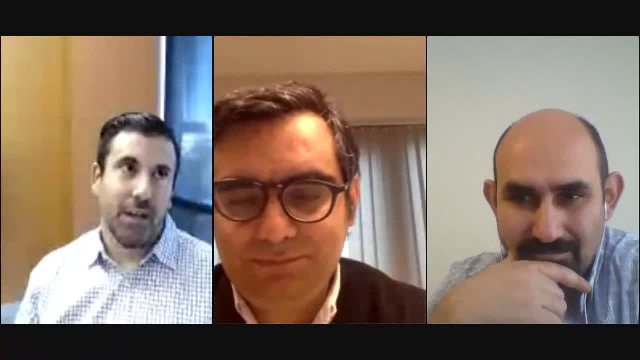 the support path for a range of bio links as well. and so that really shows I links as well, and so that really shows I links as well, and so that really shows. I think that any you need the crosslinker, think that any you need the crosslinker. 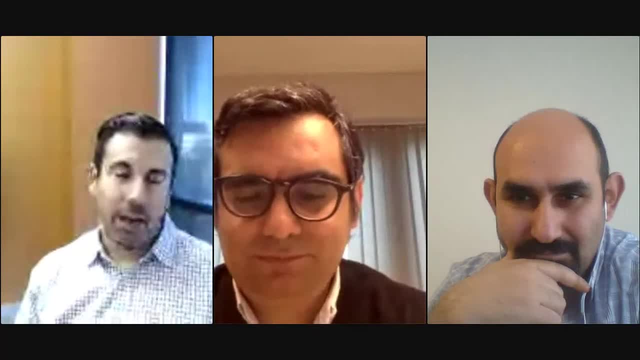 think that any, you need the crosslinker in the support bath ideally, and then you in the support bath ideally, and then you in the support bath ideally, and then you know, you know as long as it gels. know, you know as long as it gels. 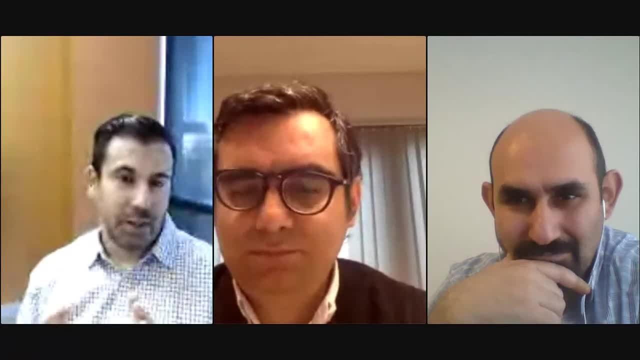 know. you know, as long as it gels, rapidly. or you're good to go now, you rapidly, or you're good to go now, you rapidly, or you're good to go now. you can print other materials that don't gel. can print other materials that don't gel. 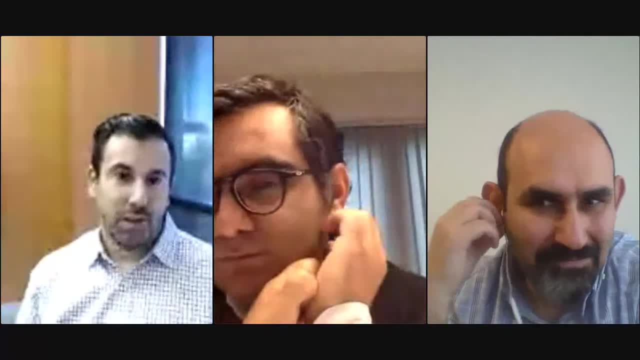 can print other materials that don't gel rapidly. if they're not missable in the rapidly, if they're not missable in the rapidly, if they're not missable in the. in the support bath: right, so we can. in the support bath, right, so we can. 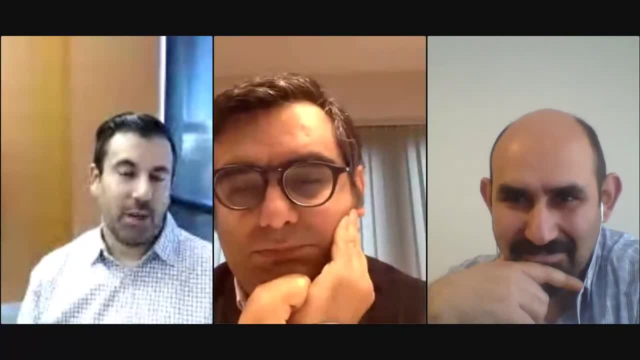 in the support bath. right, so we can print PDMS, for example, even though it's print PDMS, for example, even though it's print PDMS, for example, even though it's not cured because it's so hydrophobic- not cured because it's so hydrophobic. not cured because it's so hydrophobic. it's not gonna go anywhere, it just stays. it's not gonna go anywhere, it just stays. it's not gonna go anywhere, it just stays where you put it. so there are other where you put it, so there are other. 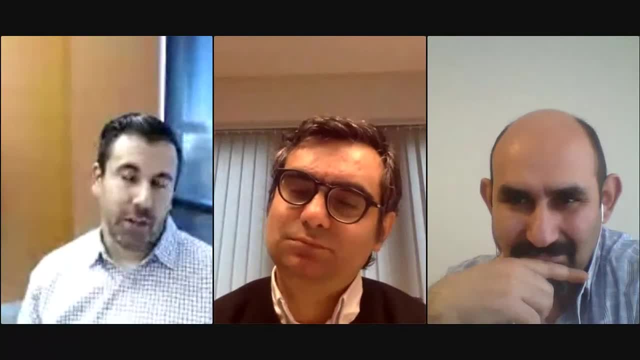 where you put it. so there are other biomaterials you potentially print as biomaterials. you potentially print as biomaterials. you potentially print as well. and we actually have some work. well, and we actually have some work well, and we actually have some work we're doing on a soft robotics project. 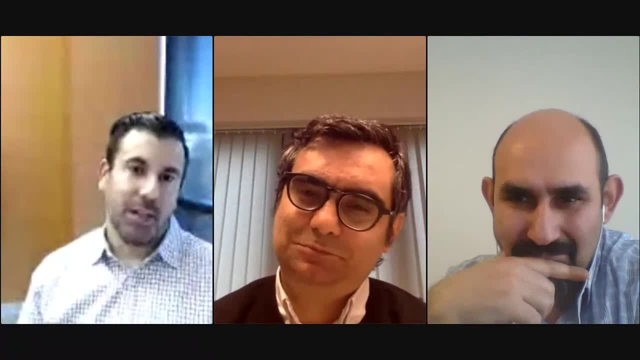 we're doing on a soft robotics project. we're doing on a soft robotics project where we're printing cells and PDMS in, where we're printing cells and PDMS in, where we're printing cells and PDMS in the same system to build like a little. 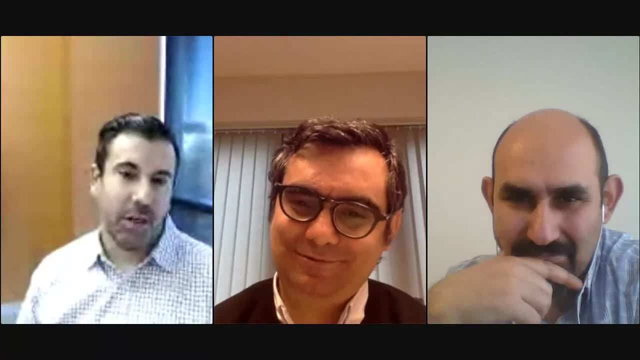 the same system to build like a little. the same system to build like a little soft robotic type device, that's muscle soft robotic type device, that's muscle soft robotic type device, that's muscle powered, so that if that is feasible, so powered, so that if that is feasible, so 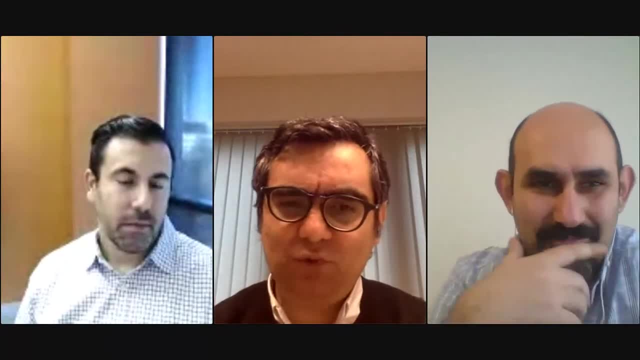 powered so that, if that is feasible, so cool that's interesting. but speaking of cool, that's interesting. but speaking of cool, that's interesting. but speaking of diffusing of the diffusion challenge, diffusing of the diffusion challenge, diffusing of the diffusion challenge with the, with the buying you mentioned, 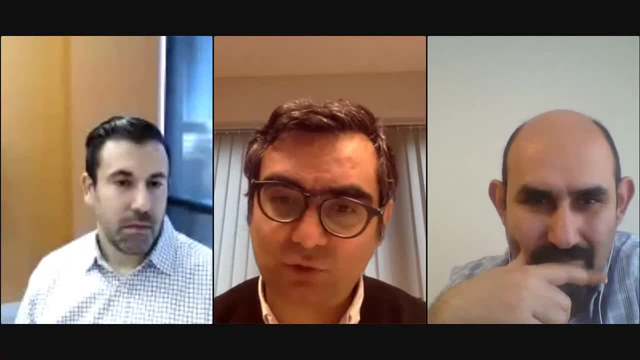 with the, with the buying you mentioned, with the. with the buying, you mentioned that you incorporated growth factors in that you incorporated growth factors, in that you incorporated growth factors in your buying. have you had any issues your buying? have you had any issues your buying? have you had any issues with the diffusion of budget, for example? 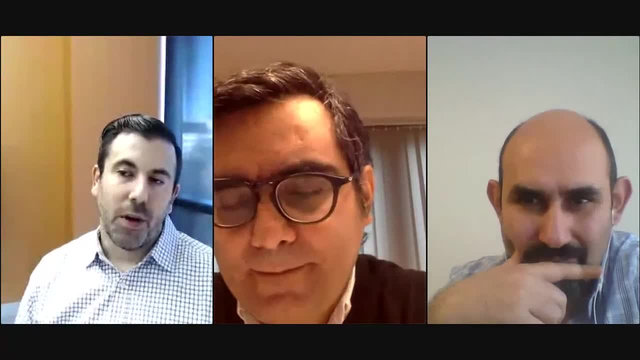 with the diffusion of budget, for example. with the diffusion of budget, for example, from the buying into the into the bath, from the buying into the into the bath, from the buying into the into the bath. yeah, it's a good question, so we. yeah, it's a good question, so we. 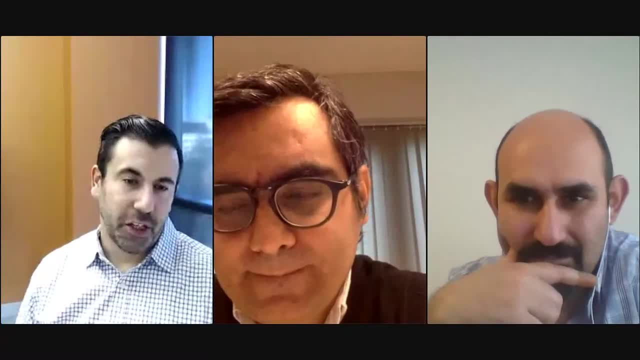 yeah, it's a good question. so we typically use something to help with. typically use something to help with. typically use something to help with that. so in the case of that Jeff and that. so in the case of that Jeff and that. so in the case of that Jeff and PDGF, it's fibronectin. so if I react and 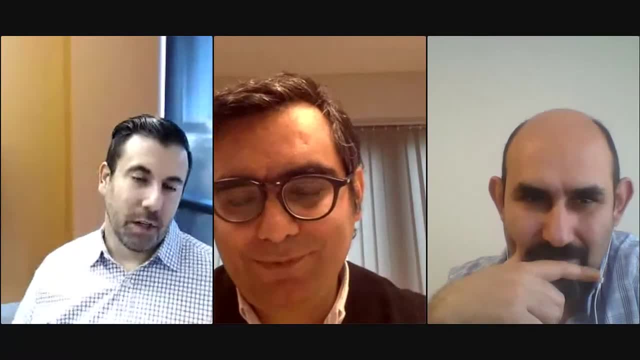 PDGF it's fibronectin. so if I react and PDGF it's fibronectin, so if I react and it's kind of acting as our glue, if you it's kind of acting as our glue, if you it's kind of acting as our glue, if you will, to help you know. you know if I will to help you know you know if I will to help you know. you know if I read: combines the collagen. the growth read combines the collagen. the growth read combines the collagen. the growth factors behind the fibronectin it does. factors behind the fibronectin: it does. 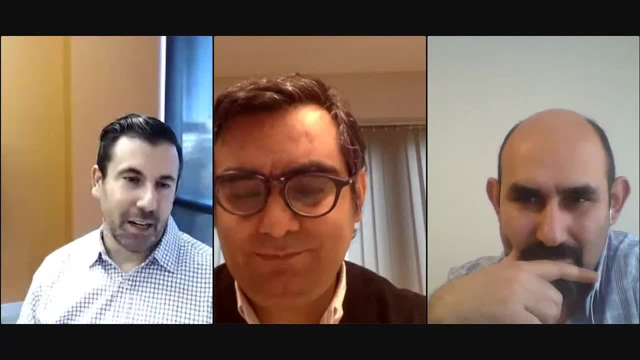 factors behind the fibronectin. it does help retention. we haven't rigorously help retention. we haven't rigorously help retention. we haven't rigorously quantified it. I guarantee you we're quantified it. I guarantee you we're quantified it. I guarantee you we're losing some, obviously, but that's that's. 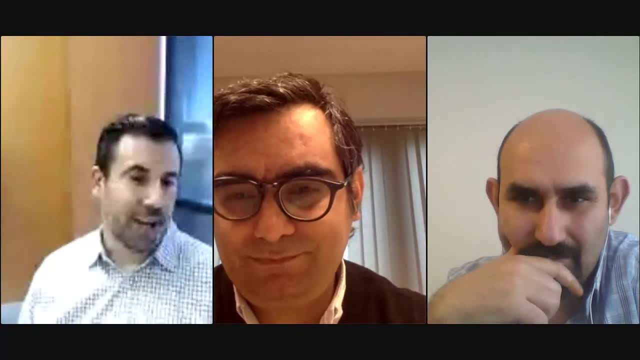 losing some obviously, but that's that's losing some obviously, but that's that's one way we do it. you could obviously one way we do it. you could obviously one way we do it. you could obviously also also tether it using other kinds of. also also tether it using other kinds of. 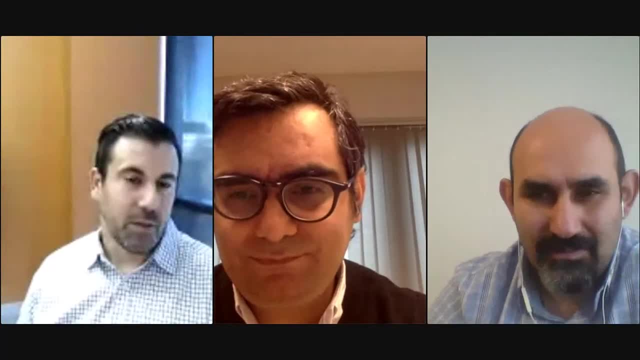 also also tether it using other kinds of chemistry is more more directly into the chemistry, is more more directly into the chemistry, is more more directly into the system. so, but that's the approach we've system. so, but that's the approach we've system. so, but that's the approach we've taken so far. we've also done a lot with. 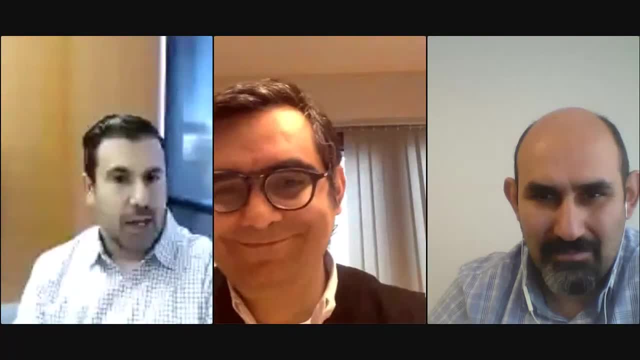 taken. so far. we've also done a lot with taken. so far. we've also done a lot with the decellularized matrix. because you the decellularized matrix, because you the decellularized matrix, because you know most decellularized matrix is, know most decellularized matrix is. 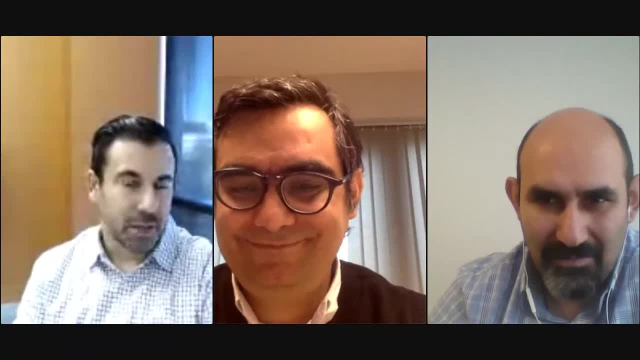 know, most decellularized matrix is mostly collagen. so it prints with the mostly collagen, so it prints with the mostly collagen, so it prints with the same basic gelation mechanism, as a same basic gelation mechanism, as a same basic gelation mechanism as a collagen. and you know, in that case we do. 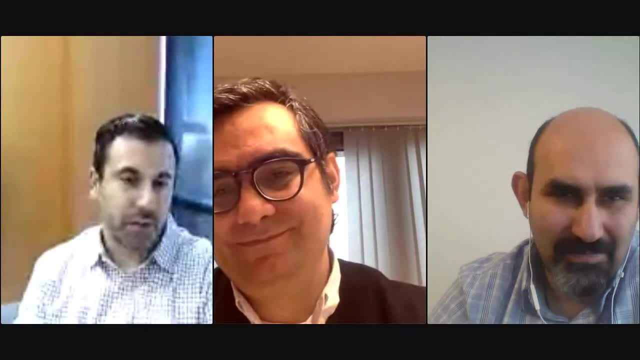 collagen. and you know, in that case we do collagen. and you know, in that case we do retain a lot of what we're printing, but retain a lot of what we're printing, but retain a lot of what we're printing, but obviously some of it you do lose through. 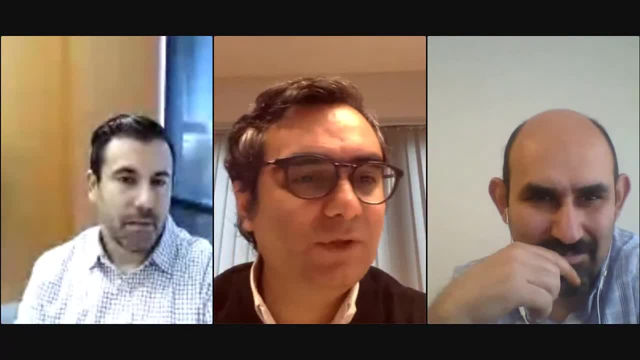 obviously some of it you do lose through. obviously some of it you do lose through diffusion: mm-hmm cool, good. yeah, just to diffusion. mm-hmm cool. yeah, just to diffusion. mm-hmm cool. yeah, just to add to dr Feinberg comment: just follow up. 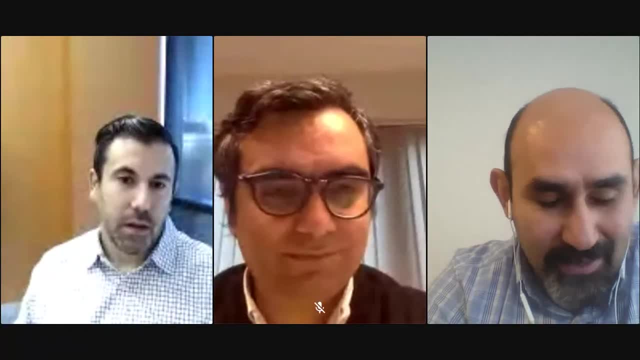 add to dr Feinberg comment. just follow up. add to dr Feinberg comment. just follow up. we use the the fresh print printing. we use the the fresh print printing. we use the- the fresh print printing technology to print the bio elastomers technology to print the bio elastomers. 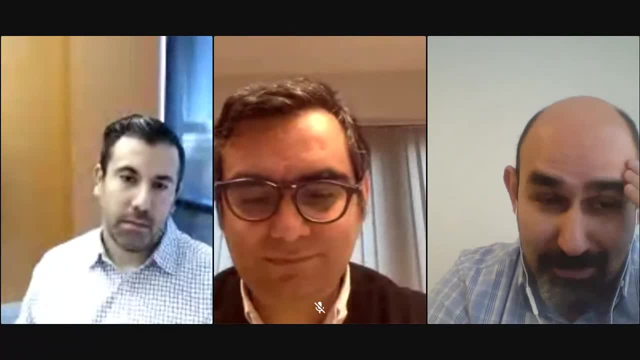 technology to print the bio elastomers, polyester based by elastomer. so since polyester based by elastomer, so since polyester based by elastomer. so since that the by elastomer was like was not that the by elastomer was like was not that the by elastomer was like was not rapid, cross-linkable big movie. so we 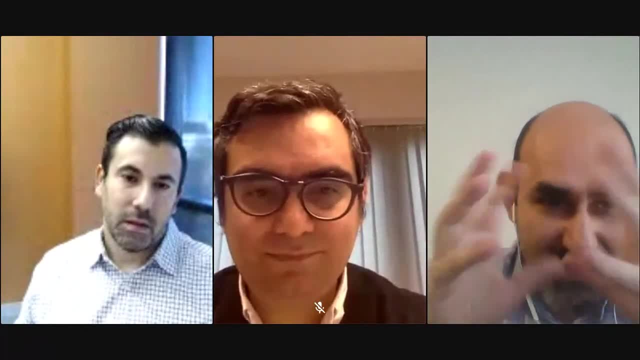 rapid, cross-linkable big movie. so we rapid, cross-linkable big movie, so we just try to you know, integrate it in the. just try to you know, integrate it in the. just try to you know, integrate it in the hydrogen, keep it and later on shine UV. 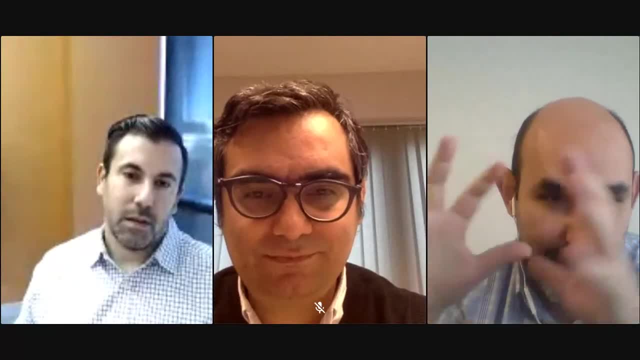 hydrogen- keep it and later on shine UV. hydrogen- keep it and later on shine UV, and then it keeps the structure in hand, and then it keeps the structure in hand, and then it keeps the structure in hand intact after we wash out the acrylic intact. after we wash out the acrylic. 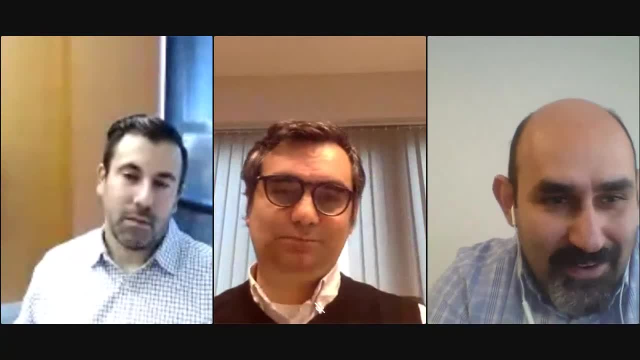 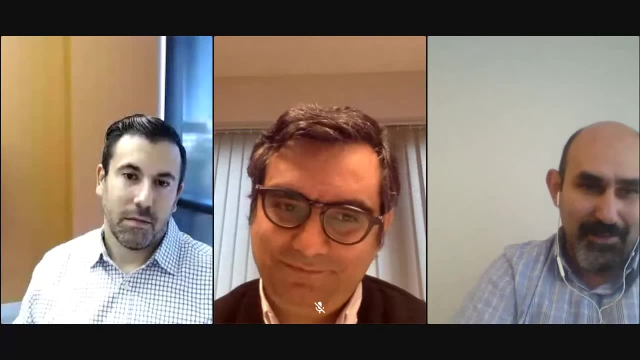 intact after we wash out the acrylic base, the other kind of you know base, the other kind of you know base, the other kind of you know hydrogen, and then then then gelatin, so hydrogen, and then then then gelatin, so hydrogen, and then then then gelatin. so it's pretty like you know very, very 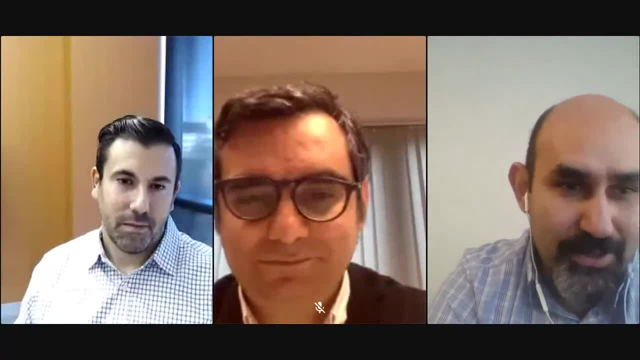 it's pretty like you know very, very. it's pretty like you know very, very versatile technique to do different. you versatile technique to do different. you versatile technique to do different. you know by materials, as you mentioned. we know by materials, as you mentioned. we know by materials, as you mentioned. we just just just to add that, yeah, that's. 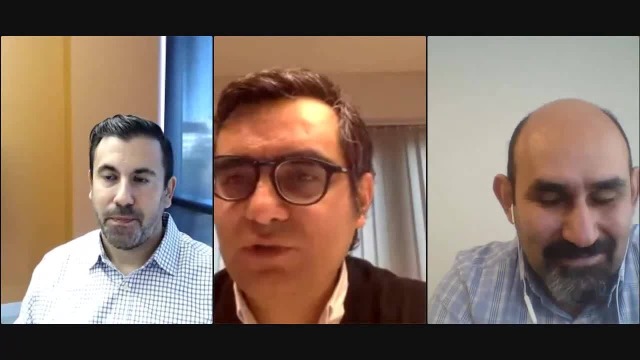 just just to add that. yeah, that's just just to add that. yeah, that's great, so we're running out of time. it's great, so we're running out of time. it's great, so we're running out of time. it's almost 1030 Pacific time and I'm sure 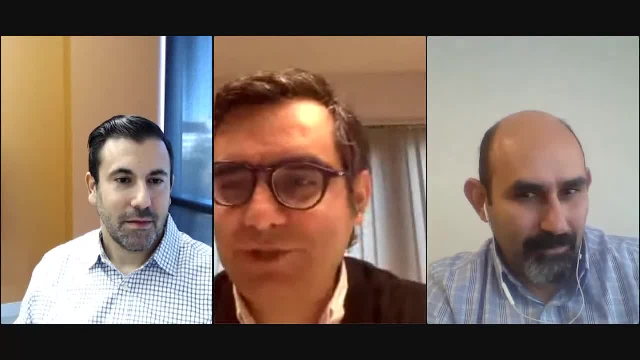 almost 1030 Pacific time and I'm sure almost 1030 Pacific time and I'm sure dr Feinberg also he's busy. I mean he's dr Feinberg also, he's busy. I mean he's dr Feinberg also he's busy. I mean he's running to two teams. one is his lab. 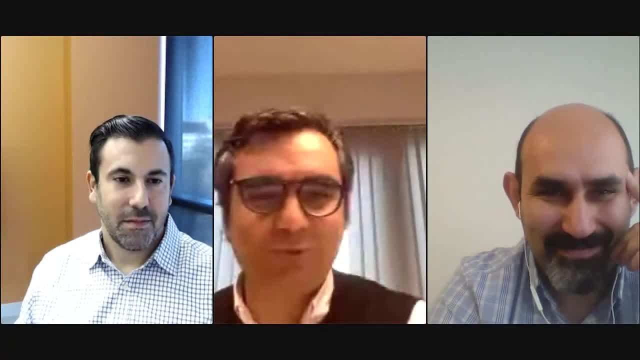 running to two teams. one is his lab running to two teams. one is his lab, which is you saw many, many students are, which is you saw many, many students are, which is you saw many, many students are working with him, and then also he is working with him and then also he is. 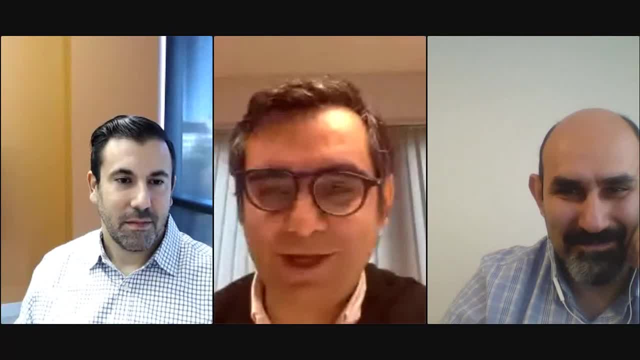 working with him and then also he is: he is the CTO of a company, so it keeps him. he is the CTO of a company, so it keeps him. he is the CTO of a company, so it keeps him. like that position also keeps him. like that position also keeps him. 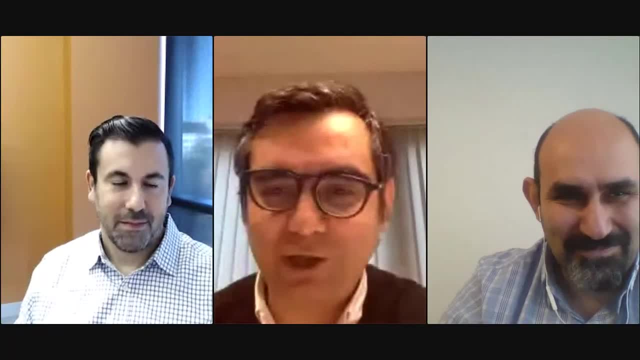 like that position also keeps him pretty busy. I have the same situation pretty busy. I have the same situation pretty busy. I have the same situation and I don't know how you guys handle and I don't know how you guys handle and I don't know how you guys handle. this is many things because I can't. I 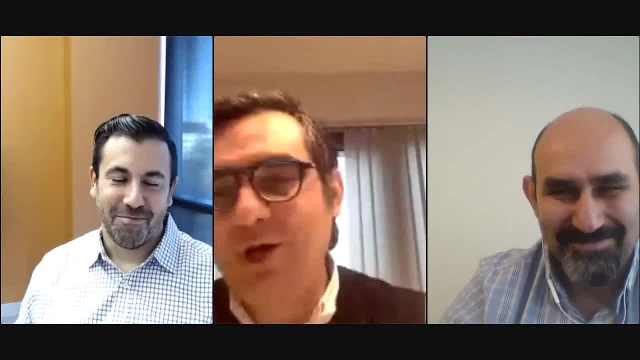 this is many things because I can't I. this is many things because I can't. I mean that, so so with that. I would like mean that, so so with that, I would like mean that, so so with that. I would like to thank our speaker, dr Feinberg, for. 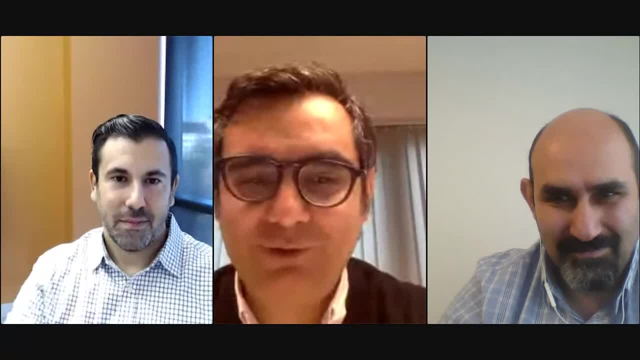 to thank our speaker, dr Feinberg, for to thank our speaker, dr Feinberg, for his amazing talk. it's always great to his amazing talk. it's always great to his amazing talk. it's always great to hear the new technologies and the new. 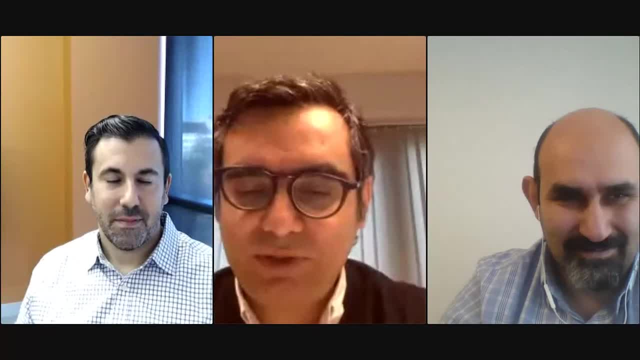 hear the new technologies and the new. hear the new technologies and the new advancement that you're making in the advancement that you're making in the advancement that you're making in the field of 3d by printing and particular field of 3d by printing and particular. 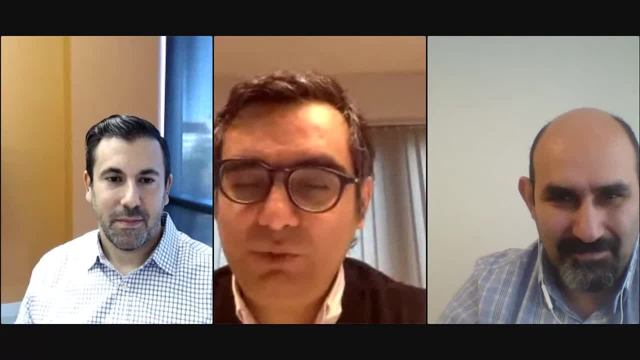 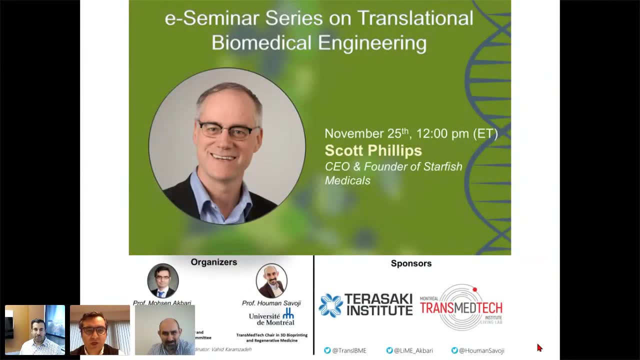 field of 3d by printing, and particular cardiac tissue engineering. thank you, and cardiac tissue engineering, thank you, and cardiac tissue engineering, thank you. and also, I would like to remind everyone also, I would like to remind everyone, also, I would like to remind everyone that our next speaker is mr Scott. 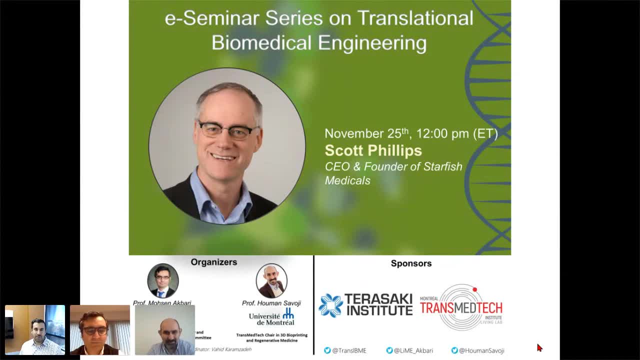 that our next speaker is mr Scott. that our next speaker is mr Scott Phillips, the CEO and founder of Phillips. the CEO and founder of Phillips, the CEO and founder of starfish medicals, one of the largest starfish medicals. one of the largest starfish medicals, one of the largest biotech companies in in Canada also, I 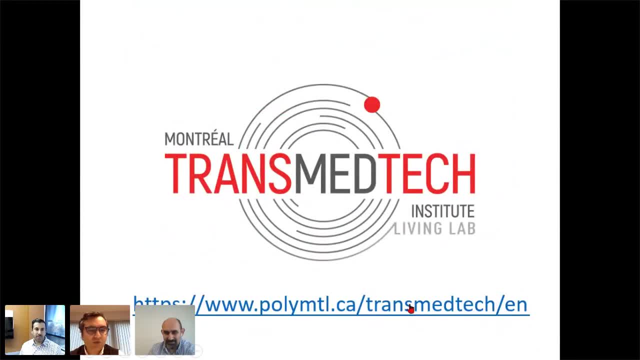 biotech companies in in Canada also. I biotech companies in in Canada also. I would like to thank our sponsors, would like to thank our sponsors. would like to thank our sponsors: Montreal transmit tech and selling for Montreal transmit tech and selling for Montreal transmit tech and selling for supporting, for always supporting us. 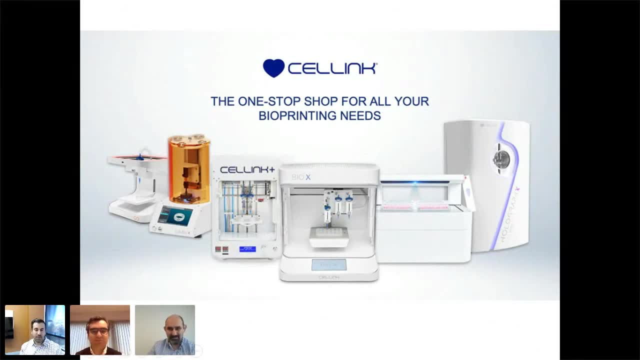 supporting for always supporting us, supporting for always supporting us, especially selling. who supported this, this, especially selling. who supported this, this, especially selling. who supported this, this presentation. so with that also, I presentation. so with that also, I presentation. so with that also, I would like to thank the participants and 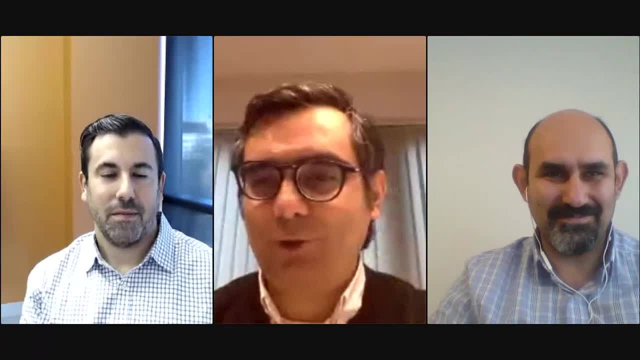 would like to thank the participants. and would like to thank the participants and then wish you all a great day or night. then wish you all a great day or night. then wish you all a great day or night. ahead of you, take care. thank you so much. ahead of you, take care. thank you so much. 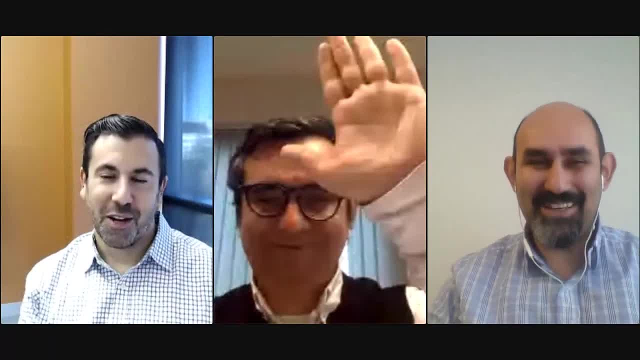 ahead of you take care. thank you so much. thank you both really appreciate it. thank you both really appreciate it. thank you both really appreciate it. thank you everyone. thank you everyone. thank you everyone. 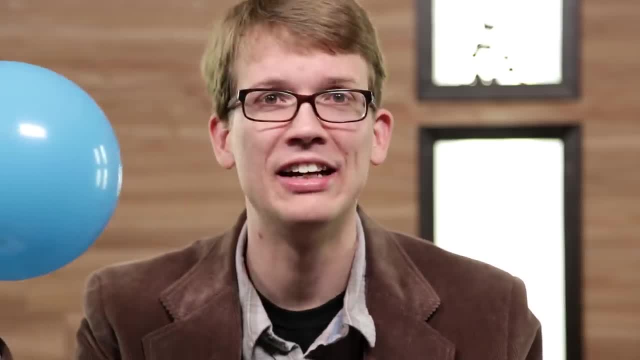 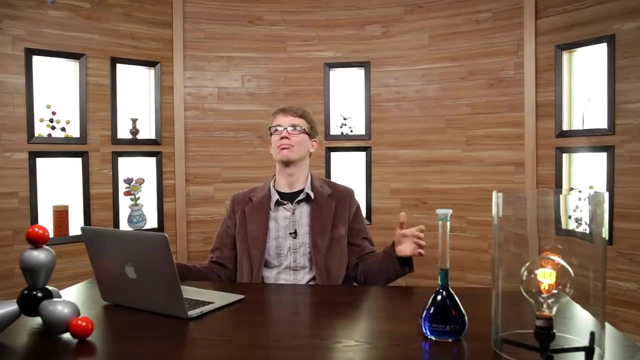 Gas. It's all around you, It's in space, It's on Mars, It's dissolved in your blood and in your soda. It's everywhere And it's easy to forget that we're submerged in an ocean of gas, but it's there all the time. You can feel it if you wave your arms around.